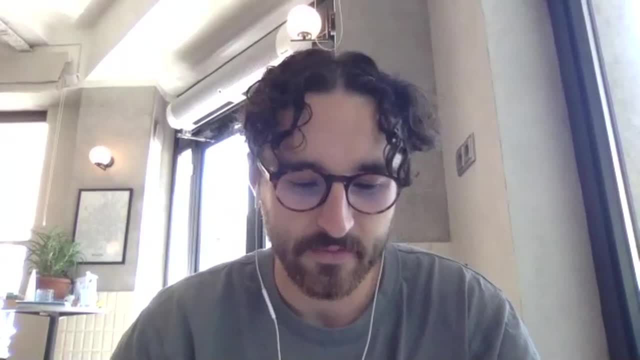 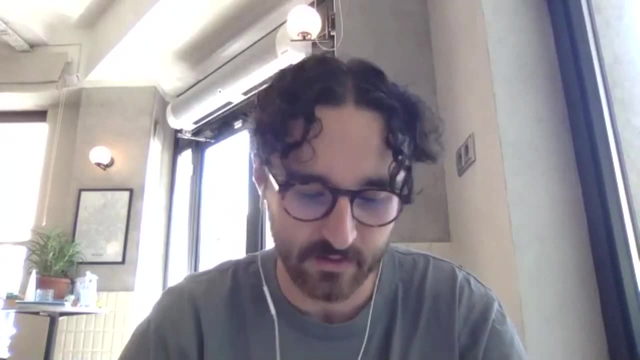 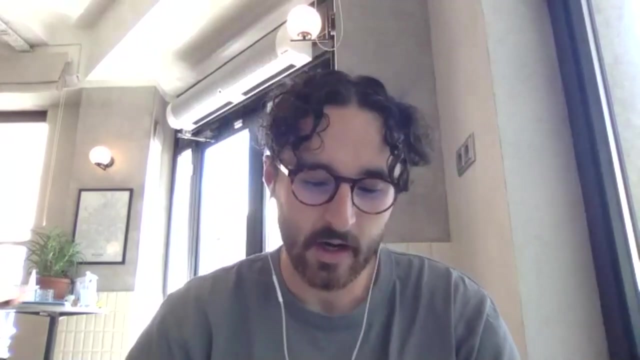 have now quite a sizable industry. This became really fascinating to me and particularly in the last few months I've been very dedicated to learning about this field. I'm now writing this article for National Geographic, As I think you all know, and the angle of my article is looking specifically at how Artemia 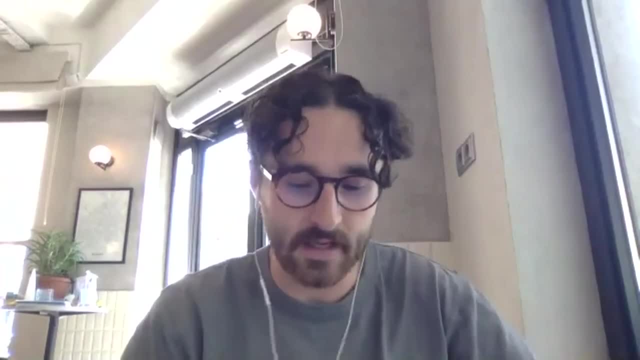 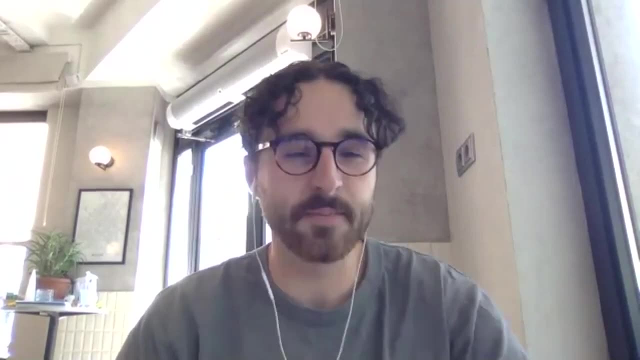 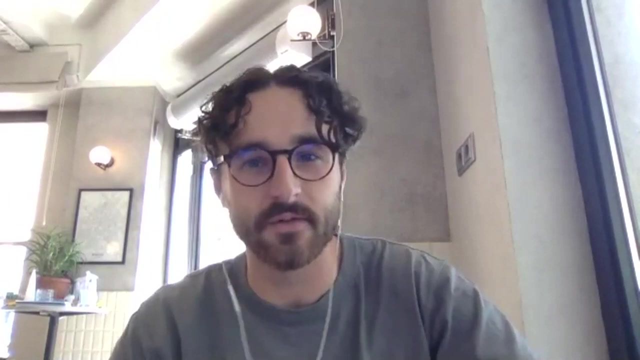 can be an alternative economic resource- and already is- for communities that are grappling with climate change and water management issues, And at this moment in time, my reading and my learnings have been more focused on the Aral Sea region and GSL, so it's really really exciting for. 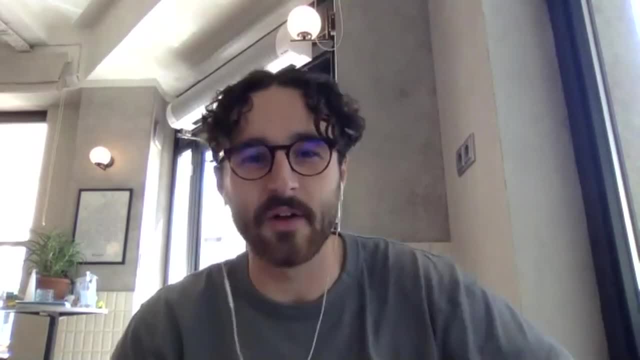 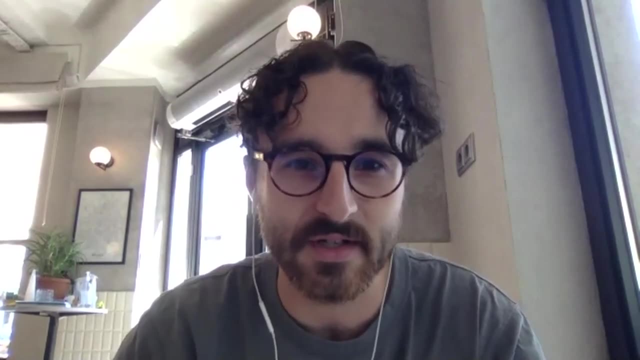 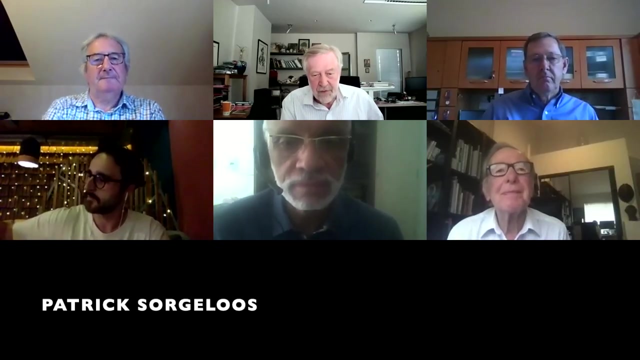 me to be speaking with so many different people from around different areas of the world And to hear about how Artemia is operating in all of your countries. So, without further ado, I will pass the floor on. I retired in 2013 from Ghent University as a professor of aquaculture. I got involved. 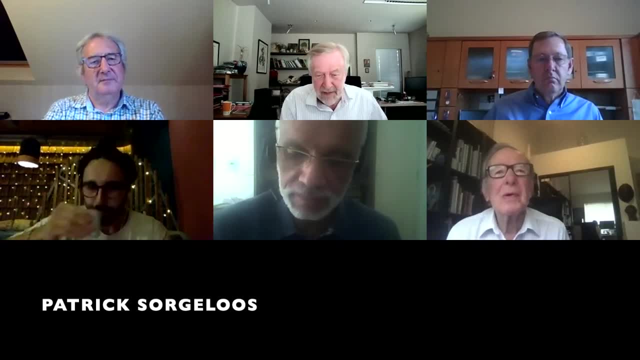 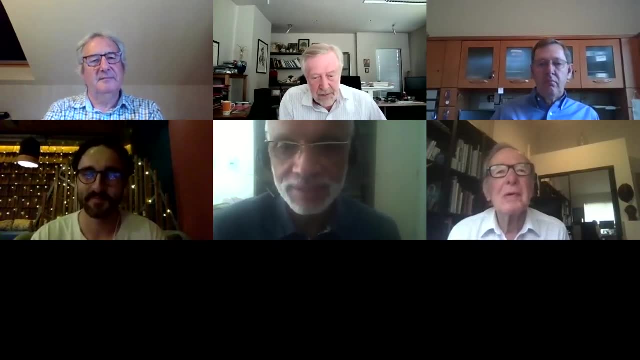 with Artemia research. yeah, ever since 1969, but we will hear from some other person who started even earlier, First for my MSc and PhD studies with Artemia and later. I must say that I have been working with a fantastic team of co-workers in Ghent and colleagues. 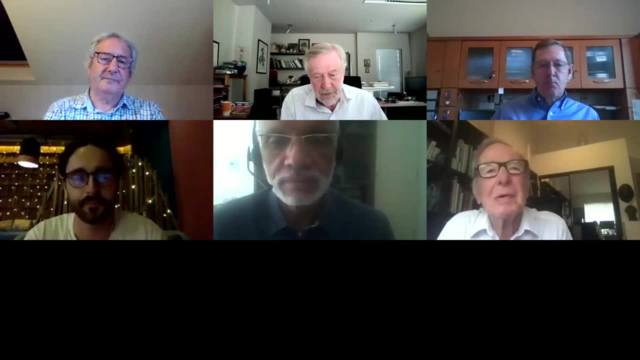 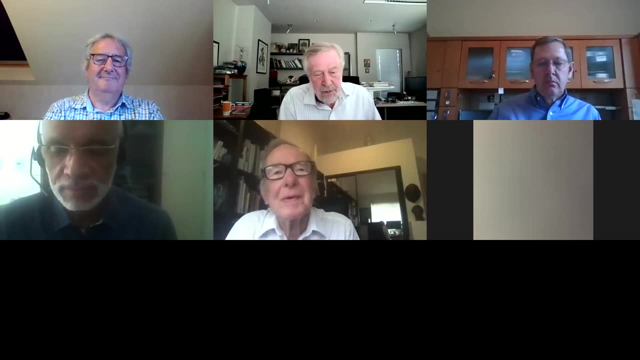 from all over the world in research and development aspects of Artemia. I enjoy my retirement and I try to help and facilitate new developments with Artemia and in aquaculture, but I wish I was 30 years younger, As we live in very exciting times for more research and applications. 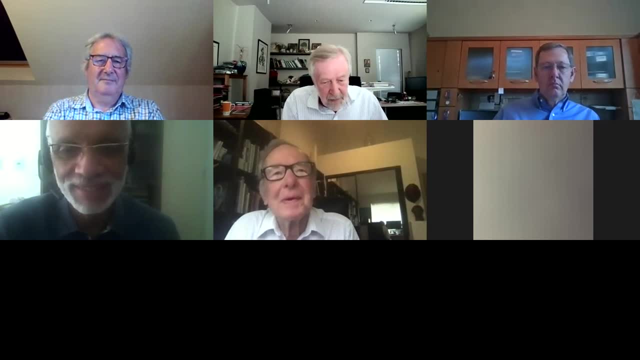 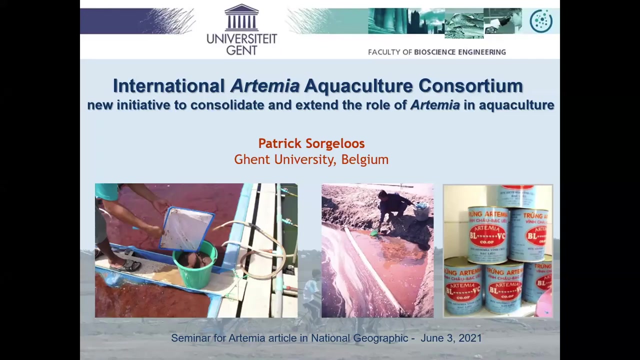 with Artemia, As we will hear in the next few days. Thank you, Saxon, for showing so much interest in Artemia to prepare an article for National Geographic. I will share the screen and I will start with my presentation. So my presentation. 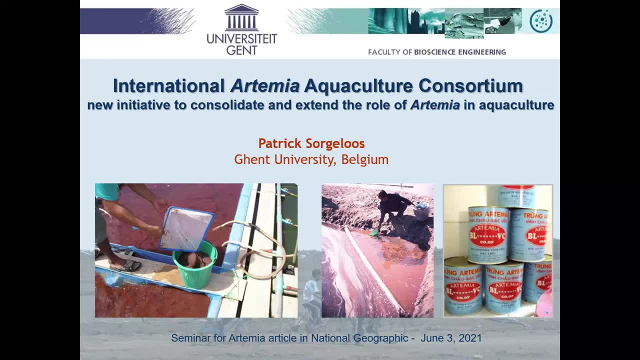 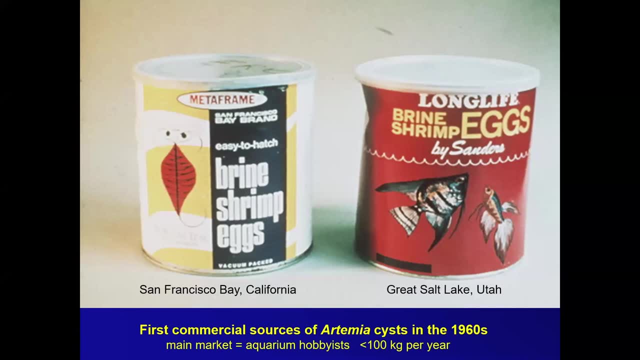 will deal with the new initiative, the International Artemia Aquaculture Consortium, And to bring it in perspective. we are starting back in 1960s, when only two sources in the United States were used, And the first source was in fact the aquarium hobbyist. It was quickly thereafter that the 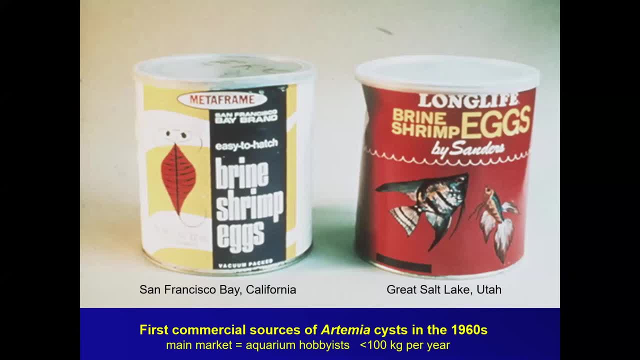 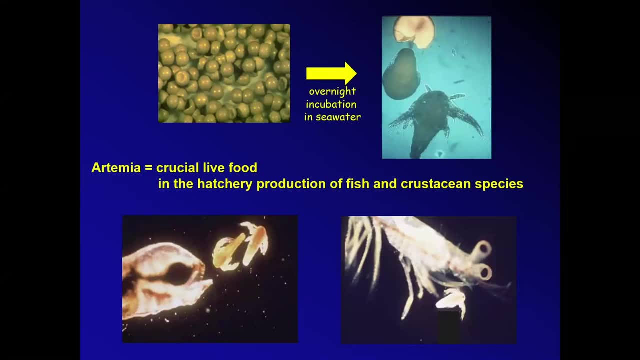 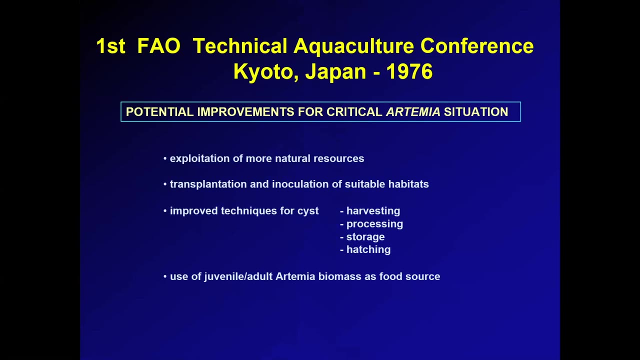 Japanese were the first to see that for modern aquaculture and hatchery production that Artemia could be used as a very ideal replacement for plankton in feeding all kinds of larval stages of fish and crustaceans. But in 1976, when FAO was organizing the first Technical Conference on aquaculture, it turned. 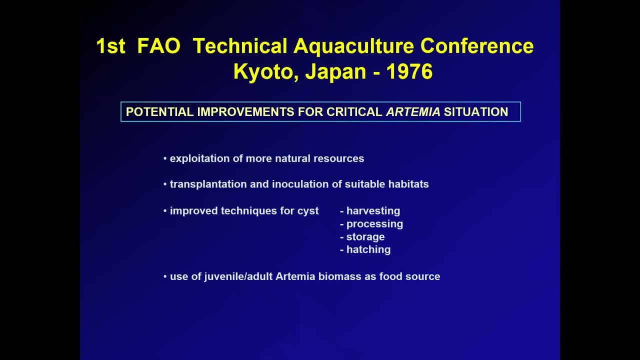 out that it was very risky because it would be very dangerous to see the formation of new species and the development of a new ecosystem. It was very interesting Because, first of all, it was very risky, And so when the United States first announced the concept of agency, that 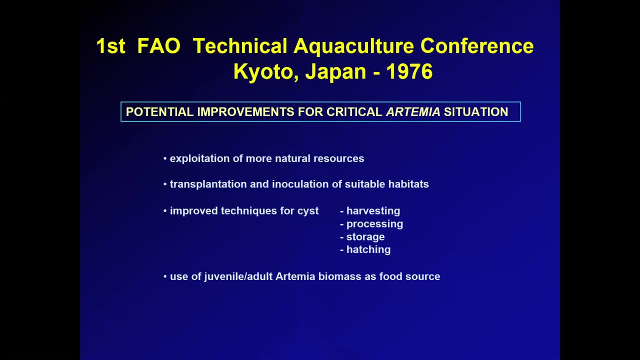 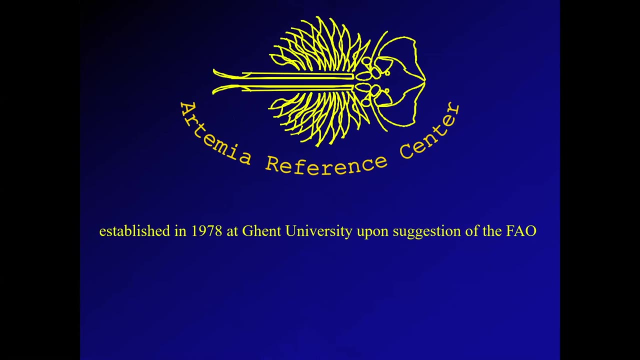 to develop a new aquaculture system with the hatcheries when you have to depend only on sources from one single country. So this is where we tried to explain that there were opportunities for other sources, other developments and, upon suggestion of the FAO, in 1978 we set up the 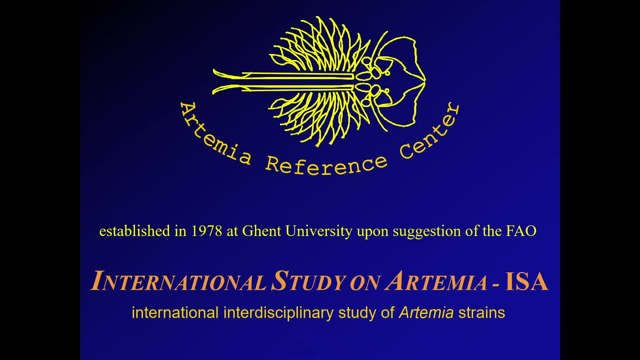 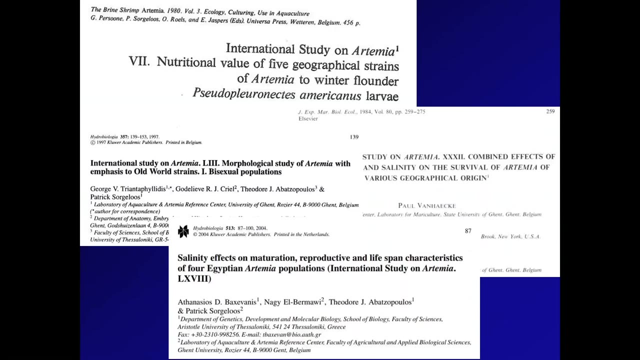 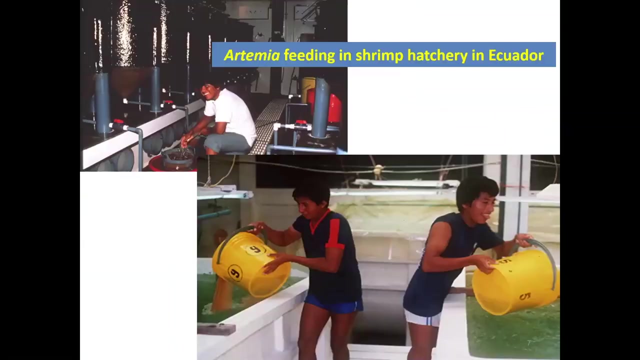 Artemia Reference Center and, most important, was that right from the setup, we were looking into the possibility to bring scientists together in different disciplines to look for solutions in using Artemia, And many, many papers, manuals, handbooks, conferences were organized which indeed resulted in improved utilization of Artemia from different sources. 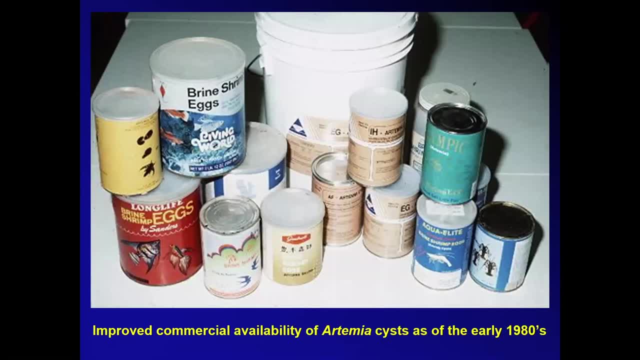 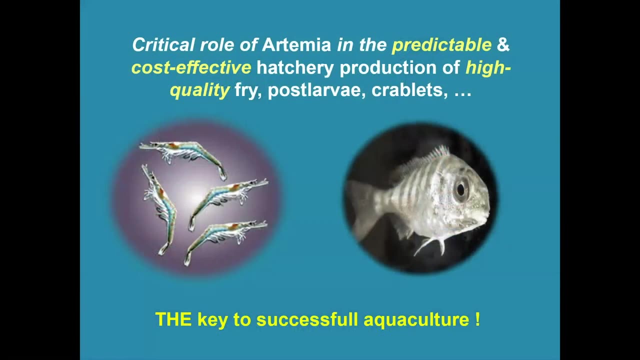 as we went forward. We will hear in the next presentations So quickly. we have seen already in the 1980s that Chinese, Australian, Brazilian, different new sources of Artemia came in the market. But that was also at the time that we have seen a real- I can call it an explosion of hatchery activity with different 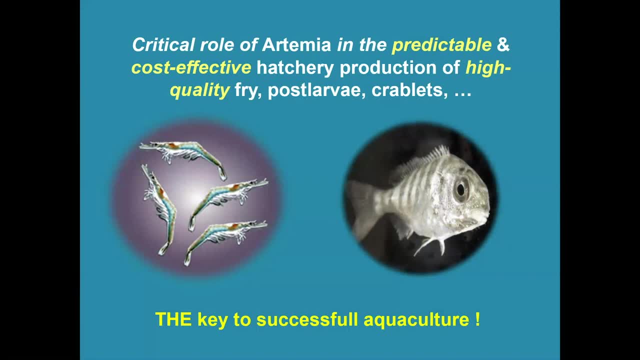 crustacean and fish species And, as you see at the bottom of the screen here, even today, we can still say that the key to successful aquaculture is the availability of hatcheries, the availability of the live food sources, like Artemia for these hatcheries. With such a spectacular development, 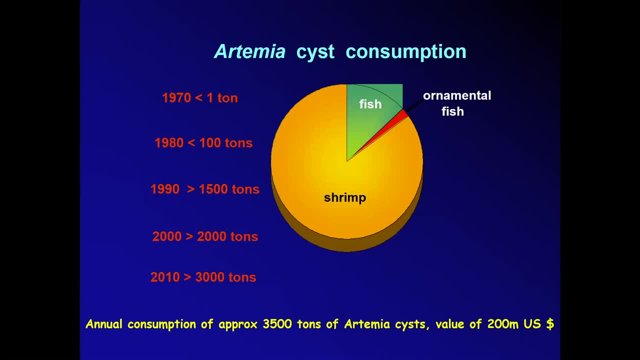 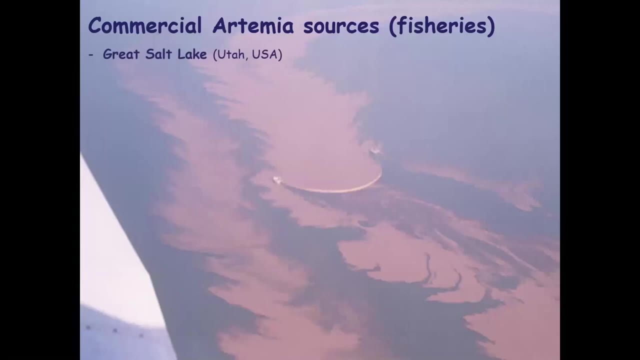 in hatchery aquaculture we have seen, indeed, also a spectacular increase in demand and, lucky enough, also offer of Artemia for feeding all these billions of fish and shrimp larvae And the commercial sources that were developed over time and again we will hear in a number of 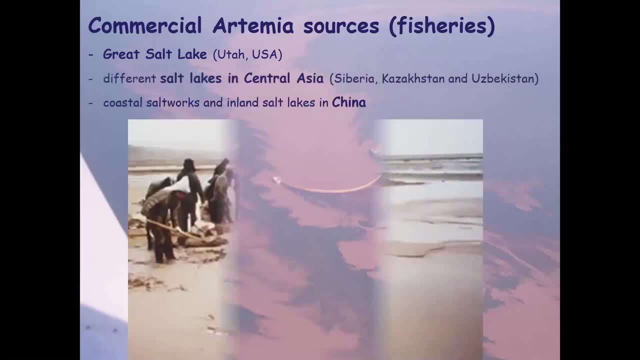 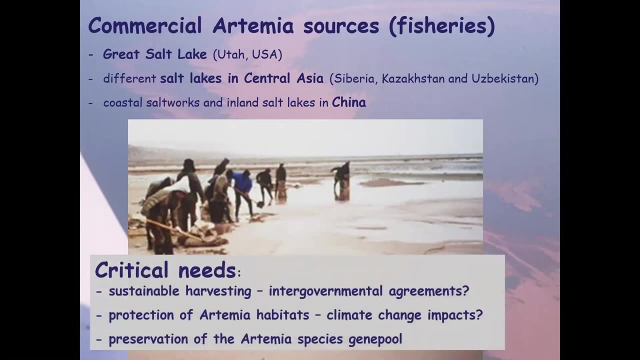 presentations that the Great Salt Lake is playing an important role. then there are a number of places in Central Asia, in China, but there are critical needs. It's very nice and fantastic to see that there has been such a development, but there are a number of issues where we need to. 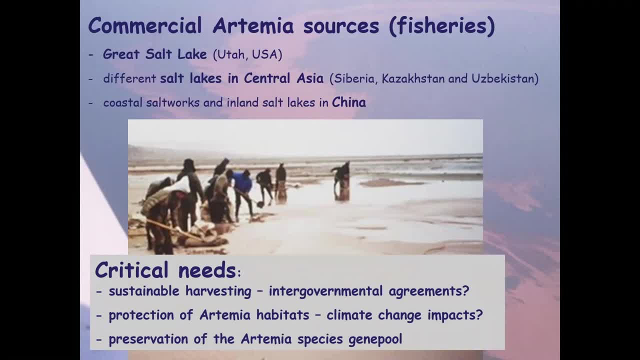 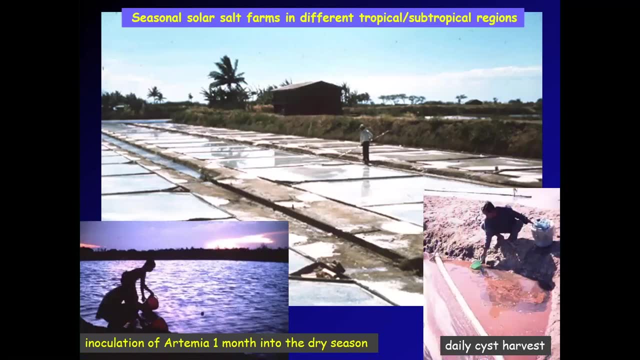 express some concern when it comes to sustainable harvesting, when it comes to the production of Artemia habitats, the preservation of the gene pool. In the meantime, we see that, next to the sources from nature, that there have been very interesting developments in producing in controlled 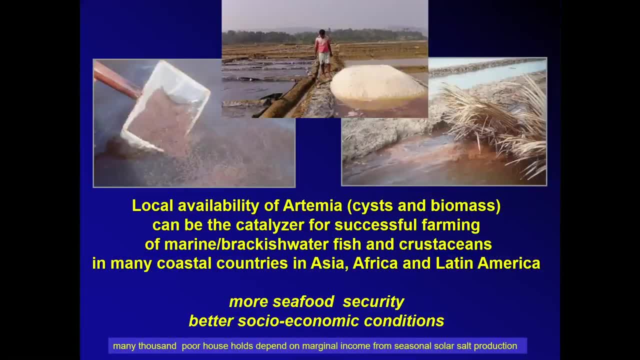 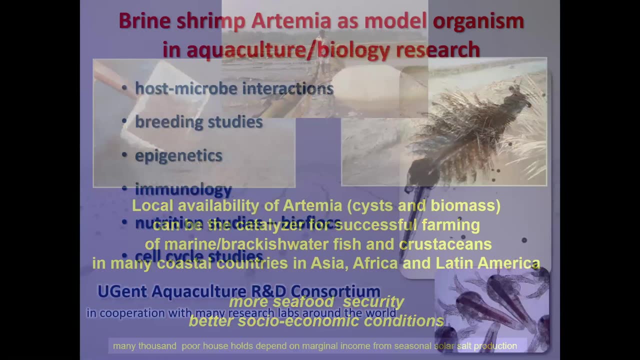 production, pond production of Artemia, And in fact in a number of countries we will hear about in the presentations tomorrow. this is a catalyzer for local new aquaculture developments, with important socio-economic development Next to that. but no time to go into the details except with also some presentations we will hear. 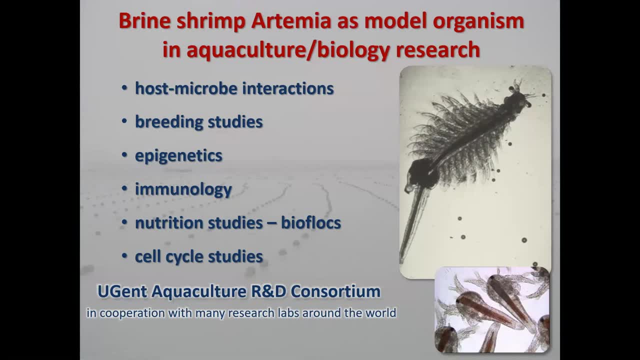 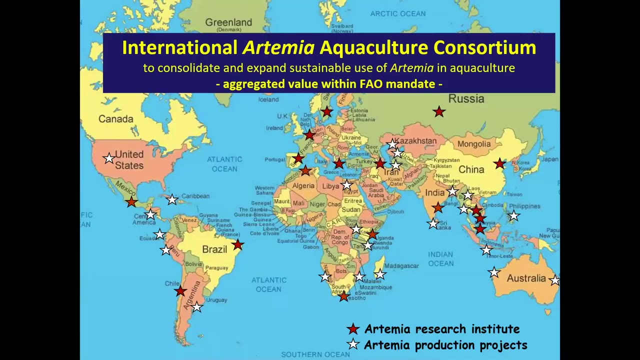 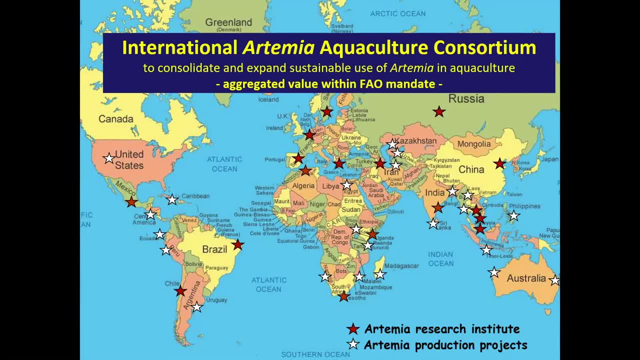 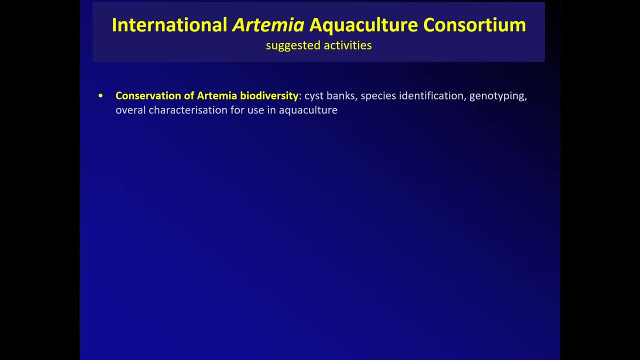 White stars representing Artemia, research institutes representing Artemia projects. There is a real world interest, and this came to the attention of the Food and Agriculture Organization- who really wants to see and support the establishment of such an international consortium, where a number of key issues that I addressed earlier and that are listed here without going. 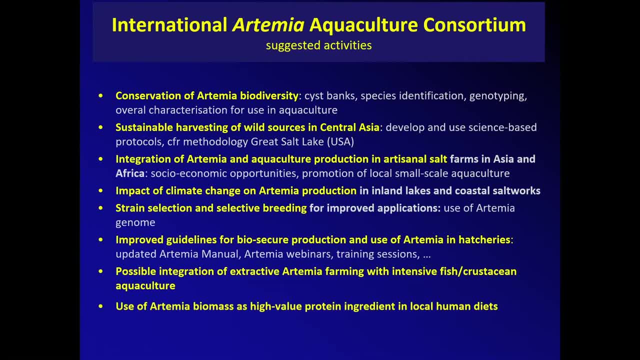 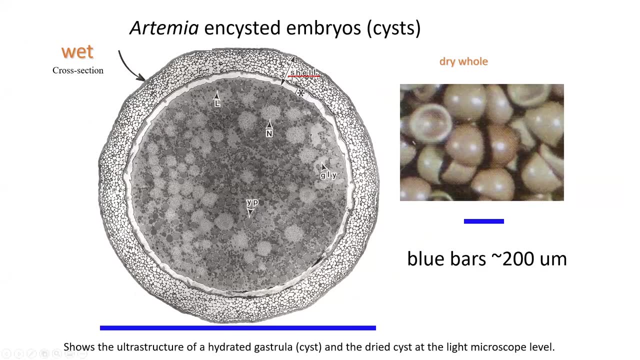 into the details Or, in fact, an opportunity to look into consolidation on one hand with Artemia on the other hand, explore new opportunities. Thank you, Yes, I am Jim Clegg. I've been interested in using Artemia as a model system for. 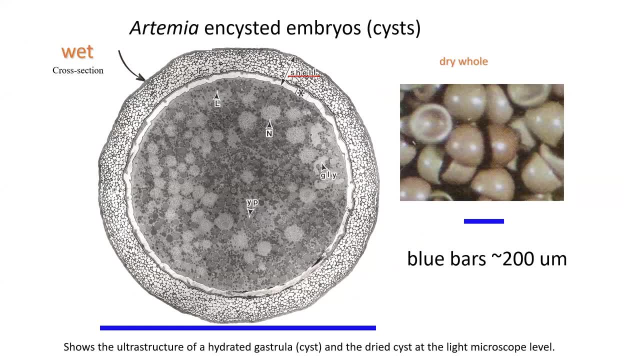 quite a few decades. Today, I'm going to address chiefly the two issues that are eclipsed. First and foremost, we talked about the subgenital, a huge variety of environmental insults. I will give one example to start, and that is its ability. 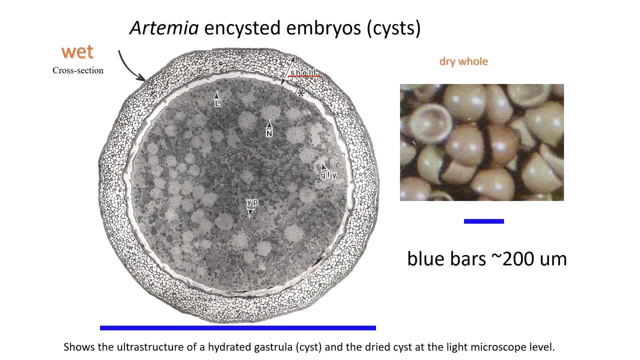 to lose virtually all of its water. All of its liquid water is lost by evaporation without killing the embryo, And I've been interested in trying to understand how this embryo does something that kills the vast majority of animals of any stage Right. Very few creatures can. 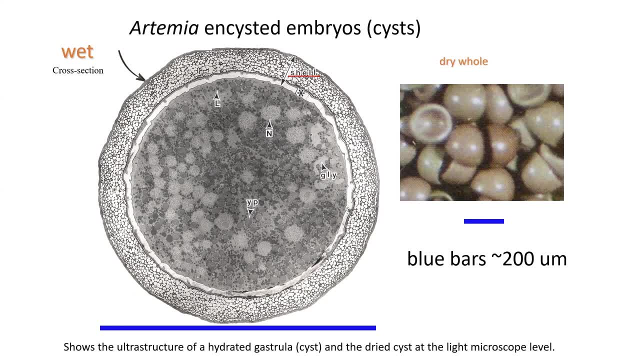 withstand total desiccation, as artemia can, And that's why I said some years ago that we should consider the brine shrimp artemia as an animal extremophile, because it has this astonishing ability to withstand stresses of various kinds. To the right, you see the dried cyst. It's very difficult. We found it. 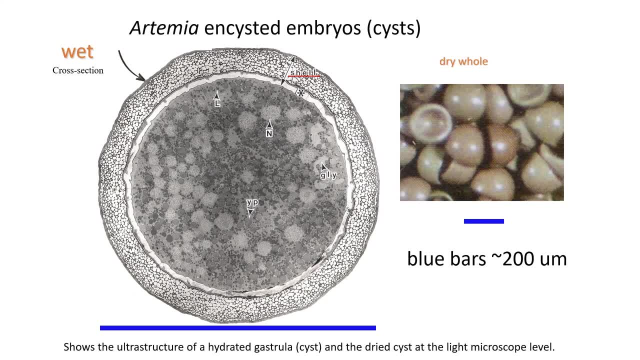 impossible to get electron microscope images of the dried embryos, But at the light microscope level they are amorphous, They seem to disappear into a background, And I'll give you a reason to suspect that we know what that is Okay. Central to artemia's abilities of various kinds is a disaccharide. 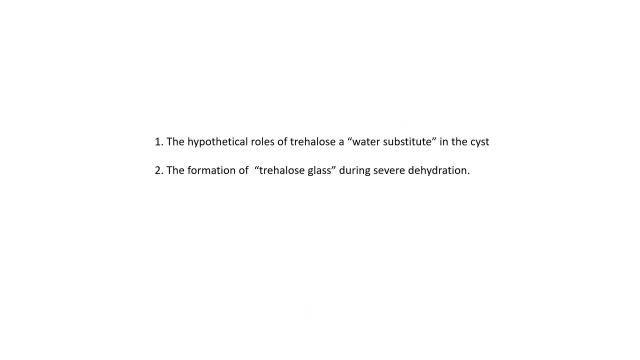 called trehalose. It's a molecule consisting of two glucose molecules hooked together and themselves, And they always return to their original location. And if you remove this molecule you can see that they have separated out very small sections of the blood and there's no way for. 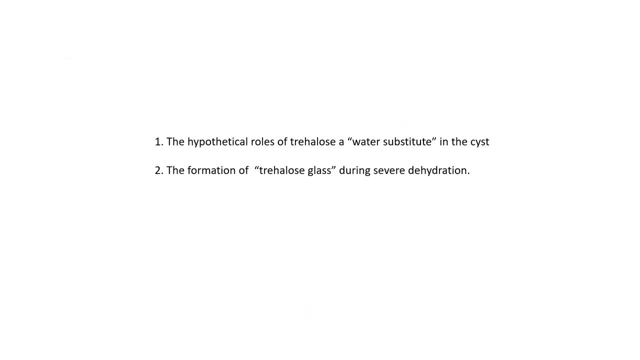 them to be together in a certain way. And this trehalose, we believe, does two major things. that is involved with the resistance of the artemia embryo And, as the water is lost, this would normally result in the damage, denaturation of macromolecules. 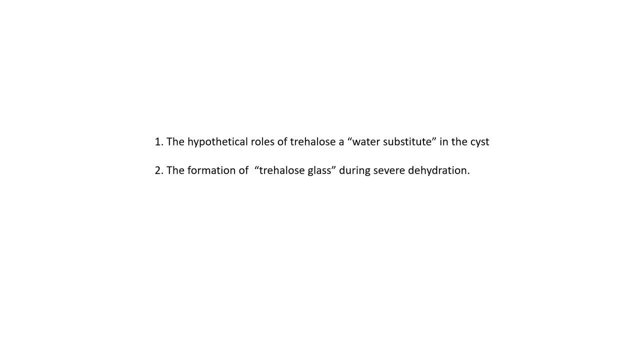 of all kinds that rely on water for stability, And that includes membranes, And of course, cells are chock full of membranes of all kinds in different organelles. Now we believe, on the basis of some evidence, not conclusive, we believe- that the trehalose 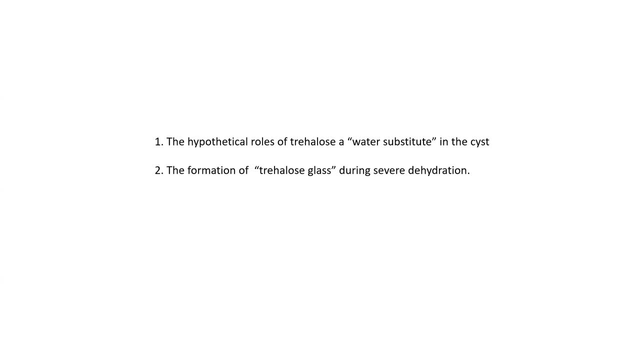 replaces the water that's lost, thereby stabilizing the macromolecules and membranes, So it is a substitute in that sense. Another function of the trehalose is to form a glass at very low water contents When the water contents get close to zero. 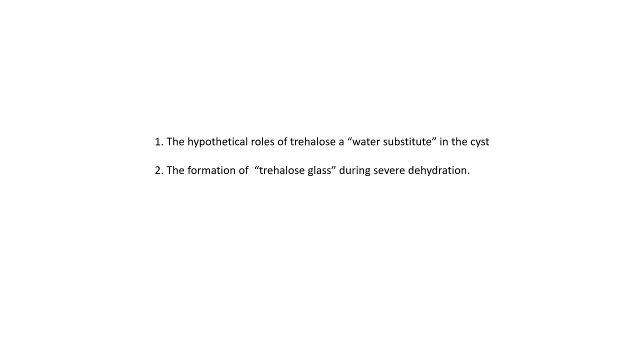 they never really get to zero but close. the trellis forms a glass And, as you all know, glass is a very stable structure in the sense that we know it. but trellis glass is also very stable and we believe, and have reason to believe. 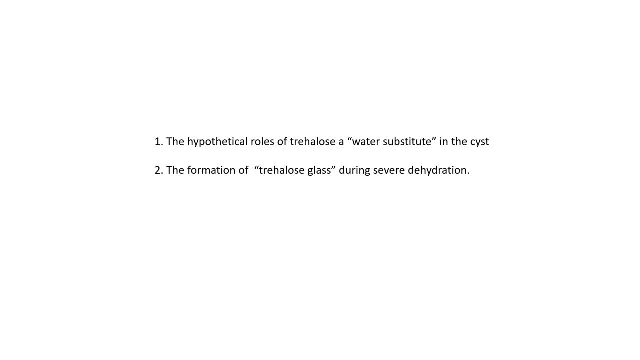 that the components of the artemia cells in the cyst get embedded in the glass, in the trellis glass, thereby becoming very stable and yet becoming reversibly functional. Okay, so the two major roles are the formation of trellis being a water substitute. 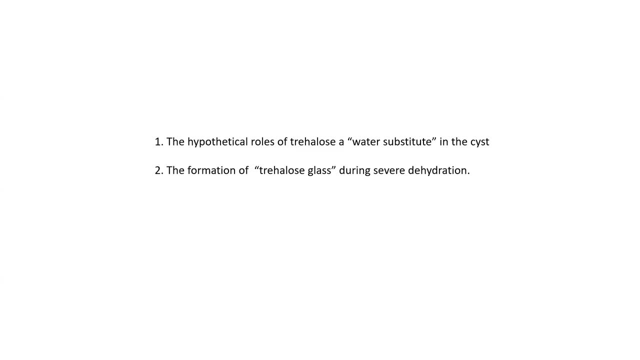 and the formation of a glass. Okay, so this molecule is very important. By the way, I don't think I mentioned that the amount of trellis in an artemia-incisted embryo is massive, about 20% of the dry weight. 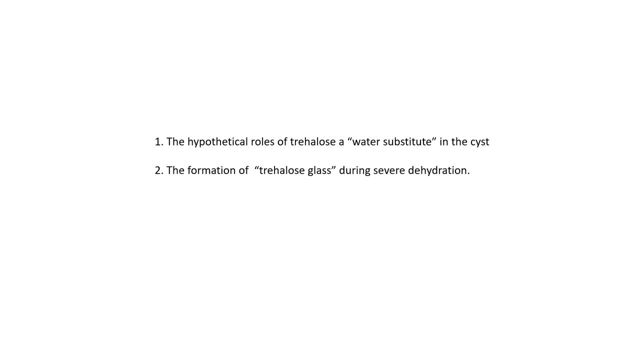 That is a huge amount of, that is a huge amount of trellis, And so the ability of the embryo to synthesize this molecule is crucial to its subsequent stability in the presence of threatening stresses. Okay, the artemia embryo also has the ability to undergo hypoxia. 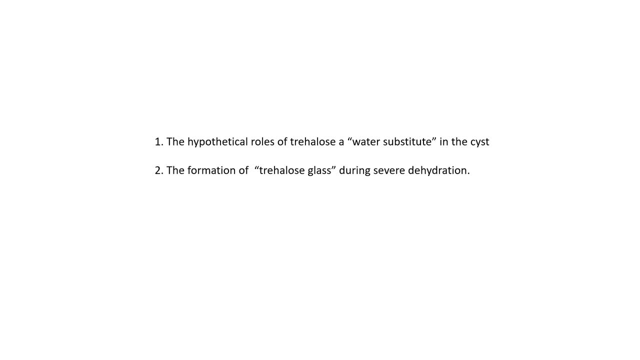 the absence of oxygen for months and months. And it does that we discovered by just stopping. It just comes to a standstill metabolically, and that's quite an achievement. In that stable state it is able to survive in the absence of oxygen for months. 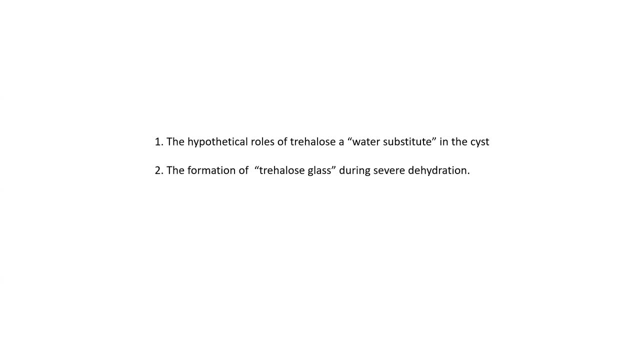 And months. We're not sure how long, but it's certainly a long time compared with other animal forms, whatever the life cycle stage we're talking about. Okay, so desiccation and resistance to oxygen lack are just two of the very impressive abilities. 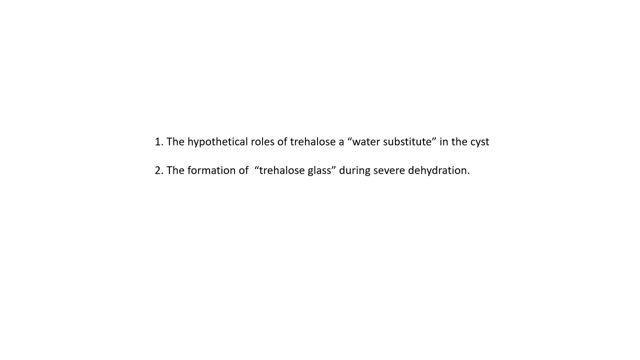 and capabilities of the insisted gastrula embryo. The embryo- if conditions are suitable, the embryo- and by that I mean adequate water and adequate oxygen. the embryo then develops and hatches from the cyst as a noplius larva. The noplius larva then undergoes subsequent growth. 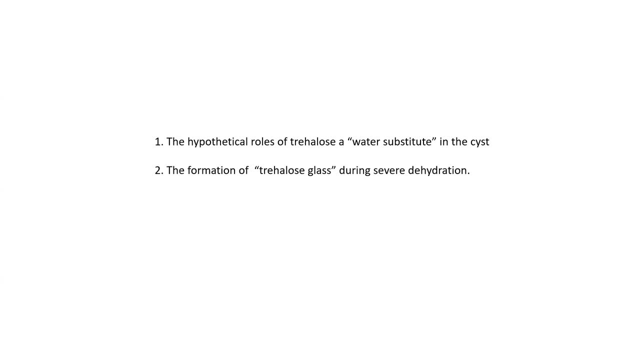 and molting and eventually forms the adult male embryo Or female artemia. One of the very impressive abilities of the noplii and the adult and stages in between is the ability to tolerate very high sodium chloride concentrations- Once again, conditions that are very, very dangerous. 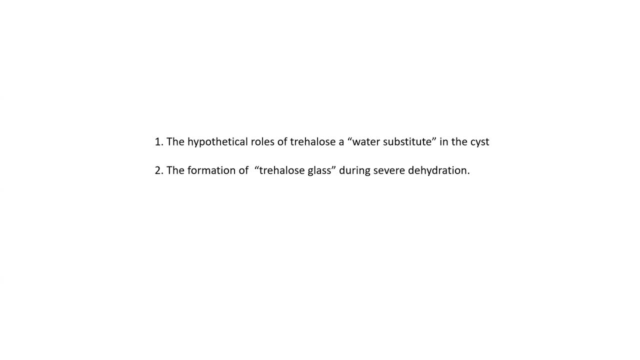 for the vast majority of aquatic invertebrates. the noplius, indeed, has a very special gland in its neck, called poetically the salt gland, which helps handle the exposure to very high sodium chloride concentrations. and so that's a unique morphological characteristic of the noplius larvae, the intermediate larval stages and the adult. 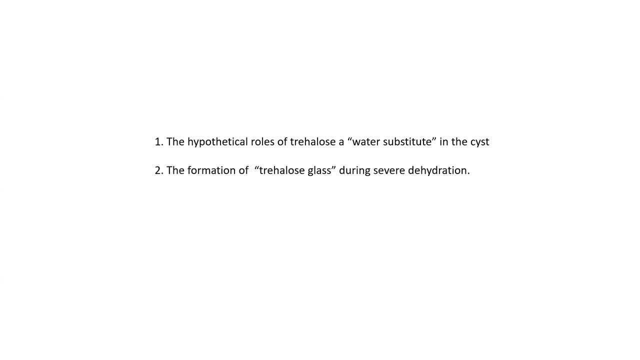 also have cells that are specialized to cope with sodium chloride. so the larvae and adults are also extremophiles in the sense that they, in the sense that they can withstand exposure to sodium chloride, so they can withstand exposure to sodium chloride, so they can withstand exposure to sodium chloride, so they can withstand exposure to that usually threatening condition. 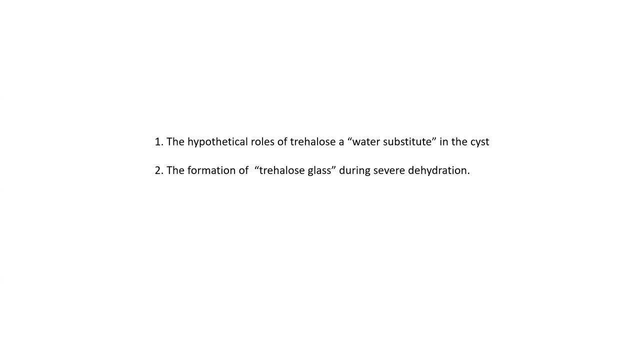 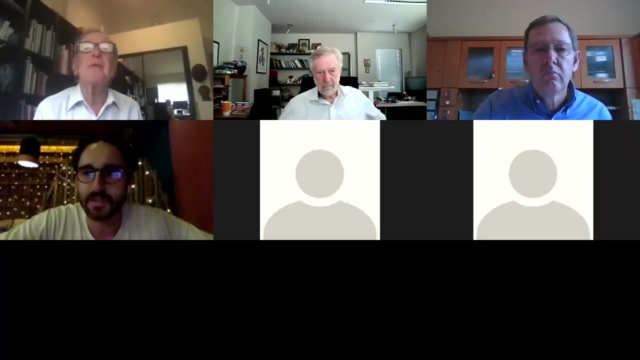 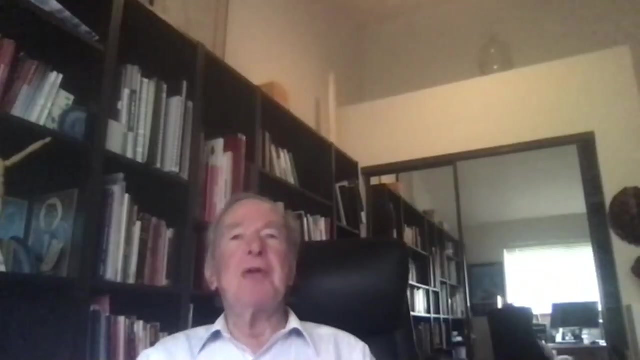 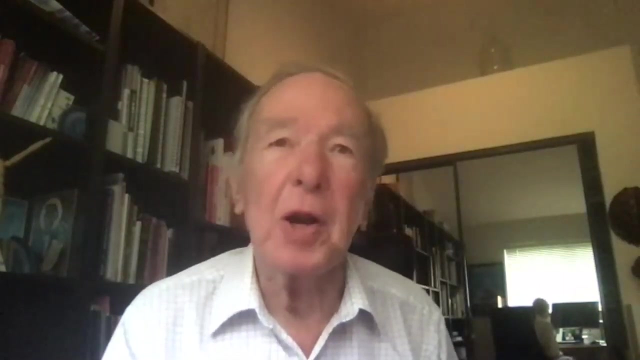 of hypersodium chloride. so, in quick summary to the talk, artemia really is an animal extremophile of extraordinary capabilities and future research will continue to reveal the very, very good treatment. Thank you. I could mention an application. Tralos has been used to stabilize mammalian red blood cells to be used in battlefield. 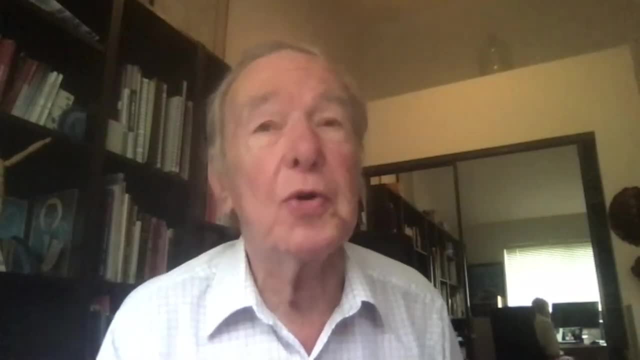 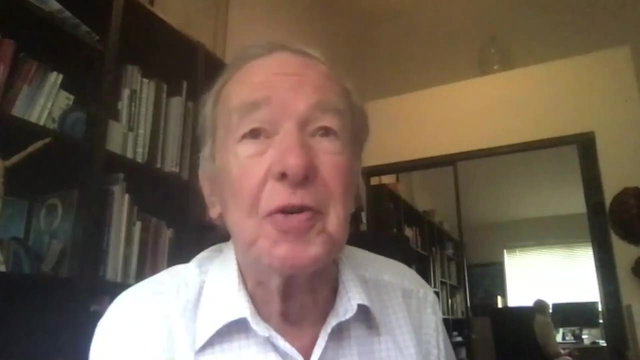 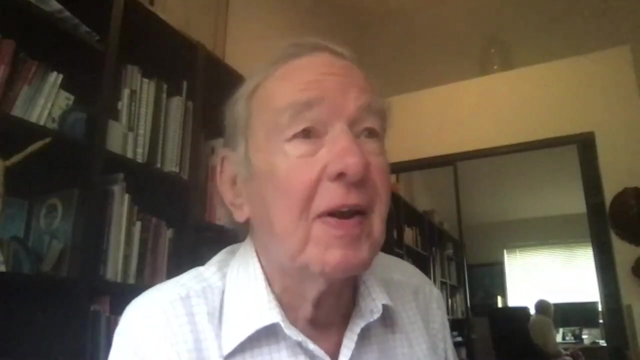 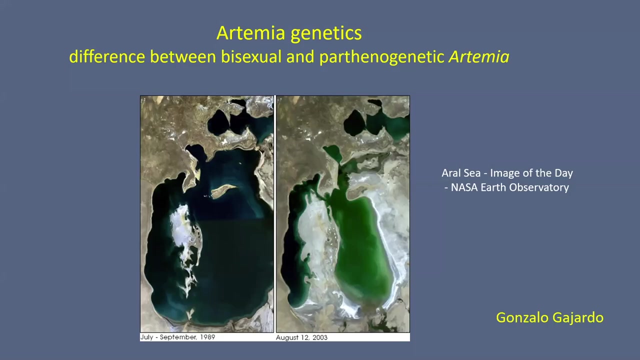 circumstances, as well as storage in hospitals that lack adequate refrigeration. So that's one application of Artemia's basic science: the understanding of Tralos and how it works. Okay, thank you very much. I'm Gonzalo Gajardo, from Chile. I got involved in Artemia research. 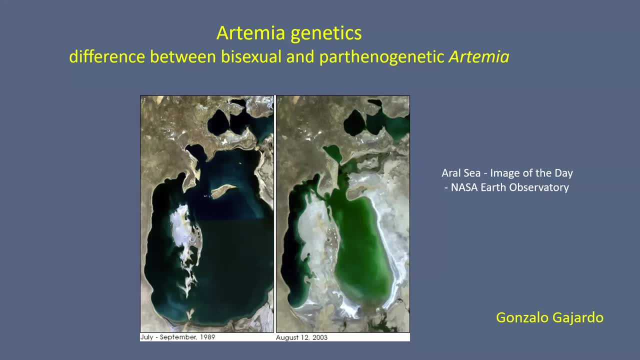 since my postdoctoral days in UK, in Wales, And since then I have been related with the Artemia Reference Center. I think I'm lucky in Chile to have two of the sexual species in very different environmental setups In the Atacama Desert in the north. 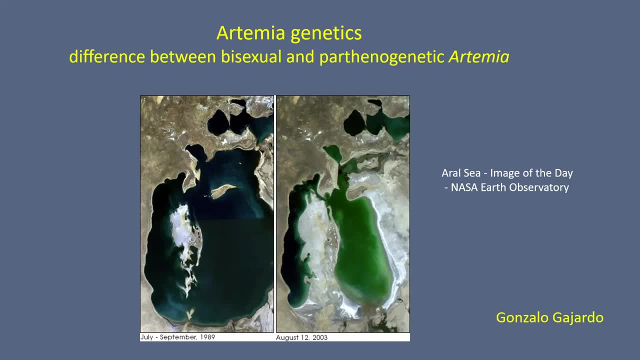 where Artemia franciscana ends its distribution, and also in southern Chile, in the Patagonia, where Artemia franciscana ends its distribution, And also in southern Chile, in the Patagonia, Persimiles is located. So I'm lucky about that And I must say that I'm really intrigued about 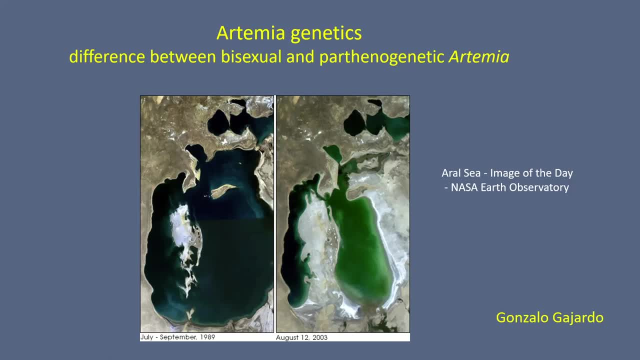 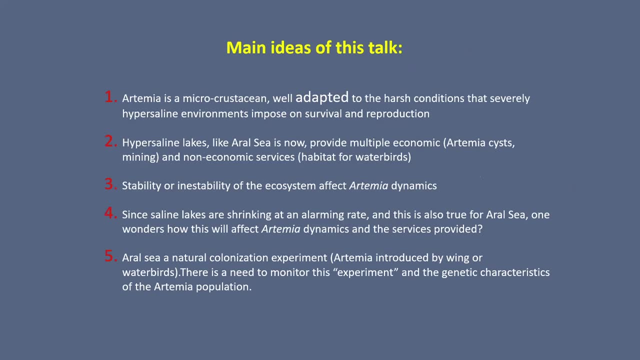 what is happening in Aral Sea, So I'm grateful for this invitation. Next, Patrick, please. My ideas in this talk is that, as Jim said, Artemia is well adapted to very difficult environmental conditions thatипersaline environment impose on survival and reproduction. 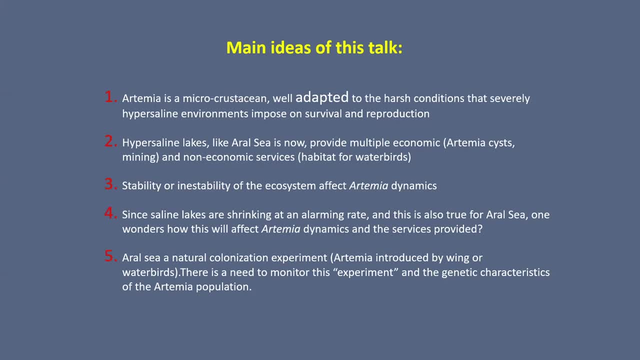 Thathypersaline environment impose on survival and reproduction. Number two: hypersaline lakes like Aral Sea. now I read that salinity is very high now. Number two: hypersaline lakes like Aral Sea. now I read that salinity is very high now. 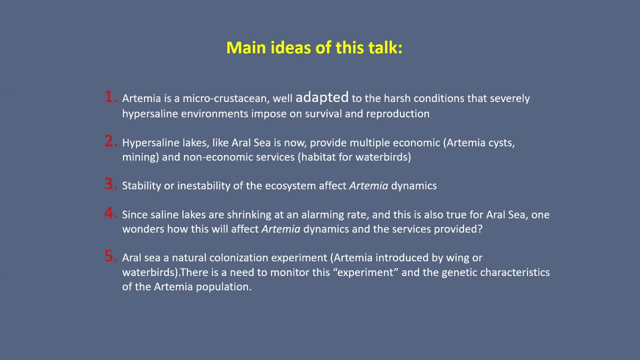 provide multiple economic, as in Aral Sea, resources like Artemia, cysts, Etser, hernias. **** theirpage to create a Ariel Sea, which is now a Penelope Lake from the estudist and isn't outside the tour of Aral Sea. as you have seen, There are several related issues. 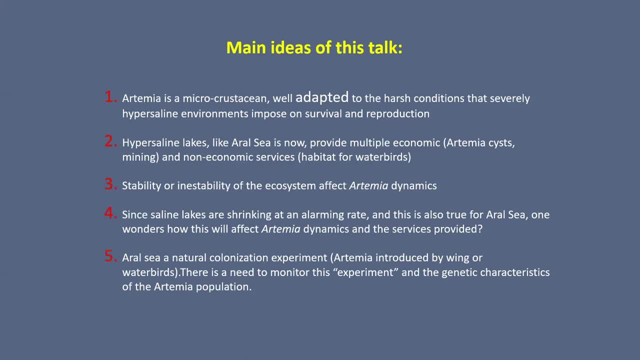 There are several related issues, but also in other places is mining and also non-economic services like habitat, habitat for water birds. number three: stability or instability of the ecosystem affect artemia dynamics and also can influence the economic business. uh, the number four is important because saline, saline lakes are. 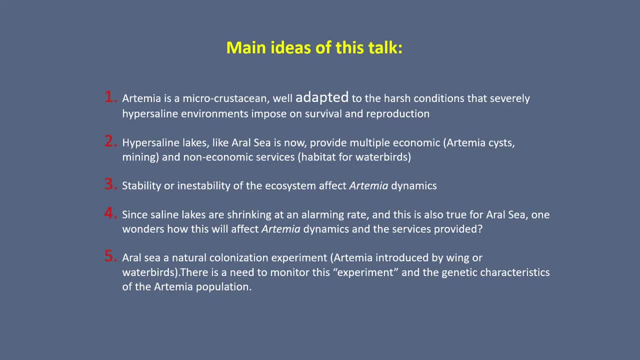 shrinking at the lanar alarming rate, and this is also true for era c, and one wonders uh how this will affect that tinea dynamics and the services uh provided. also, i i see rlc as a natural colonization experiment. artemia was introduced by wind or water birds. 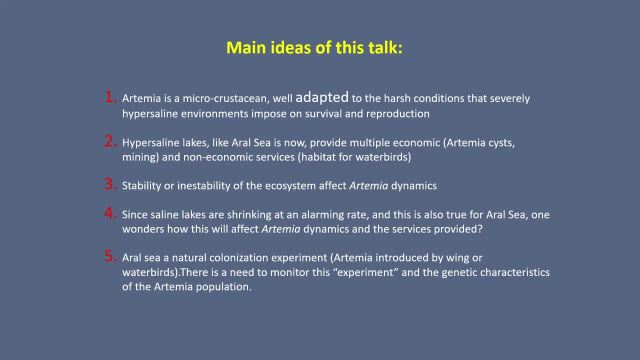 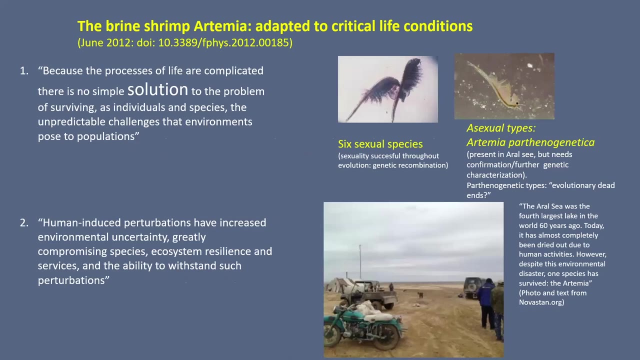 there is a need to more monitor this experiment and the genetic characteristics of the artemia population there. that is, artemia partinogenetica. next, patrick, please, uh, i said before, uh, the branch stream. artemia is an example of adapted to critical life conditions. 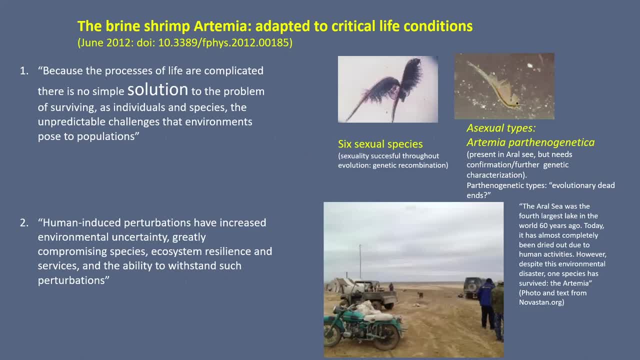 and, as you know, because the processes of life are complicated, there is no simple solution to the problem of surviving, as individuals and species, the unpredictable challenges that environments pose to populations. so in the case of artemia, we have two solutions: uh, sexual species or bisexual and asexual types. like storage, it contain a particular genetic. 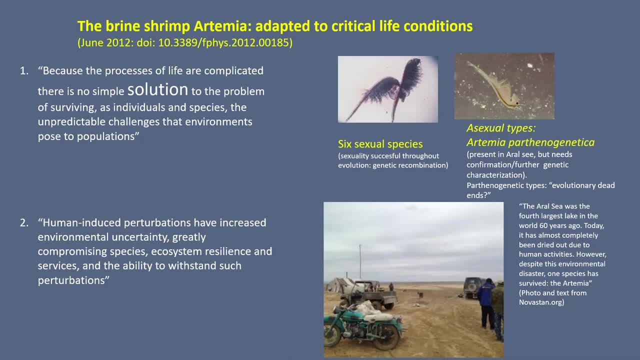 uh, i think sexual species are really privileged during the evolution. uh, because of genetic rfg information. emphasize the importance of beliefs. róactic combination- this is important since my화 moisturizer is still one of the consumers- is important when a male and female share genetic information. 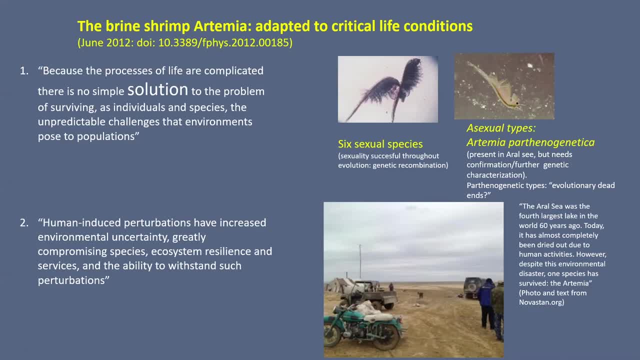 Instead asexual types like Artemia parthenogenetica for textbooks. they represent evolutionary dead ends. They are supposed to be difficult to thrive in different environments. And the second point I would like to make here on the left-hand side is that human-induced perturbations 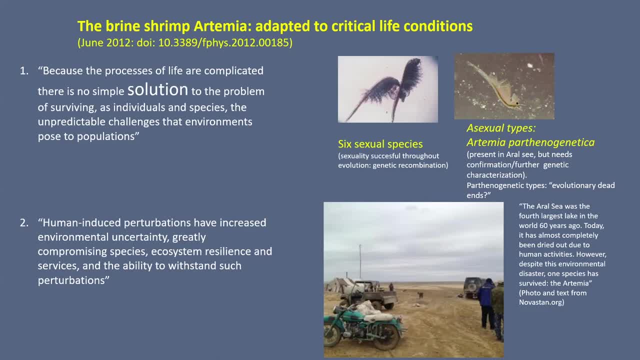 have increased environmental uncertainty, greatly compromising species, ecosystem resilience and services, like seeds being produced in aral seed and the ability to withstand such perturbations. I got this image photo from aral seed from a web page. 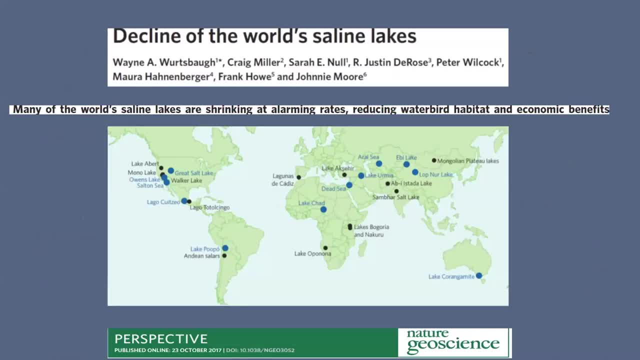 And next, please. As I mentioned, many of the world's saline lakes are shrinking at alarming rates, reducing water, birth, habitat and economic benefit. So this was very important And the paper I read for previous presentation. Next, Patrick. 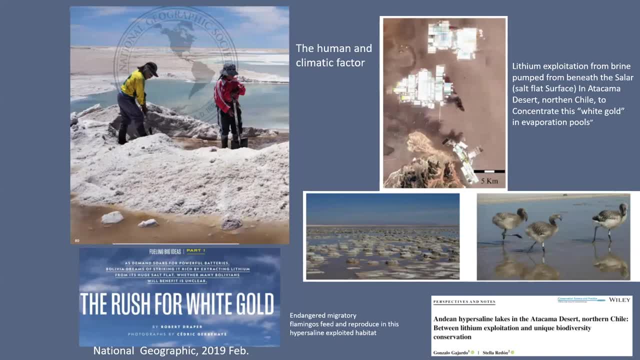 Since we are talking about national geographic, I came across with this paper called The Rush for White Hole And it show. It shows how It's how. in Bolivia, Lake Uyuni has a huge deposit of lithium, So the government is planning to exploit it. 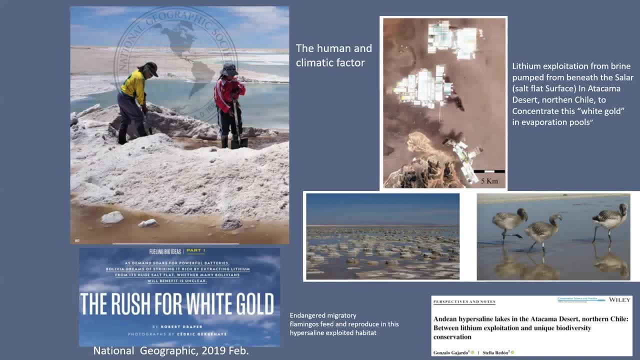 for economic benefit. And also, on the right hand side, we have the Atacama Desert, where salty lakes co-exceed with the huge- I think it's the most important lithium extraction being performed in the world. And what is the problem is that 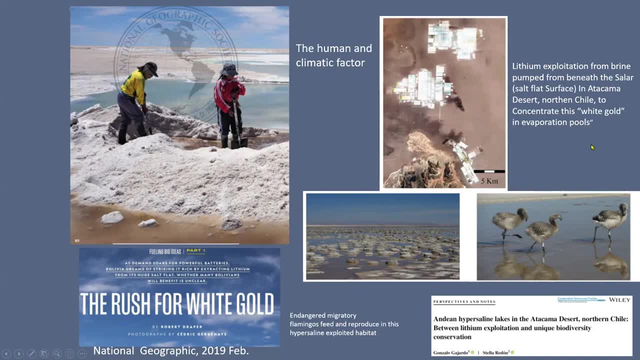 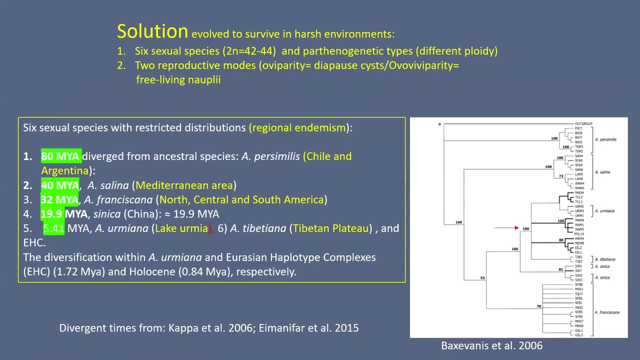 brine. pump it from beneath the solar surface in Atacama Desert may impair the habitat for flamingos. Okay Next, So continuing with this evolutionary solution to survive in harsh environments. I think Artemia is a peculiar and very important example of extremophile. 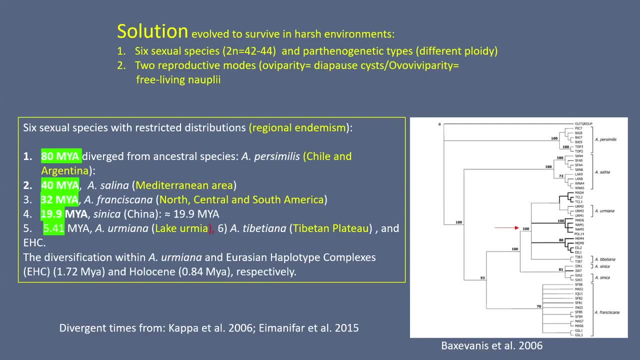 Well, we have six sexual species. as said before, Patrick wanted me to highlight some of them. We have some genetic characteristics And I mentioned here they deployed a number of most species is 2N42, but Artemia persimilis is one of the few with 2N44.. 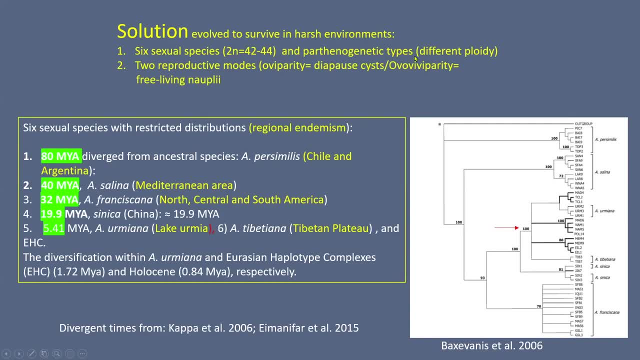 And there are many parthenogenetic types with different levels of ploidy, And this is something very amazing. And point number two is very interesting Also. there are two reproductive modes of the parity. That means the production of a diapose cyst. 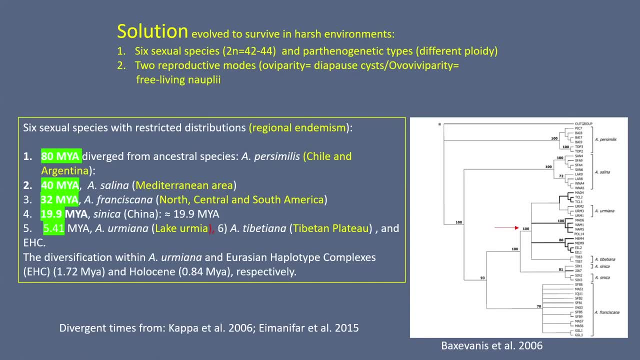 and also Oboviparity, the production of free living nauplii. Both sexual and asexual species produce both. So it's important for you to know that here are the sexual species, and I ordered them because in relation to the oldest diverger. 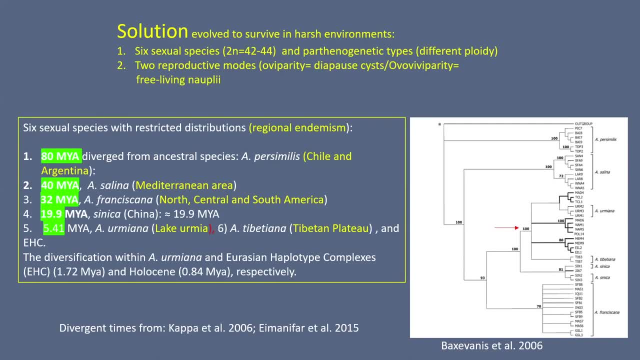 from an ancestral species, Artemia persimilis, found in Chile and Argentina. as I said before, is the oldest, So you have a. The time past seems divergent from ancestral species: is more or less 80 million years ago. 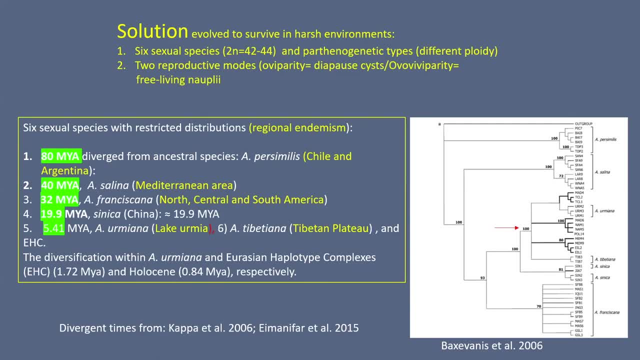 So it's a good time. Then we have Artemia salina that is found in the Mediterranean area 40 million years ago, And Artemia franciscana, that is very common in North, Central and South America. And, as said before, Artemia canadensis is about. 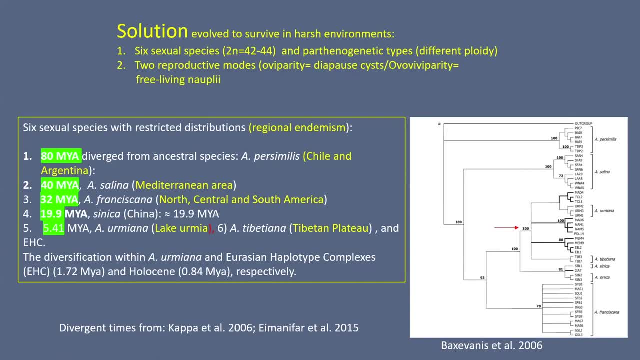 it's very important in aquaculture 32 million years ago. Then we have Seneca 19 or close to 20 million years ago, And then Artemia urmiana from Lake Urmia, Artemia tibetiana from the Tibetan plateau. 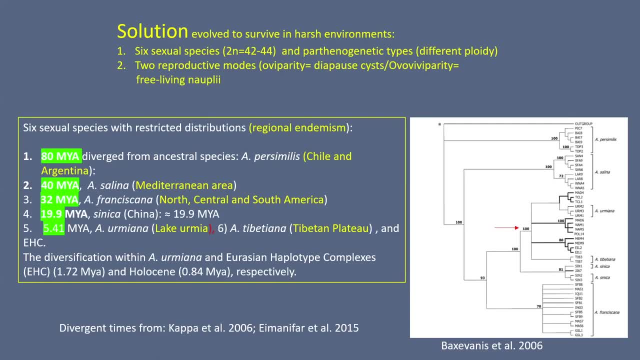 and several Eurasian apple type complexes that are very young. So here on the right you have the phylogenetic tree got by Baxivanis from Greece. So you have the similarities and differences between species, What is very important. no, 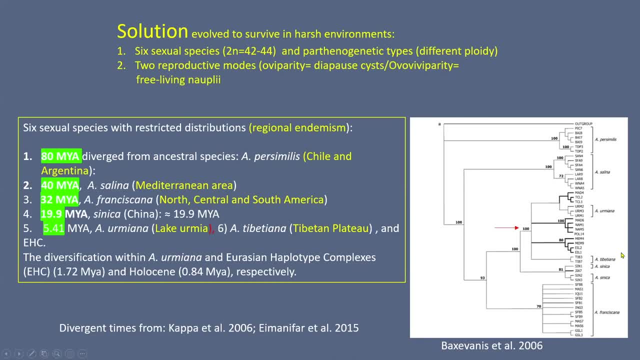 what is very important is shown by the red dot. there You see in black, very thick black, Artemia parthenogenetica that may be related, very related with Artemia urmiana. So when you saw the first slide and you see the proximity of Lake Urmia and Aral Sea, 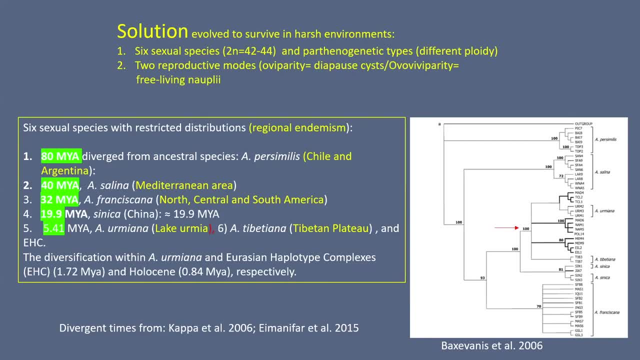 you can understand that Artemia parthenogenetica is very close to Lake Urmia. You can understand why Artemia parthenogenetica could colonize Aral Sea. Okay, next, please. This is very common, but again. 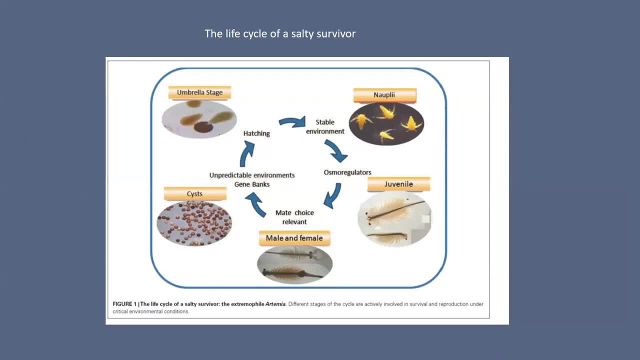 just to highlight that Artemia female can produce nauplii when the environment is stable. on the right: Yes, thank you. And cyst that is important for Aral Sea? when the conditions are not stable, I should say that no one knows very well. 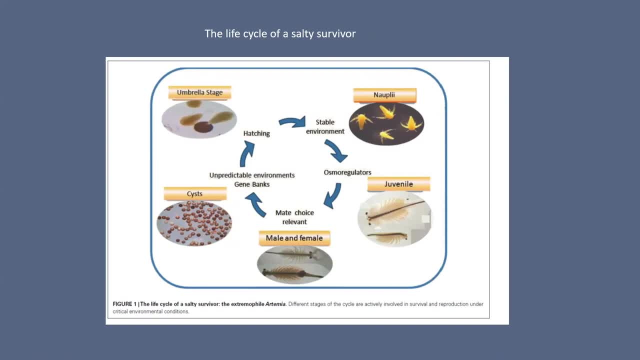 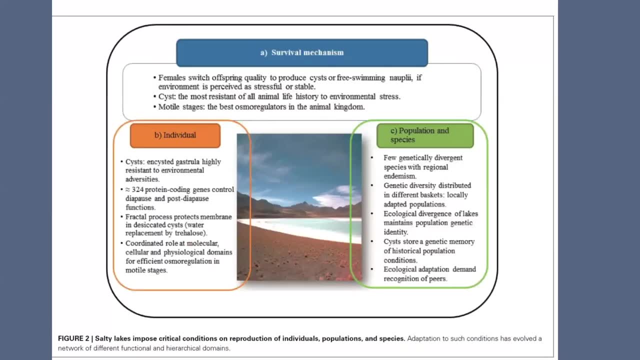 what stable or unstable conditions means. Next, Patrick, please. This is just to summarize What I have said before, So you see in A minor here what is said already and here in B, for individual, what Jim Clegg said. very important metabolic and physiological mechanisms. 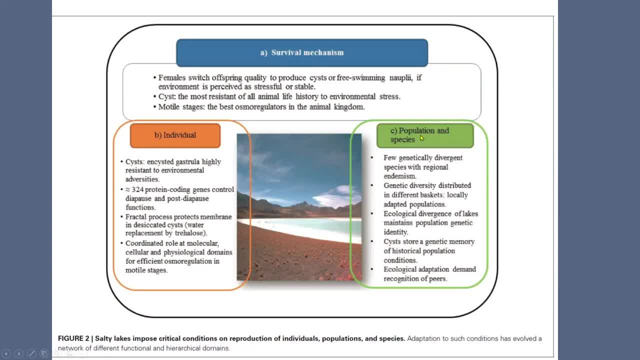 And here on C, some very important characteristics of the Aral Sea. And this is a very interesting example of Artemia franciscana: There are few genetically well the sexual species, few genetically different species, with regional endemism. 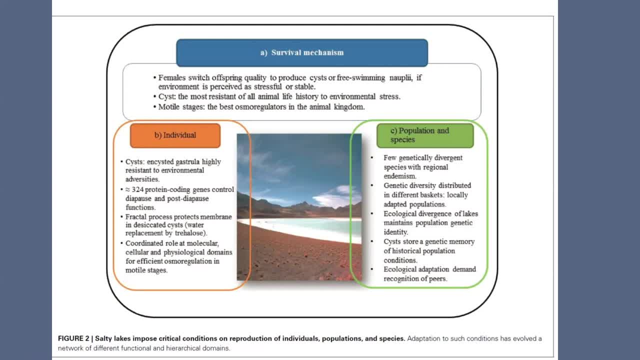 In Artemia franciscana, mainly genetic diversity that is very useful for resilience is distributed in different baskets. This is like in banks with your investment. So I just wanted to show that This means locally adapted population. So artemia franciscana is well distributed. 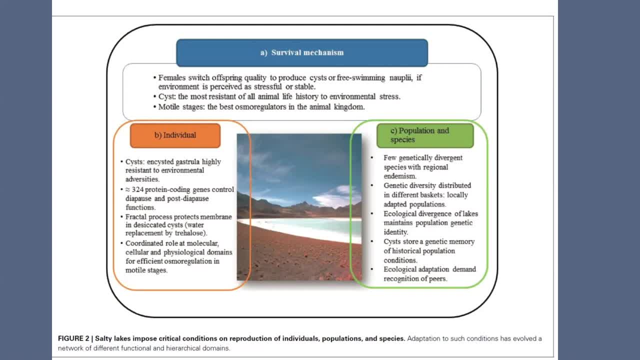 in different places, So every population has particularities. I will go to cyst here. that store a genetic memory of historical population condition. So this is very important, I guess, to understand also in Aral Sea And ecological adaptation demand recognitions of peer. 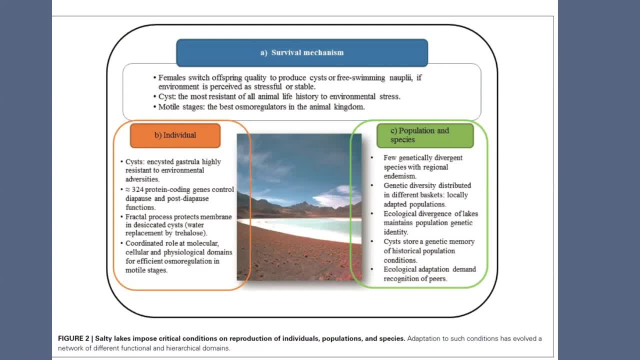 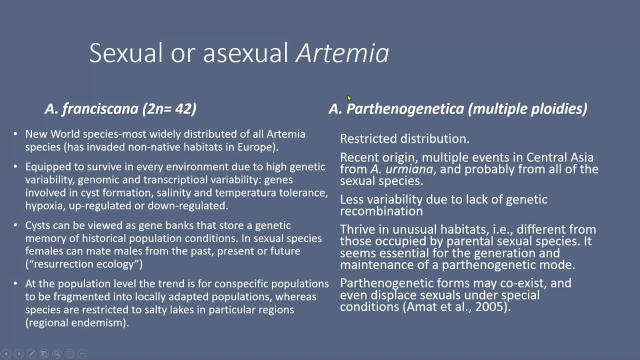 For example, special species. they need to. I wouldn't say courtship with mates, but they do this. Next, Patrick, Just to summarize, you have on the left artemia franciscana. Okay, New world species Very widely distributed. of all artemia species, 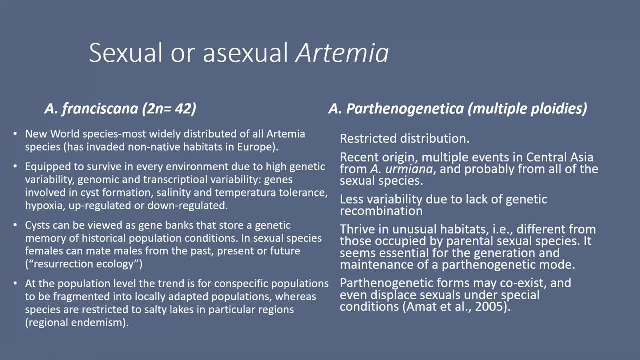 are very well studied, Equipped to survive in many environments, due to the high genetic variability, genomic and transcripts variability, biomechanics, biochemical genetics and genetic Genes involved in cyst formation, salinity and temperature tolerance, hypoxia, as mentioned. 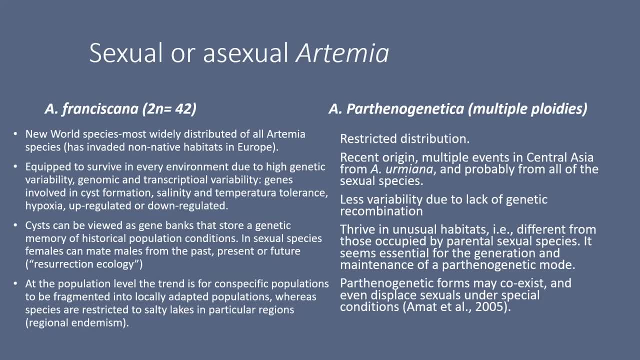 are upregulated and downregulated depending on the conditions. Cysts can be viewed as gene banks that store a genetic memory of historical population condition In sexual species. females can mate males. this is weird, but it's true from the past, from the present. 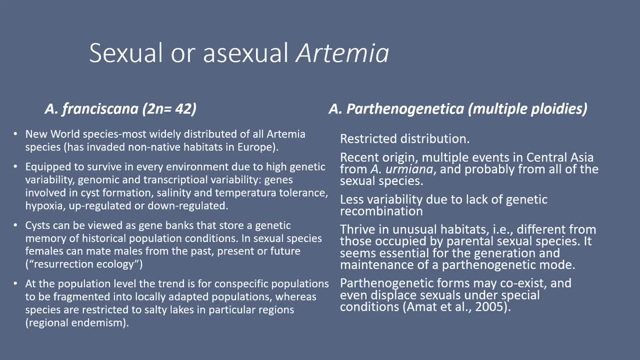 or from the future, And there are some studies that show that females prefer contemporary males. This is amazing. How do they do? it is interesting. Well, I go to Artemia parthenogenetica, not to take much time. It has a strict distribution. 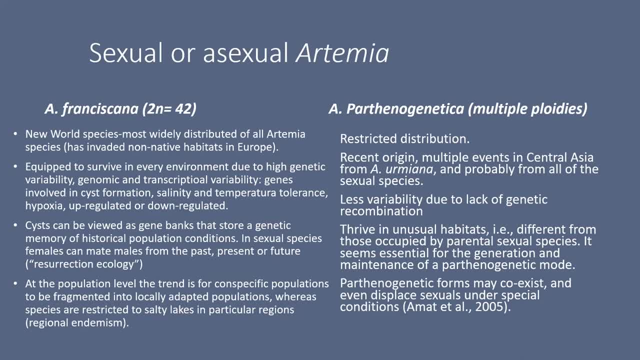 Recent origins. I've mentioned it before: multiple origin events in Central Asia, from Artemia urbiana and probably from all the sexual species. Less variability due to the lack of genetic recombination and because of that they thrive in unusual habitats. That means different from those occupied. 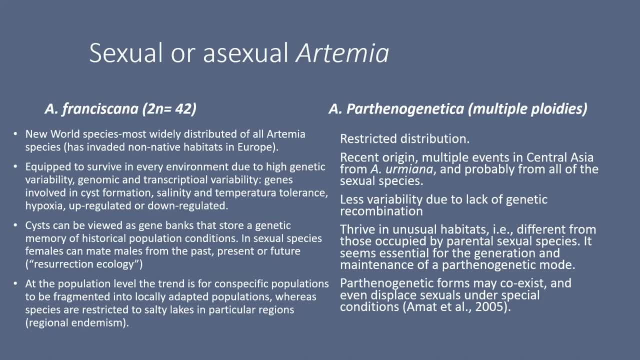 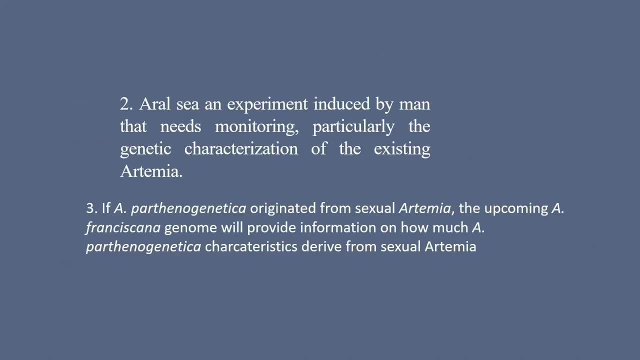 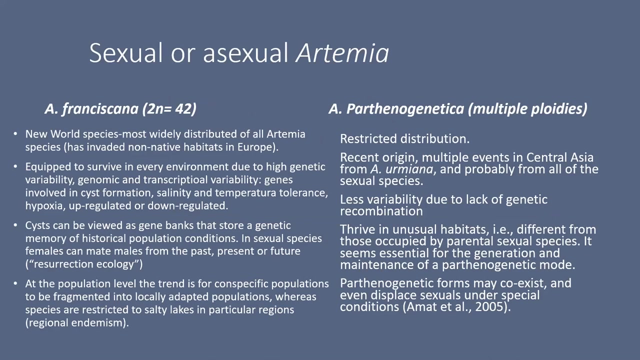 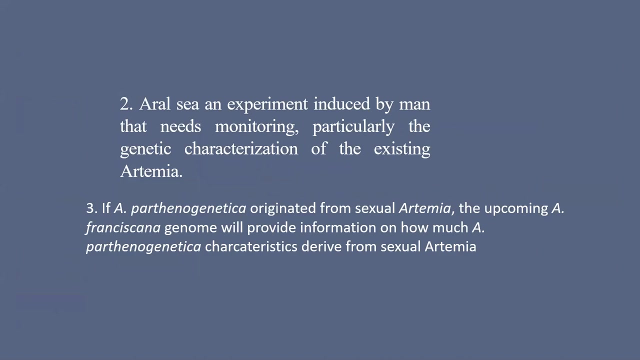 by parental sexual species And, what is surprising, and I will mention this in my last slide- parthenogenetic forms come at this place. Can you go back? can displace sexuals under very special conditions. I wanted to finish my presentation saying that ARLC is a very nice natural experiment. 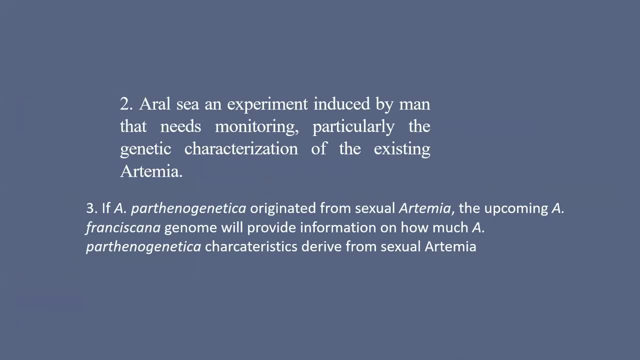 that needs monitoring, as we have seen here in Great Soul Lake, particularly the genetic characterization of the existing artemia. I think I couldn't find more information about the artemia parthenogenetica that is in the sea And also, I think, if artemia parthenogenetica originated from sexual artemia. 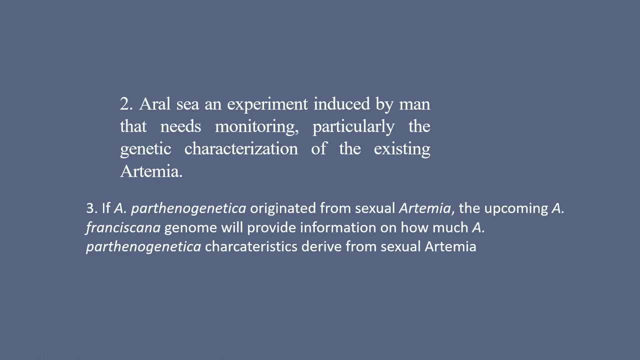 the upcoming artemia franciscana genome will provide information about the genetic characterization of the existing artemia parthenogenetica And also, I think, if artemia parthenogenetica originated from sexual artemia. the upcoming artemia parthenogenetica will provide information. 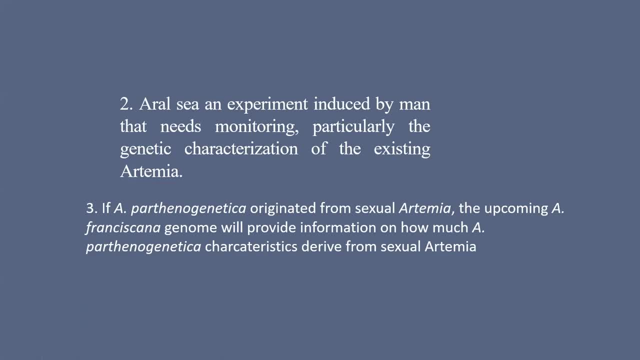 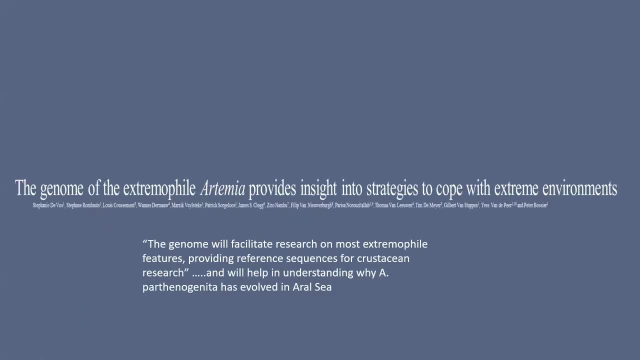 on how much artemia parthenogenetica owes to sexual artemia. So next, please. This is the paper that is soon to come out, where Jim and Patrick and a lot of people from Belgium are involved, So the genome will facilitate research on most. 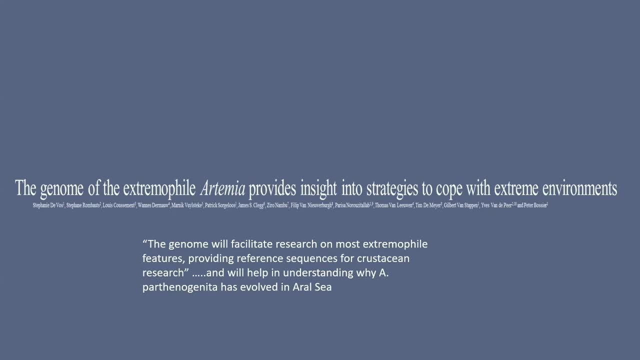 most extremophile features, providing reference sequences for crustacean research, And my personal opinion is that it will help in understanding many of the features that have made possible that artemia parthenogenetica evolved in ARLC. Okay, thank you. 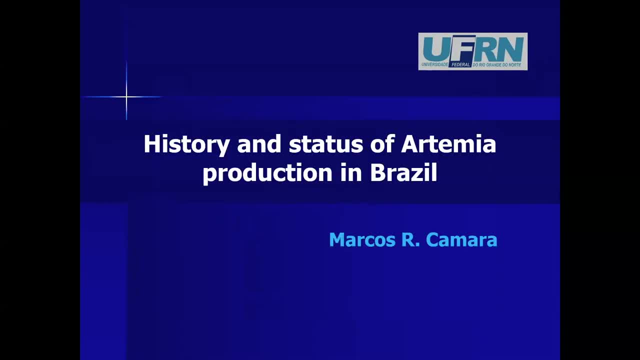 My name is Marcos Camara and it's nice to be here today with you. I am a full professor at the Federal University of Rio Grande do Norte in northeastern Brazil, And I am a professor at the University of Rio Grande do Norte in Brazil. 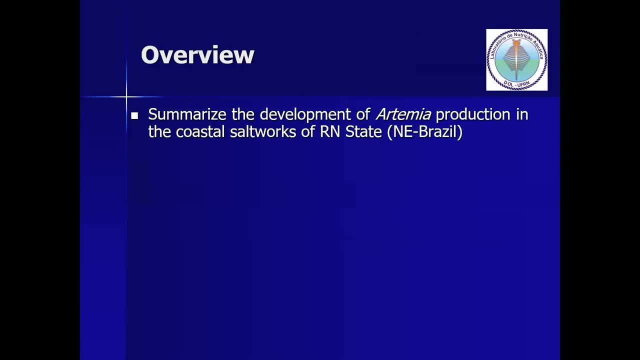 And I am a professor at the University of Rio Grande do Norte in Brazil, And during my talk I will summarize the development of artemia production in the coastal salt works of Rio Grande do Norte state. I will also review current seed harvesting practices and try. 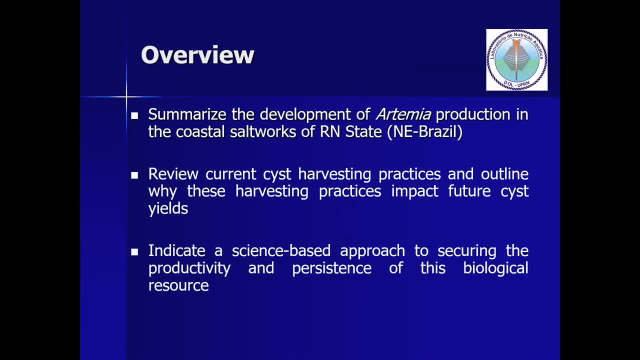 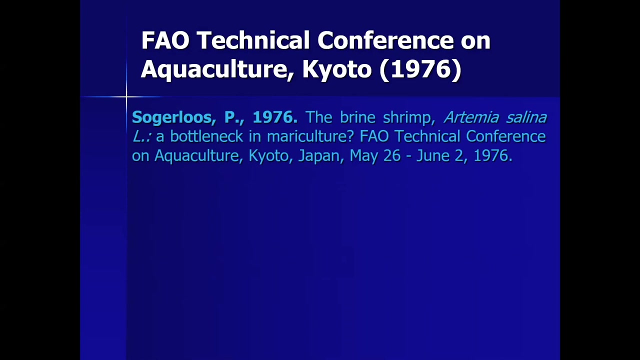 to outline why these harvesting practices impact future seed yields. And finally, I will indicate a science-based approach to securing the productivity and persistence of these biological resources. Well, as you have mentioned before today, it all started in Kyoto in 1976,. 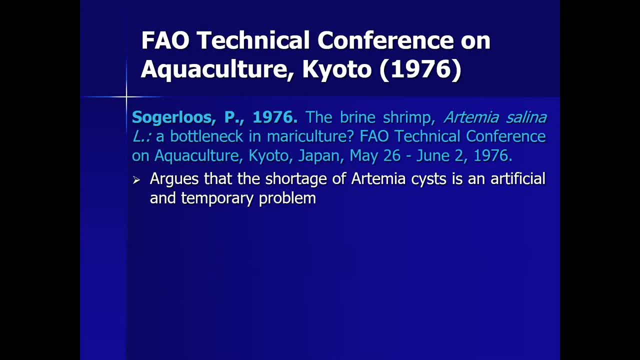 when artemia was considered problem to the expansion of aquaculture and Patrick argued that this shortage was an artificial and temporary problem and he funded through efforts in the following years to make this production of artemia viable in developing countries, As Ed in essence just mentioned. 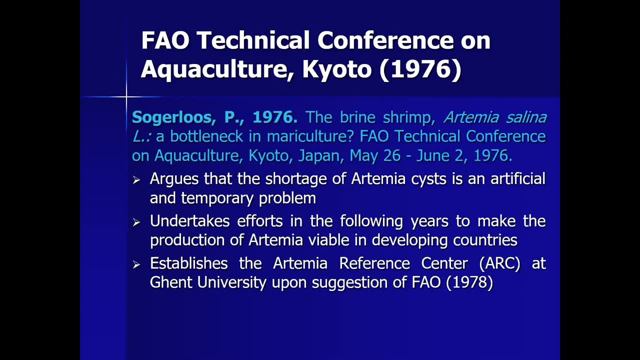 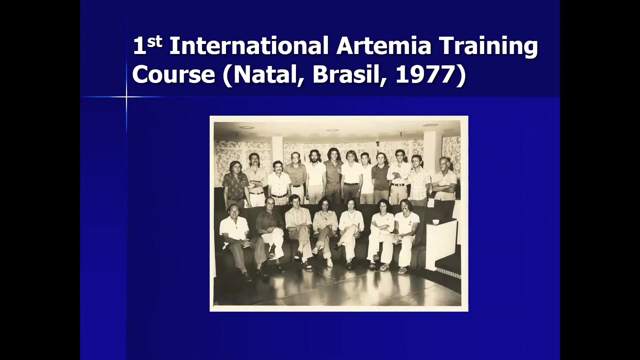 he funded the establishment of ARC at Ghent University upon suggestion of FAO in 1978, and the organization of several international artemia training courses thereafter. And by chance, the first international artemia training course was in a town, my hometown. 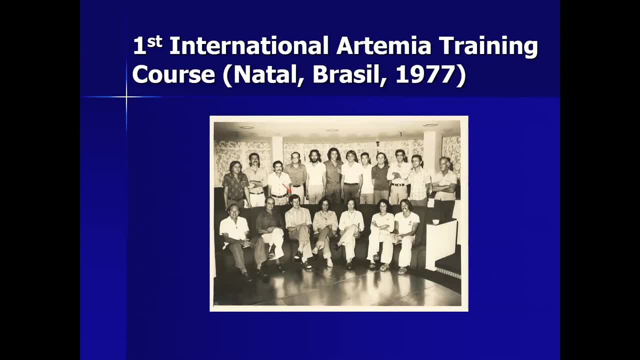 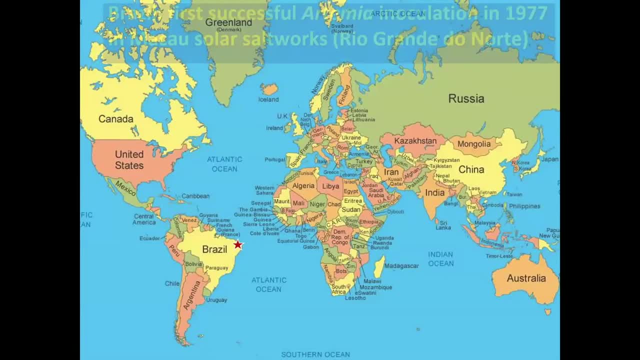 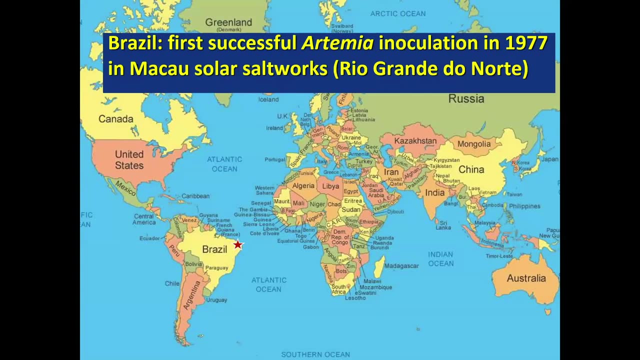 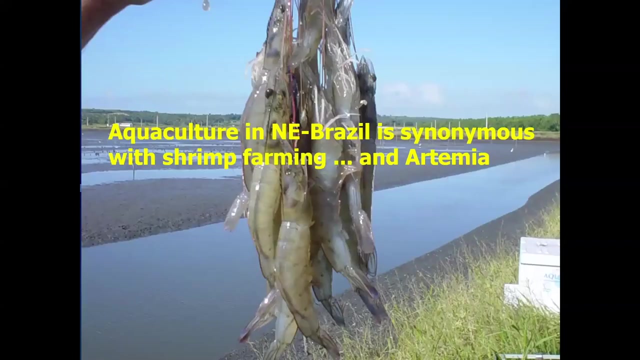 in 1978.. In 1977, here, Patrick, and it made viable the first inoculation of artemia in Brazil, in Macau Solar Softworks. And before going into more detail, I'd like to make this connection. 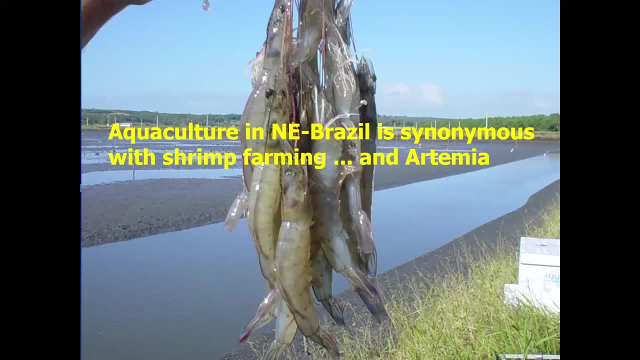 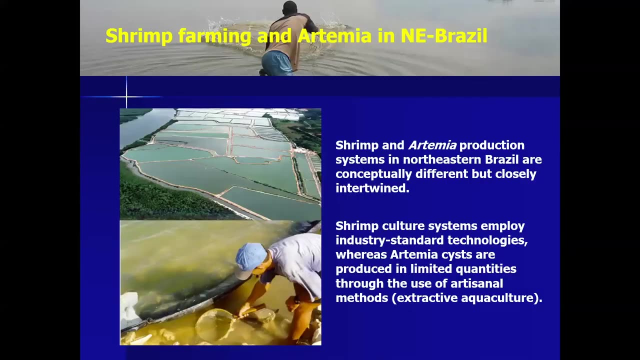 Because aquaculture in northeastern Brazil is practically synonymous with shrimp farming and artemia. These two systems are conceptually different but they are closely related. Shrimp culture systems employ industry-standard technologies, but artemia are produced in more limited quantities and they are not produced in large quantities and they are not produced in. 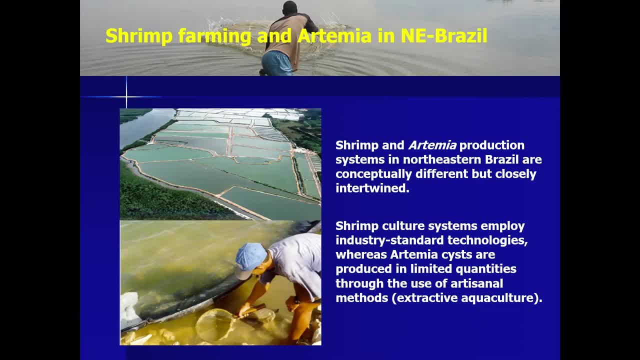 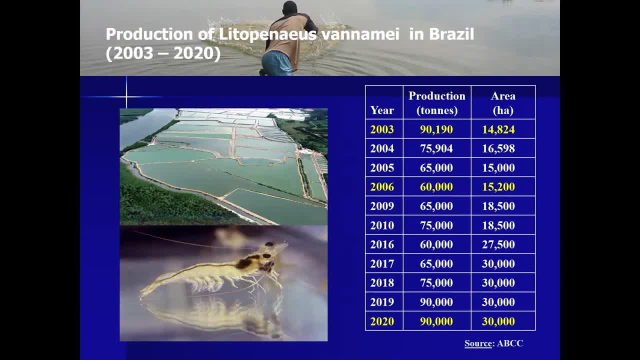 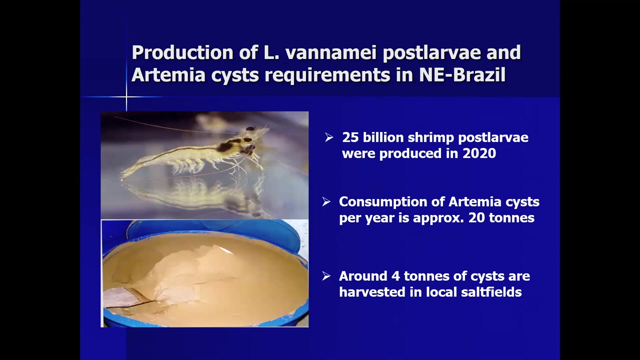 Okay, in this table you have an idea of production figures for Lithopneus zonami, which is the global shrimp species, and it's also farmed in Brazil. So in 2020, About- homegrown shrimps become massively. 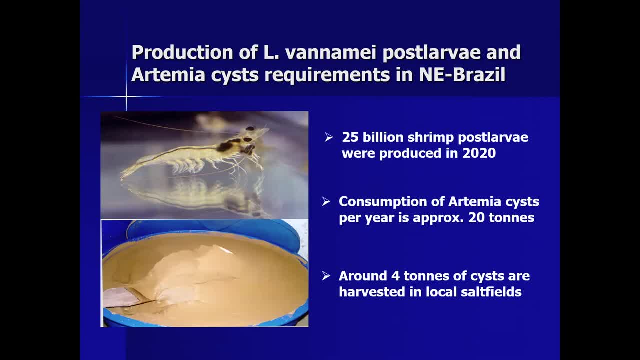 polynguia. Okay, All right, Thank you everyone. we'll keep talking. Thank you. The last year production was around 90,000 tons, 30,000 hectares of production area. 20 billion shrimp larvae were produced and this amounts to about 20 tons of consumption of artemia systems- Around 4%. 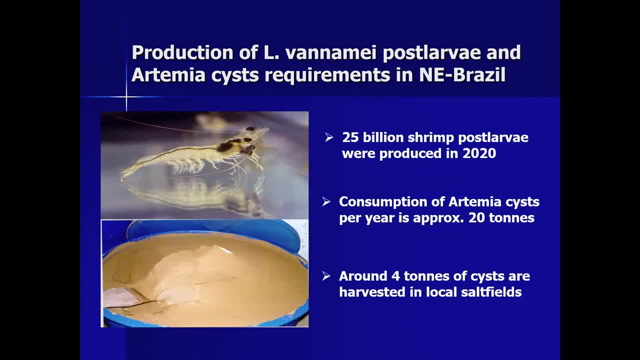 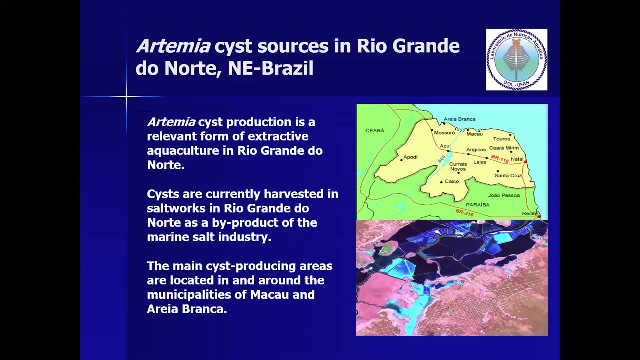 tons. So around 20% of these demands are fulfilled with cysts harvested in local salt fields. So you have some pictures here. So the production of artemia cysts are quite relevant and it's a form of extractive aquaculture in Rio Grande do Norte. 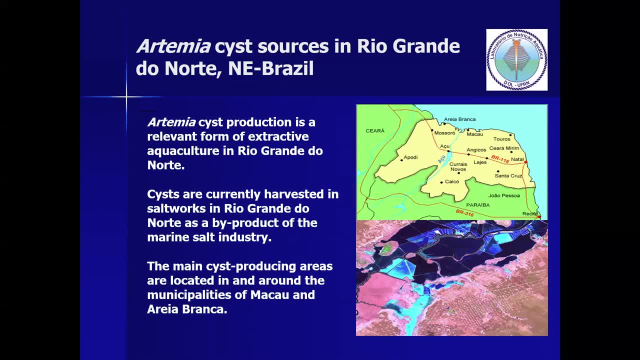 These cysts are harvested in salt works as a byproduct of the marine salt industry, which produces about 95% of all marine salt consumed in Brazil. So it's quite important to the economy of Rio Grande do Norte state. The main cyst producing areas are: 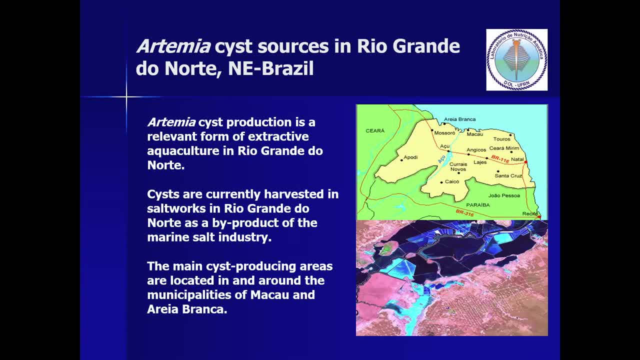 located in and around the municipalities of Macau and Areia Branca, also here in Grossos, around Mossoró. This is the capital, Natal, where the main campus of Federal University of Rio Grande do Norte is located, and this is where I live. 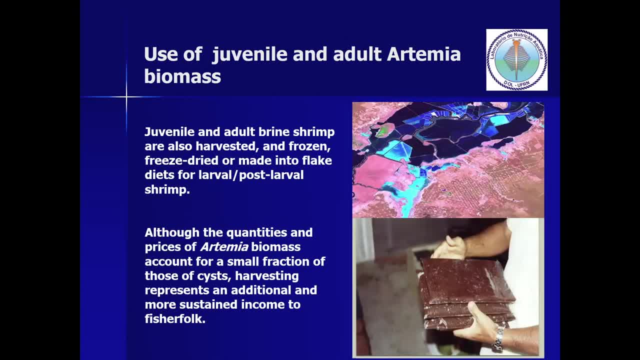 So a few details about also the use of the biomasse. So it's also collected in these huge salt production operations. They are harvested, frozen, freeze-dried or made into flake diets for larval, post-larval shrimp. 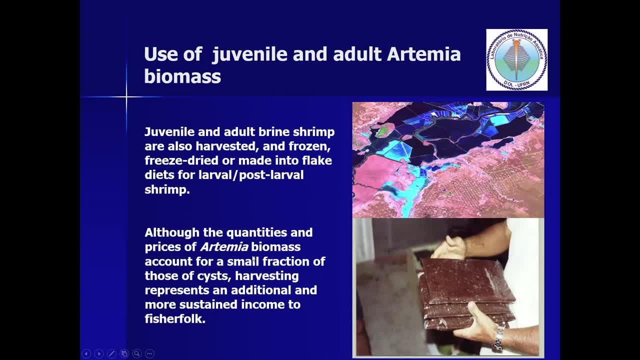 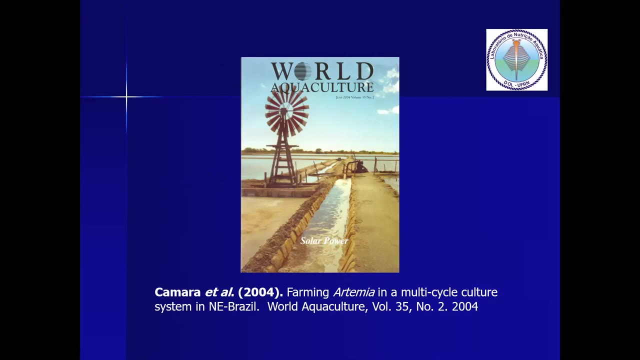 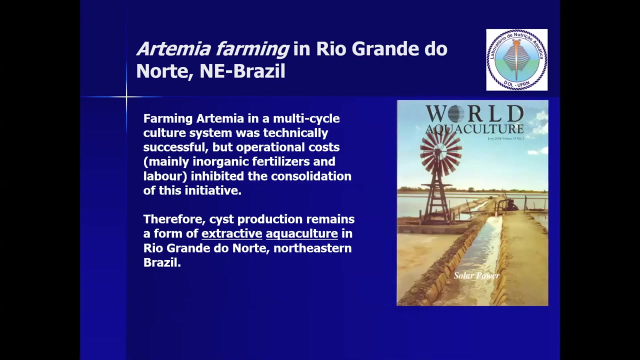 This is quite important because, although the quantities and price of these biomasses represent just a small fraction of those of cysts, this activity represents an additional and more sustained income to fishermen. Well, I will just briefly talk about farming artemia in northeastern Brazil. So it was technically successful, but the operational costs. 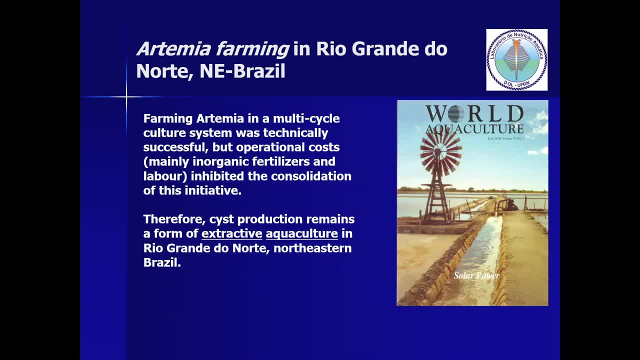 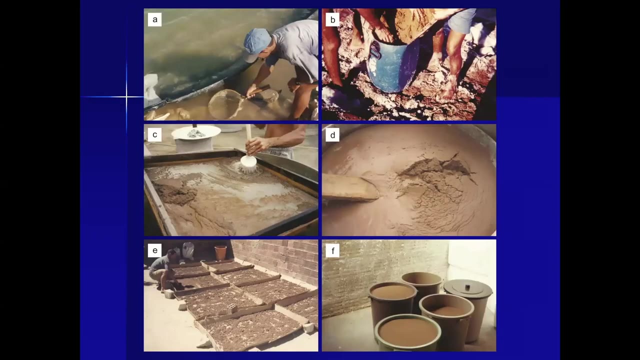 basically inorganic fertilizers, and labor inhibited the consolidation of this initiative. So this production still remains as the form, the only form of extractive aquaculture in Rio Grande do Norte. These pictures you can view some of the different steps. 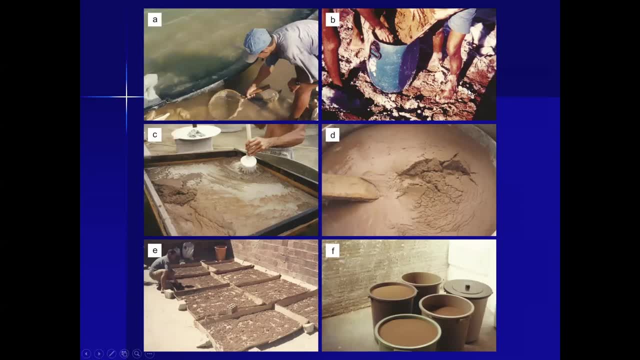 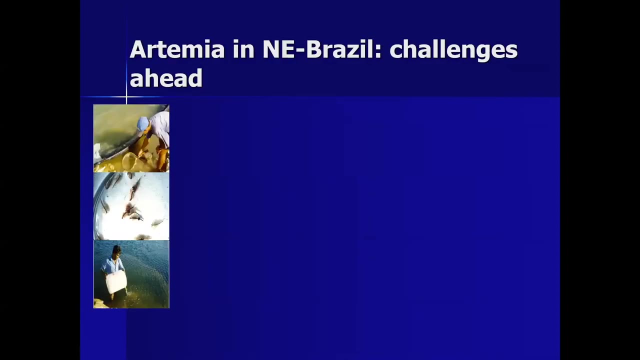 Scoping the cysts from the water or from the shore, cleaning, storing in brine, sun drying and cysts ready for sales. Well, and to finalize my presentation, I'd like to show you some of the challenges I have encountered. One is how to manage the quantity of the 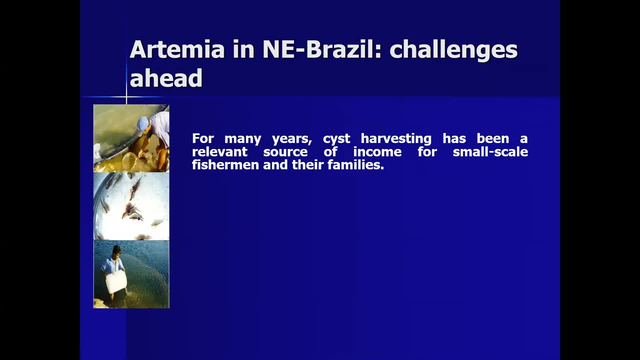 large-scale fisheries that are being harvested in Brazil or in some of the neighboring cities. The other challenge is how to manage the quantity of the large-scale fisheries that are being harvested in the EU or in the EU-M impacted by the climate change. 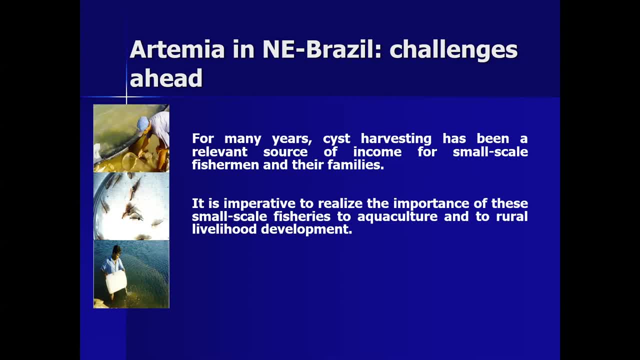 So I want to first go back to the first question, which is: does large-scale fisheries, especially large-scale fisheries in Brazil, represent a significant increase in the cost of harvesting? If so, could you tell me how do you cope with thiskl вообще da parte do vocês ver que é o problema do vocês ver que a um uso de uma única energia, no mais é tão importante do que o uso de uma antiguo uso de uma antiguo uso do aritmia em seamally in northeastern Brazil. 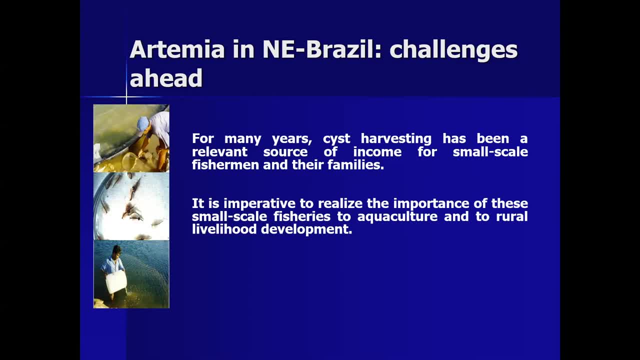 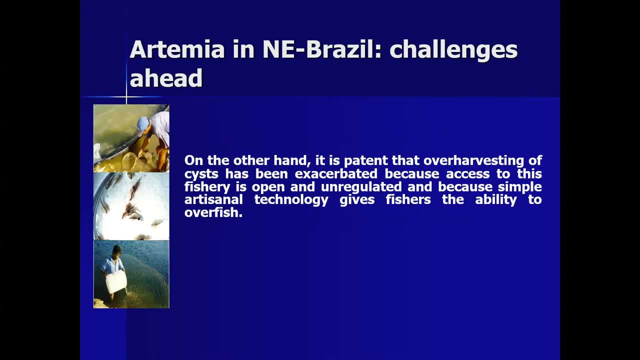 to aquaculture and to rural livelihood development and, on the other hand, it's also important that we mentioned that over harvesting of sis has been exacerbated because access to the fishery is open and unregulated, differently from what we have heard before here regarding great salt lake, for 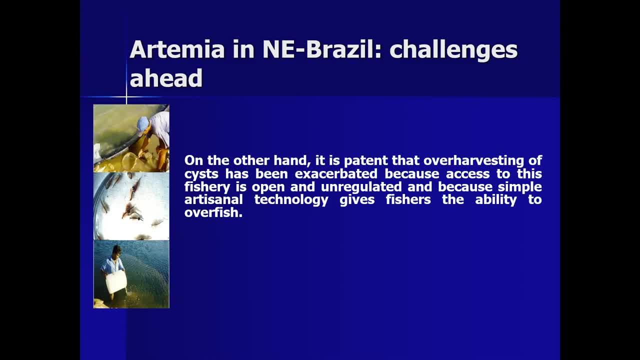 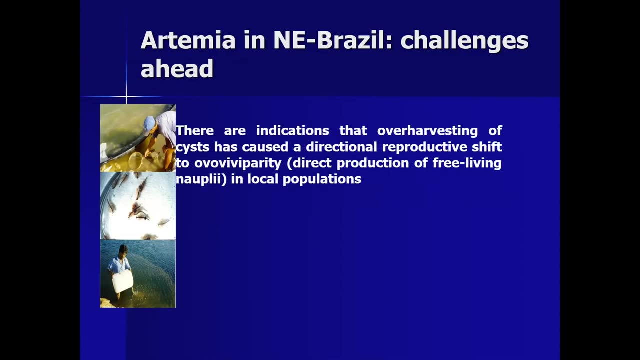 example. so, and because of this scenario, simple artisanal technology gives fishers the ability to over fish, so quite a big challenge. try to regulate this harvesting, because there are indications that the fishers are not able to over fish and they are not able to over fish. 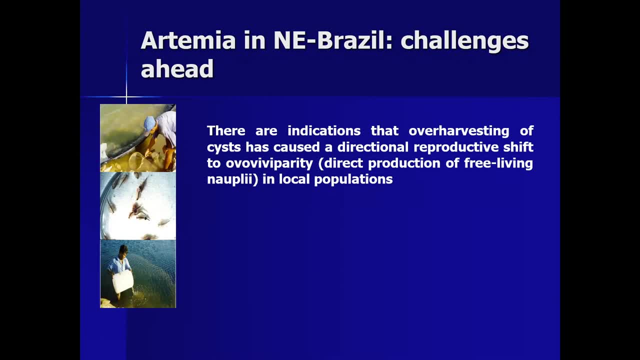 because there are indications that the fishers are not able to over fish, that over harvesting of sis has caused a directional reproductive shift to over repair it, direct production of, really in an upper eye on the local population of our team. so there is a urgent need to clarify whether harvesting is inducing genetic. 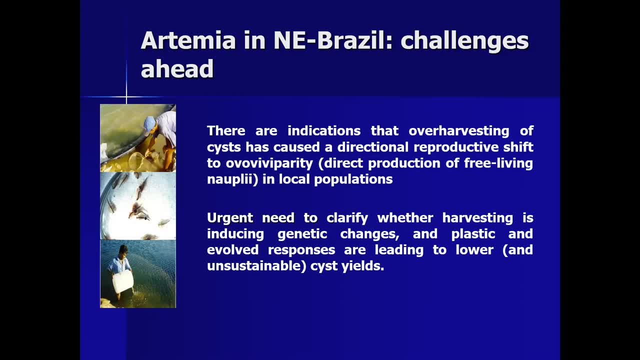 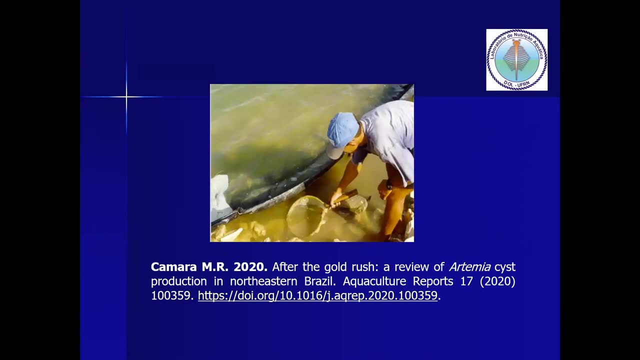 changes and the classic and evolved responses are leading to lower, and the classic and evolved responses are leading to lower and the classic and evolved responses are leading to lower and, of course, unsustainable CISP yields. Well, some of the thoughts I have presented here are detailed under this publication. 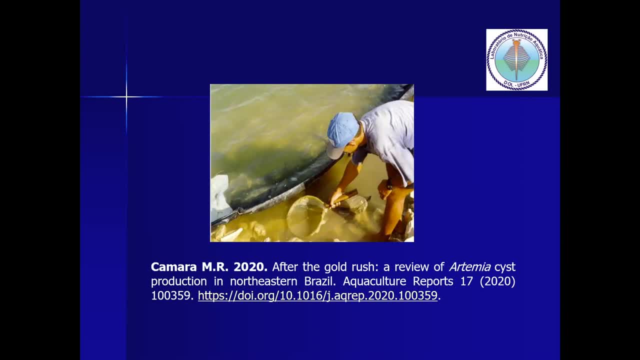 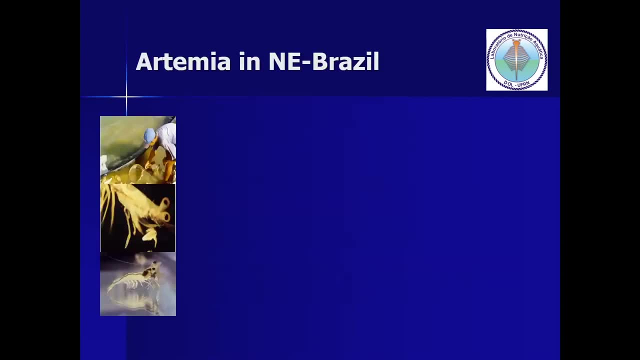 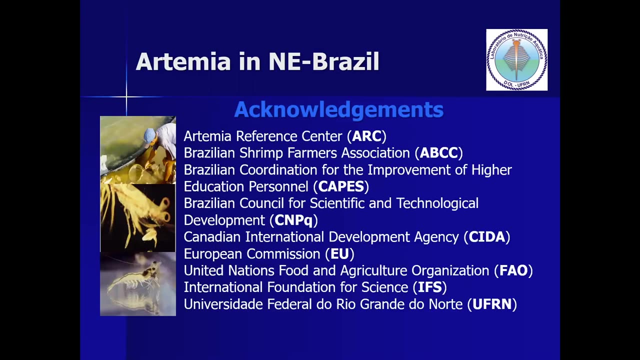 from last year, after the Gold Rush review of artemia CISP production in northeastern Brazil. And I finally like to acknowledge the contribution of these institutions. okay by alphabetic order: Artemia Reference Center, Brazilian Institutes, Canadian Agency, European Commission, FNC. 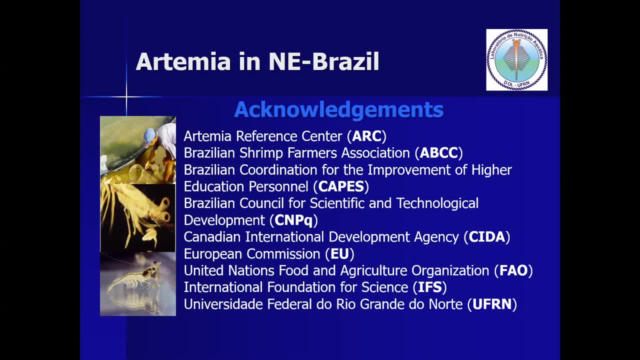 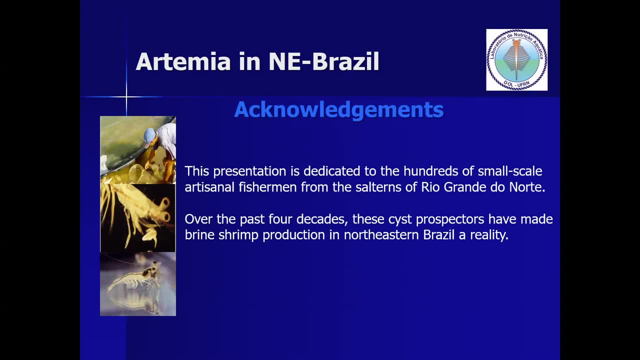 KO, IFS and, of course, my university, Federal University of Rio Grande do Norte. And finally also, I'd like to dedicate this brief presentation to the hundreds of small-scale artisanal fishermen from the sultans of Rio Grande do Norte. 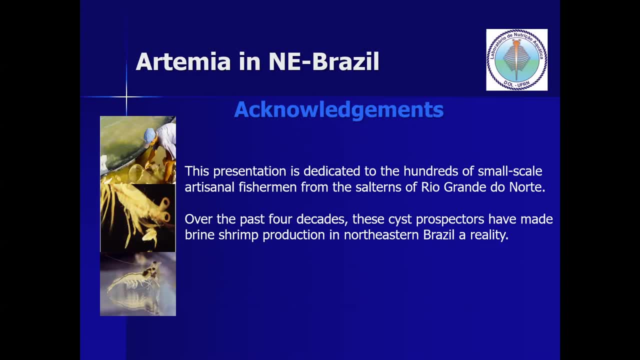 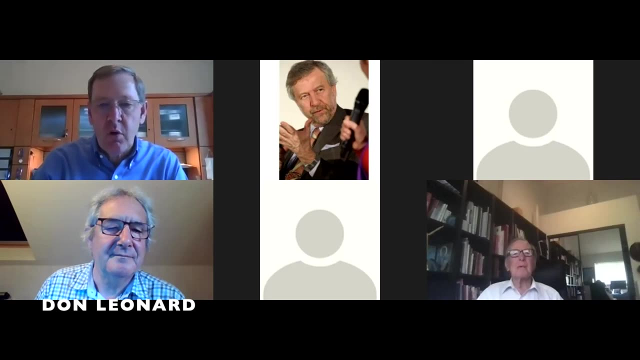 Over the past four decades, these CISP prospectors have made branching production in northeastern Brazil a reality. Thank you. My name is Don Leonard. I'm currently the chair of the Great Salt Lake Brine Shrimp Cooperative and have served as chair for the past 15 years and also as CEO of the Cooperative for 14 of those 15 years. 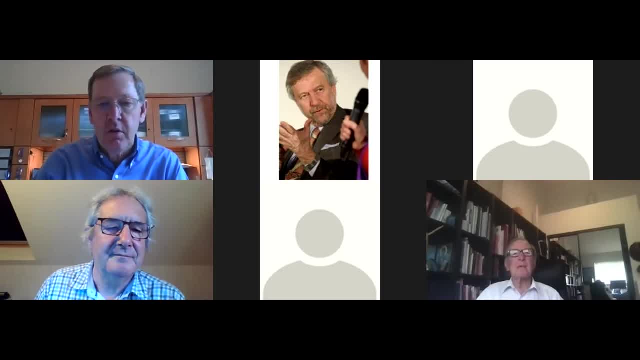 I've also served as president of the Utah Artemia Association for 27 years. I've been asked to take a few minutes to share the history of commercial harvesting of artemia from Great Salt Lake. Let me first share a few details about Great Salt Lake. Great Salt Lake is the largest saltwater lake in the entire Western Hemisphere. It's the fourth largest terminal lake in the world, which is why it retains a level of salinity that's ideal for artemia. Great Salt Lake is the 37th largest lake in the world. Its dimensions are 75 miles by 40 miles or 120 by 64 kilometers, and it does fluctuate in size due to annual variations in precipitation, but its average size is 1,730 square miles. Great Salt Lake is the largest saltwater lake in the entire Western Hemisphere. It's the fourth largest terminal lake in the world, which is why it retains a level of salinity that's ideal for artemia. Great Salt Lake is the most modern land. It has a limit of 324 miles, or 4,352 square kilometers, and is the second most dependent. 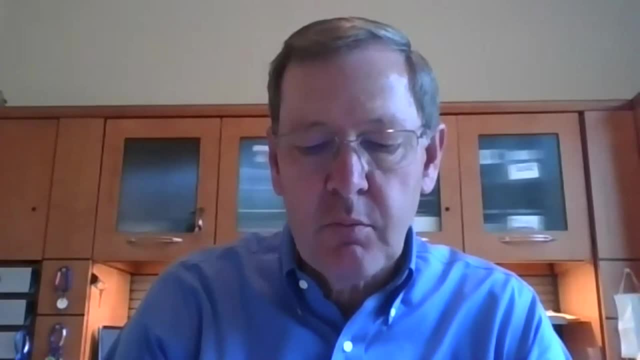 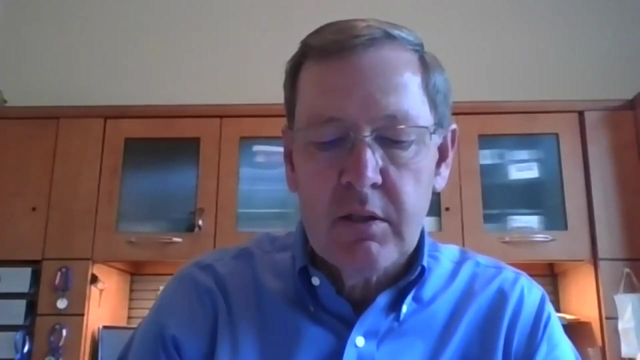 on Earth. It's important to note that Great Salt Lake is a Western Hemispheric Shorebird Reserve. Millions of birds rely upon Great Salt Lake as a stopover to gain mass and strength as they migrate. The current salinity of Great Salt Lake is 14%, or about 140 ppt in the South Arm. where the artemia flourish, but in the North Arm, where it's too salty to sustain independent populations of artemia. the salinity is 26 percent. The artemia industry on Great Salt Lake started in 1949,. 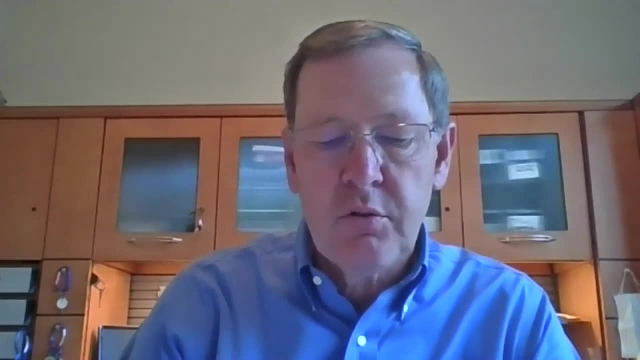 that's 72 years ago, when a tropical fish enthusiast from Ogden, Utah, named Cleon Sanders, heard that adult brine shrimp were a nutritious food that he could feed to his tropical fish. Initially, he had purchased frozen adult brine shrimp from San Francisco Bay. 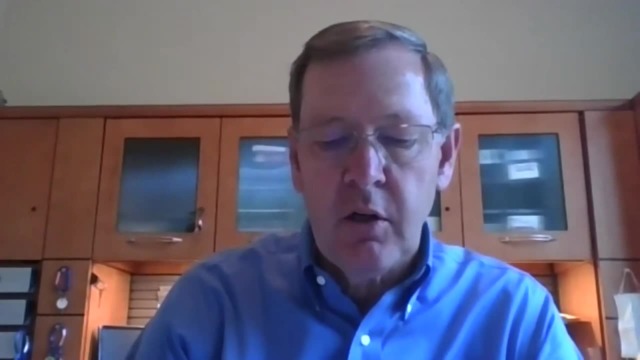 Then he heard from a friend that Great Salt Lake, right here in his own backyard, had large quantities of the tiny brine shrimp. A year later, in 1950, Sanders authored and sent an article to the Aquarium Magazine describing his fish food from Great Salt Lake. Shortly after his article, 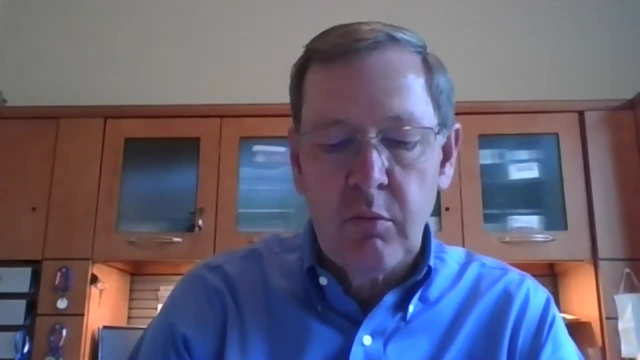 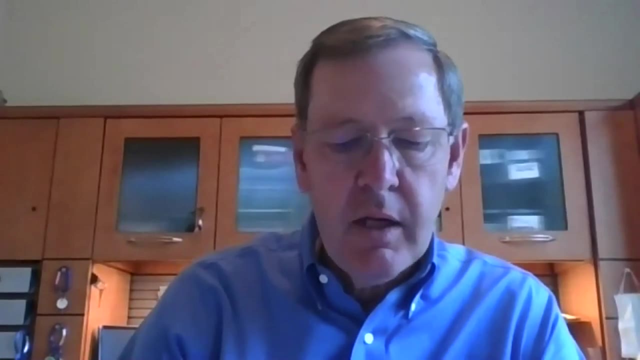 was published, he began receiving numerous requests for frozen adult brine shrimp from around the USA and formed Sanders Brine Shrimp Company to respond to those requests. In the 1970s and 1980s, the farming of various species of shrimp and fish was expanding globally. 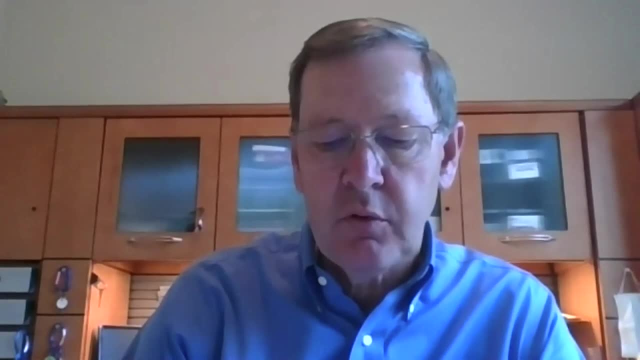 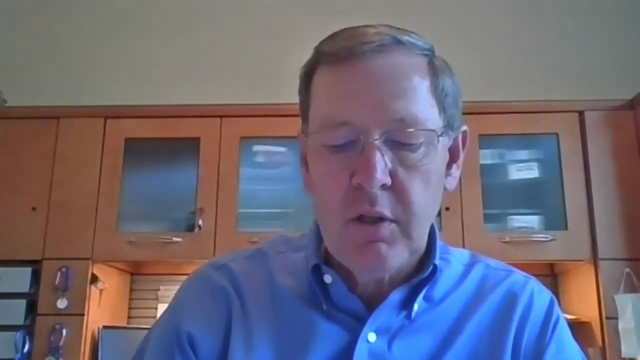 Newly hatched artemia anoplia had been found to be an ideal food for larval stage shrimp and for some species of larval fish. With the growth of aquaculture, the focus of the Great Salt Lake brine shrimp industry switched from. 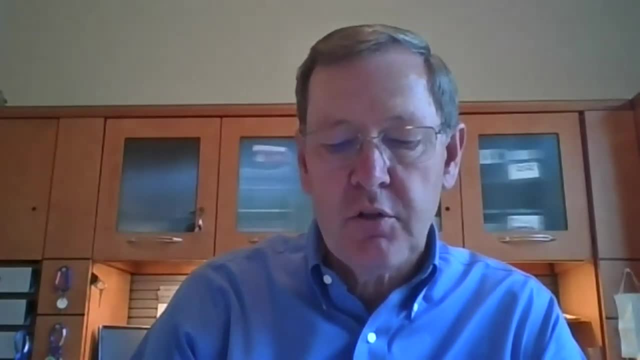 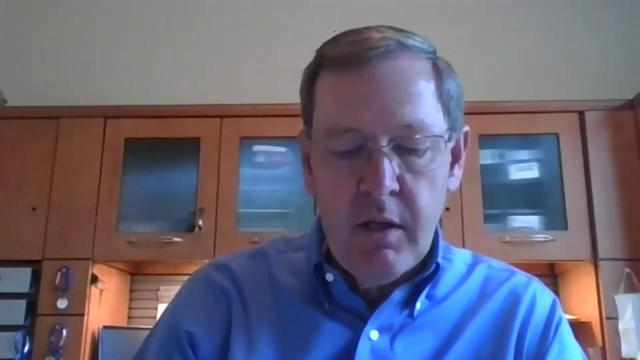 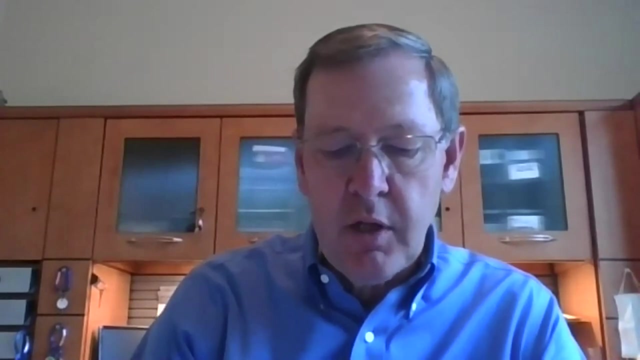 harvesting adult artemia for use by fish hobbyists to harvesting artemia cysts, also commonly referred to as brine shrimp eggs. It's important to note that, as Jim stated, cysts can be processed or dried and packaged for long-term storage so they can be shipped around. the world while making their way around the world. It's important to note that, as Jim stated, cysts can be processed or dried and packaged for long-term storage so they can be shipped around the world while making their way around the world. maintaining their hatchability, their nutritional quality and their other valuable characteristics. With this rapid growth of agriculture, demand for artemia cysts grew quickly and by the 1990s the Great Salt Lake brine shrimp industry had grown from 1 to 32 harvest companies. At that time, this increasing harvest pressure on the lake caused many of these companies to become concerned about the long-term health of the brine shrimp population and resource. You have to remember that by this time, in the early 1990s, excess harvest pressure had already. 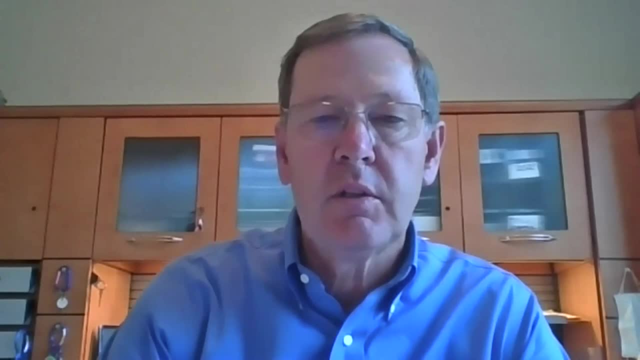 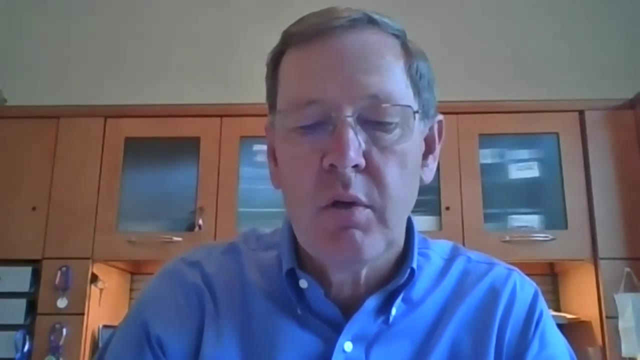 damaged or destroyed numerous fisheries around the globe. For example, the Peruvian coastal anchovy fisheries crashed in the 1970s. The sole fisheries in the Irish Sea, the West English Channel and other locations had become overfished to the point of virtual collapse. Blue walleye went extinct in. the Great Lakes in the 1980s. But it was the collapse of the cod fishery off the coast of Newfoundland in 1992 that really caught our attention. In the summer of 1992, the northern cod biomass fell drastically to just one percent of earlier levels and Canada declared a moratorium. 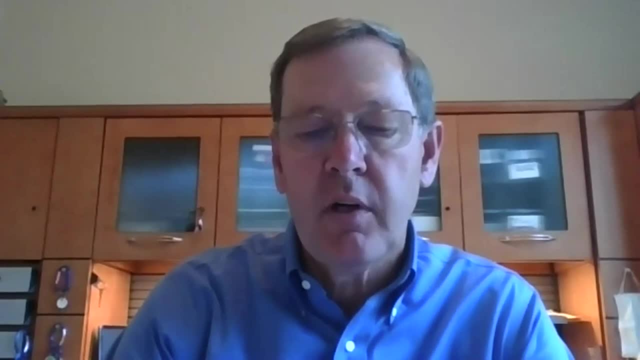 on cod fishing Of equal alarm. biomass available to feed the cod or the cod prey species and food chain virtually disappeared, undermining the ecosystem and leaving little hope that the cod could recover. In addition to the collapse of other fisheries around the world and to the rapid increase in harvest pressure on Great Salt Lake, we were 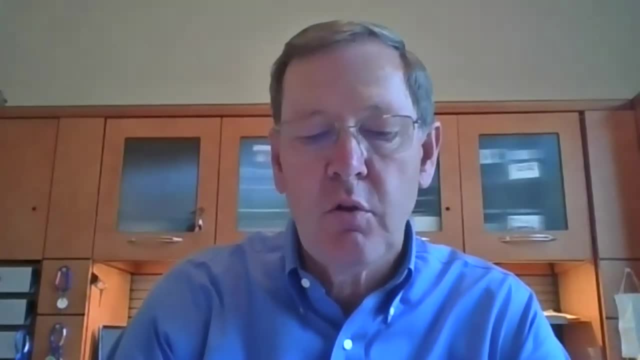 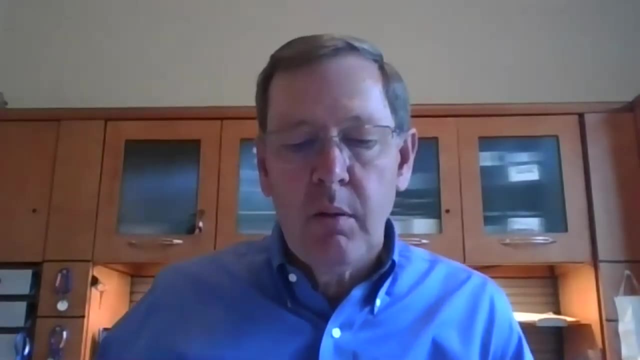 concerned about overfishing from Great Salt Lake because there was no formal state program to manage the brine shrimp resource, so there were no limits on harvest permits nor limits on quantities of product that could be harvested. There was no significant state research program for the brine. 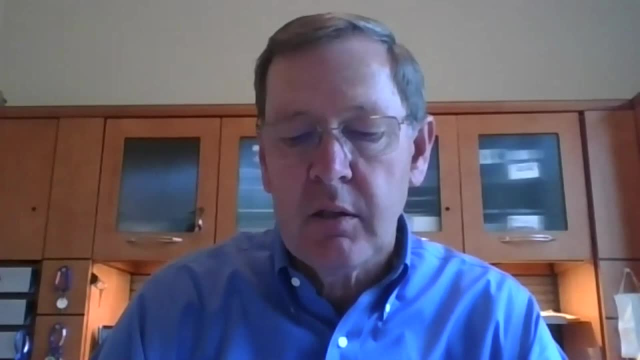 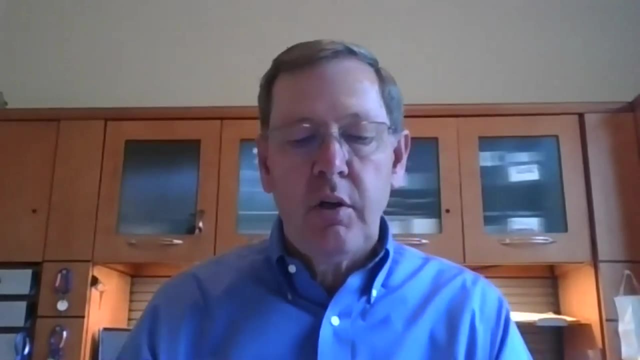 shrimp resource. so there's no understanding of how to preserve and protect Great Salt Lake Artemia And there was no state mandate to regulate the brine shrimp resource. So the Great Salt Lake industry approached the director of the Utah Division of Wildlife Resources and asked that. 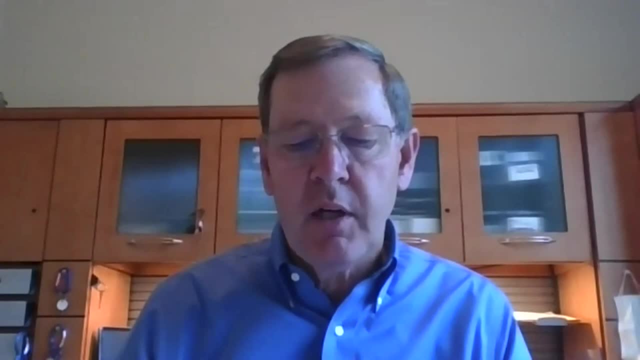 the state establish a program to manage and protect the Great Salt Lake brine shrimp resource. In support, the industry offered to provide additional ongoing funding for research management and compliance With this new research data and with the support of the industry, the Utah established a sustainable management model for brine shrimp in the Great Salt Lake. Since all adult artemia in Great Salt Lake die in the winter due to cold, lack of feed or other causes, the Utah Division of Wildlife Resources determined the number of brine shrimp eggs that must be left in the lake. at the end of the harvest season, which ends on January 31 of each year, to assure that the brine shrimp population would reemerge each spring. That equation, developed by the Division of Wildlife Resources, takes into account such factors as winter cyst survival, avian requirements, egg hatchability and other factors. 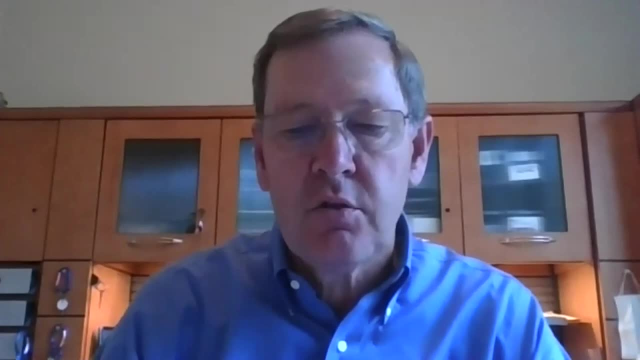 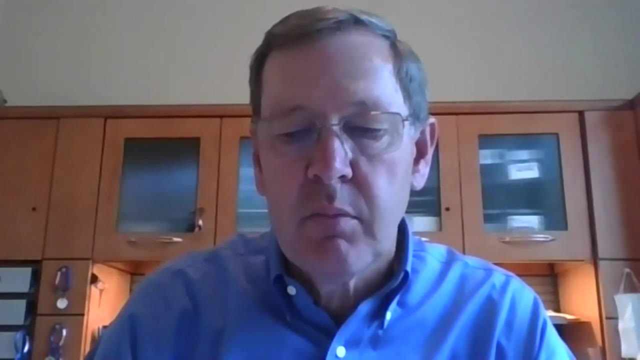 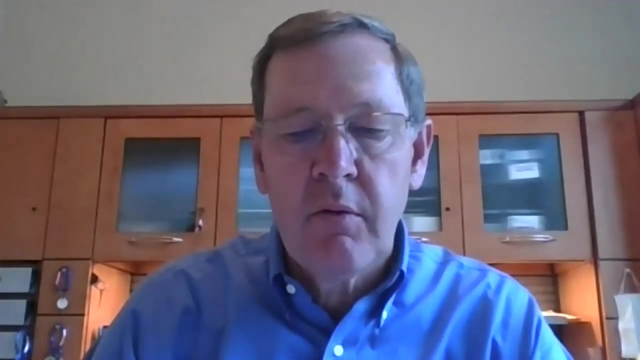 This sustainable management model allows the industry to harvest only the excess artemia cysts, with that excess being determined to be those cysts above 21 cysts per liter of water in the Great Salt Lake. This resource management model has succeeded in creating a natural, sustainable brine shrimp resource that supplies both the avian populations. and the industry with vital artemia cysts, while preserving a healthy natural population of brine shrimp in the lake. The State of Utah's resource management plan for artemia has been so successful that it is touted as a model of successful government and industry collaboration. 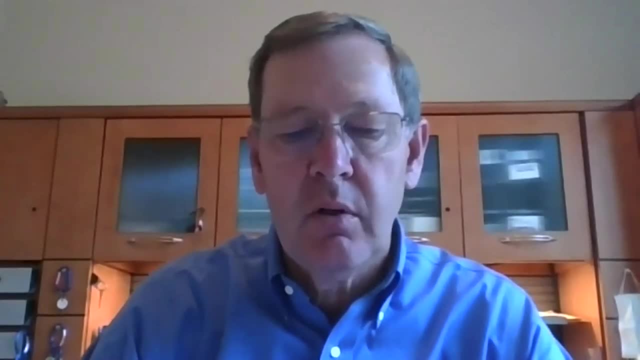 As a result, Great Salt Lake is a reliable- in fact it's the most reliable- artemia resource in the world. It's the world's largest supplier of quality artemia cysts And, of important note, annual average supplies of artemia cysts from Great Salt Lake. 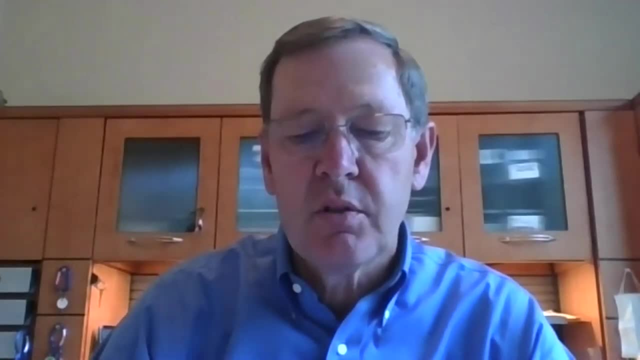 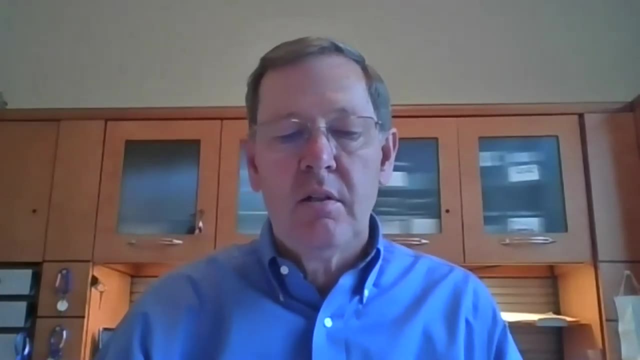 have steadily increased since implementation of the State's management plan, And GSL is by far the world's most sustainable artemia resource. The State of Utah's artemia resource management plan will continue to preserve and protect the Great Salt Lake brine shrimp resource. 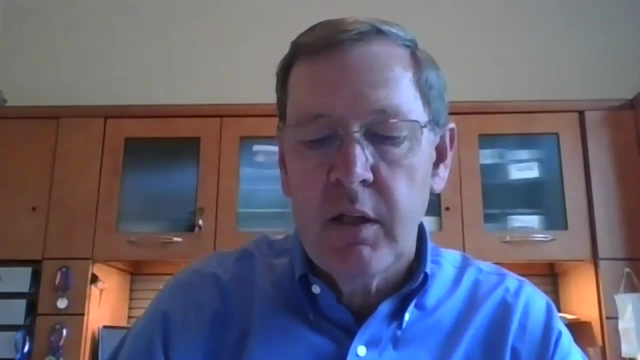 because Utah established the Great Salt Lake ecosystem program to regulate the harvest, to research and monitor the resource and to preserve and protect a healthy brine shrimp population in the Great Salt Lake. At our request, the State also established a standing technical advisory group. 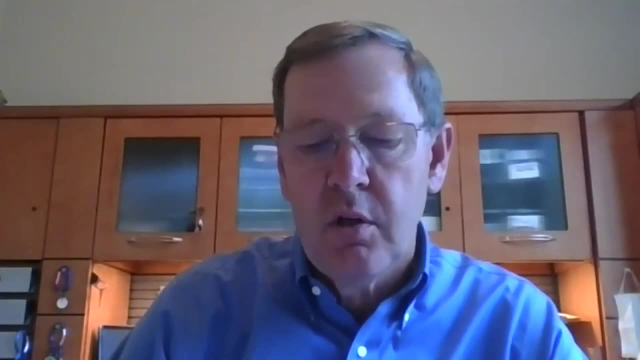 which is a science peer review committee to oversee research on brine shrimp in Great Salt Lake. The industry contributes funding for that research. We also share our own ongoing research with the State and we serve on the State's technical advisory group. So we're very optimistic about both the quality and the supply. 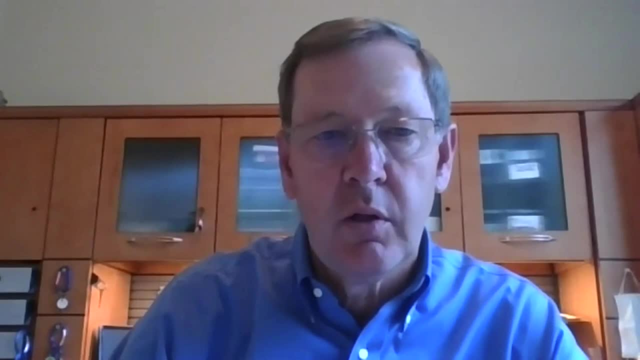 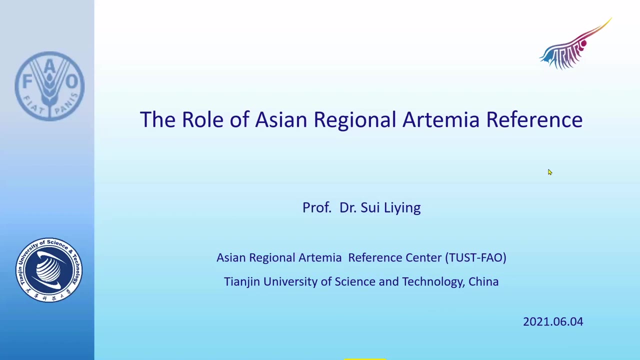 of Great Salt Lake artemia going forward. Thank you, Hello. Good morning, good afternoon and good evening everyone. So first of all I should thank a lot for the invitation from Saxon and Patrick. My name is Liying Sui. 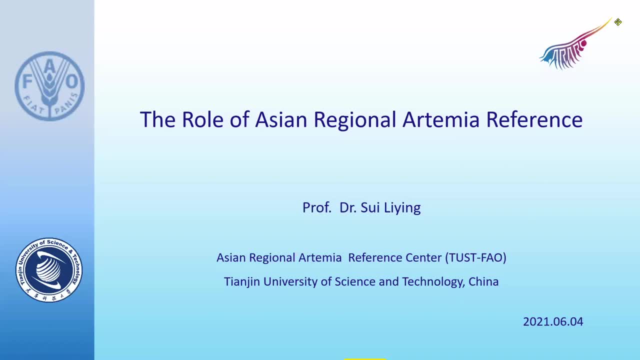 I'm the professor at Tianjin University of Science and Technology and I'm also the director of Asian Regional Artemia Reference Center. My experience on artemia research and application can be dated back 30 years ago. In the meantime, I have obtained my master and PhD doctorate degree. 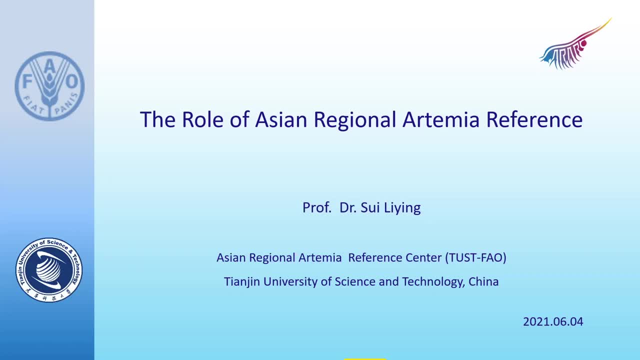 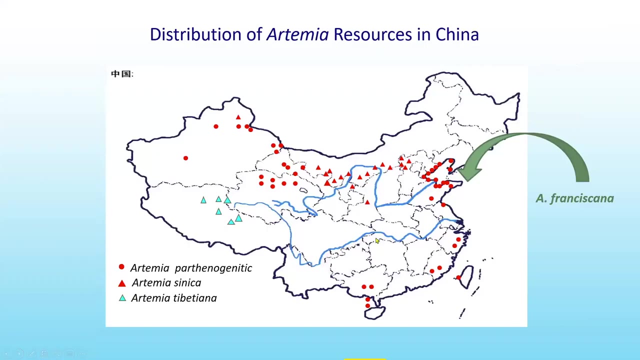 at Ghent University under the supervision of Professor Patrick Sogolos. So next, please, Patrick, Patrick, please, Yes. So I would like to start my presentation with the history of artemia resource exploration and utilization in China. China is rich in artemia, biodiversity and resources. 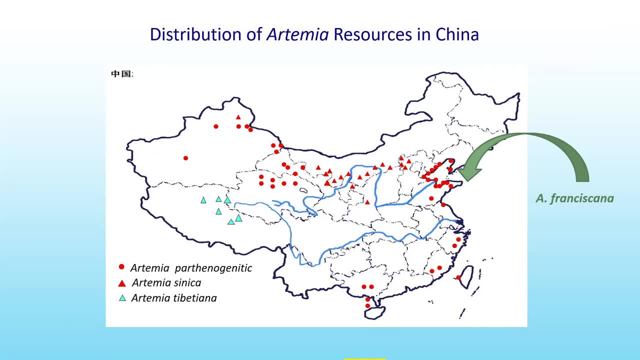 Artemia cinica and artemia tibetiana are the two indigenous artemia species, while personagenetic populations also exist in the salt works and the salt lakes. Since early 1990s, franciscana- artemia franciscana- have been existed in the Bohai Bay salt works. 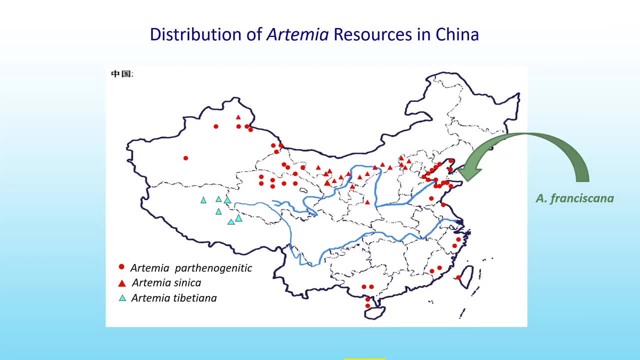 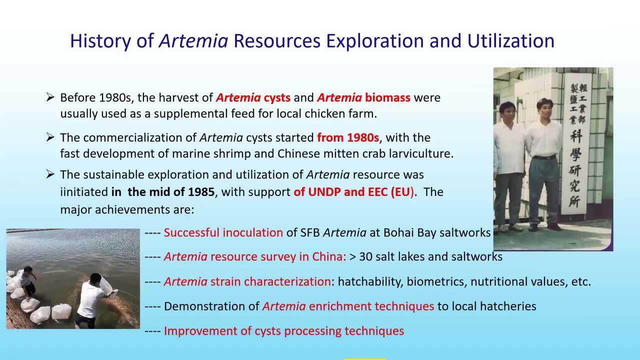 as the result of inoculation of artemia cysts from San Francisco Bay Before 1980s. the artemia cysts and biomass are usually used as a supplemental feed for the local chicken farm, resulting in a bright orange color of the egg yolks. 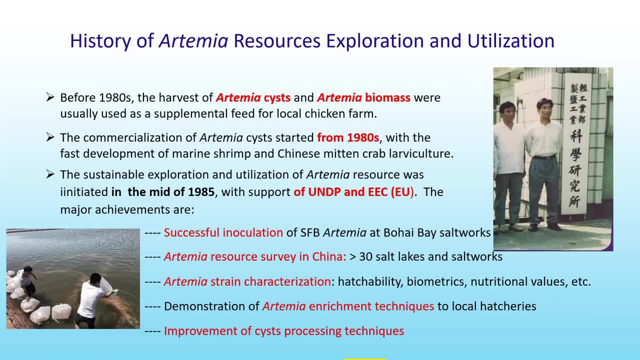 However, the commercialization of artemia resources in China only started from 1980s, later 1980s, along with the fast development of marine shrimp and the Chinese meat and crab lauriculture. Nevertheless, the yield and quality of artemia products are unstable. 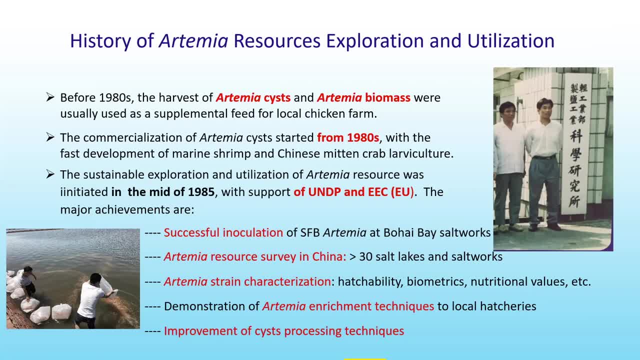 and unsatisfied. The study was initiated in 1985 at Salt Research Institute of China about artemia with the support of the UNDP, of the United Nations and the EEC, the previous EU, The overseas artemia expertise, especially the team from Ghent University. 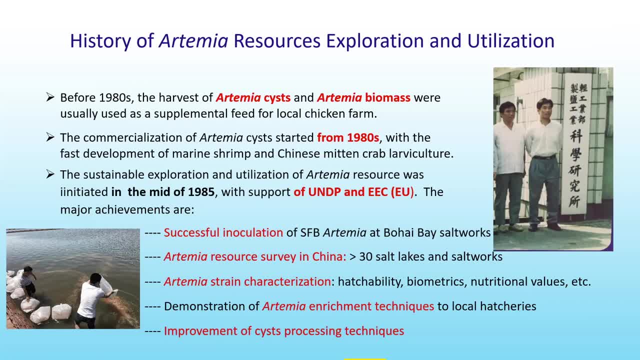 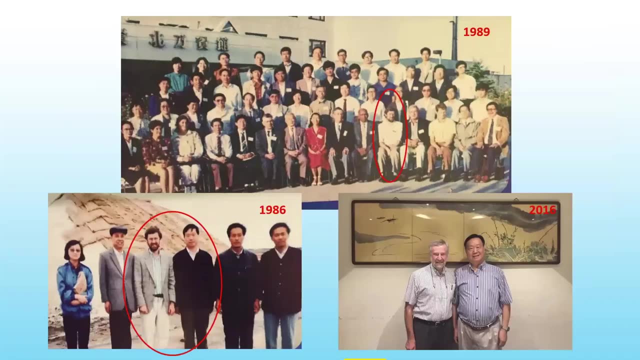 have made very important contributions to the initiation of sustainable exploration and utilization of artemia resources in China In the following 10 years. many progresses have been achieved. Next, By working together, people have made long-lasting friendship. So you can see the face of young Patrick. 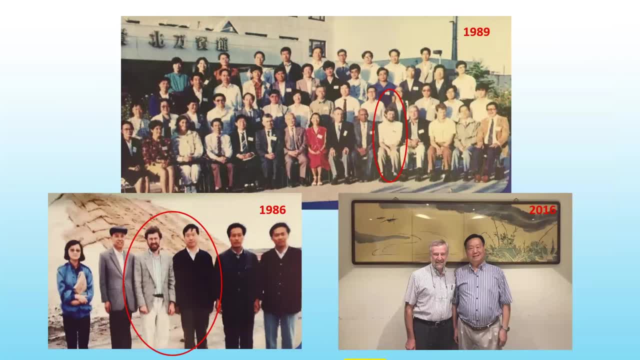 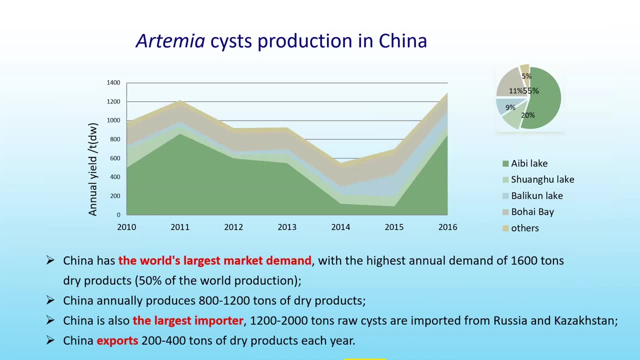 more than 30 years ago. Next, China has the world's largest market demand on artemia cysts. It is also the number one cyst producers and importers in the world. China also exports products to the other Asian countries. Next, 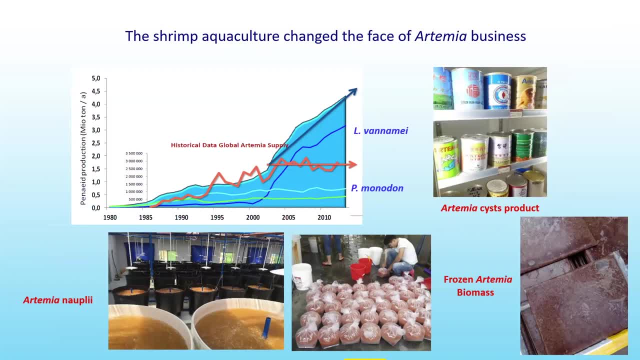 At present, more than 70% of the cysts are sold to the shrink hatcheries. Except for the cyst products, artemia are also sold in form of newly hatched artemia, noplii, fresh and frozen biomass, as well as decapsulated cysts. 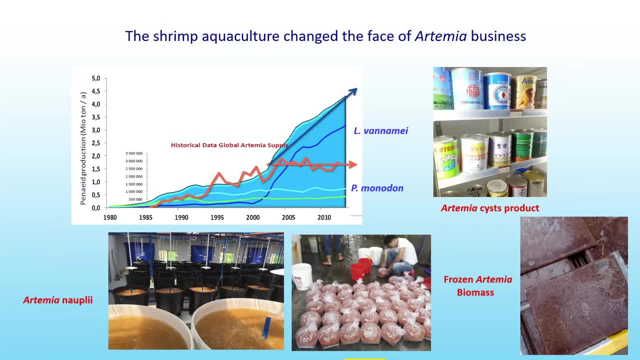 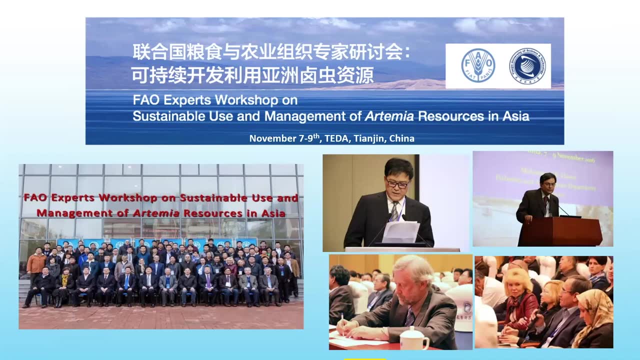 to be used in shrink hatchery, nursery and broodstock maturation. Next, Owing to the vital role of China in artemia resources producing and consuming, and to the faster development of aquaculture industry and increasing artemia consumption in Asia. 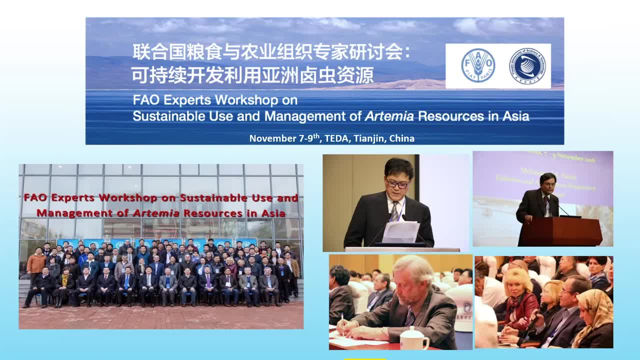 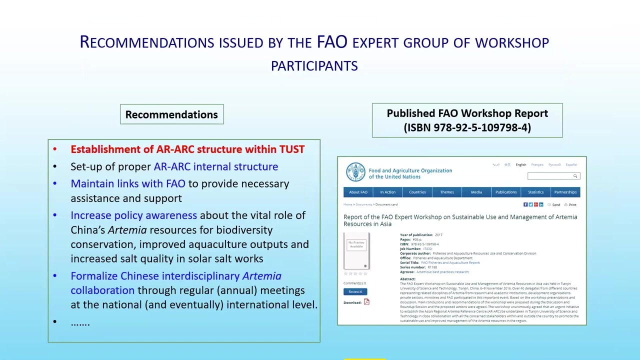 FAO expressed their interest in establishing a regional artemia reference center in Asia. In November 2016,. FAO exports workshops was successfully organized in Tianjin, China. Next, The establishment of Asian regional artemia reference center in China. 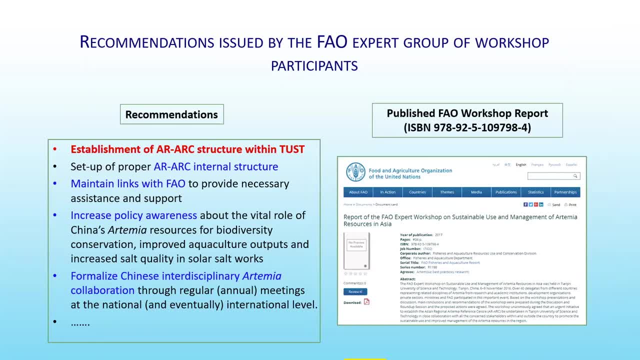 was recommended by the participants at the workshop, With the tremendous support of FAO and our university, Tianjin University of Science and Technology. the laboratory set up at ARRC has completed in the time of one year, So in April 2018,. 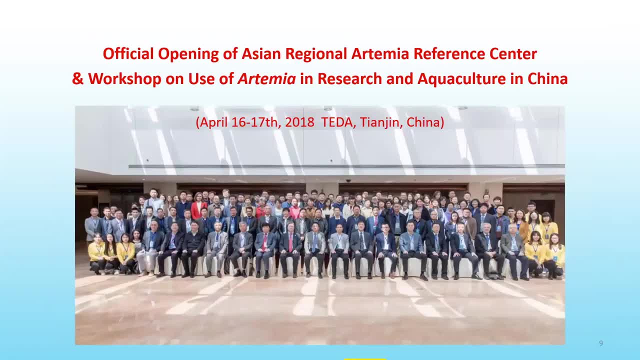 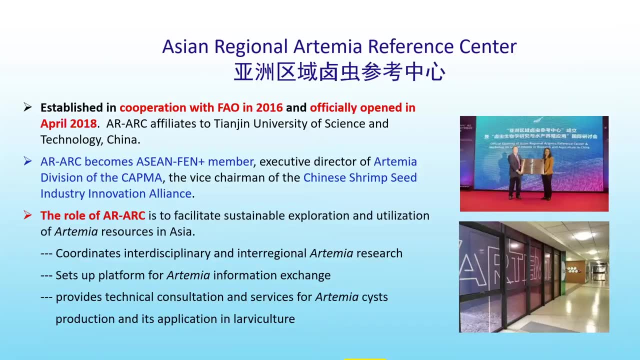 next, please. the official opening of ARRC and artemia workshop were held in Tianjin Next, So the role of ARRC is, of course, to facilitate the sustainable exploration and utilization of artemia resources in Asia through coordinating interdisciplinary. 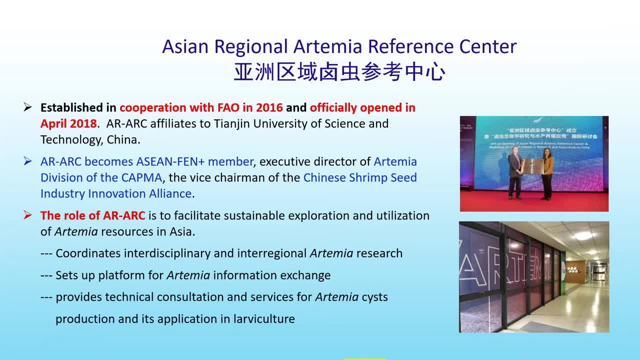 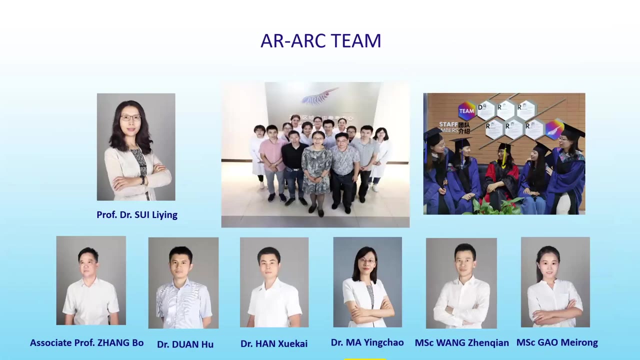 and inter-regional artemia research, setting up platform for artemia information exchange, providing technical consultation and services for artemia assist production and its application in larvae culture. Next, We have quite young staffs with specialized experiences and innovative consciousness. 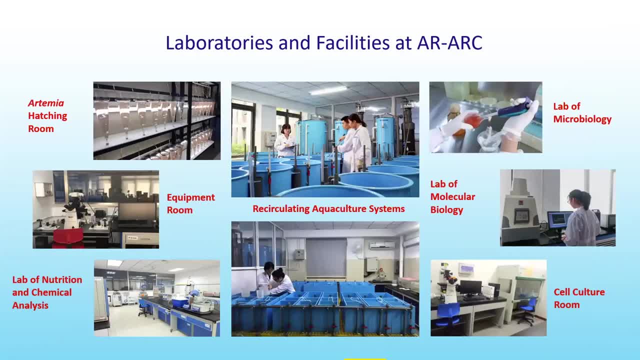 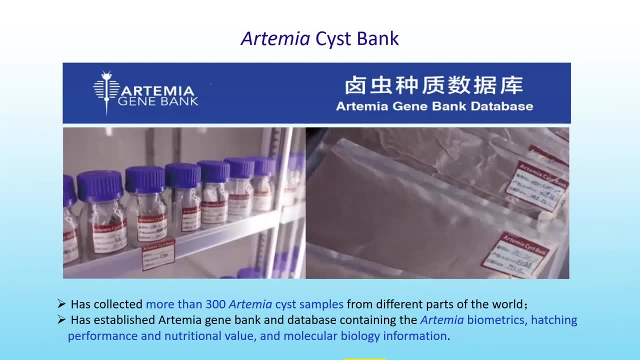 Next, And we have also advanced the laboratories and the research facilities at ARRC. Next, ARRC have preserved more than 300 artemia assisted samples and set up the database and providing and exchanging the samples with the other institutions for scientific research purpose. 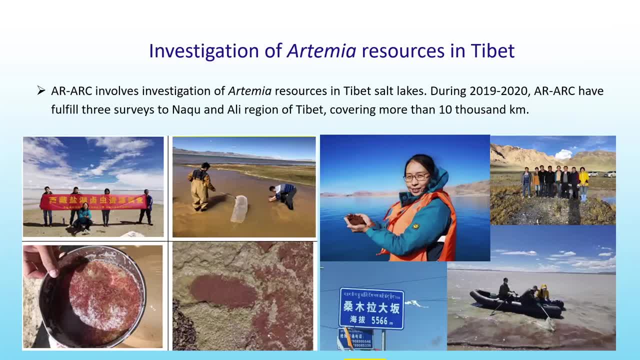 Next, Since 2019, we took initiative to survey the artemia resources in the salt lakes in Tibet. The world has the plateau. Tibet artemia has unique phenotypic characteristics in terms of dark red color, the very big size of cysts. 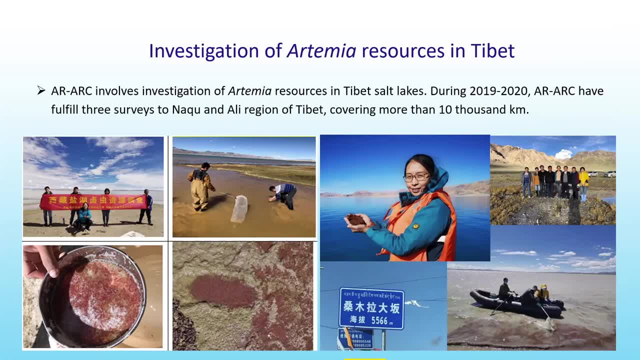 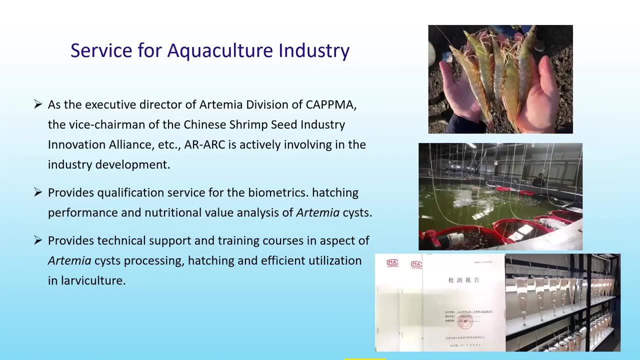 and high EPA and DHA content. Lots of artemia samples were collected from the altitude above 4,000 to 4,500 meter. Next, The services to the aquaculture industry is one of the main tasks of ARRC. 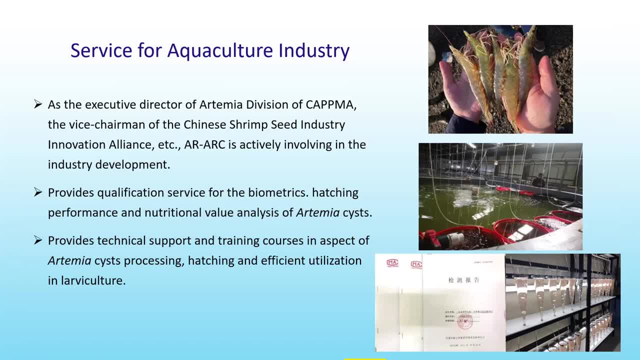 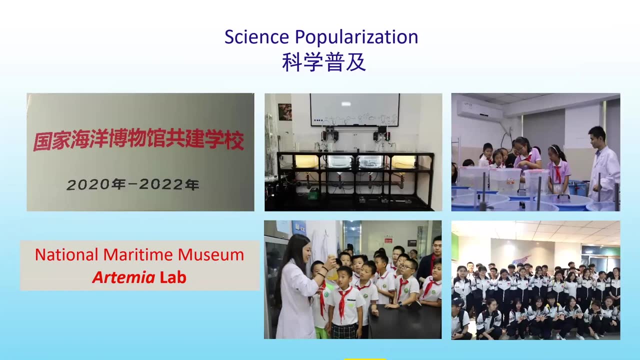 We provide the technical supports and training courses to the private sectors, to the communities in China and in the Asian region. Next, please, ARRC has made efforts for the science popularization. We have set up an artemia laboratory at the National Maritime Museum of China. 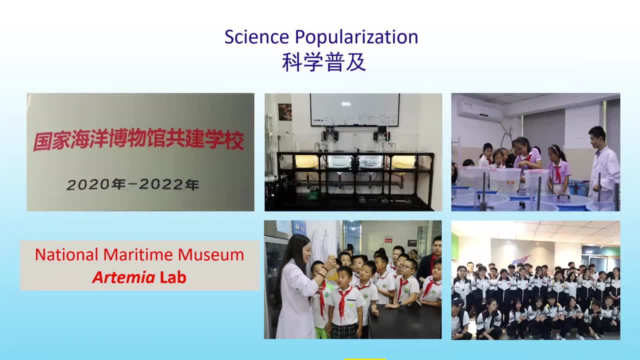 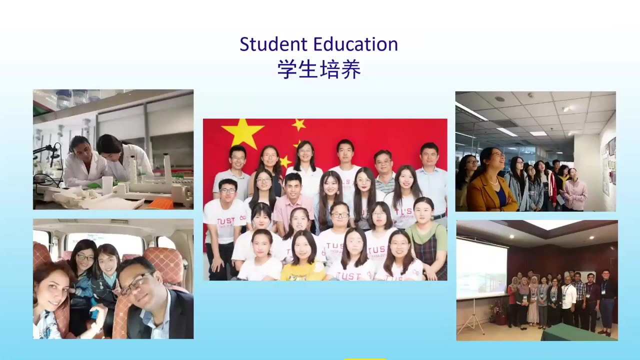 and provide short courses to the visitors. Each year, ARRC have also received lots of students from the local schools to learn about artemia and the other marine organisms. Next, Our PhD, our master and undergraduate students have also contributed a lot to the artemia researches. 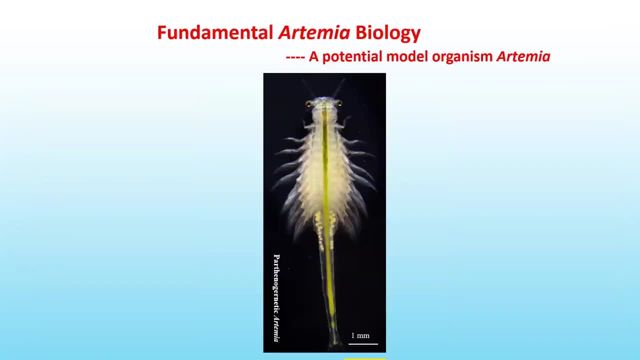 and the practical work at ARRC. Okay, next, The last but not the least, I would like to share our recent fundamental research results related to artemia biology. As you all know, artemia is such a unique zooplankton. 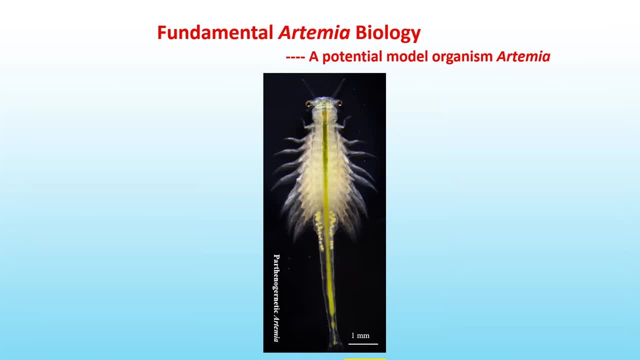 with special life phenomenon, for example the high salinity tolerance, the ovoviviparous or ovoviviparous offspring production, the dormancy and diapause termination, etc. So it is necessary, we think, to make artemia as a model organism. 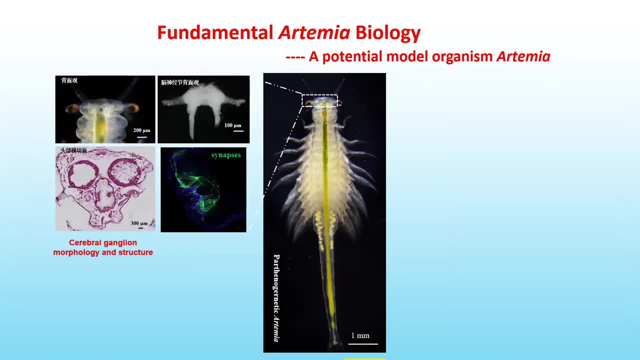 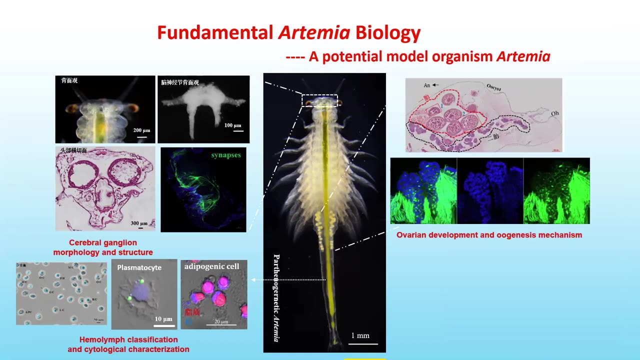 for scientific research, Patrick, please, One by one. yes, So far: the cerebral darling. morphology and structure, the classification and cytological characterization of the hemolymphy, the ovarian development and oogenesis mechanism and the morphology and the cytological characterization. 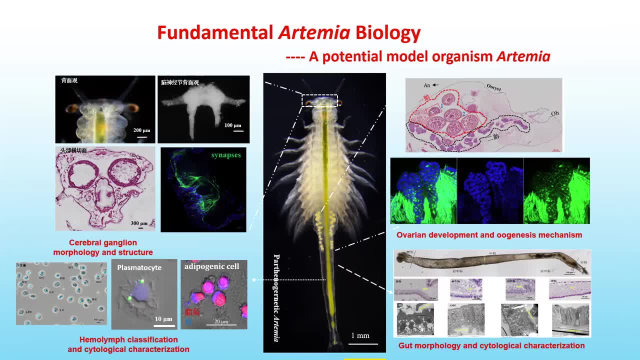 of artemia gut have been studied at ARRC. Most of these results are the brand new and, what I can say, the original study. We believe that this will facilitate the progress of developing artemia to model organisms in the near future. 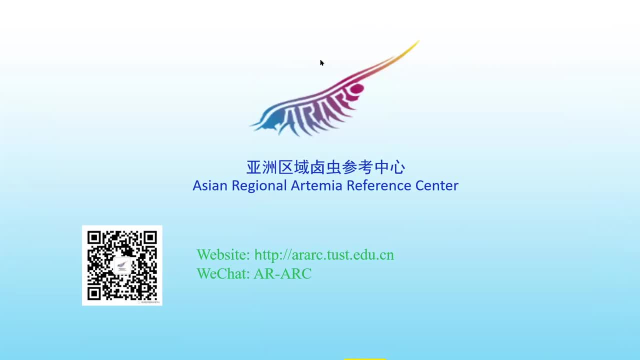 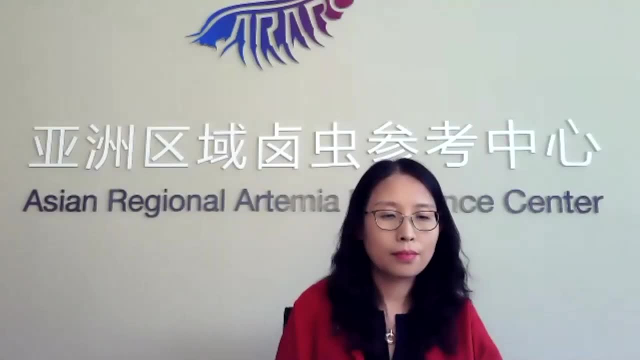 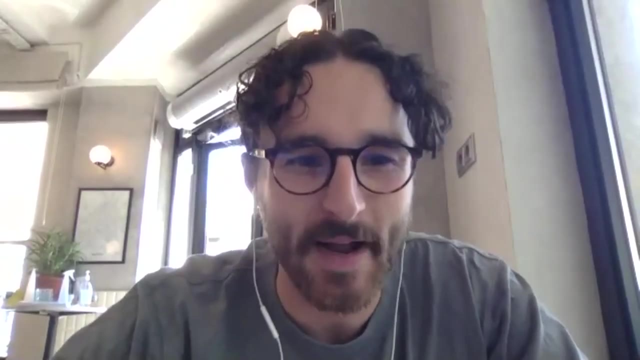 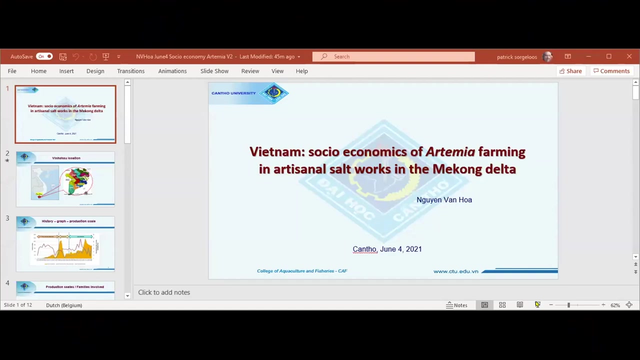 That's all for my presentation. Thank you very much. Hello again. Thank you so much for that brilliant presentation, Probably an award for the most beautiful backdrop of this meeting as well, with what you've got behind you, And also brilliant to see a young Patrick there. 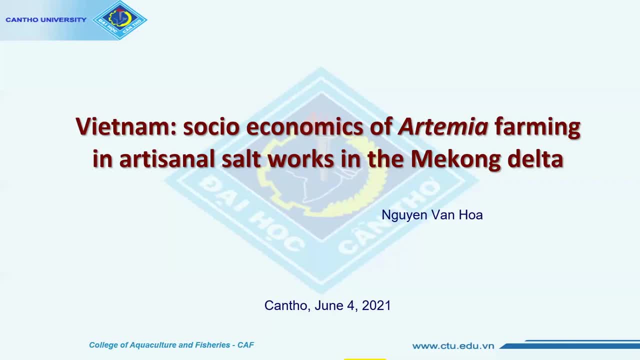 looking like a 70s rock star. Thank you so much for that. Many, many questions coming to my mind, But I believe we will pass the floor on now to Nguyen, Please. Thank you, You have the floor. You switch on camera. 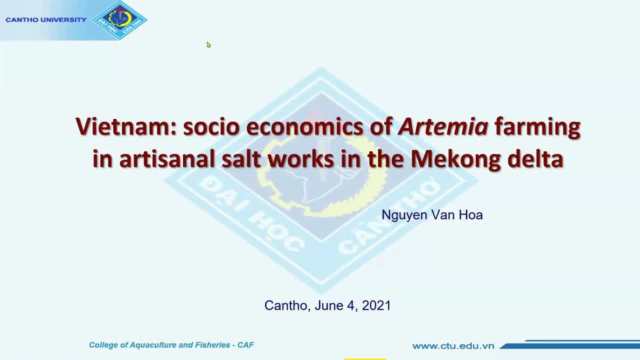 and unmute and you can start. All right, Hello everyone, To continue with. can you hear me, Patrick? Yes, OK, OK, Because it seems to be that the connection from my side is not very smooth. So I try to do my best. 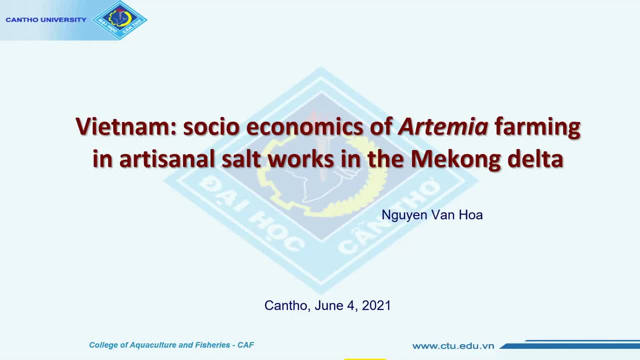 To continue with my presentation, first of all, most of you know who I am. My full name is Nguyen Van Hoa. I'm now a lecturer in Can Tho University, So we have a long term collaboration with Nguyen University for the academia research. 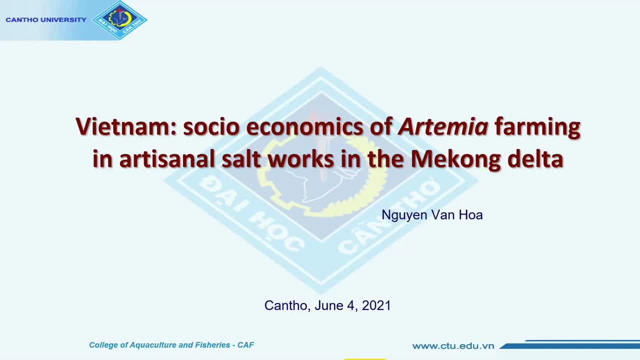 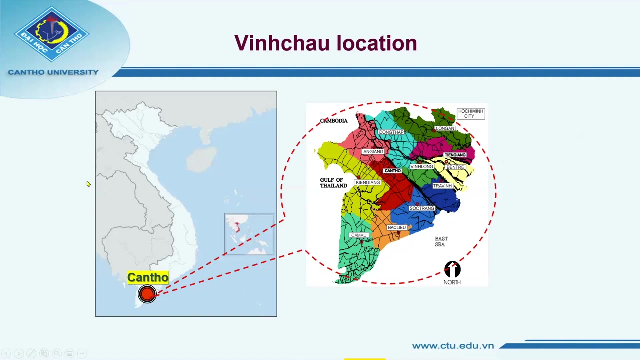 and application in the Mekong Delta, Vietnam. So my presentation today is to bring up only the social economic aspect of academia, farming and the solar source work in the Mekong Delta. Next, Patrick. So for some of you you know already where Vietnam is. 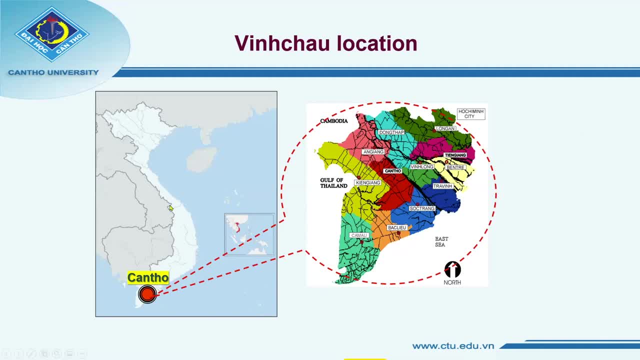 But the rest, just consider that Vietnam is located in the Southeast Asia And Vinh Chau location where we're going to do the academia. stay in very south of the country where you can see that, the Sop Trang and Bac Lieu and the East Coast. 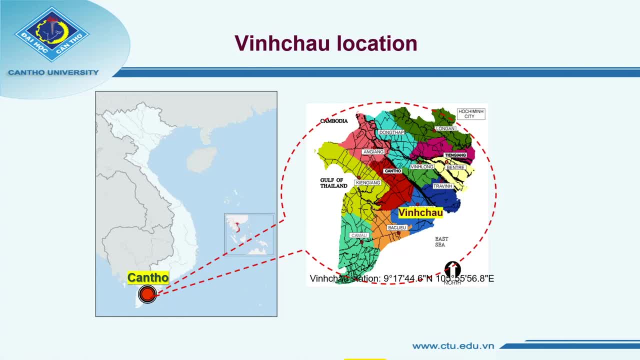 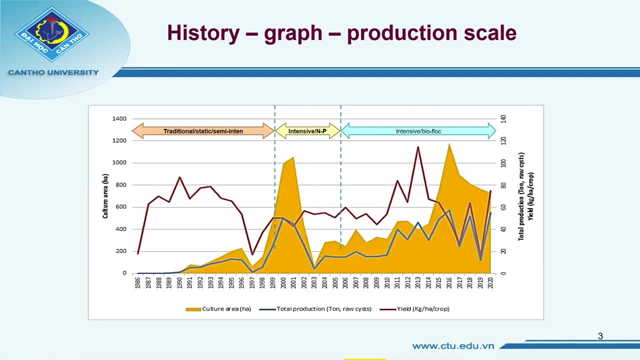 cultural life Netflix. So the figure here to illustrate that the activity of academia culture or production in Vinh Chau and Bac Lieu since 1986 until recently. So to bring up the information about the culture area, the total reaction and the year. 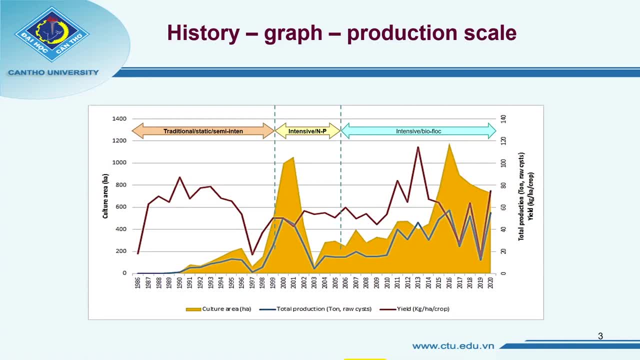 they are going up and down because of so many factors, But up to now the area. they can produce up to 60 tons of the weight weight of academia seeds And they can fulfill the needs of the local culture perfectly. So if you follow, 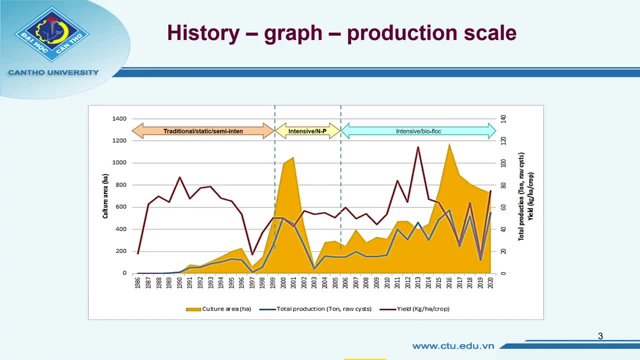 the course of the time you see that the different culture system of farming system have been applied. But we start with traditional and then follow with intensive system And now also intensive. but we apply the technology with the aim to save the environment and also to enhance. 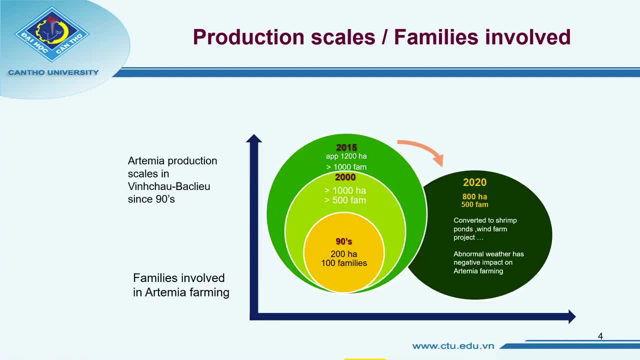 the seed production Netflix. So this graph to bring up the figure, that where you can see that we started in the year 90, a little bit earlier of 90. But up to 90, you see almost two of academia farming with 100 families involved. 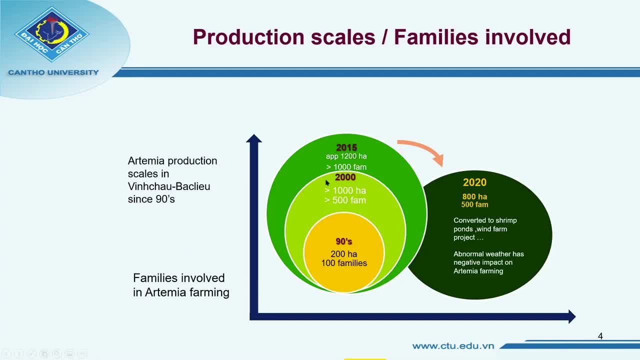 And later on up to the year 2000,. the culture area go up to 1000, where you have 500 families, And 2015,. on the day it increased up to 1,200. at that time, 1,200. 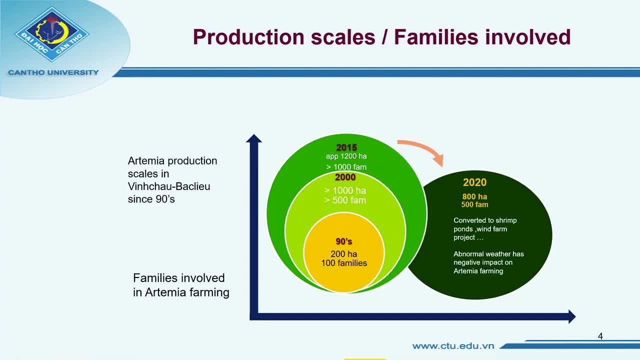 and more than 1,000 families, So it means that three, four, five farmers involved. However, until the year of 2020, only 800 hectares from 500 families involved because different reasons, where you can see that most of them. 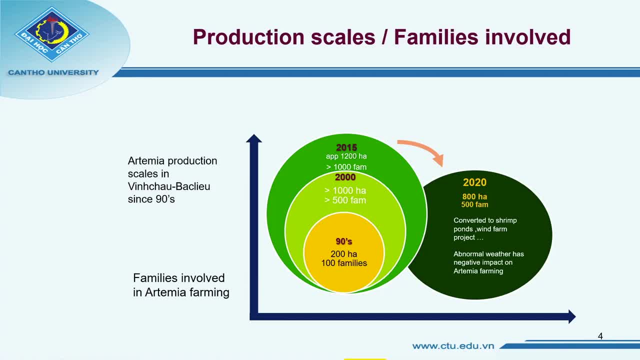 they also refer to do for the stream farming on the local area. They switch into the wind farm project for energy At the meantime. the big problem that the local people they have to face with the abnormal weather where you can see that, the early rainy season. 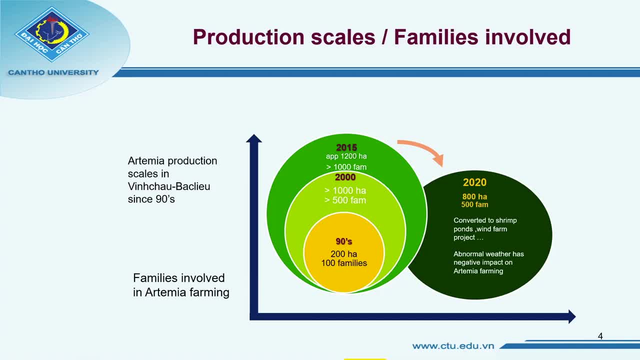 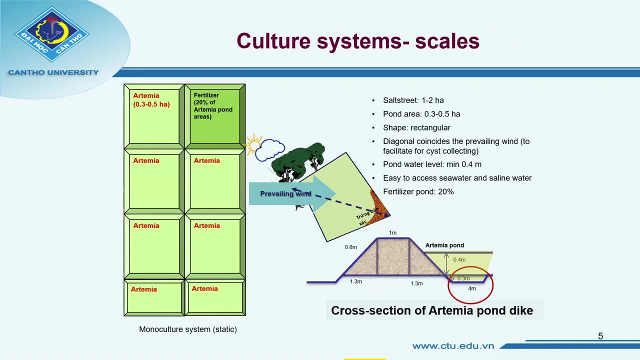 and also very short dry season. Therefore, the production area become less and less. However, we try to enhance the afternoon production by improved technical protocol. Next, please So to bring up just the information that we have in this presentation. First of all, 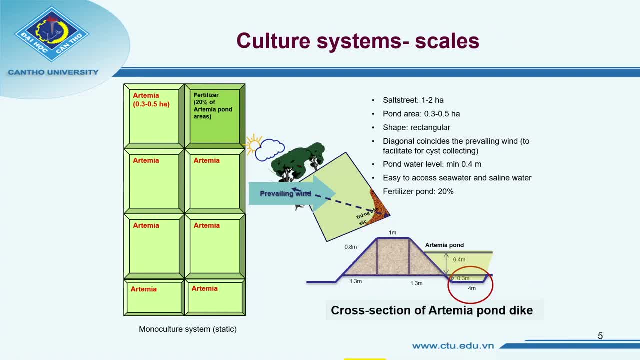 I would like to share with you some of the most important things that you need to know in this project First of all. I would like to share with you some of the most important things that you need to know in this presentation, First of all. 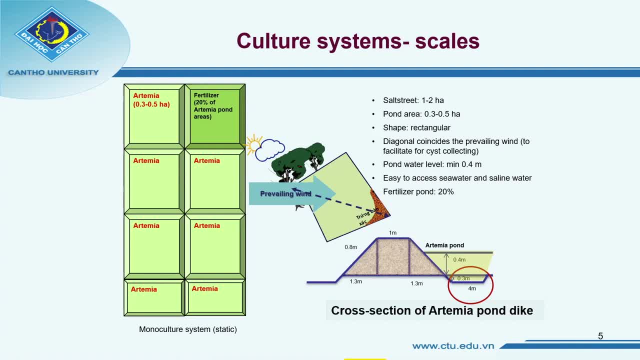 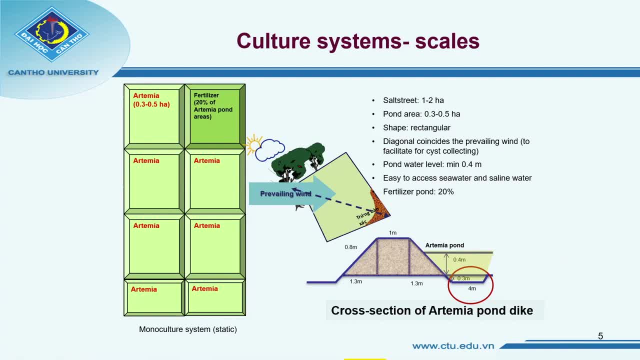 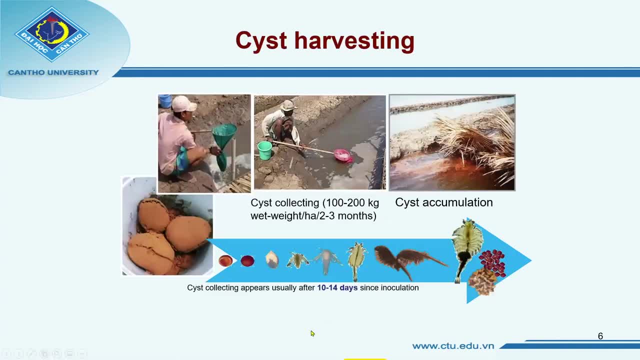 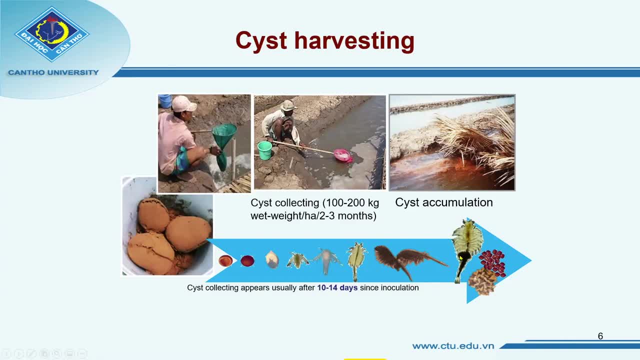 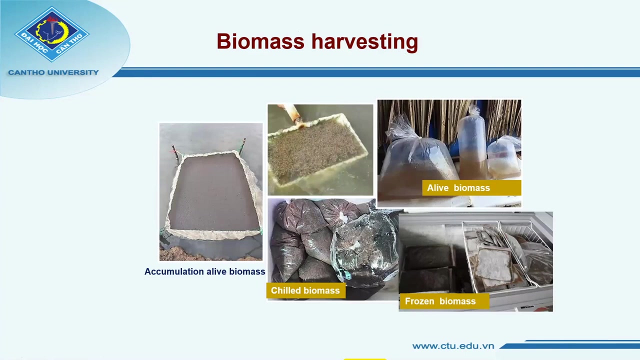 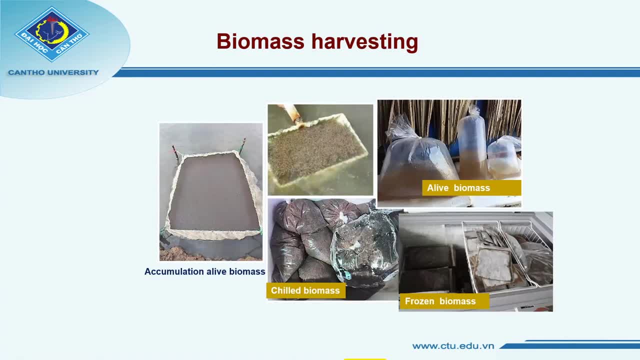 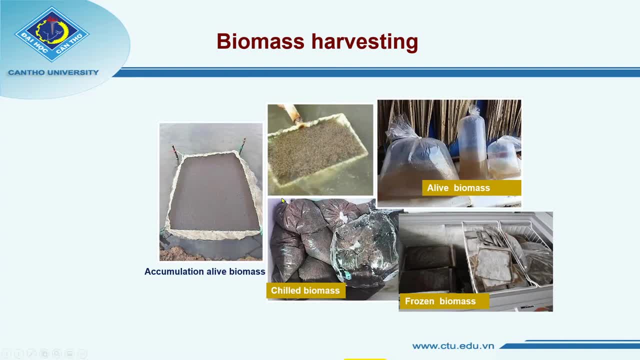 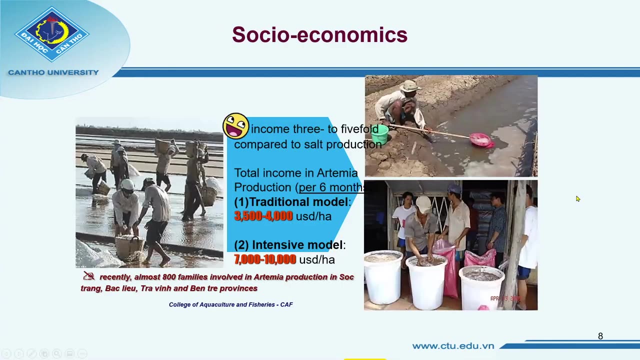 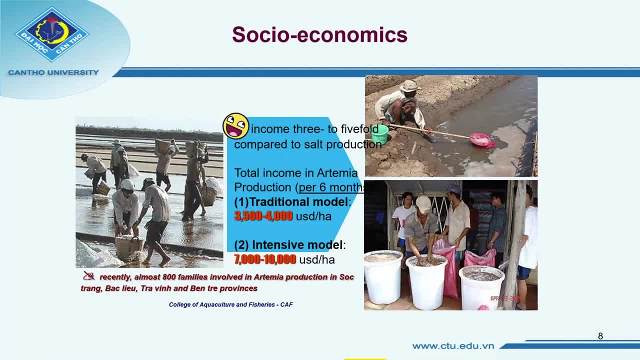 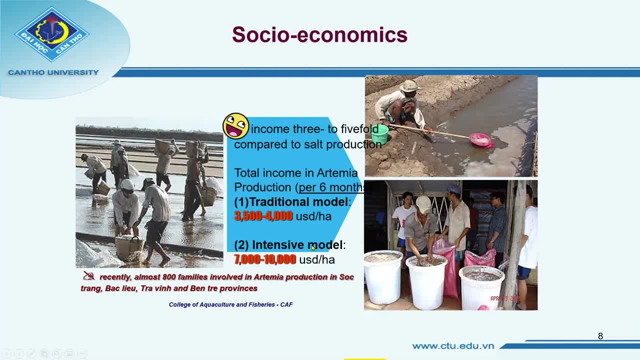 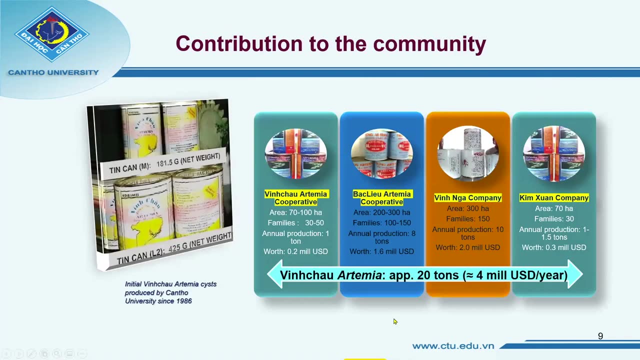 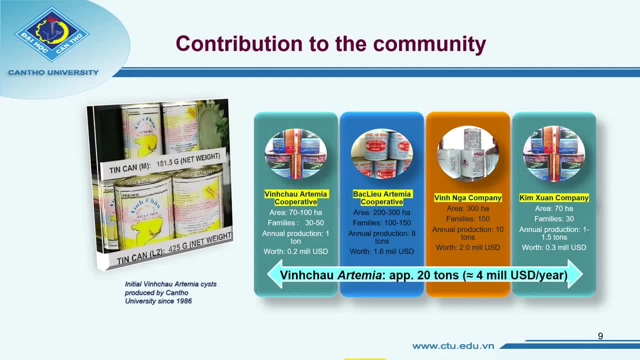 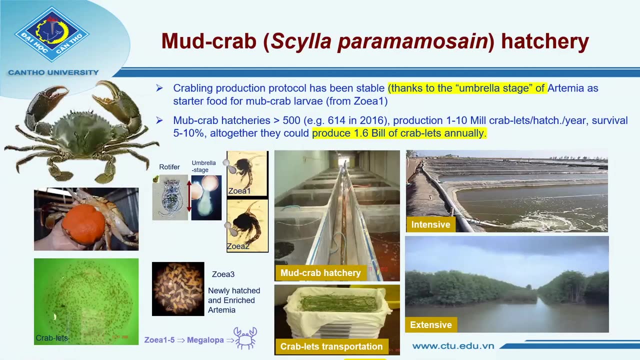 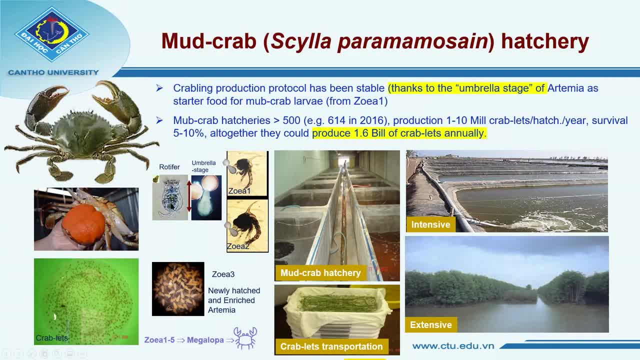 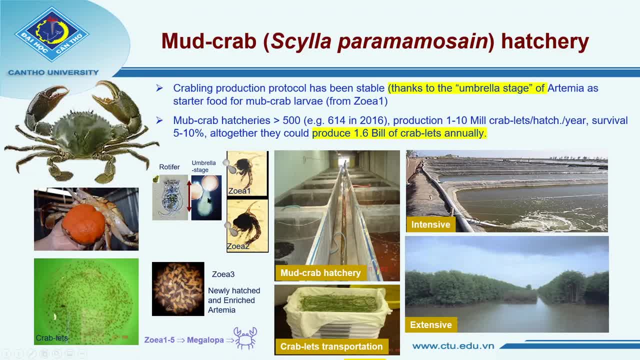 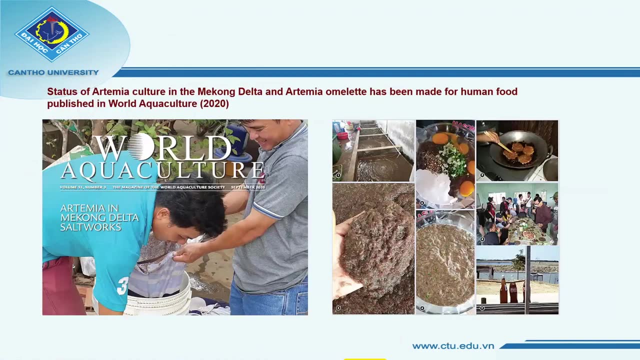 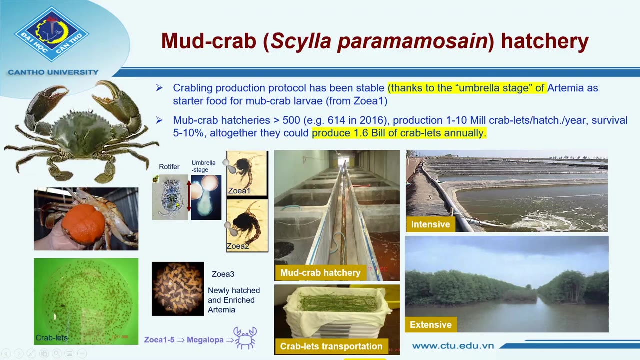 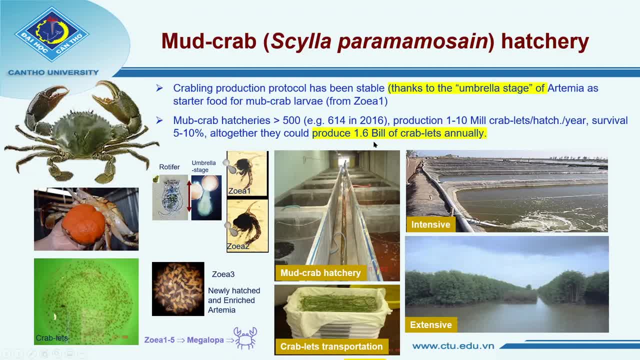 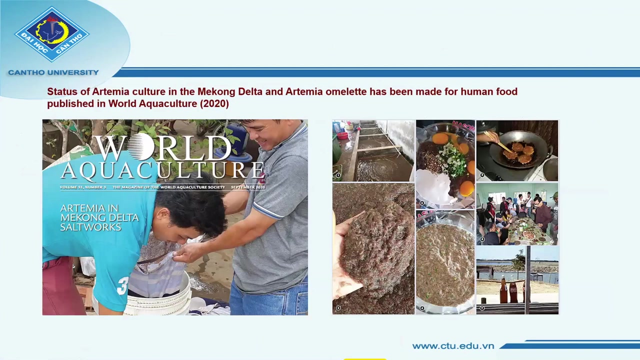 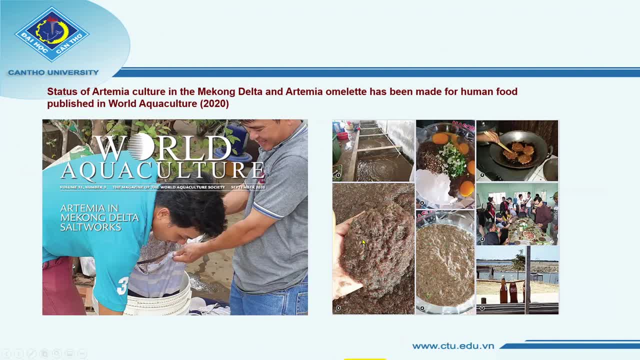 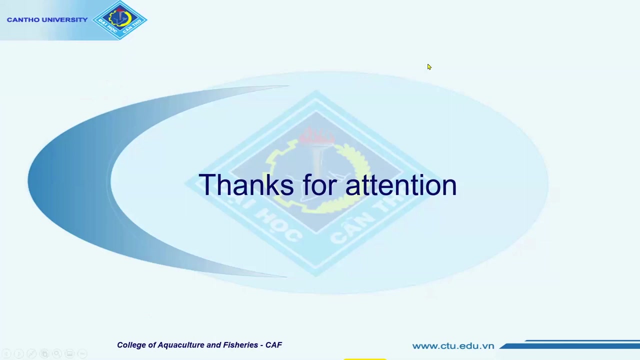 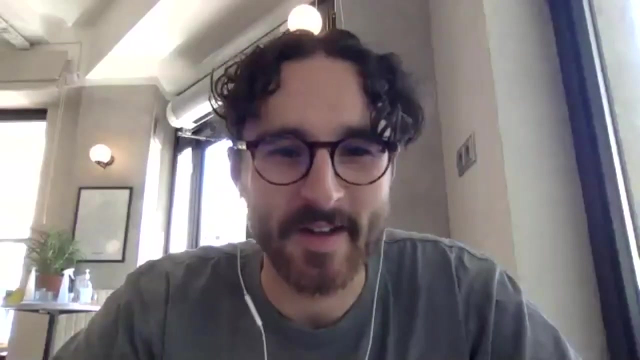 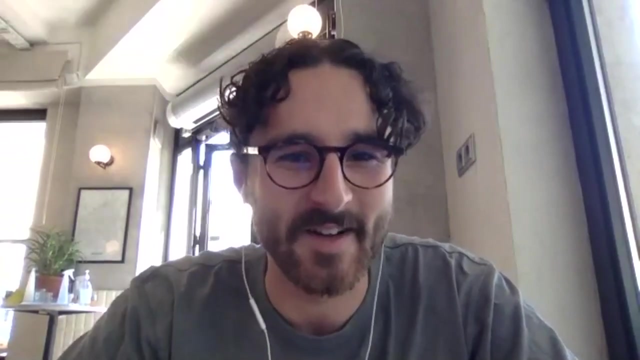 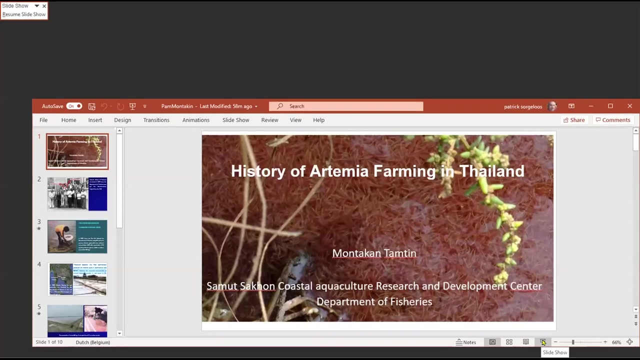 I would like to share with you some of the most important things that you need to know in this presentation. Next, I would like to share with you some of the most important things that you need to know in this presentation. First of all, I 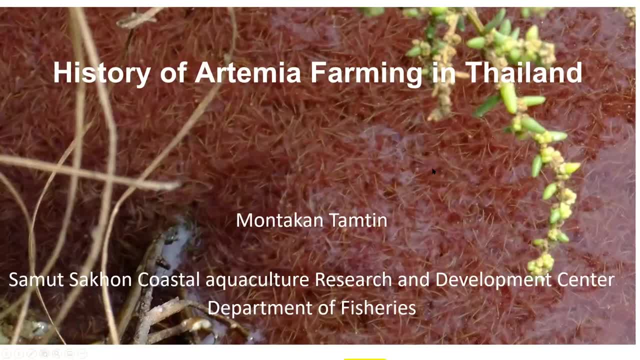 would like to share with you some of the most important things that you need to know in this presentation. Next, I would like to share with you some of the most important things that you need to know in this presentation. Next, I would like to 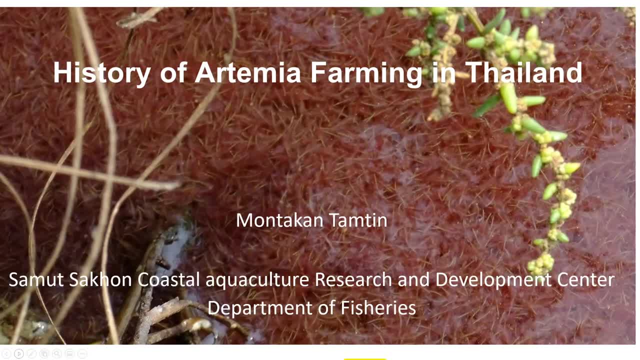 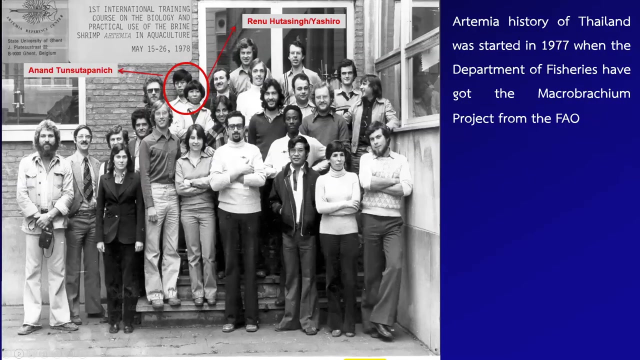 share with you some of the most important things that you need to know in this presentation. First, I would like to share with you some of the most important things that you need to know in this presentation. Next, I would like to share with you. 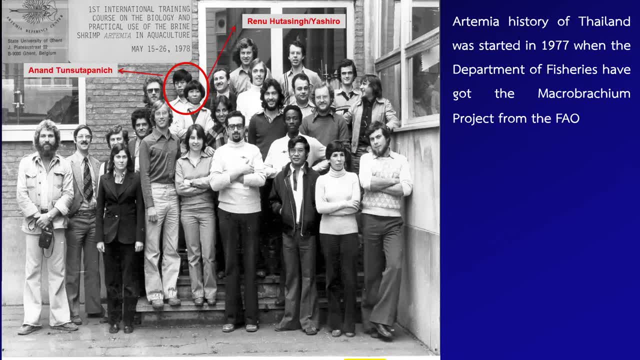 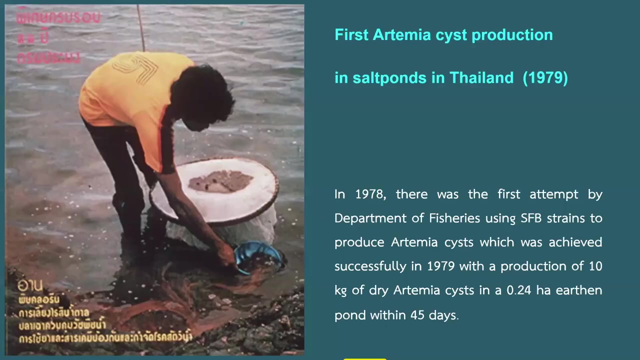 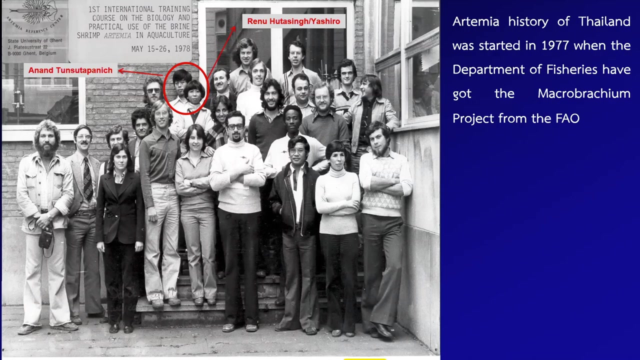 some of the most important things that you need to know in this presentation. Next, I would like to share with you some of the most important things that you need to know in this presentation. First, I would like to share with you some of the 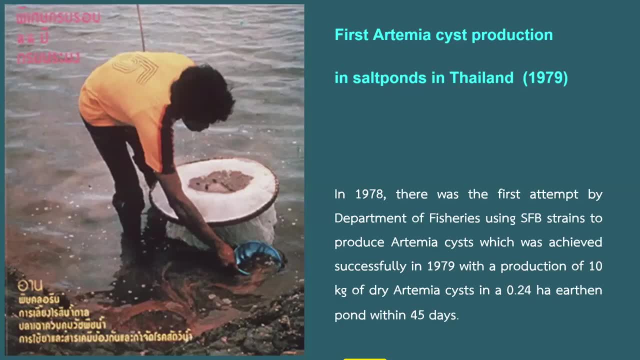 most important things that you need to know in this presentation. Next, I would like to share with you some of the most important things that you need to know in this presentation. Next, I would like to share with you some of the most important things. 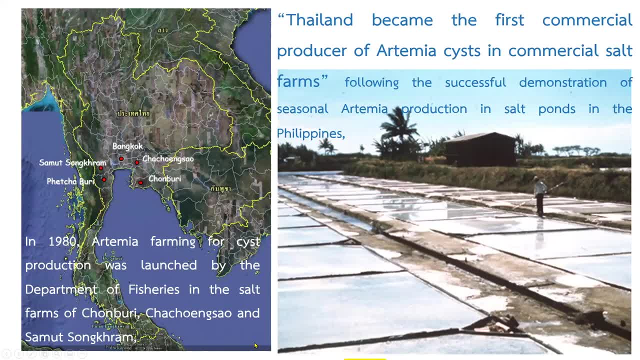 that you need to know in this presentation. First, I would like to share with you some of the most important things that you need to know in this presentation. Next, I would like to share with you some of the most important things that you need. 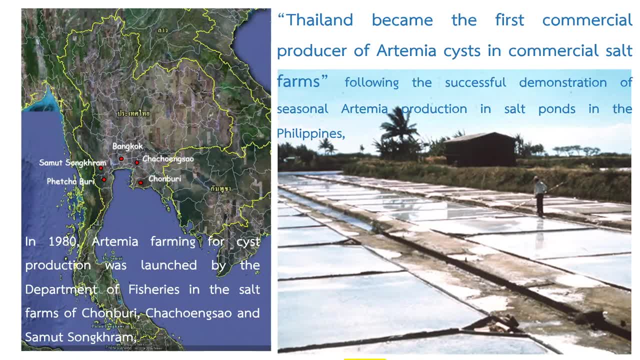 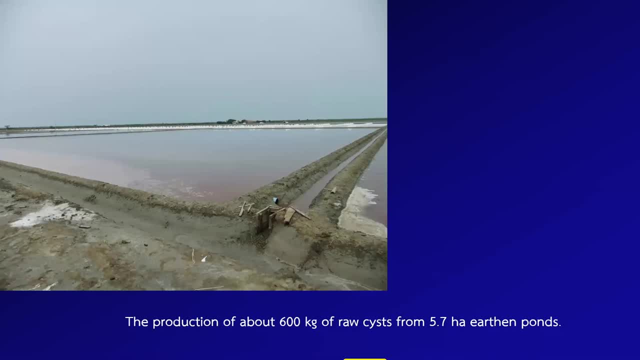 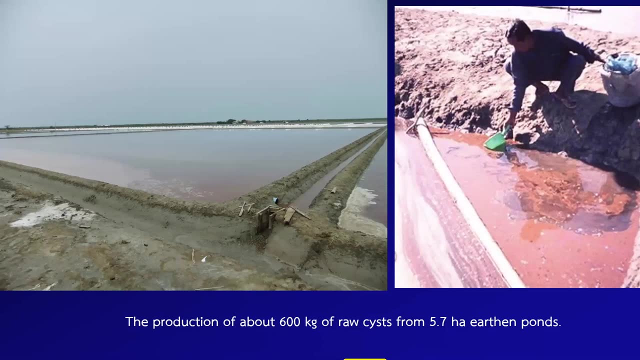 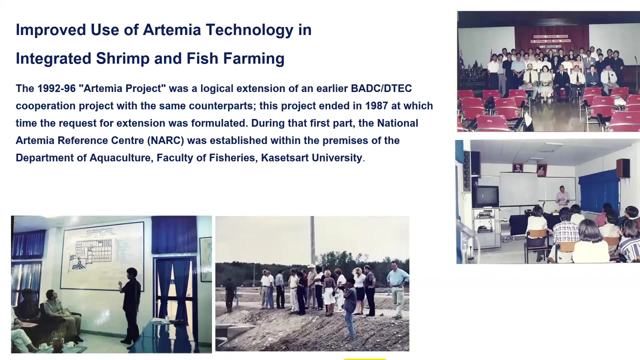 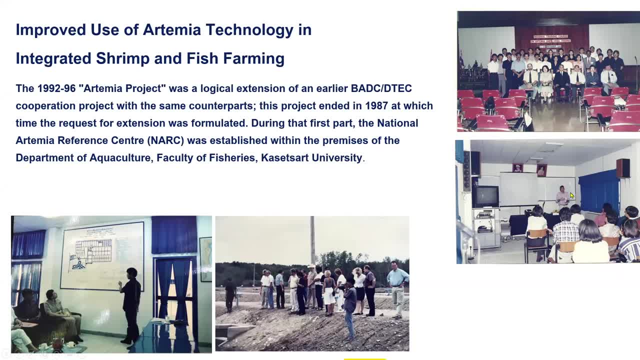 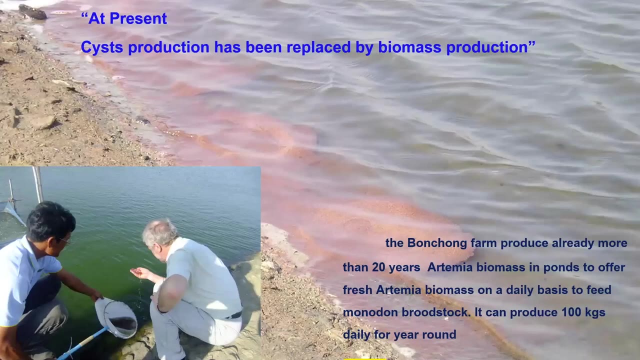 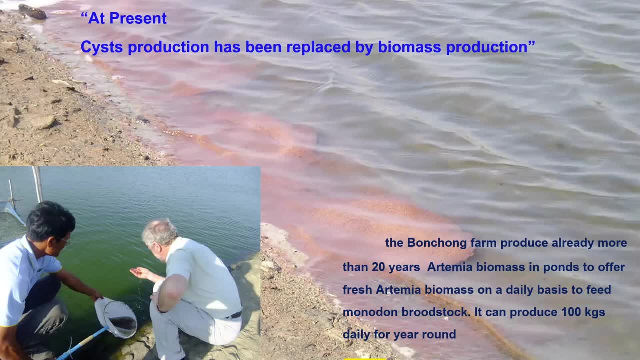 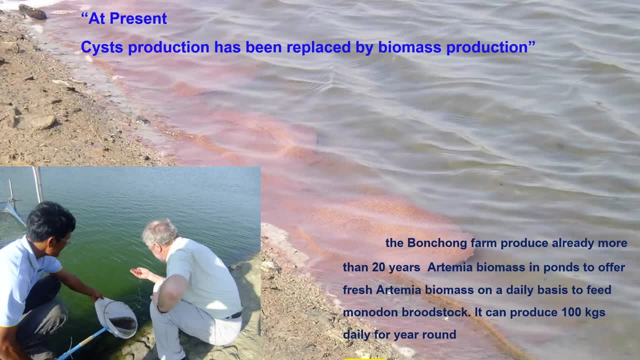 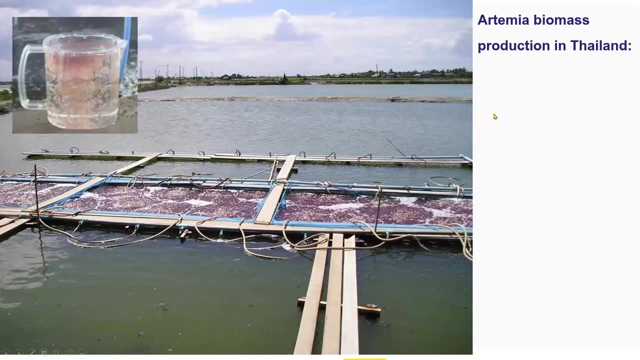 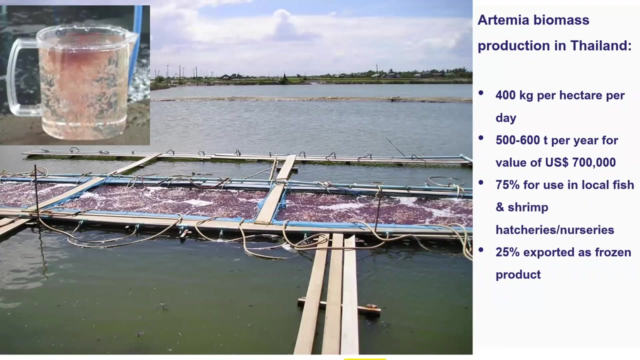 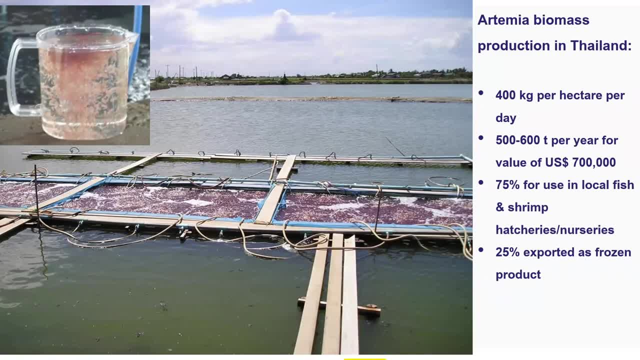 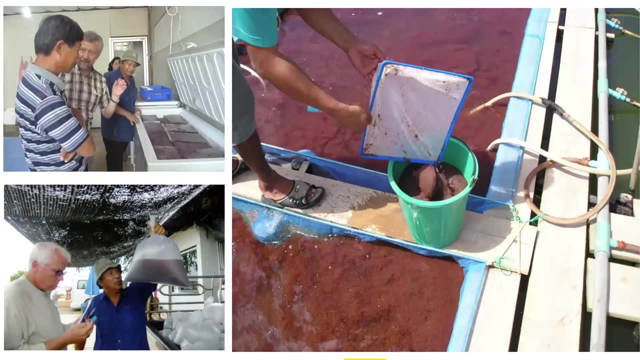 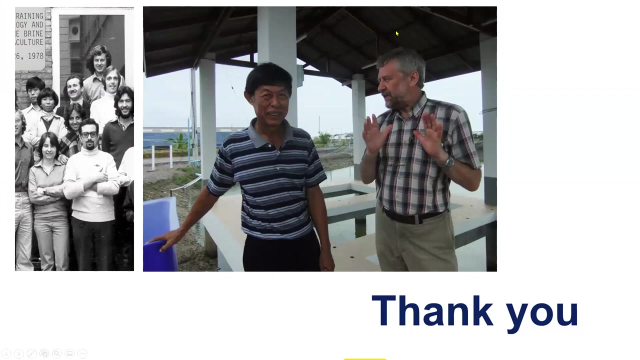 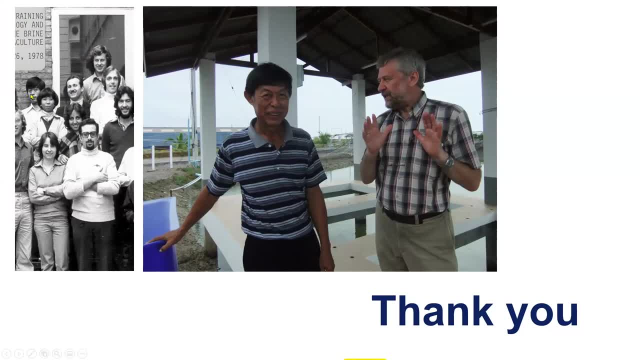 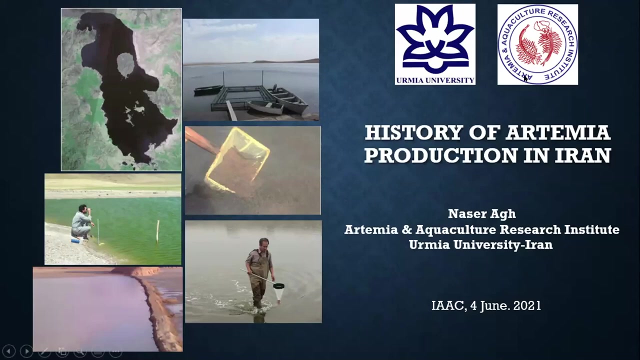 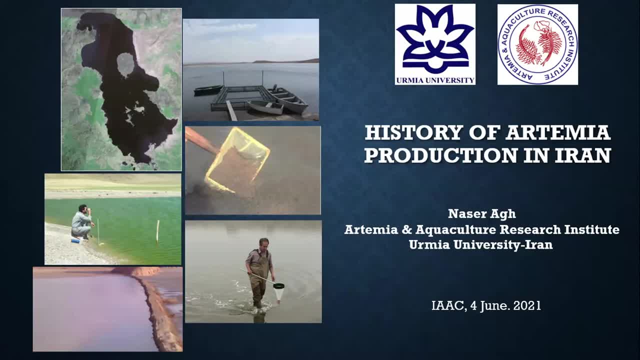 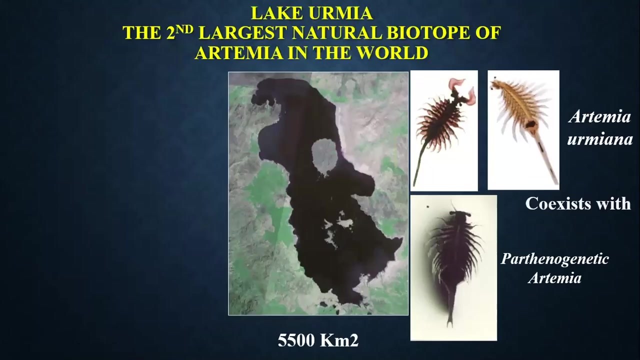 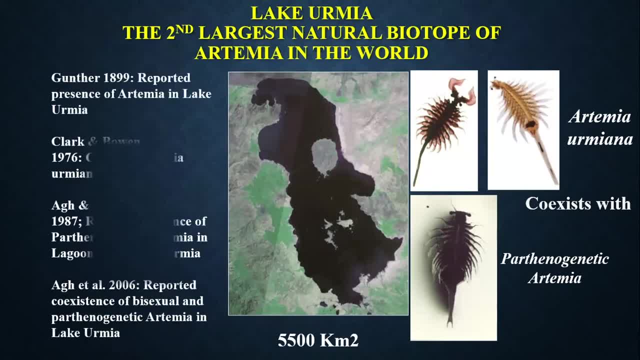 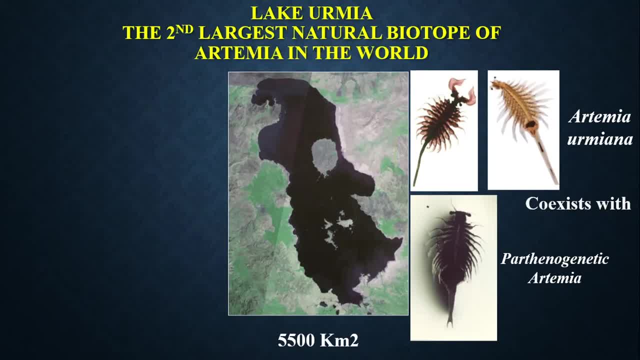 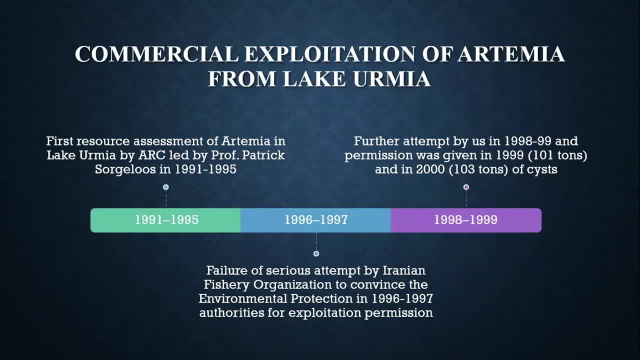 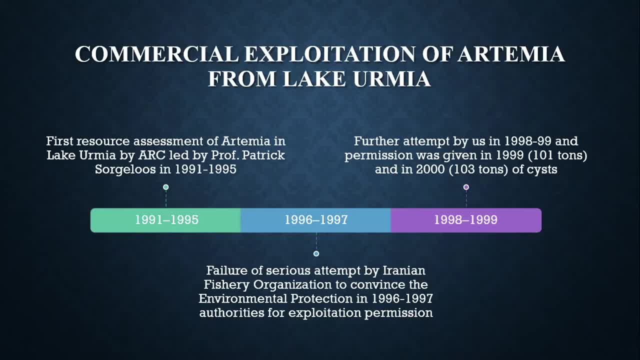 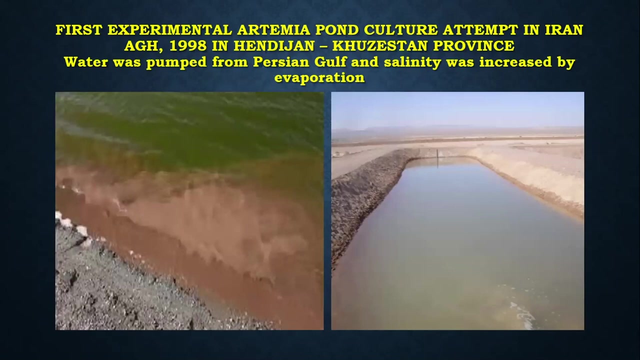 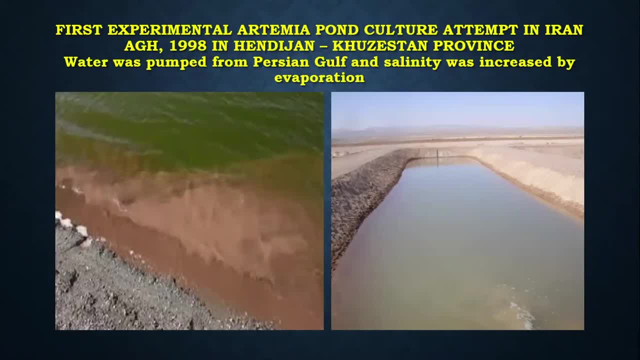 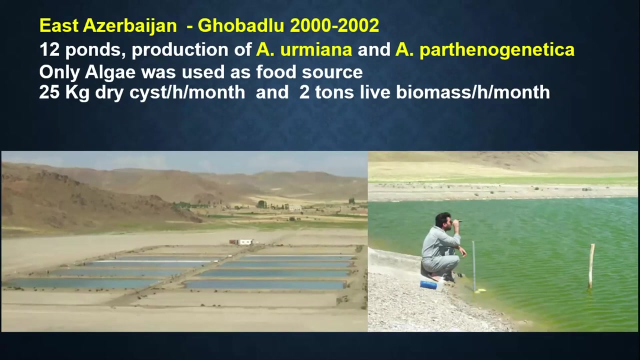 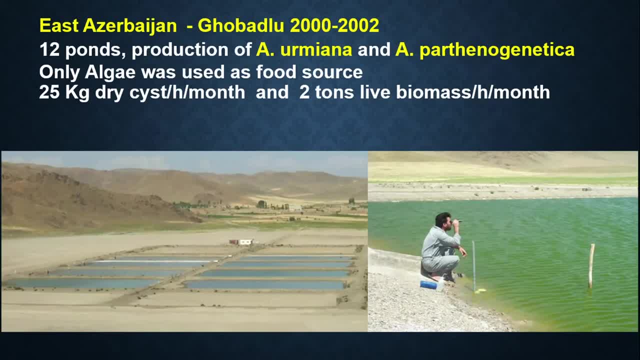 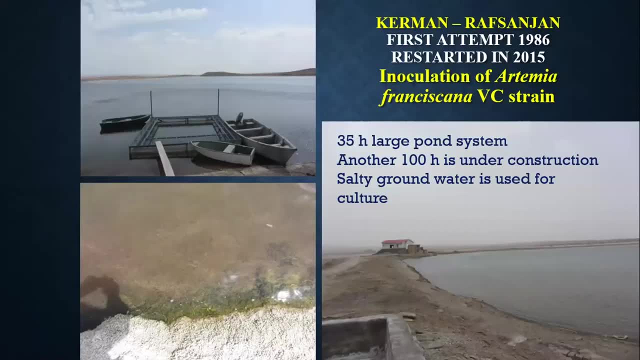 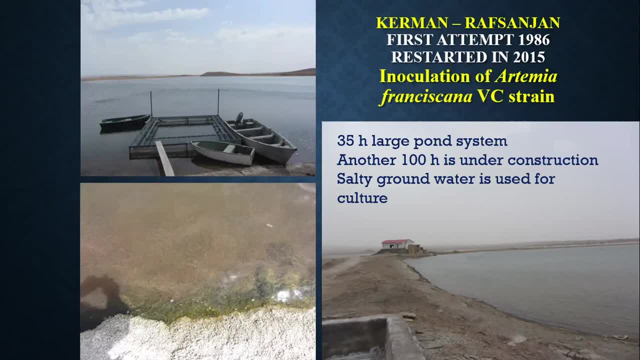 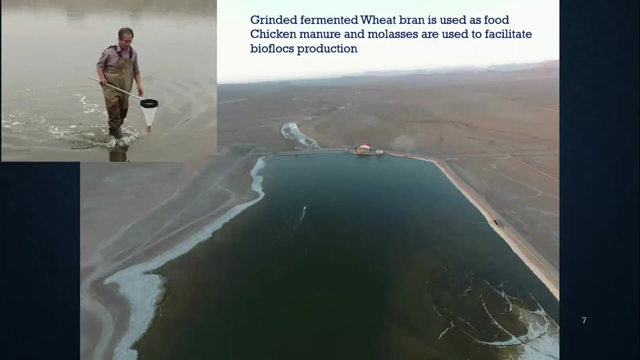 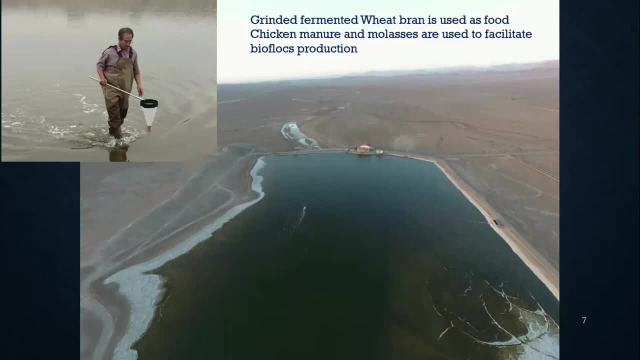 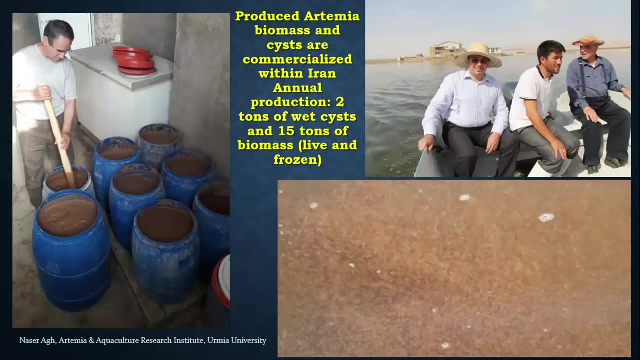 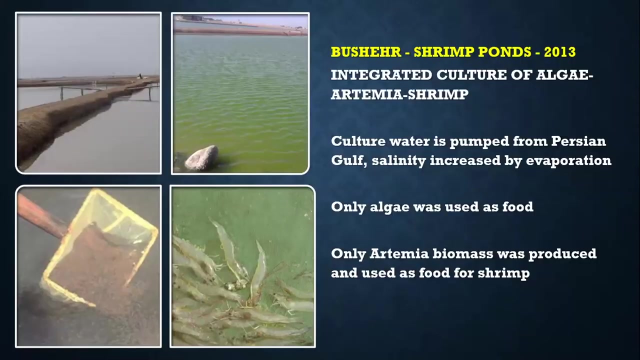 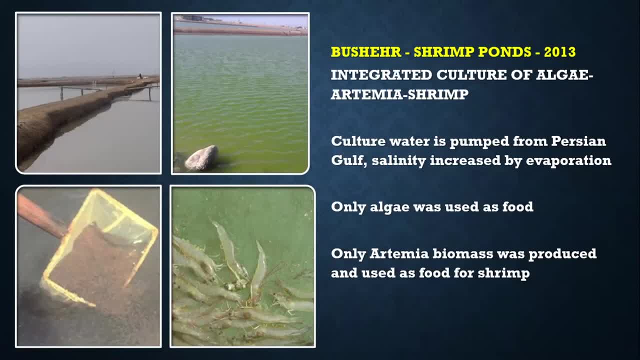 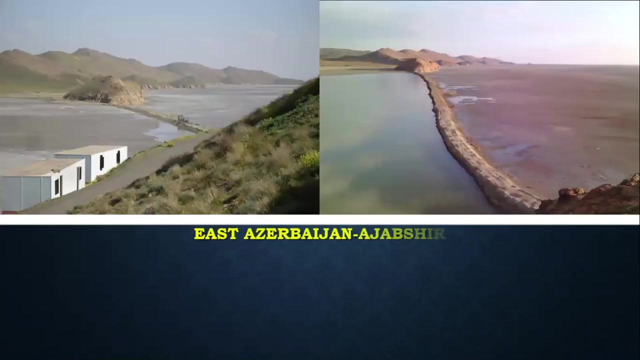 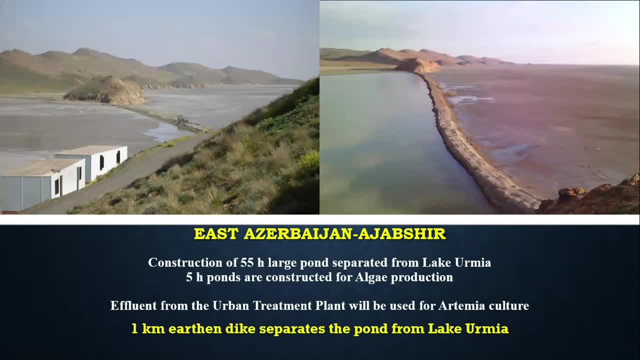 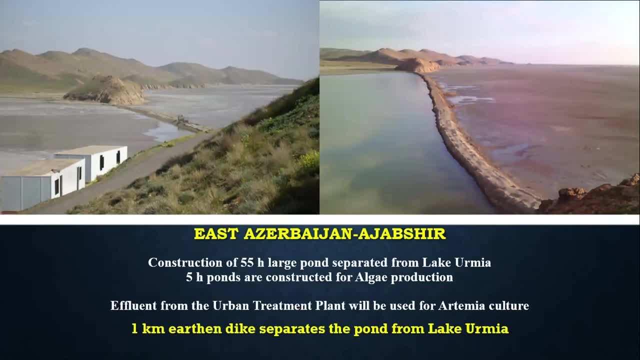 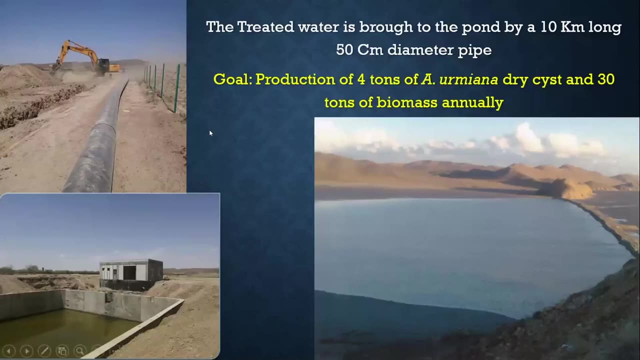 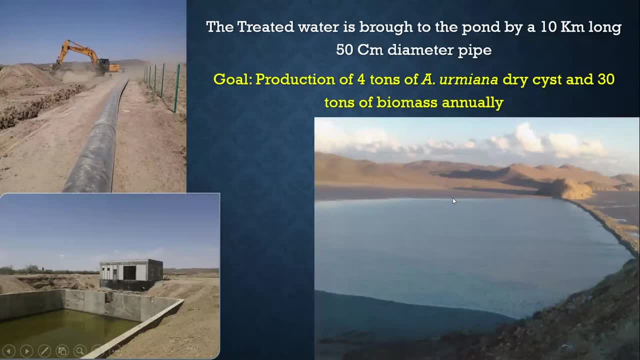 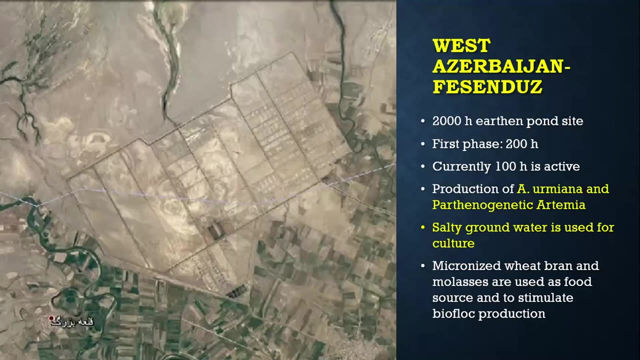 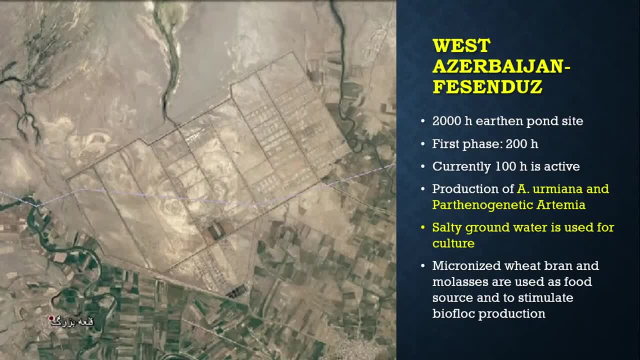 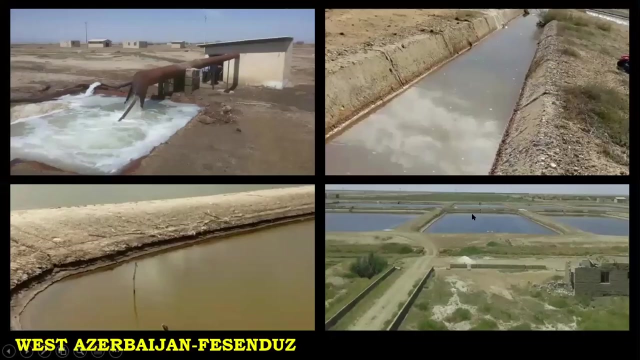 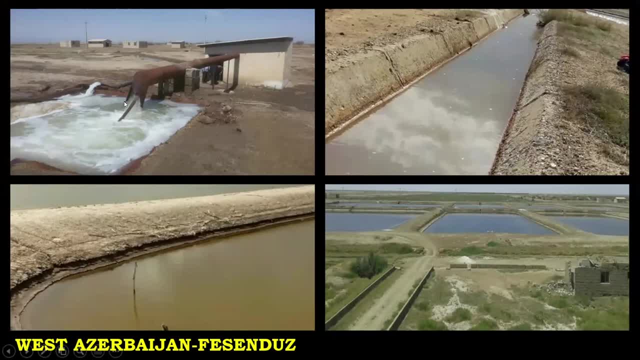 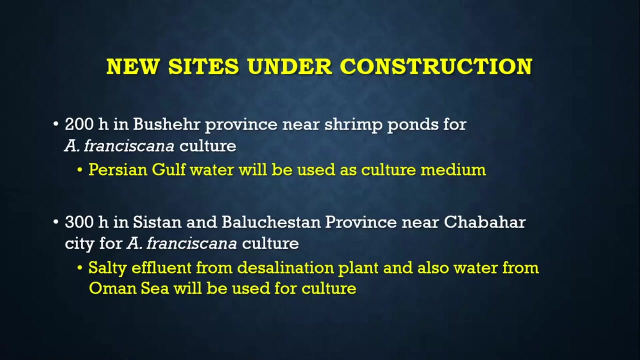 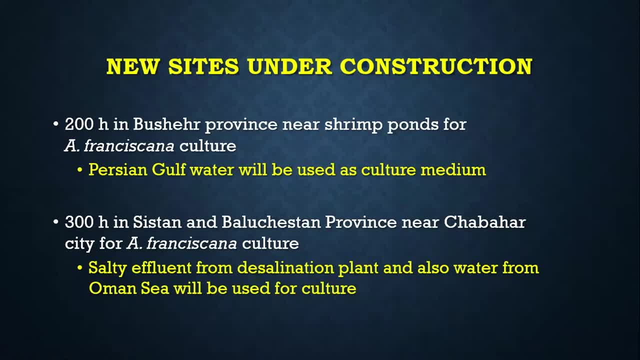 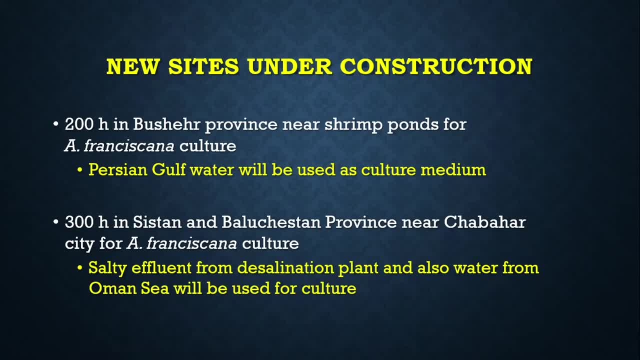 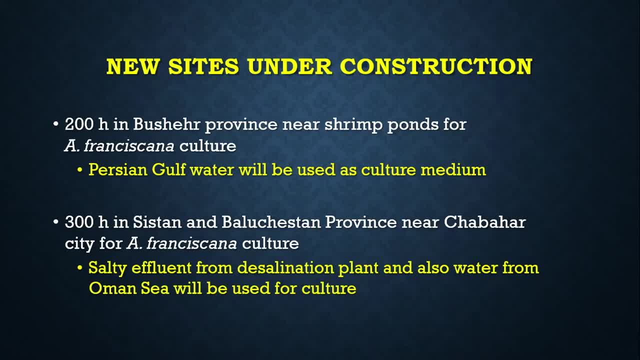 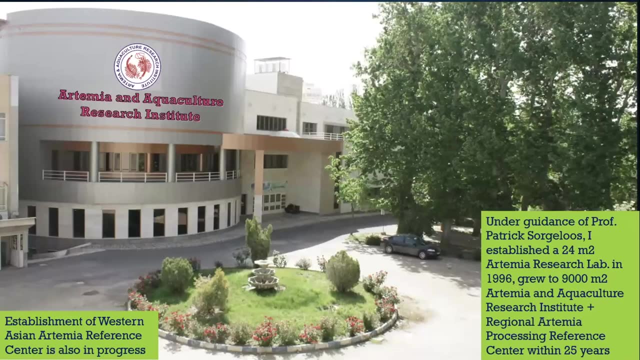 most important things that you need to know in this presentation. Next, I would like to share with you some of the most important things that you need to know. Next, I would like to share with you some of the most important things that you need. 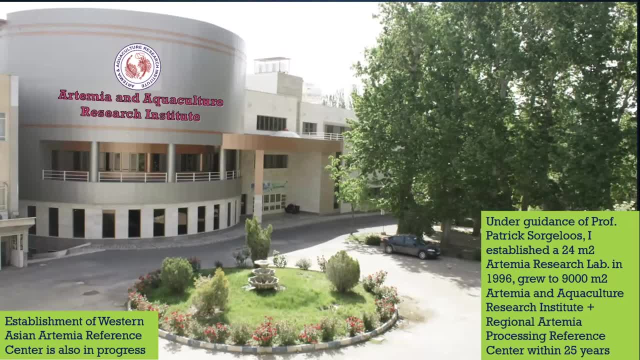 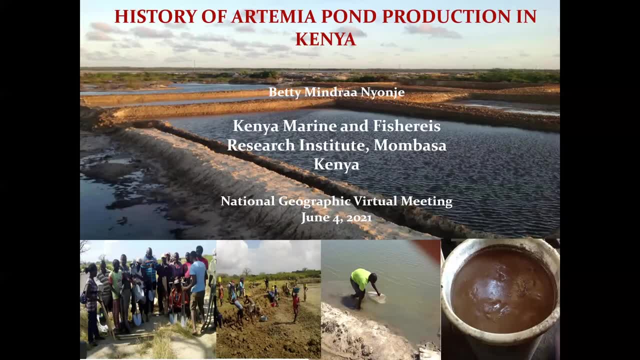 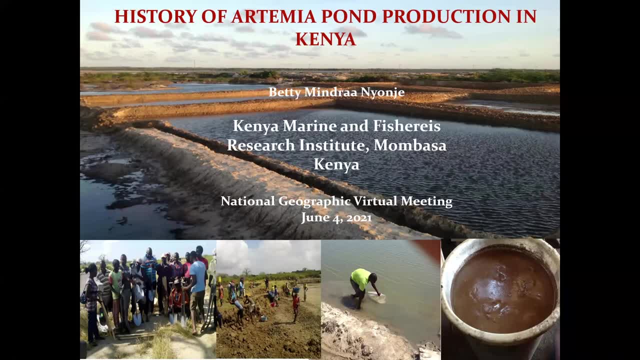 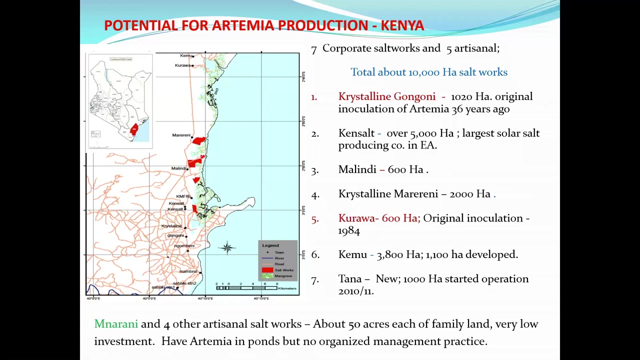 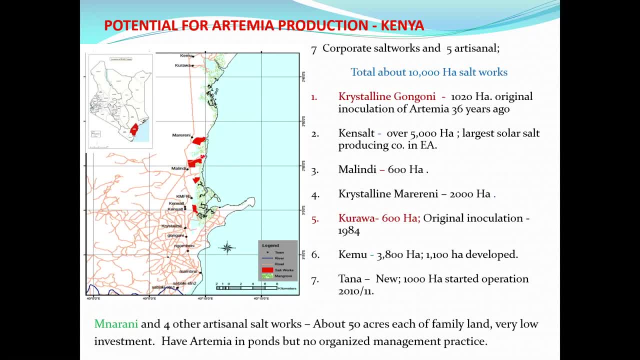 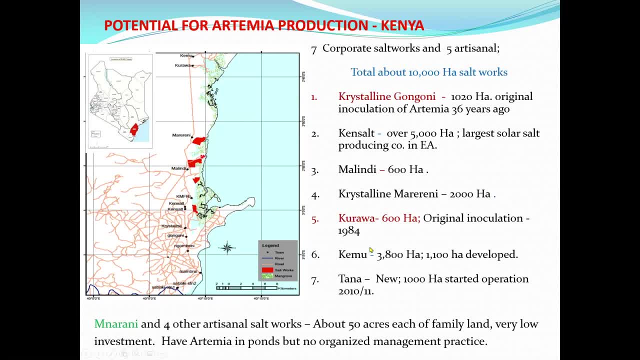 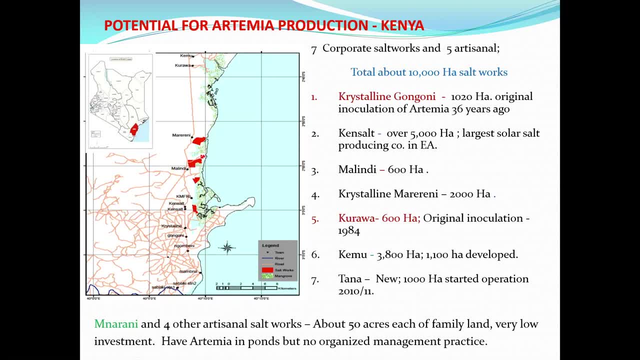 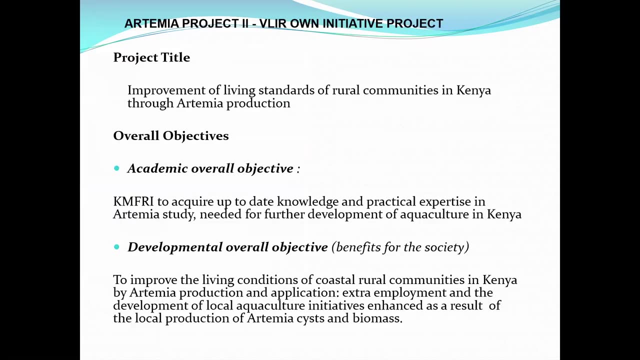 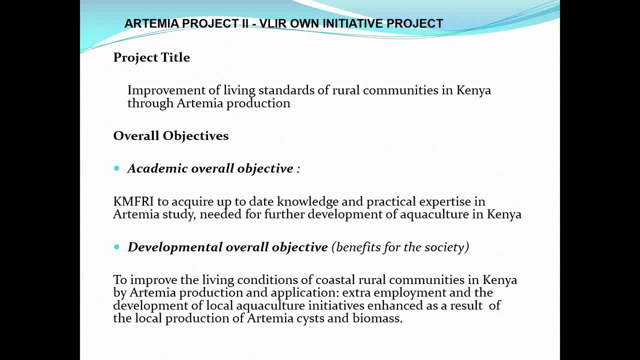 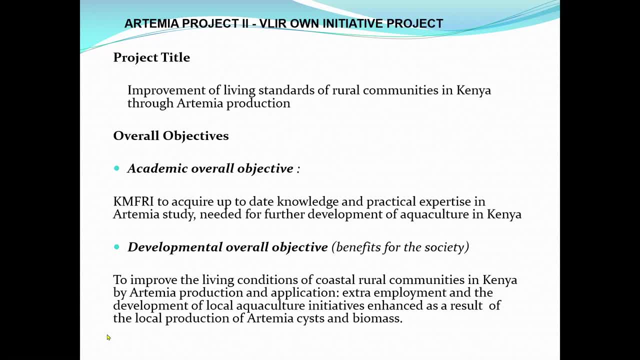 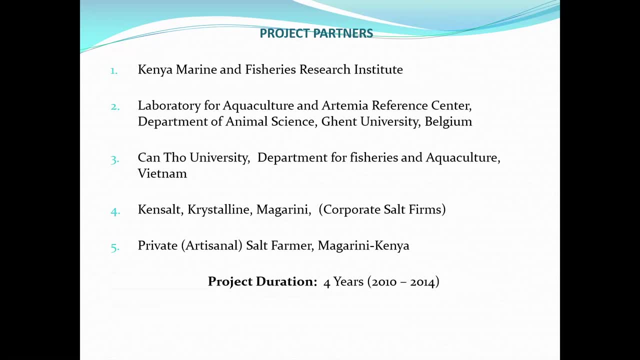 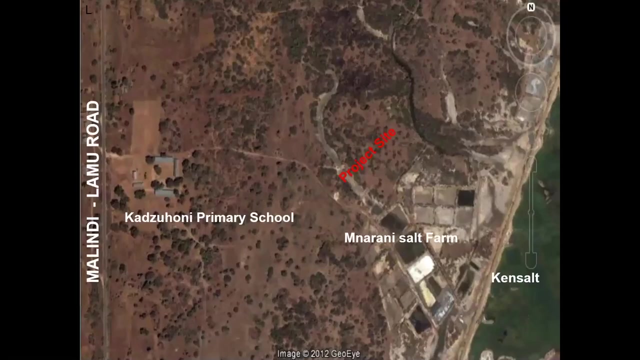 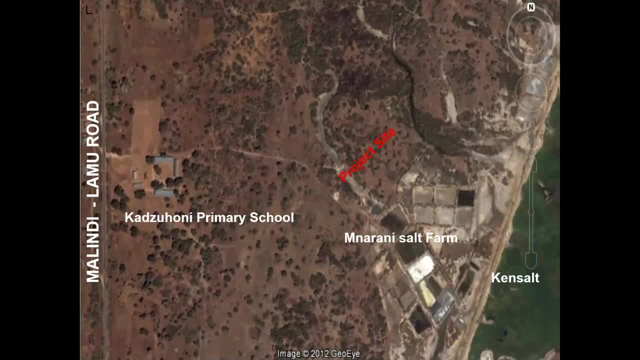 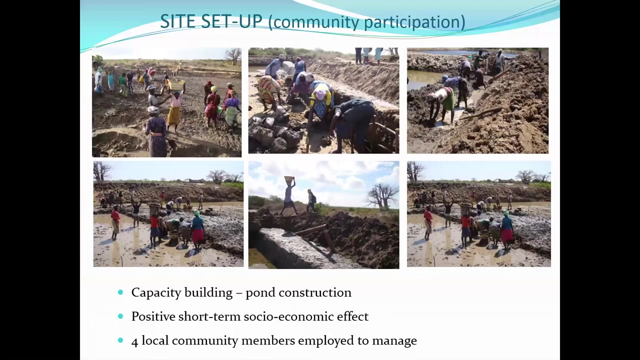 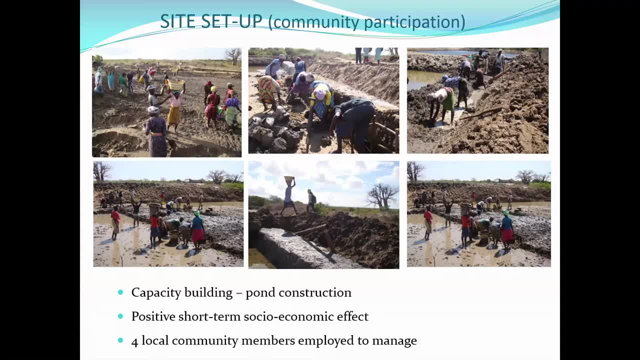 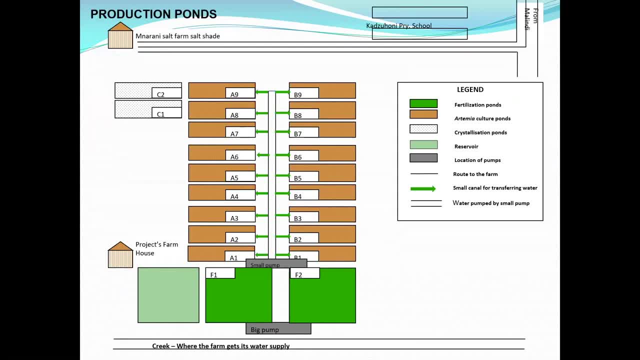 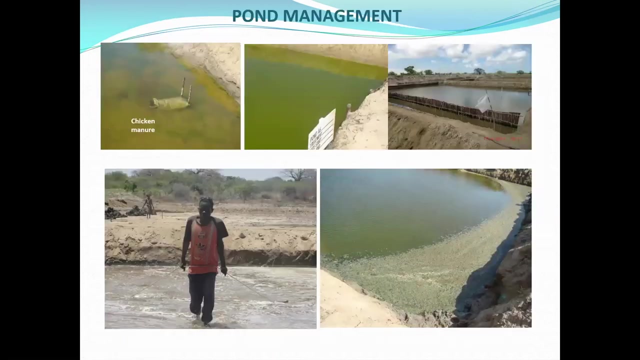 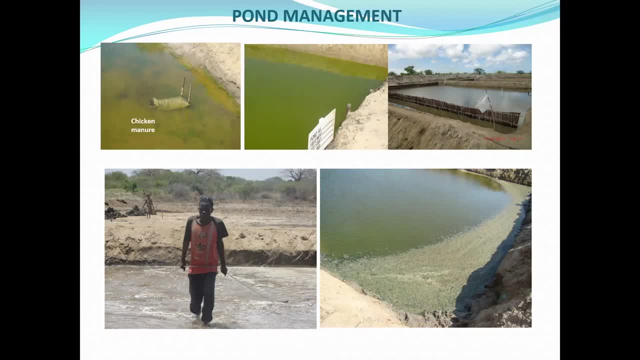 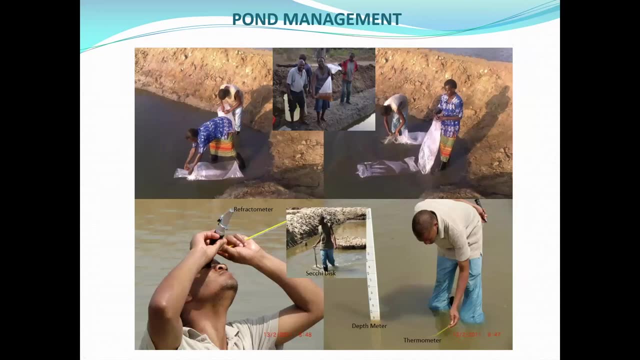 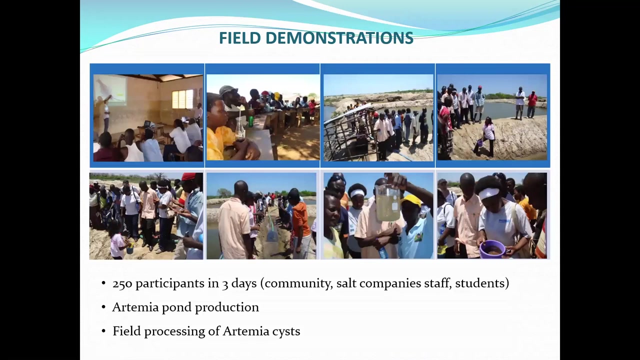 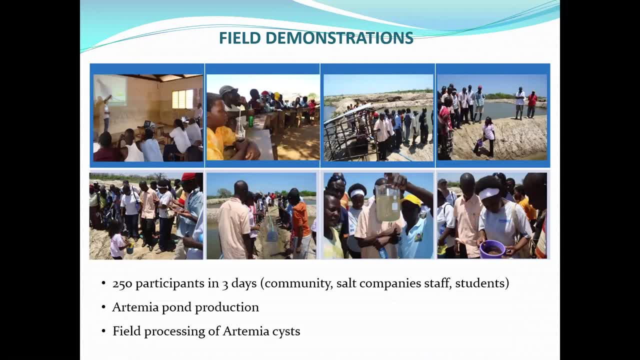 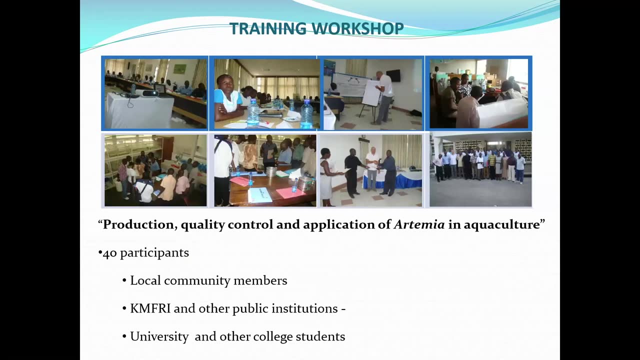 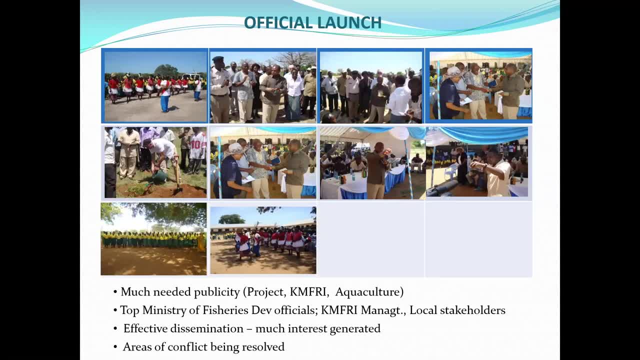 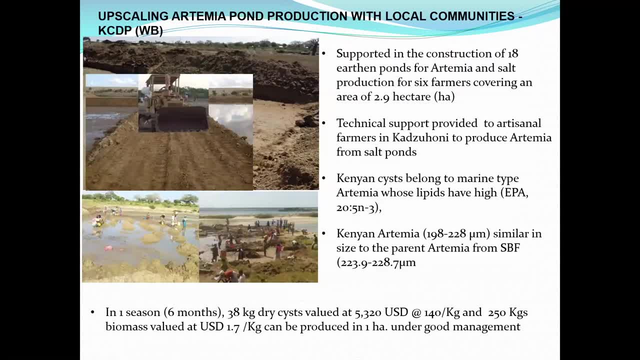 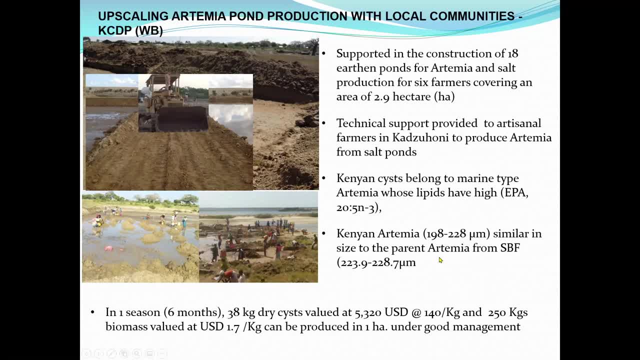 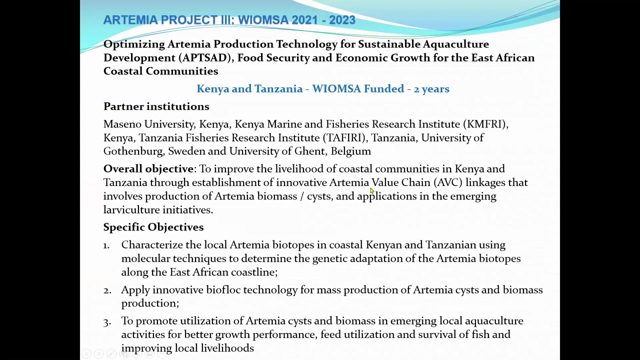 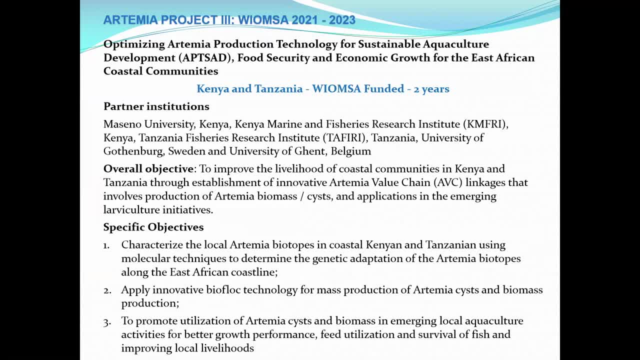 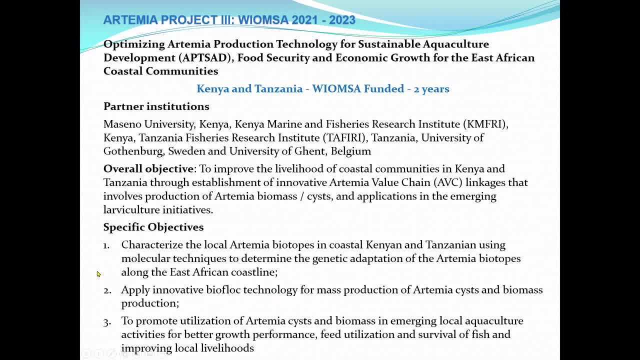 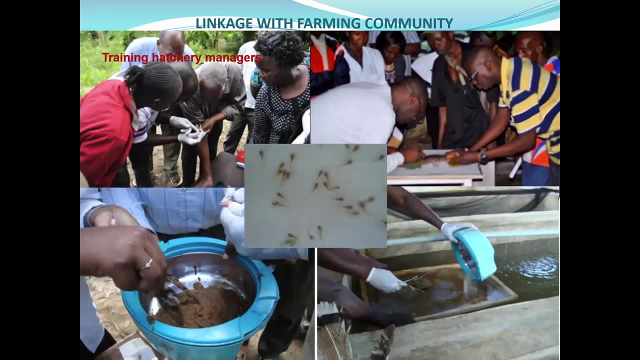 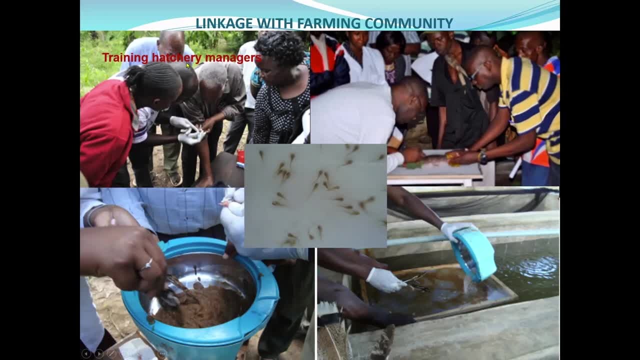 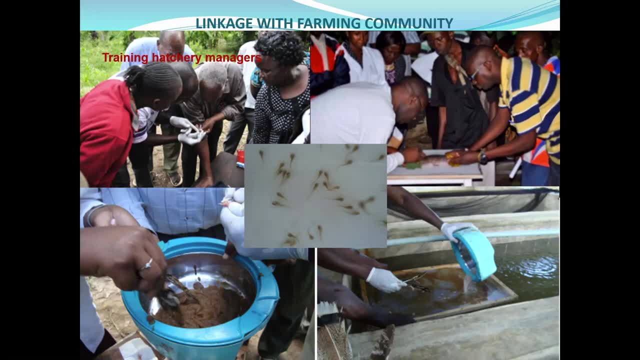 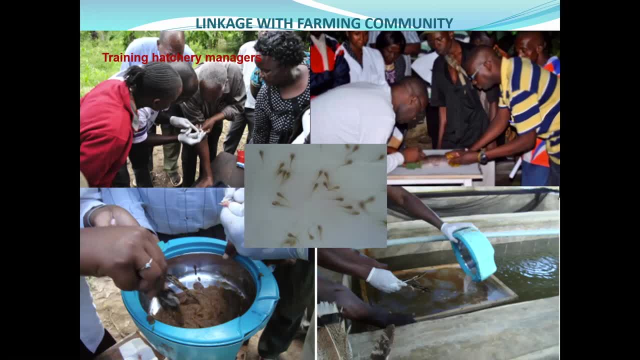 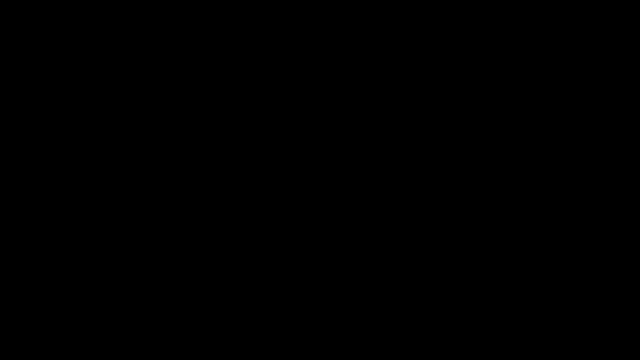 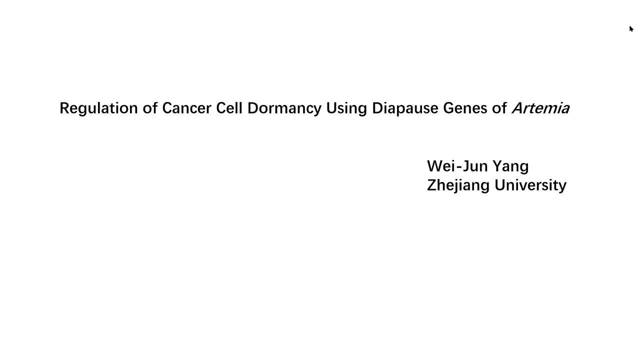 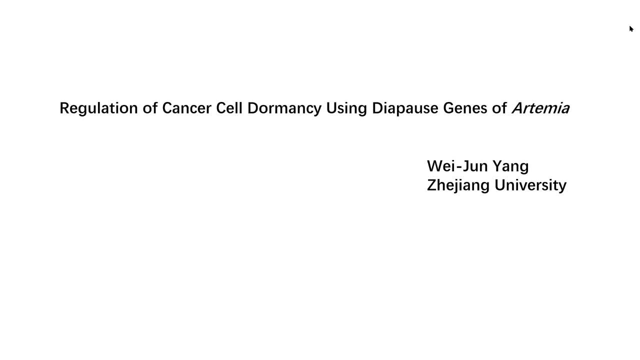 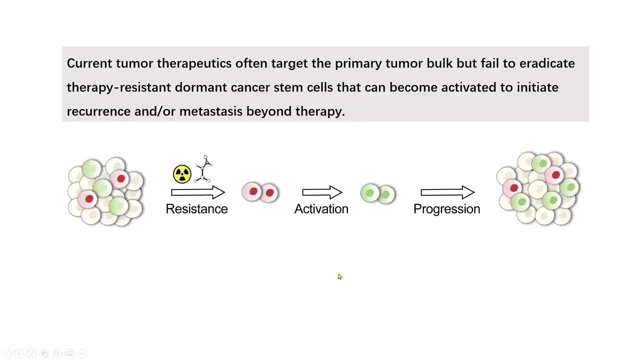 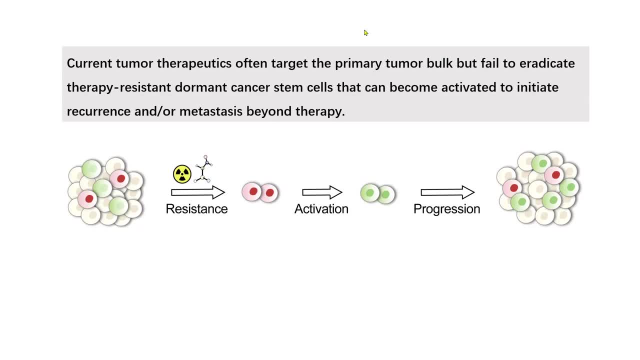 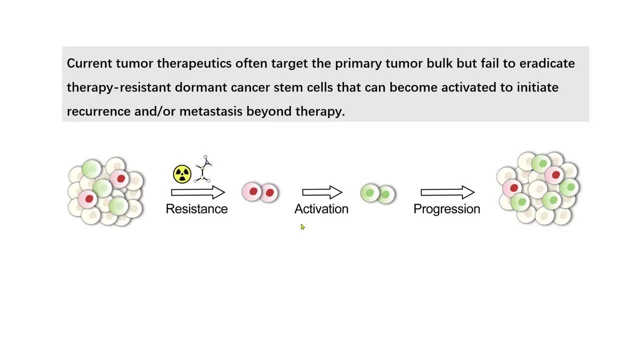 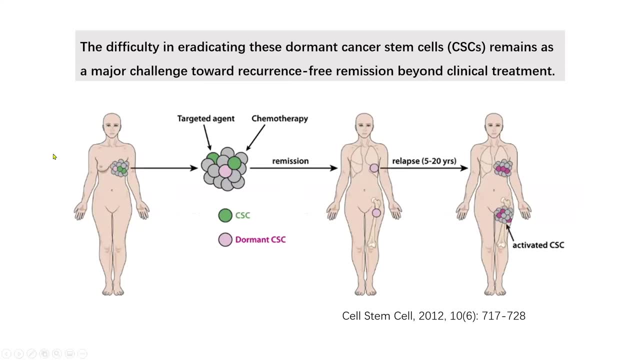 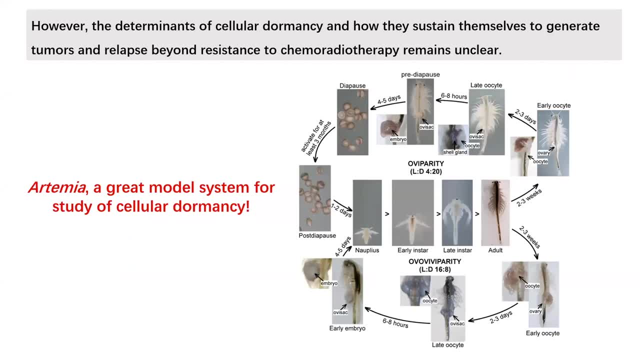 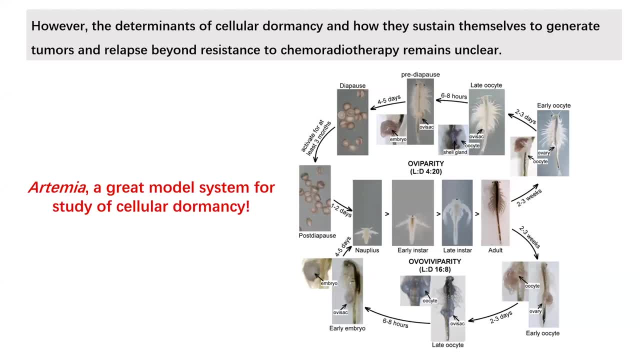 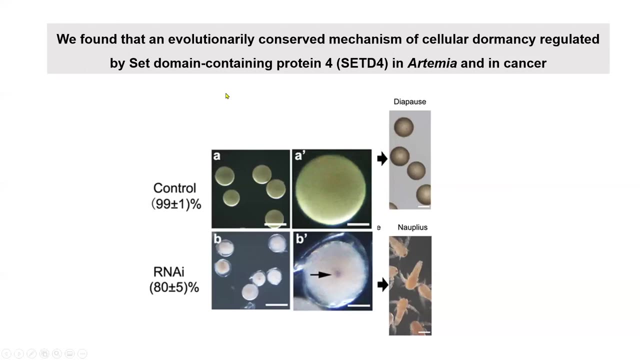 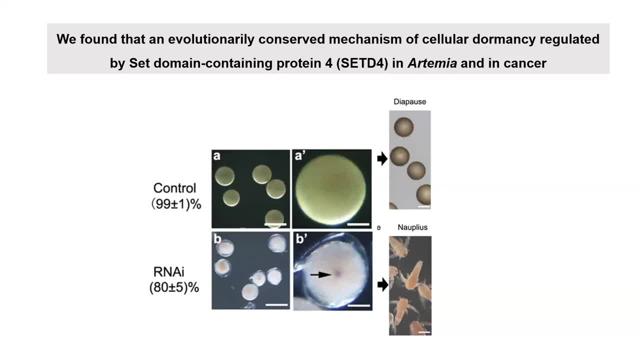 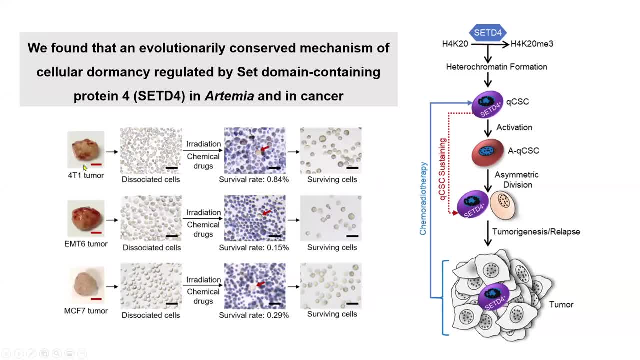 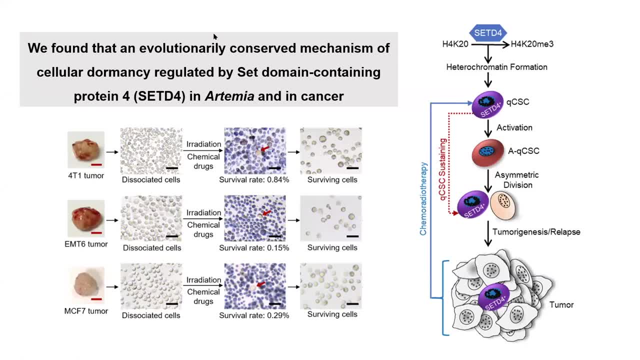 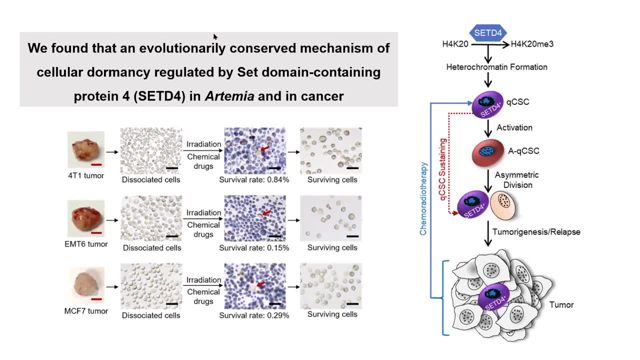 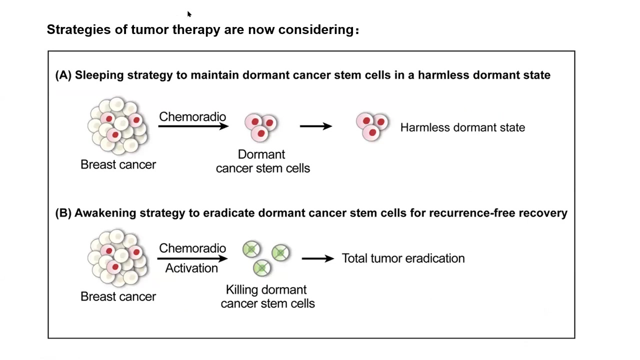 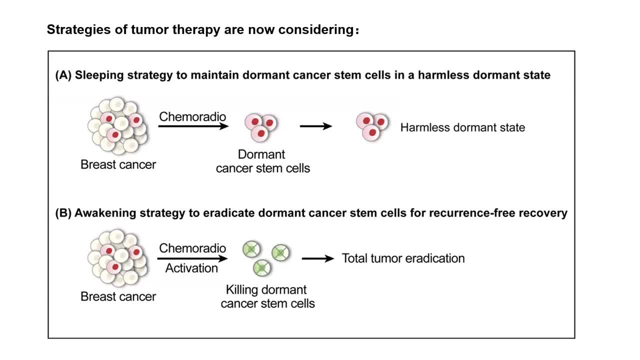 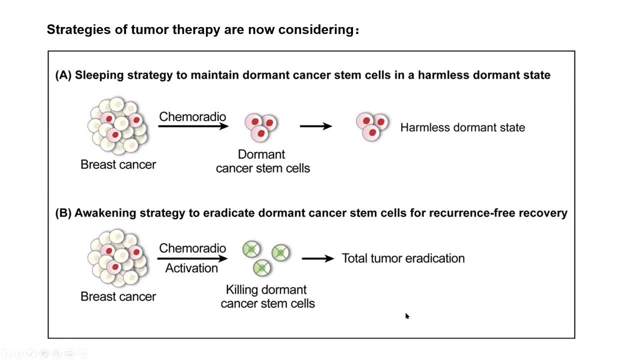 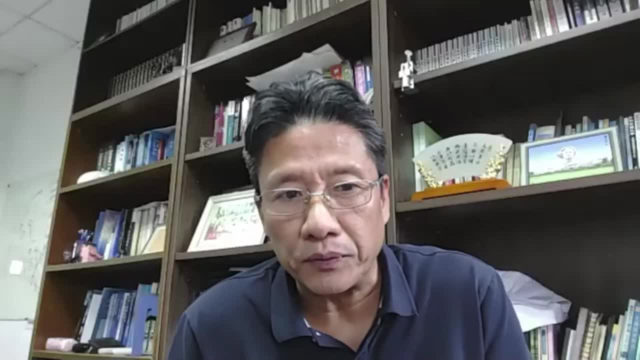 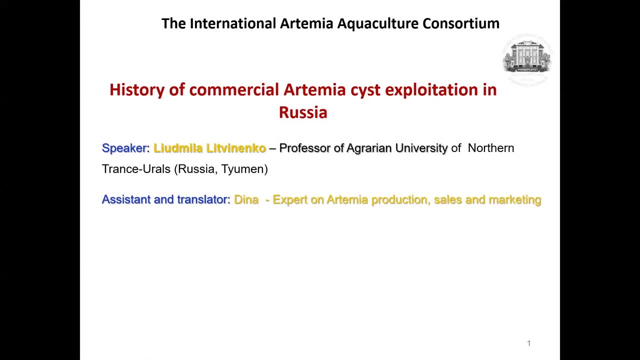 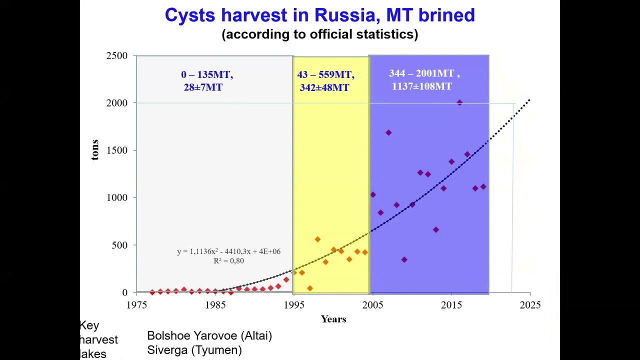 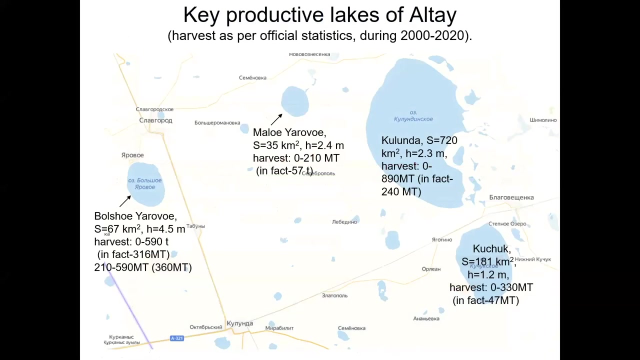 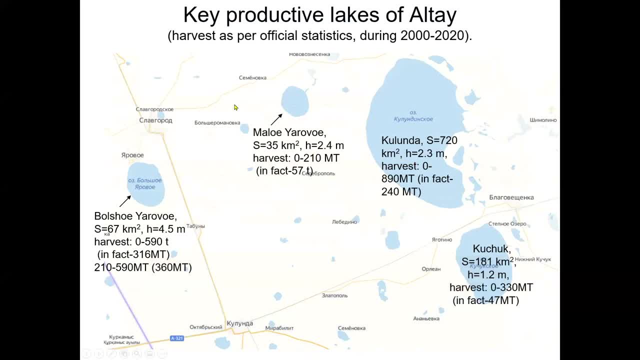 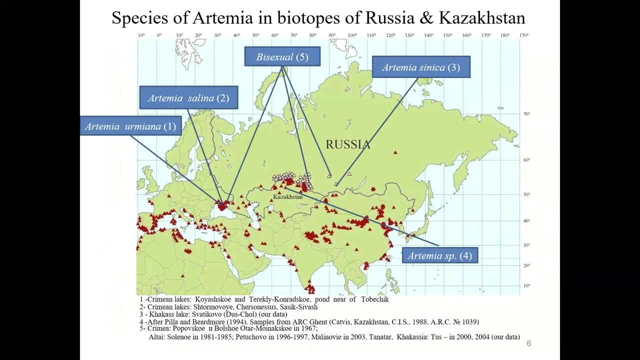 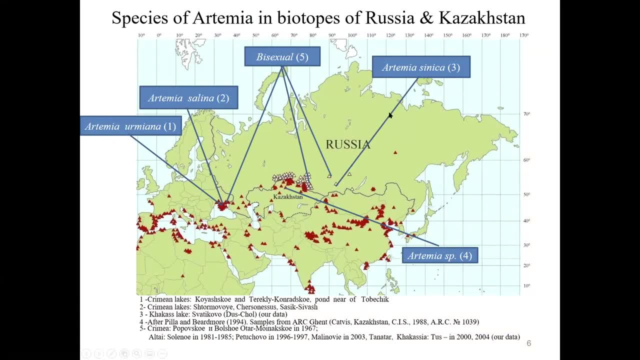 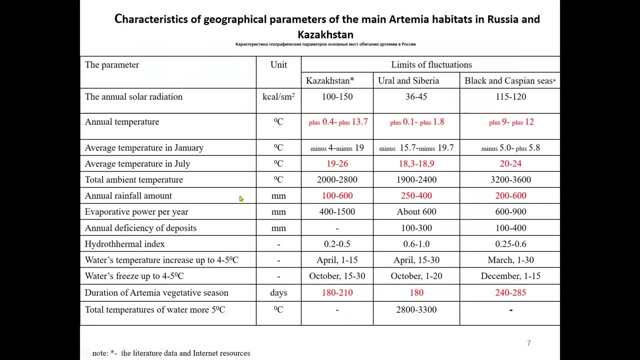 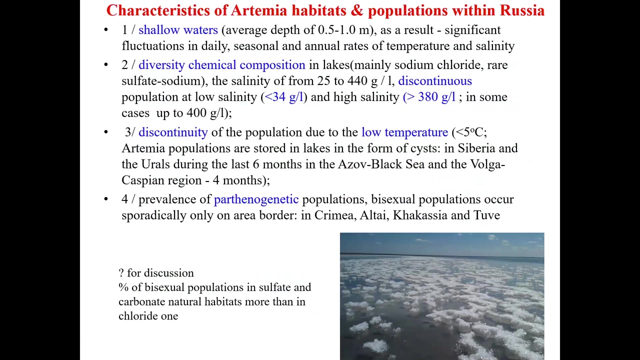 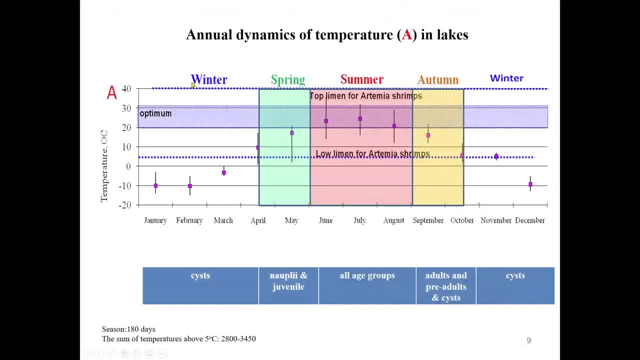 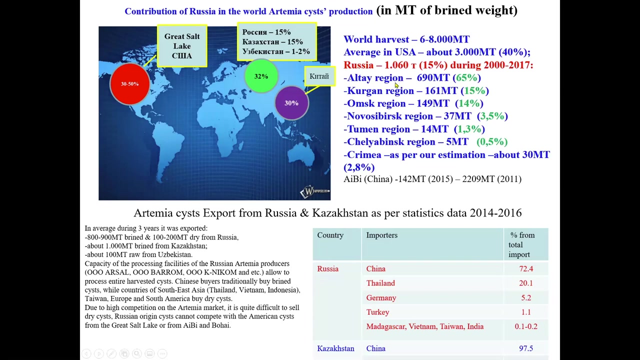 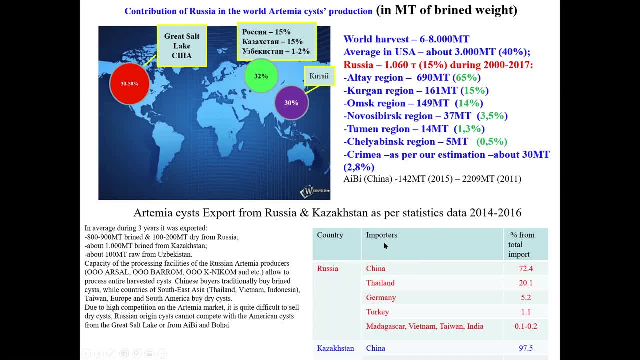 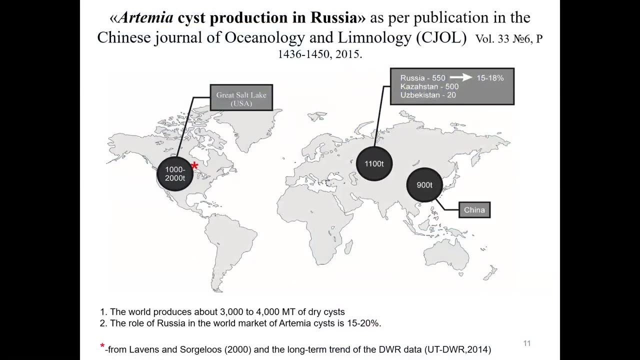 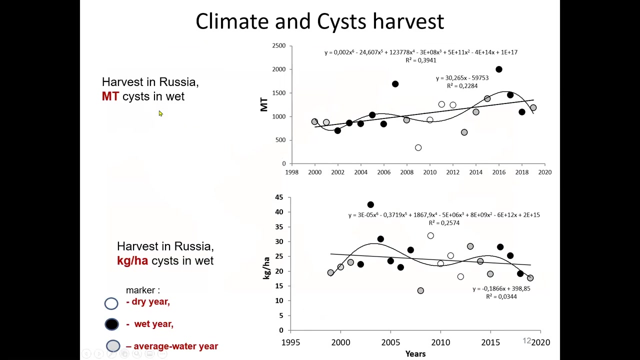 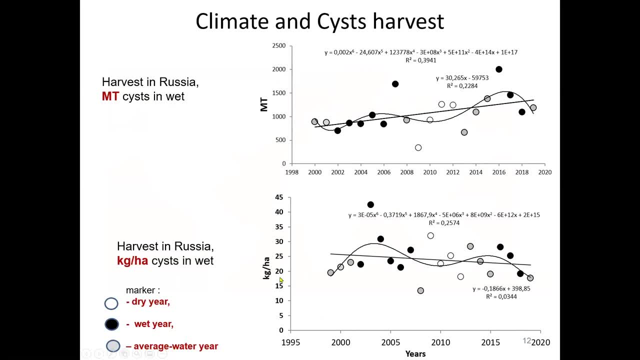 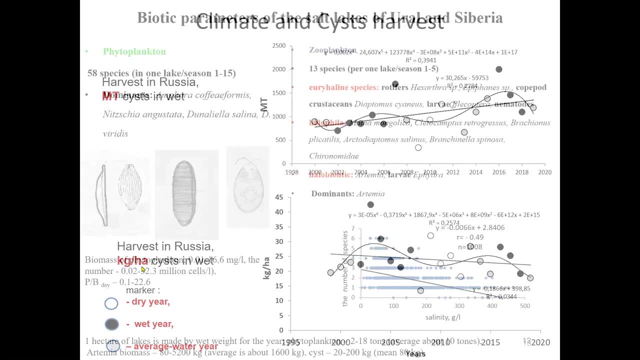 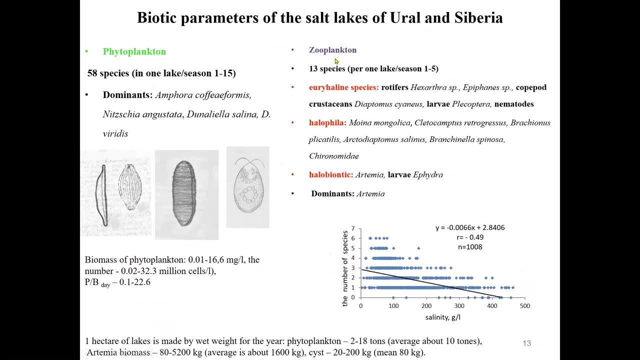 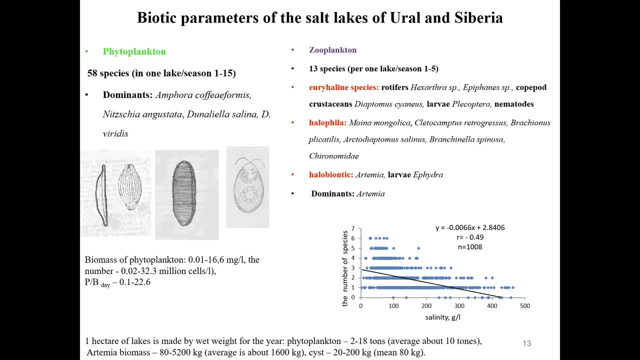 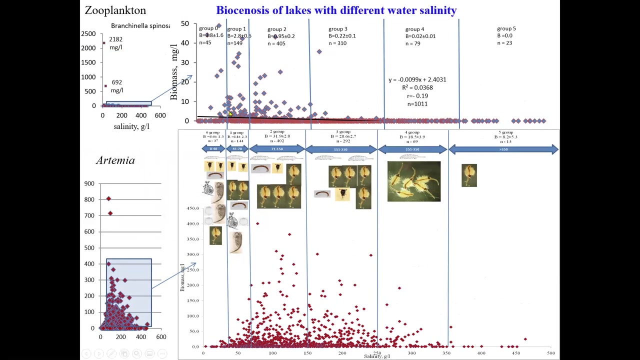 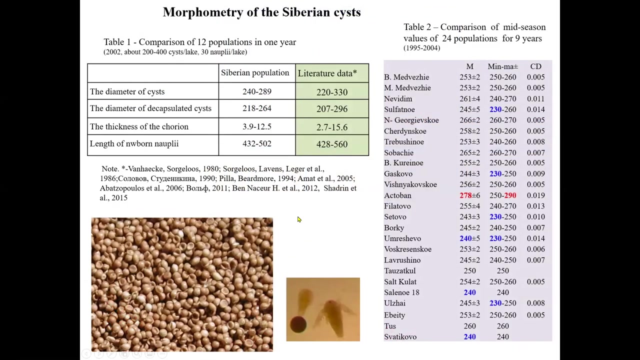 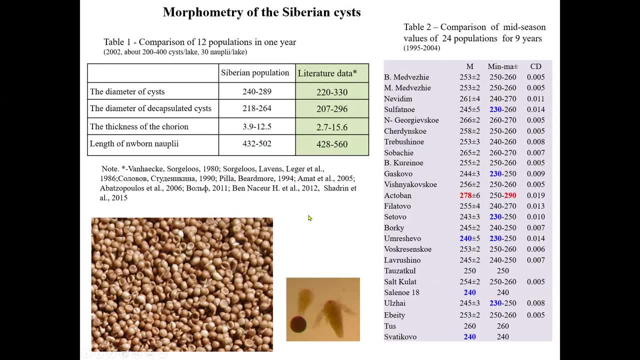 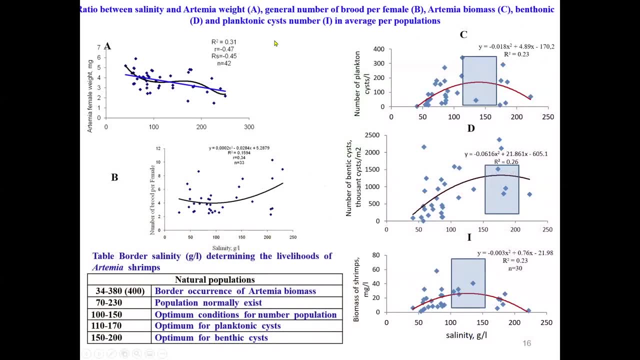 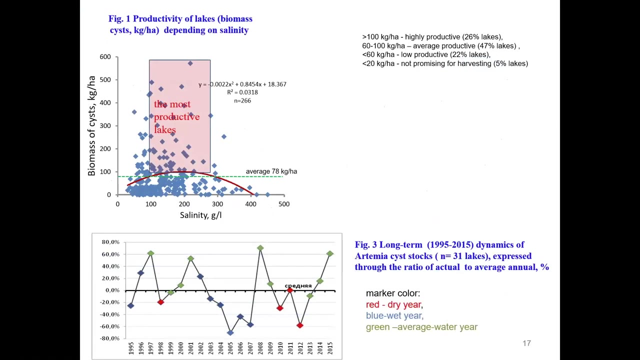 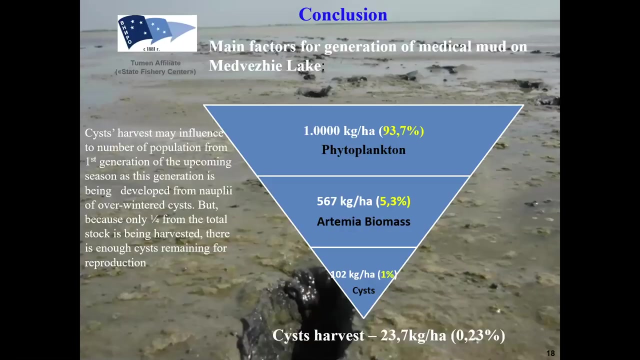 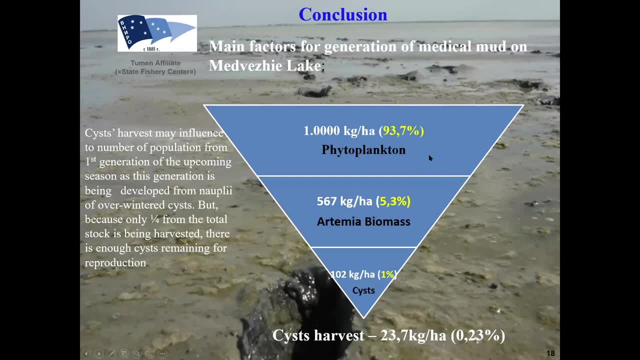 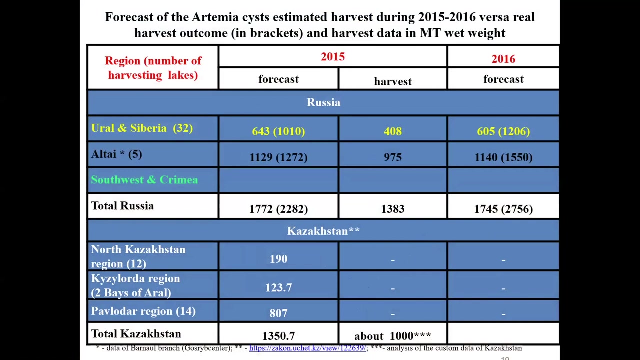 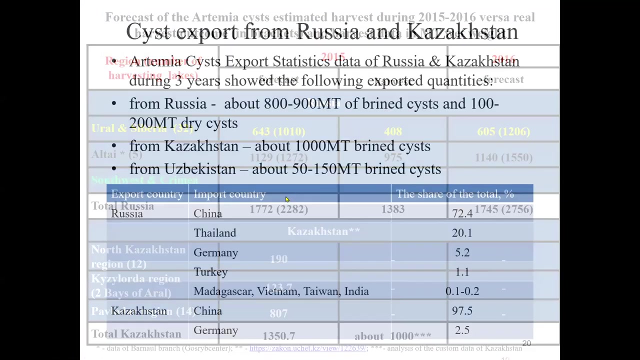 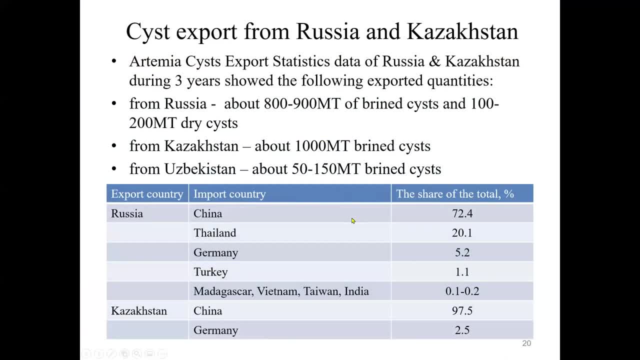 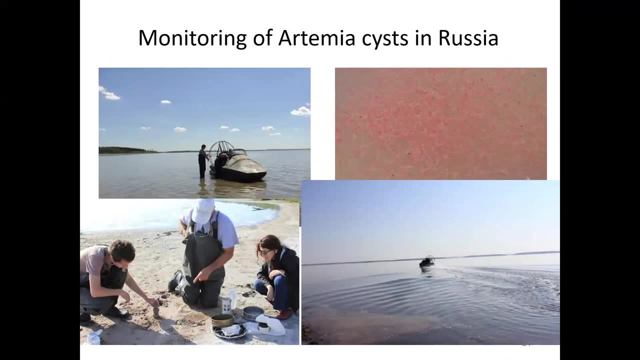 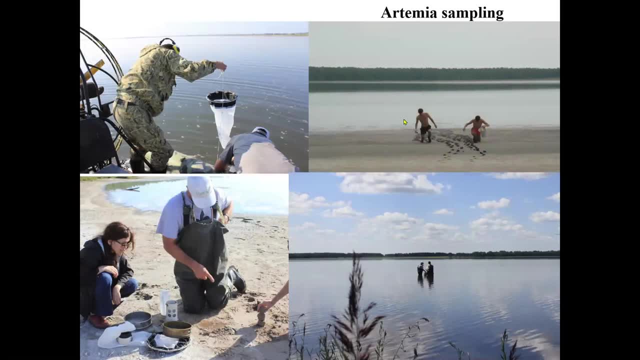 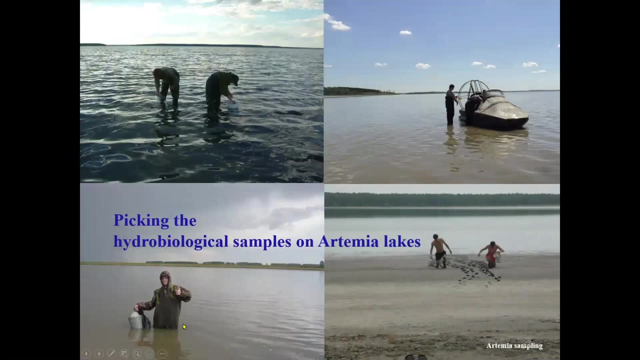 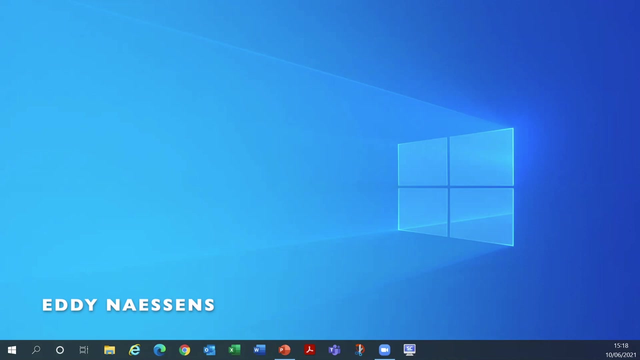 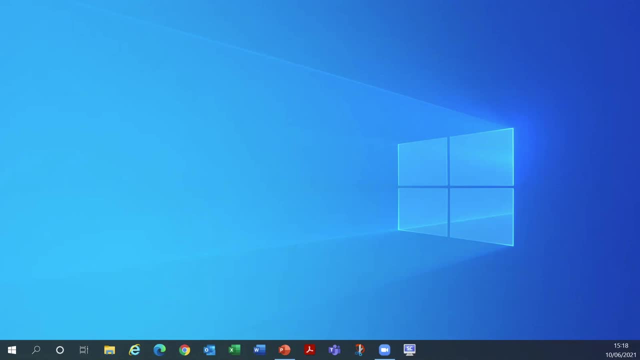 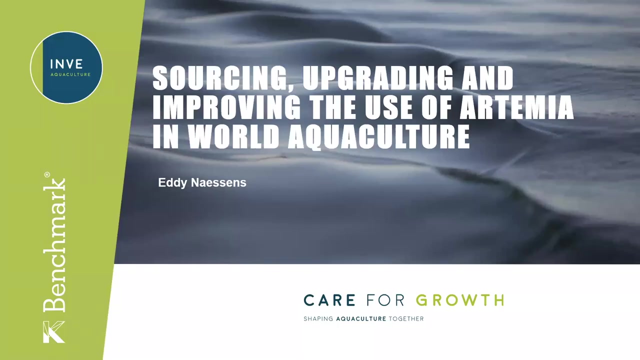 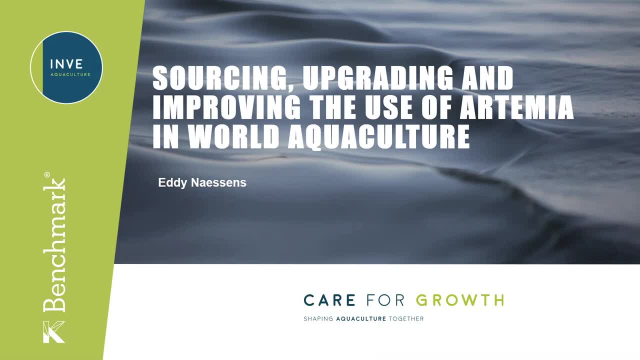 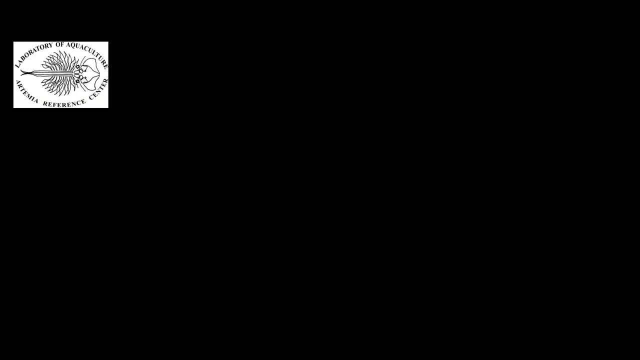 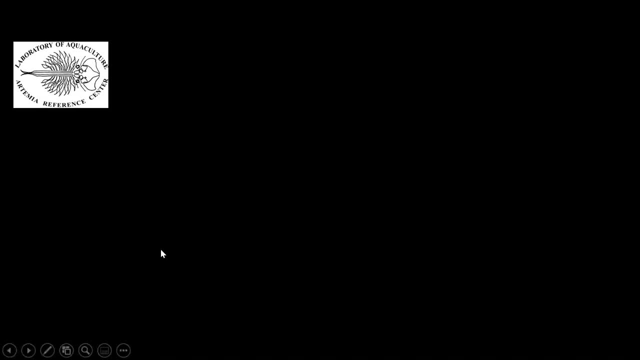 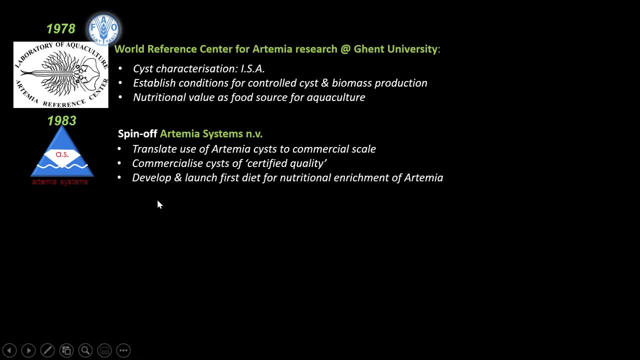 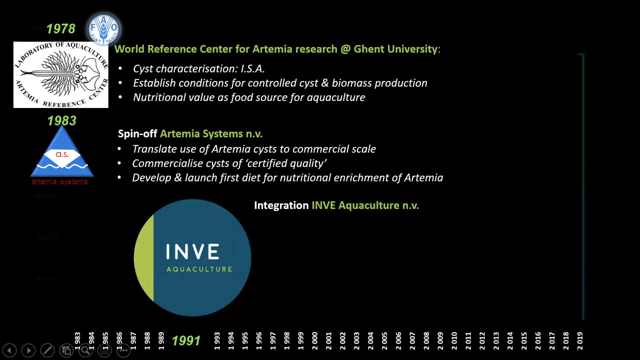 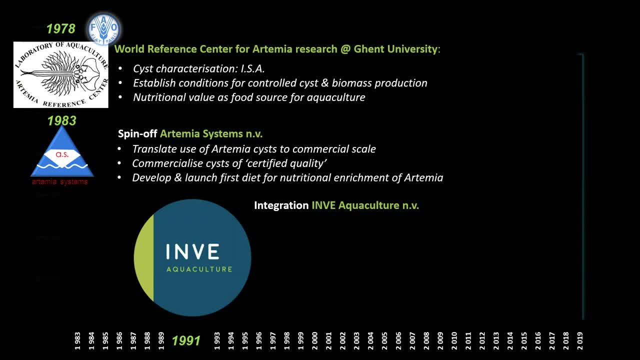 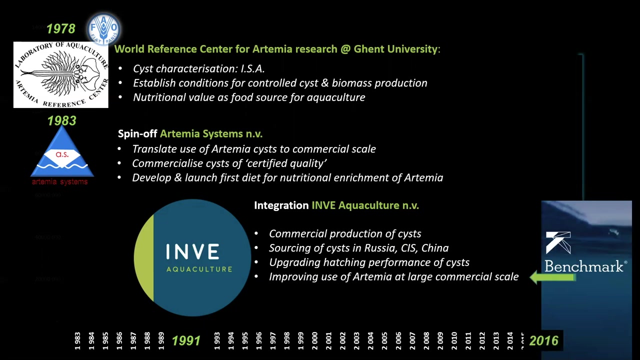 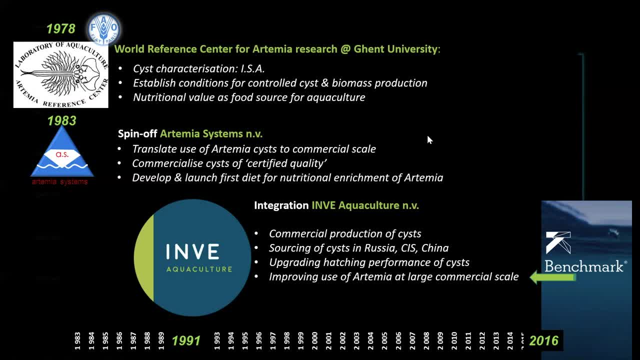 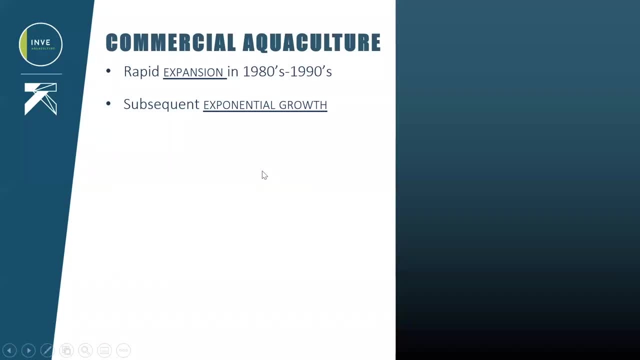 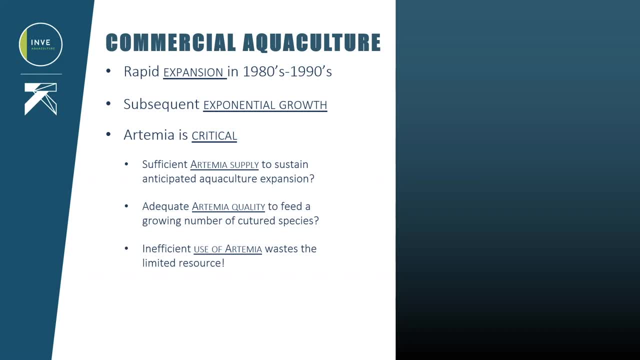 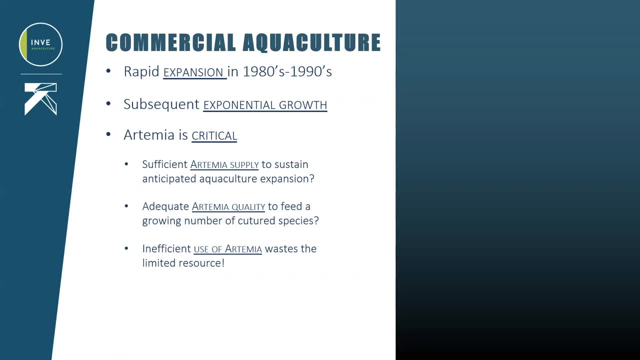 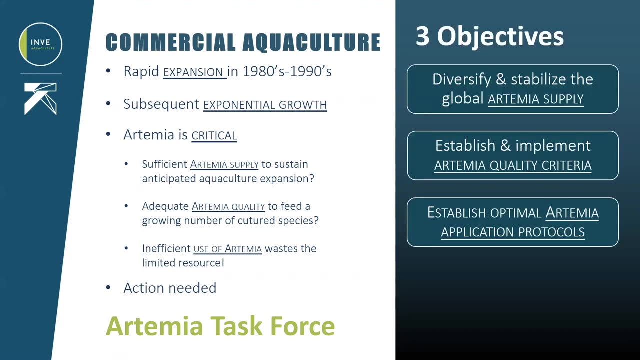 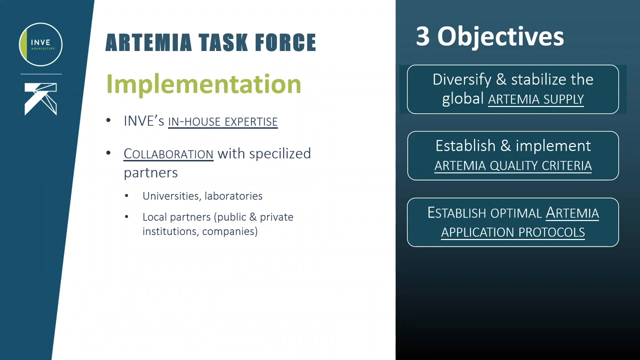 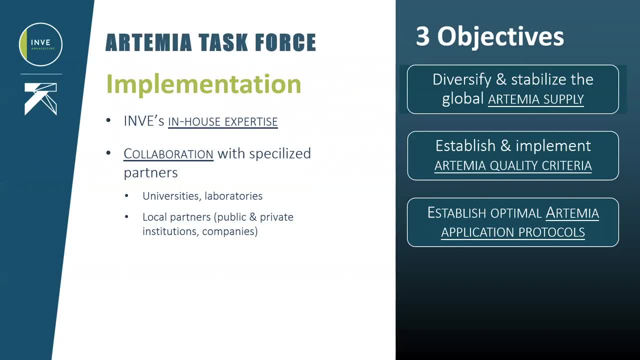 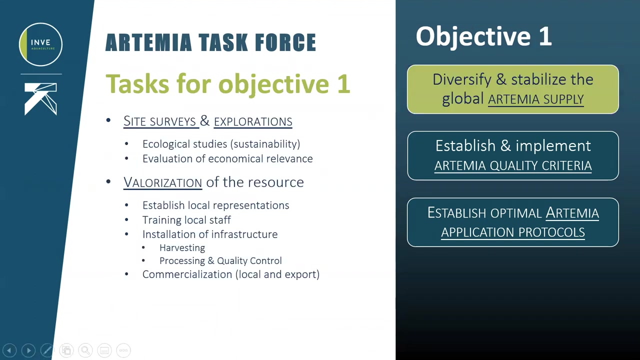 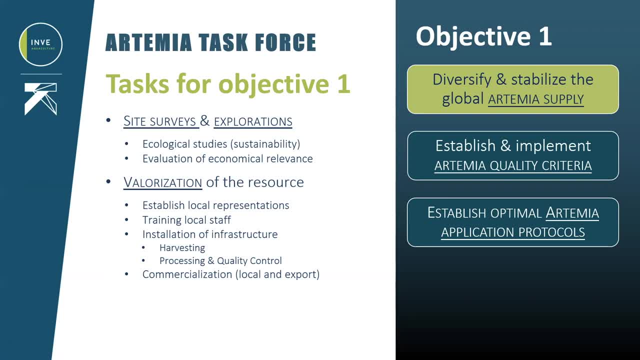 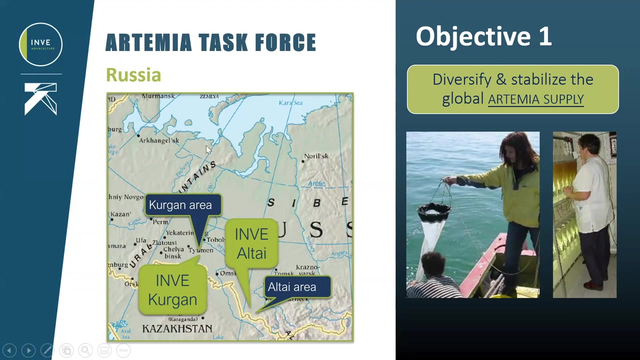 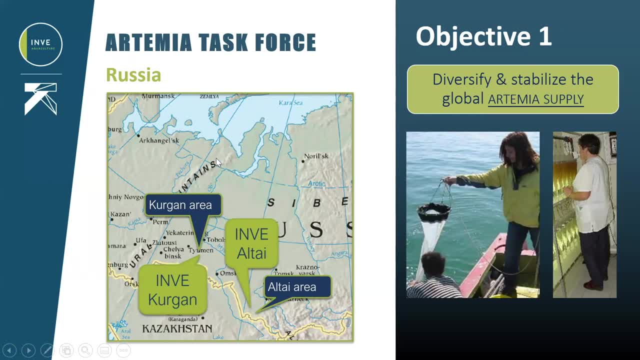 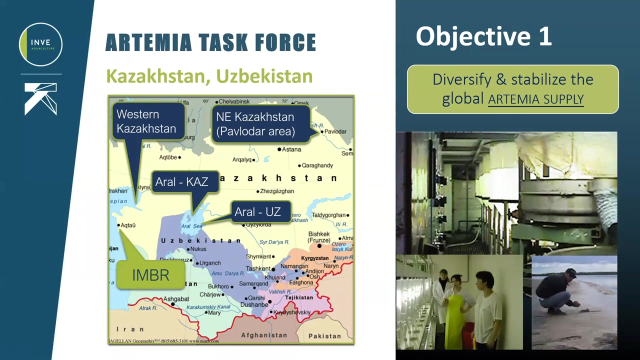 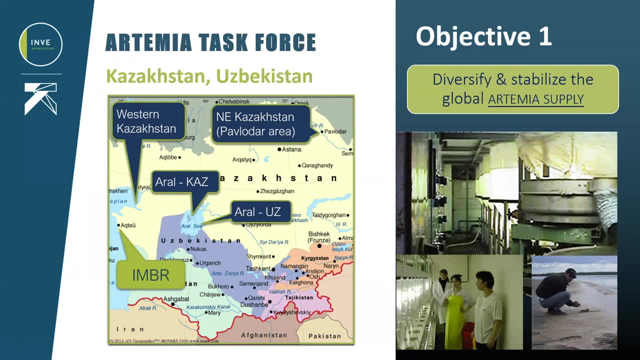 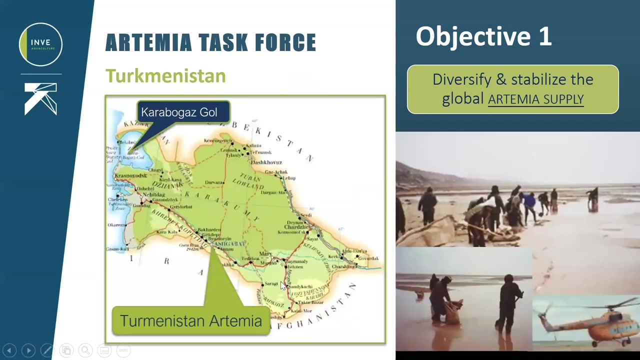 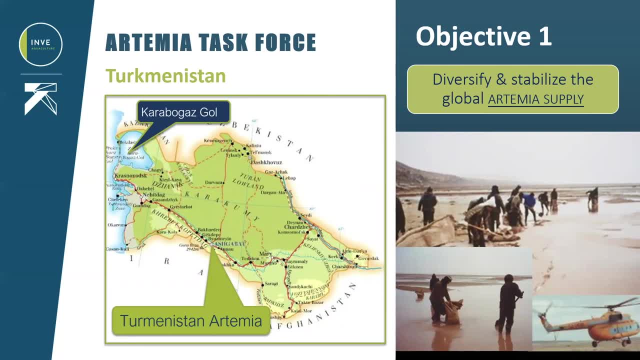 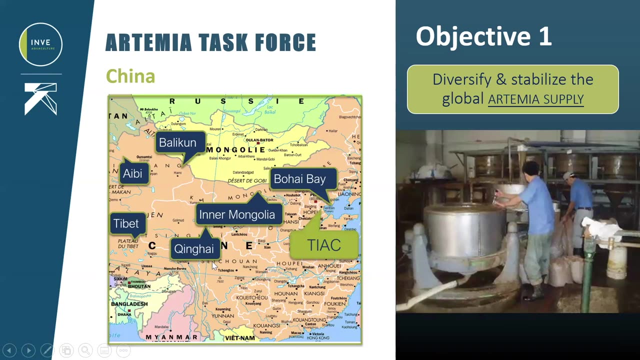 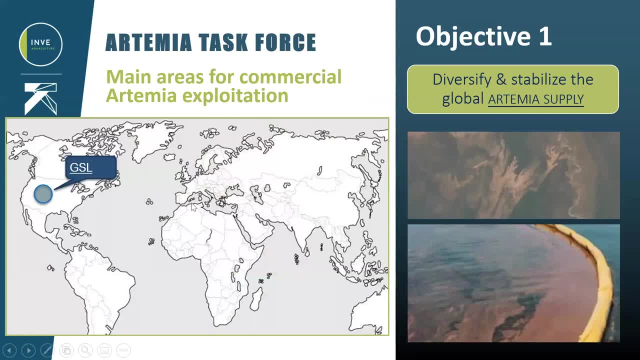 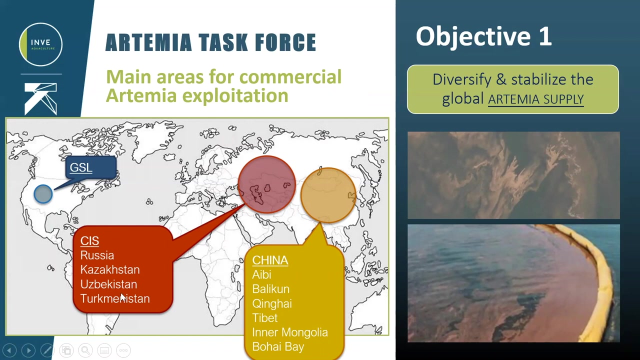 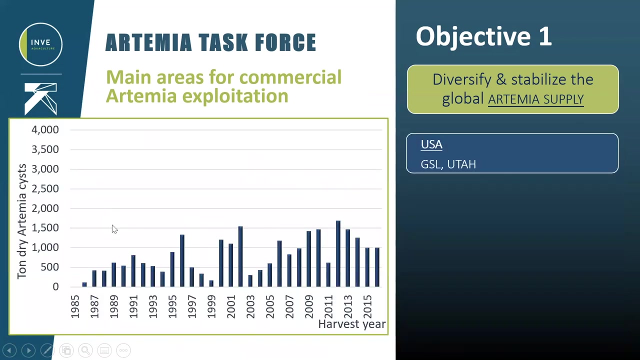 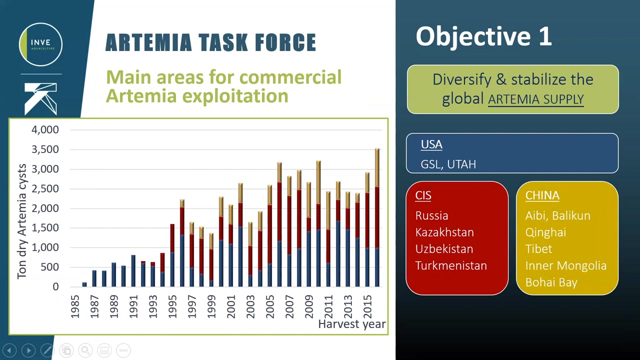 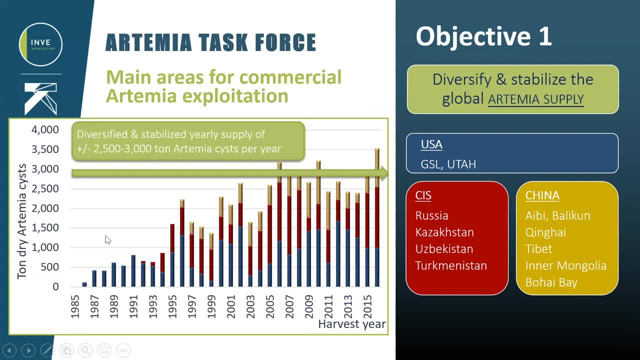 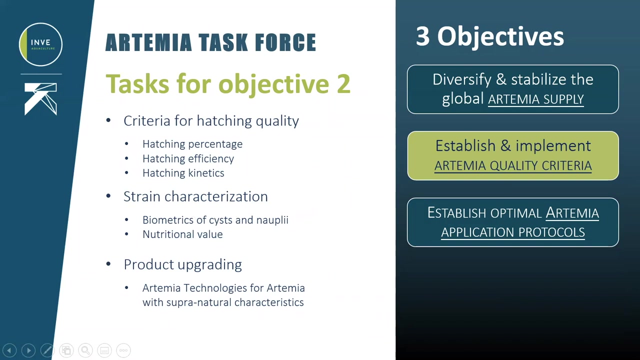 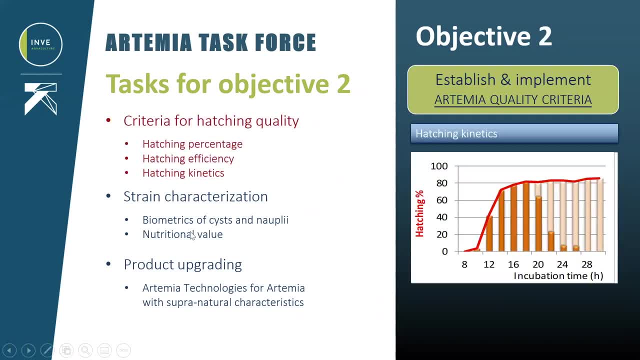 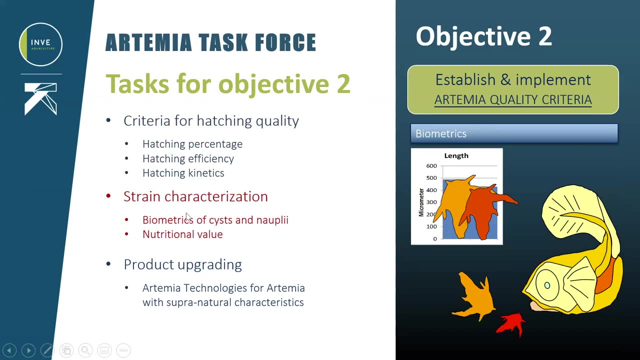 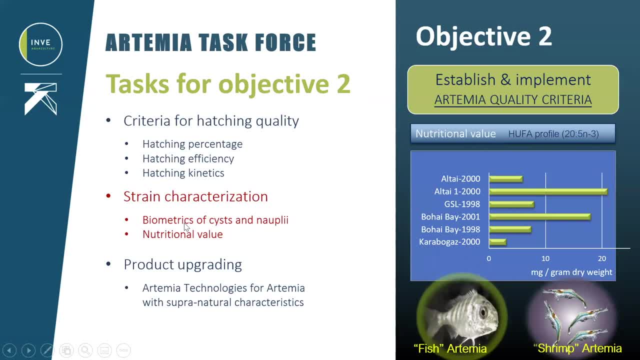 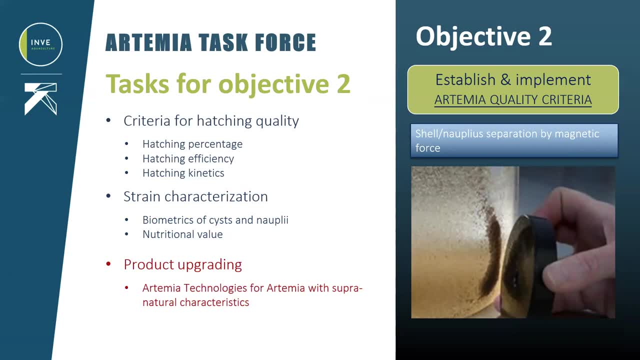 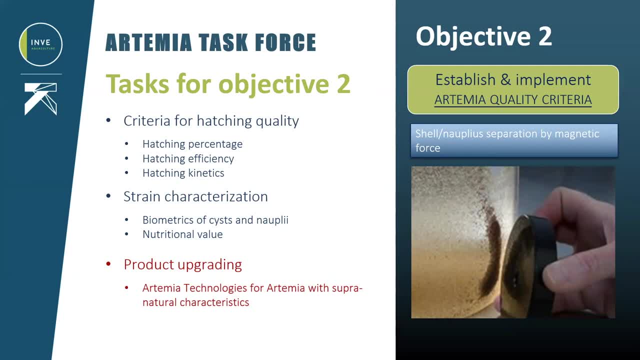 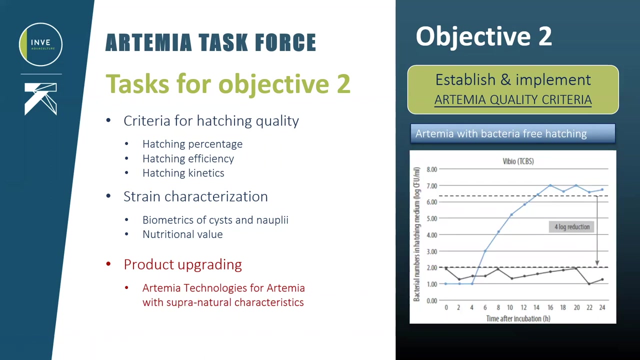 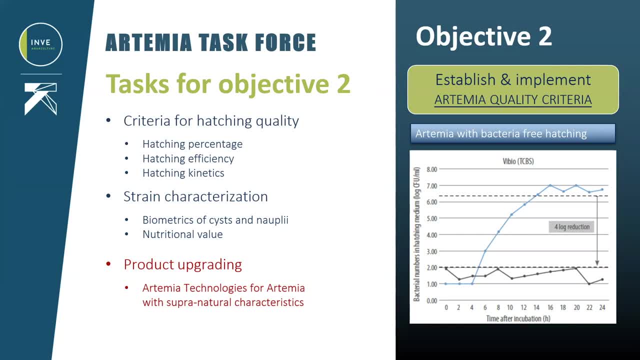 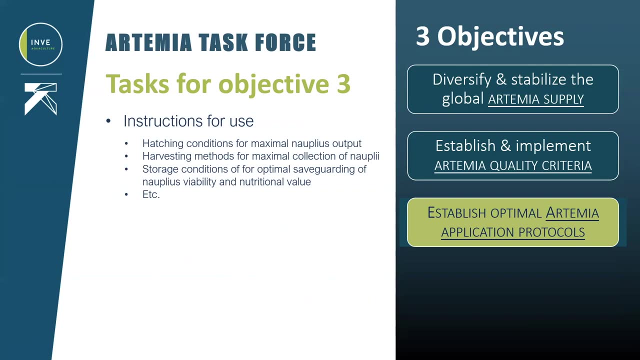 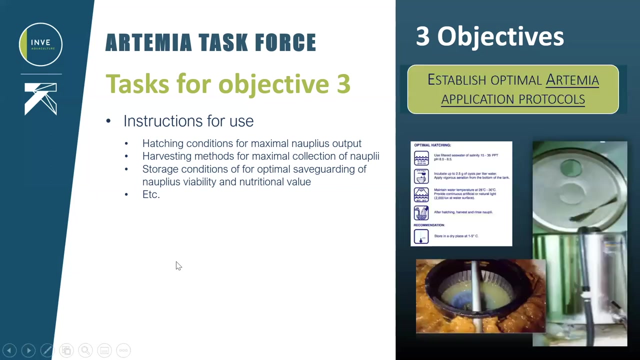 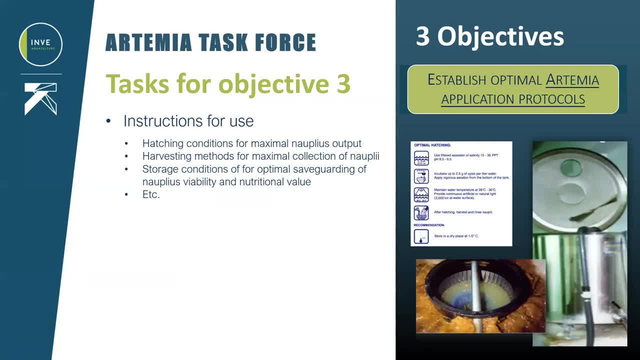 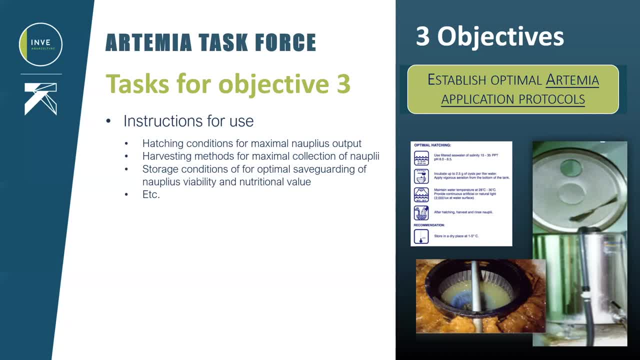 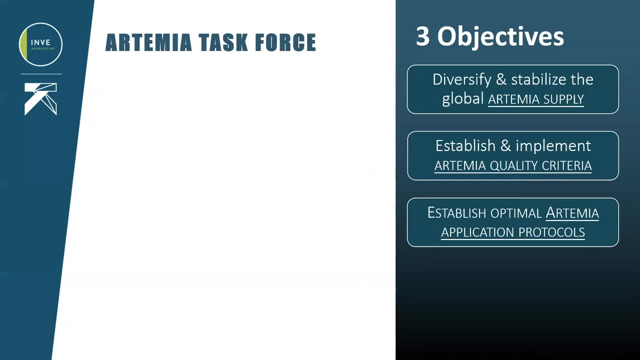 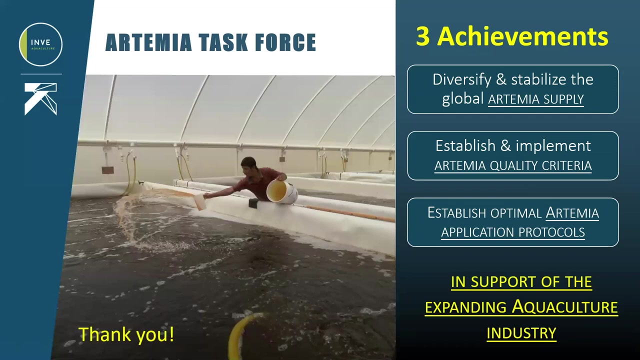 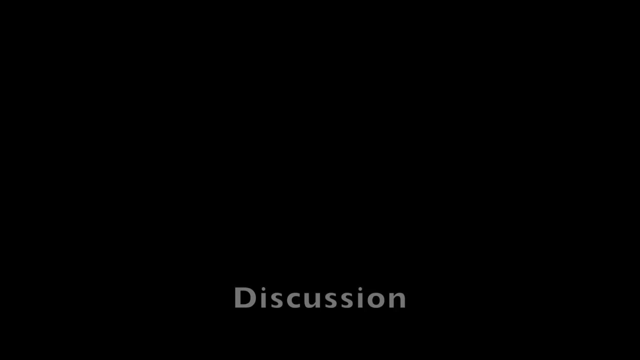 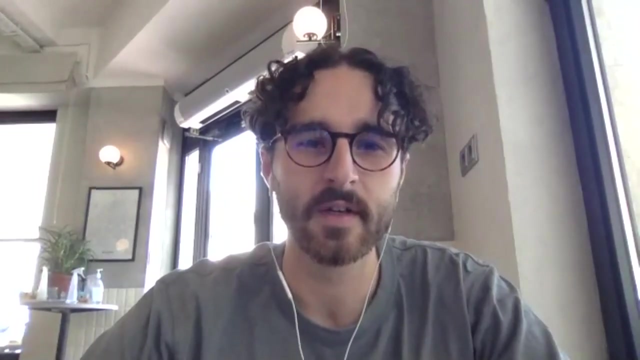 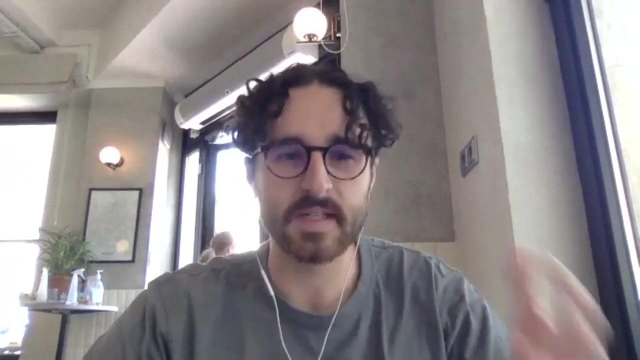 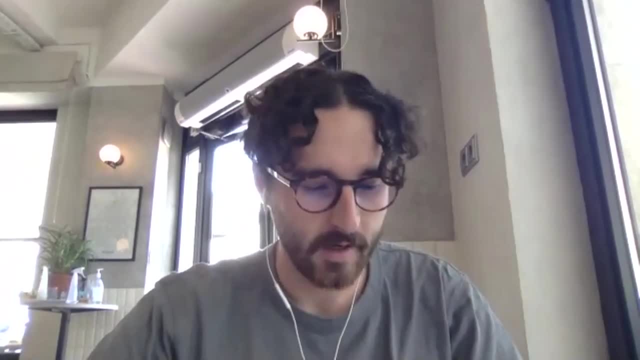 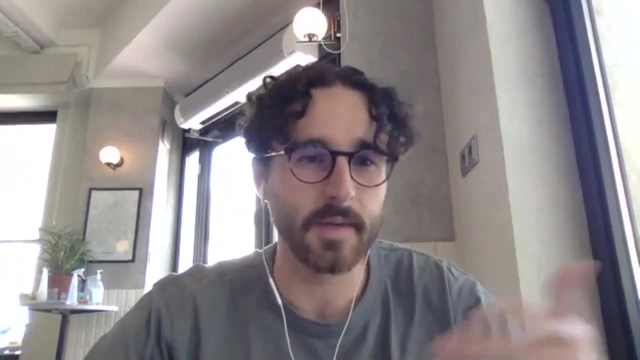 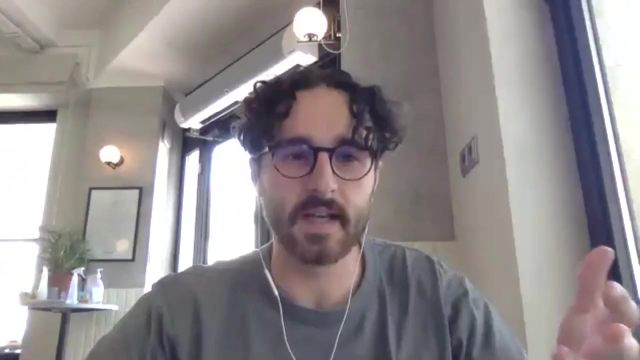 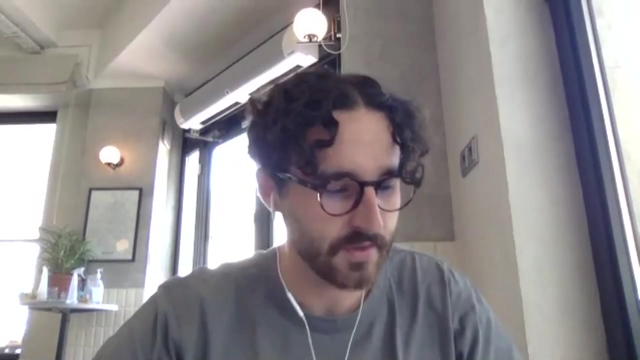 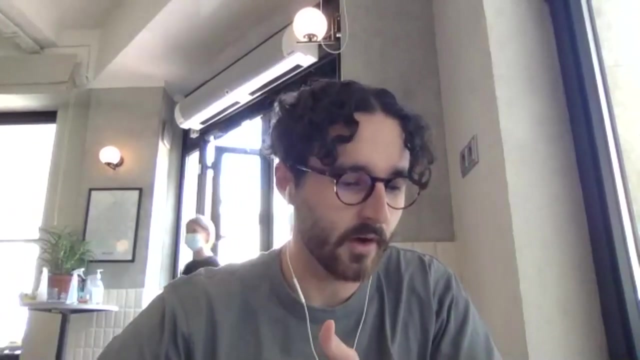 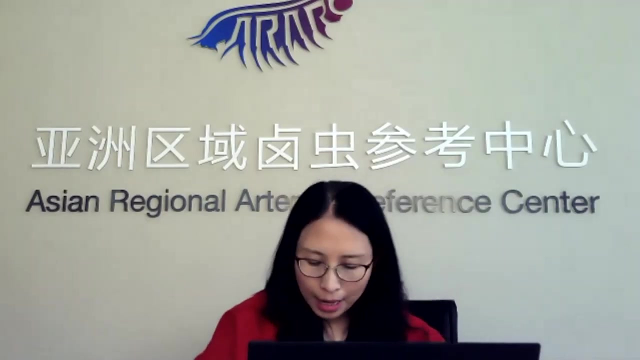 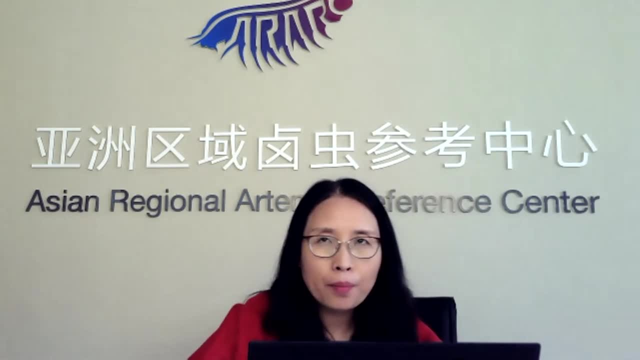 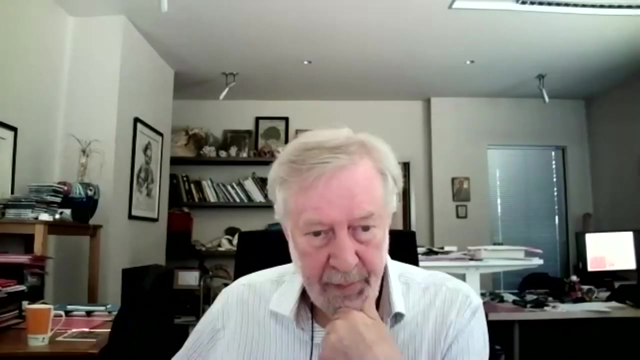 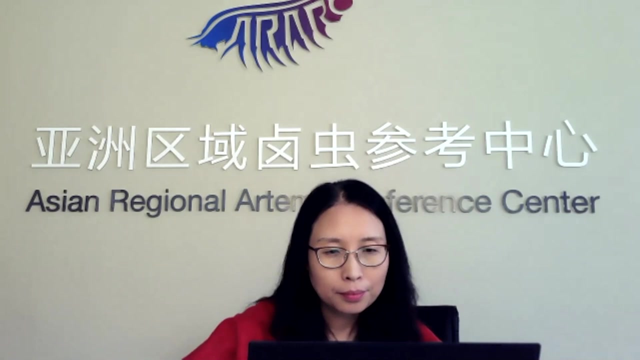 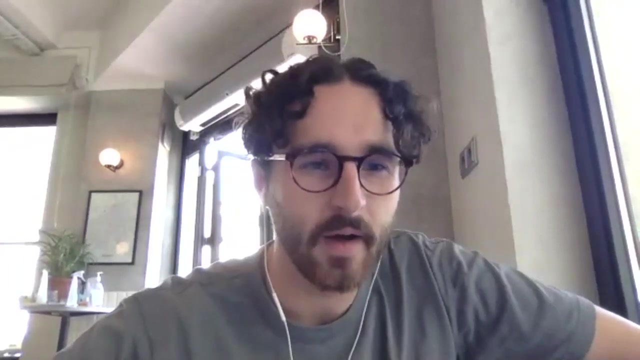 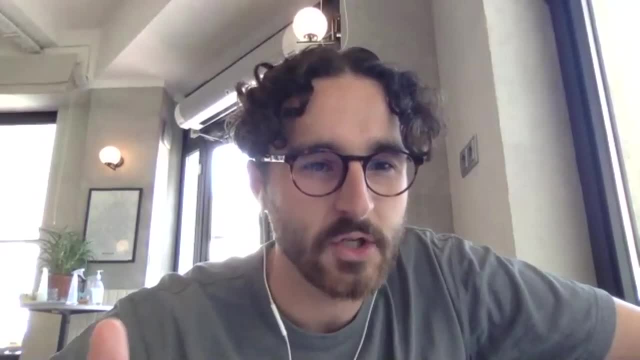 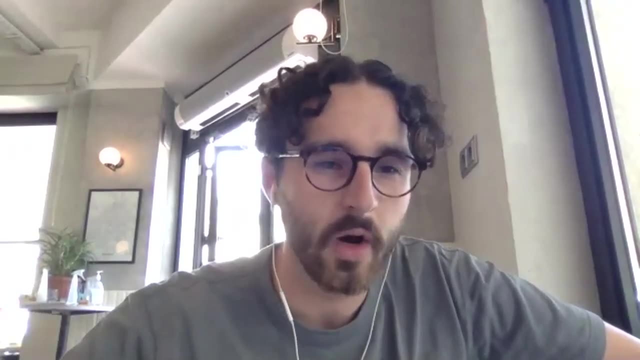 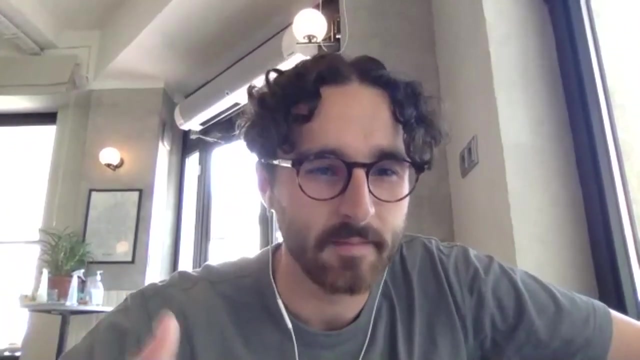 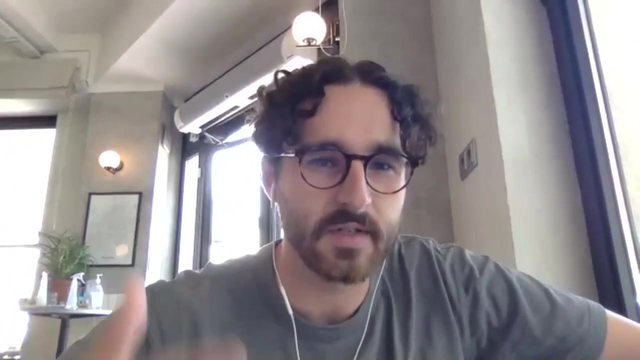 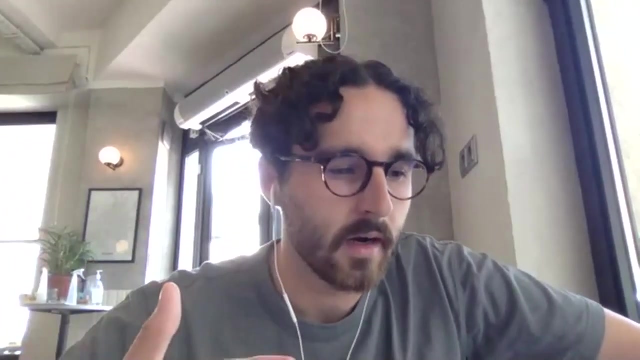 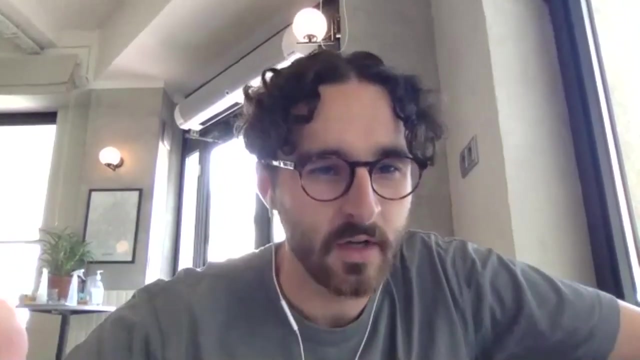 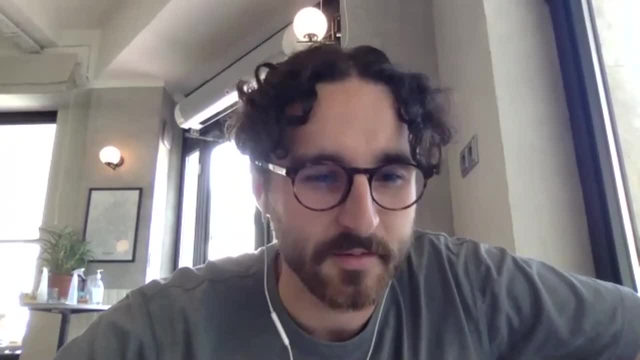 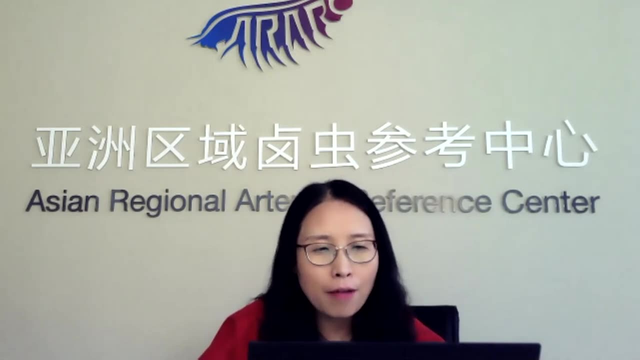 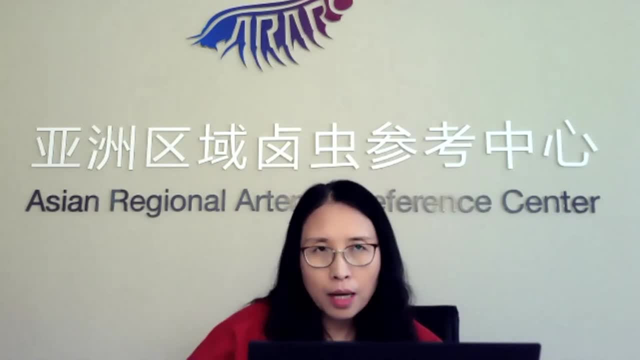 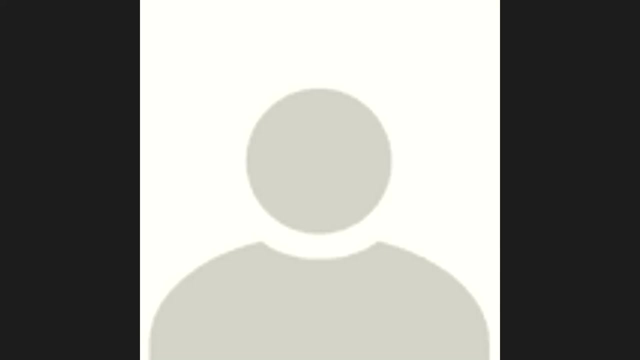 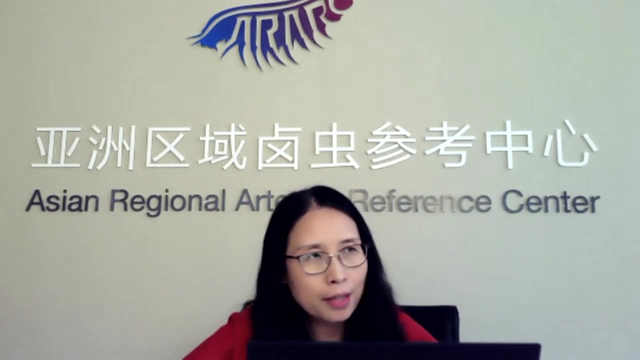 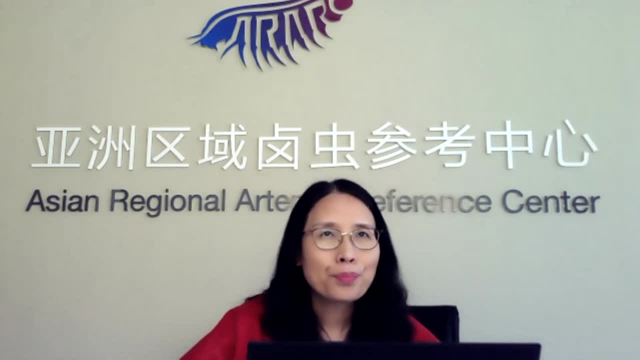 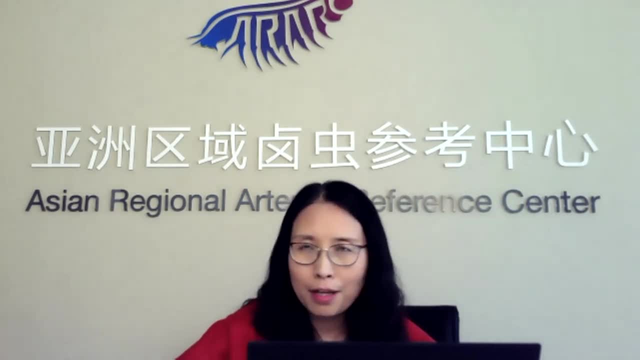 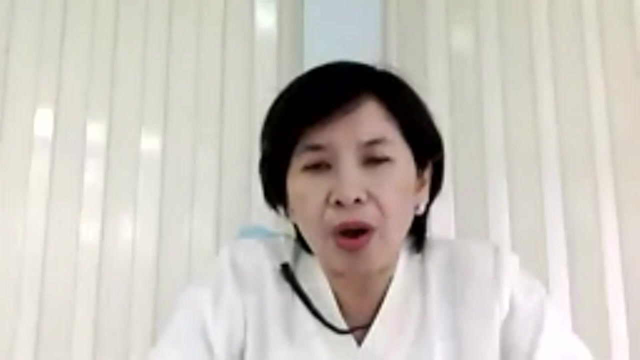 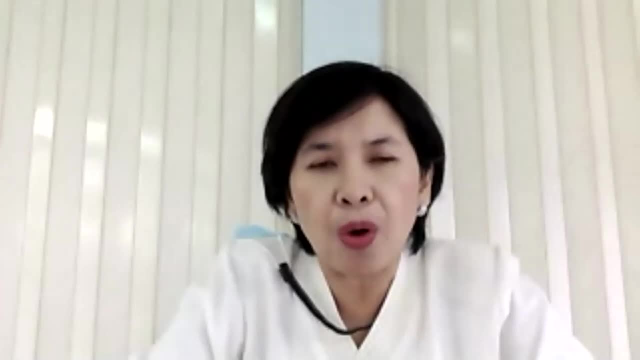 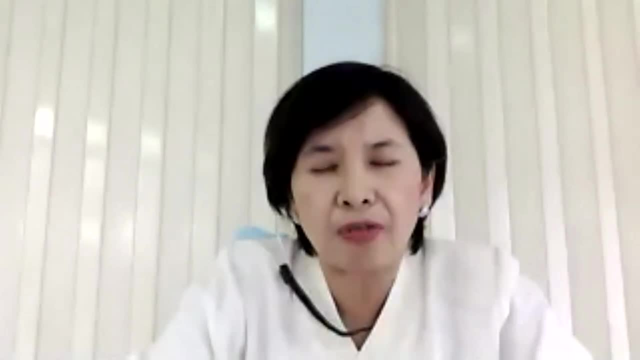 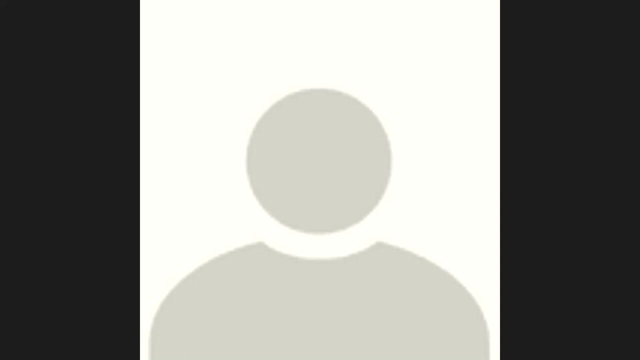 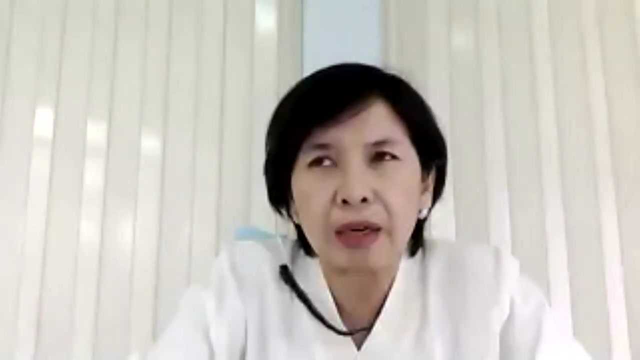 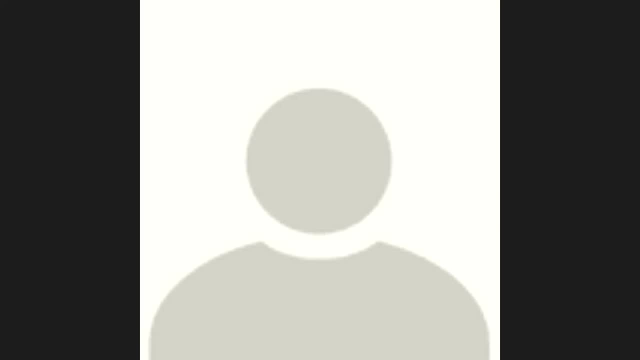 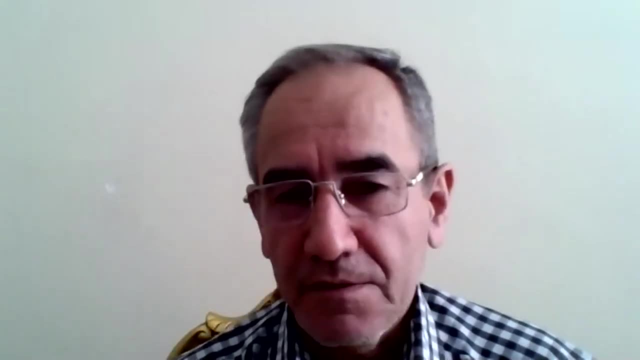 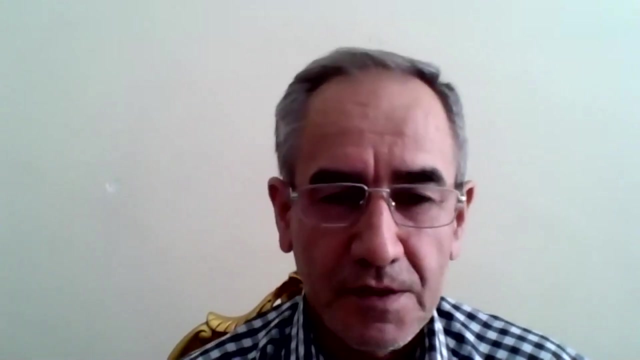 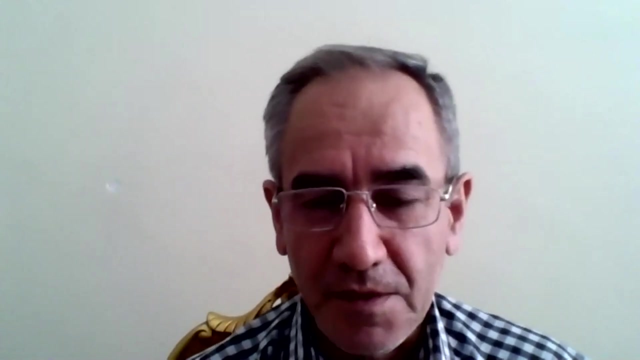 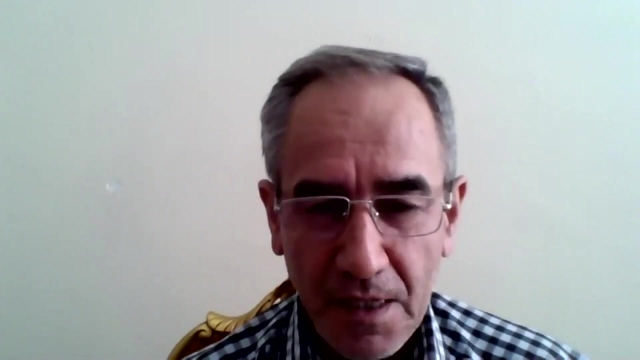 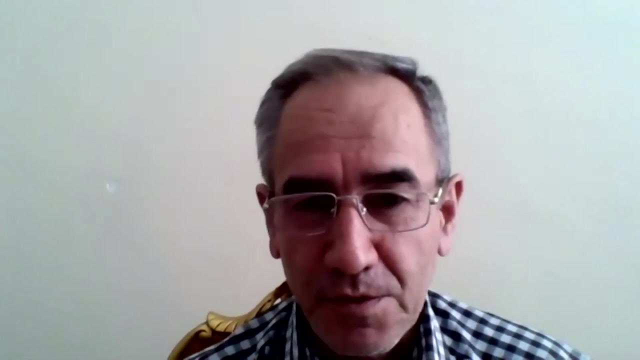 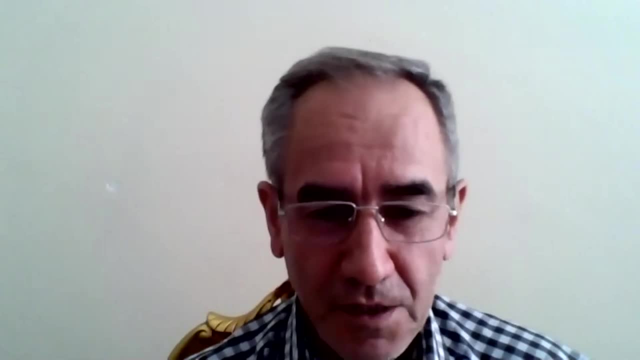 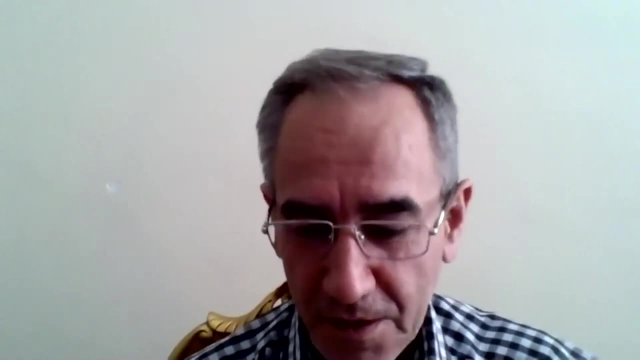 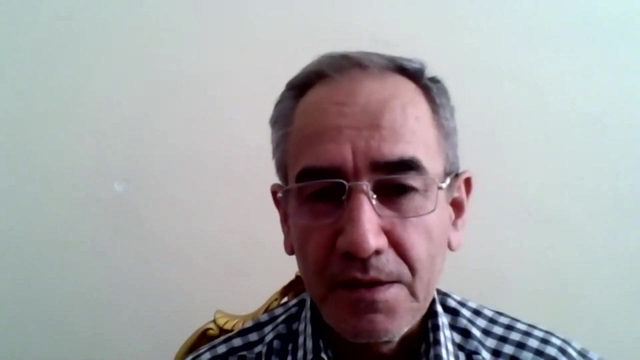 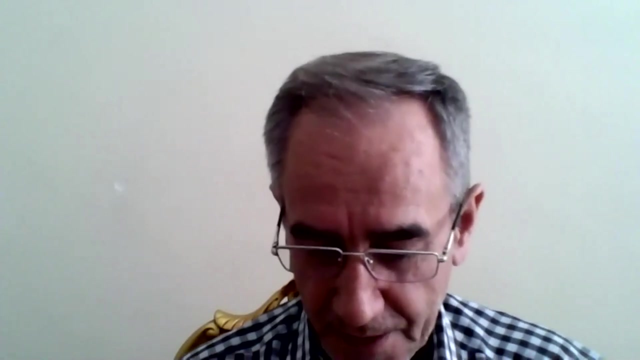 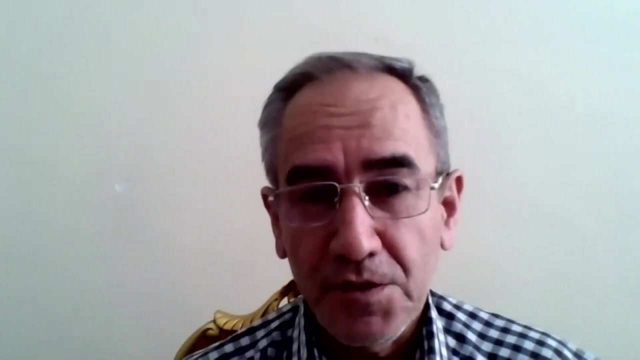 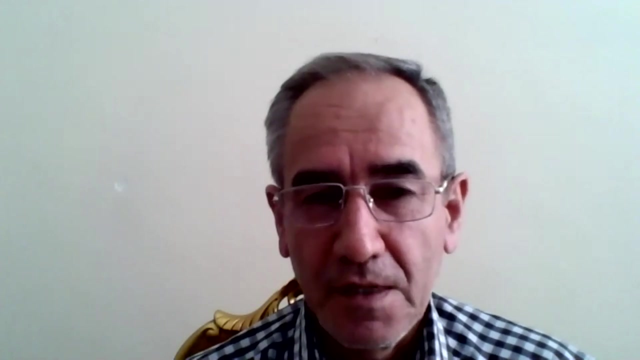 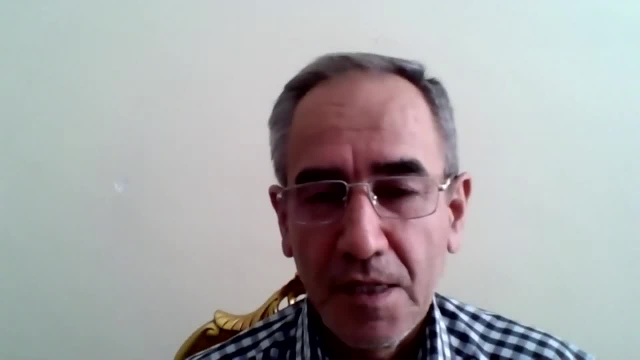 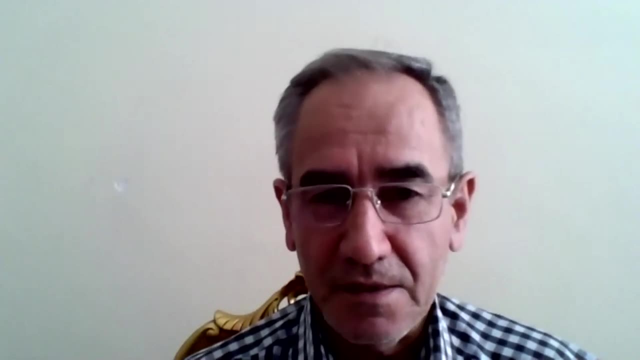 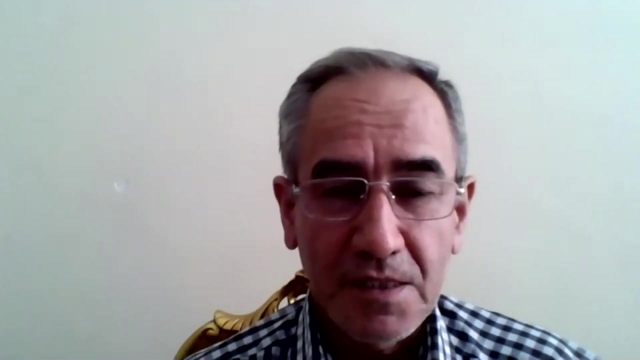 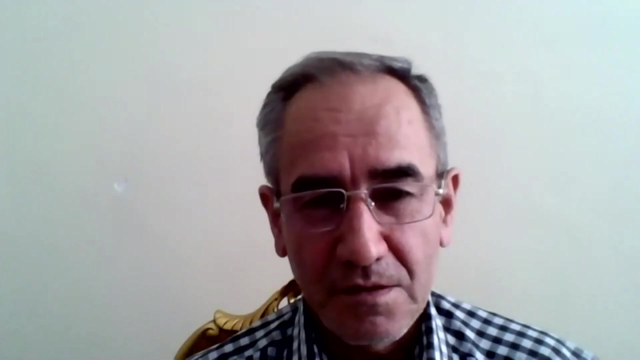 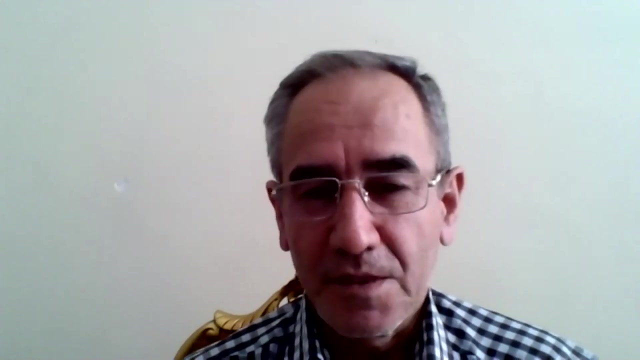 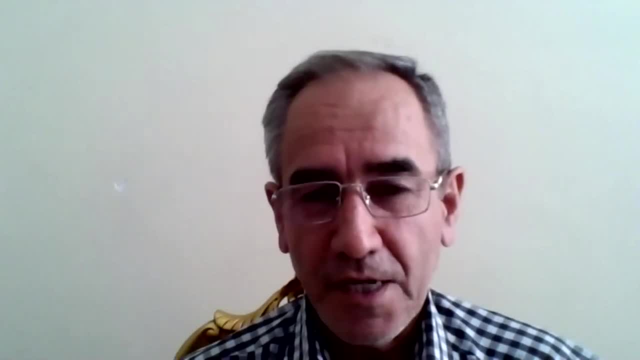 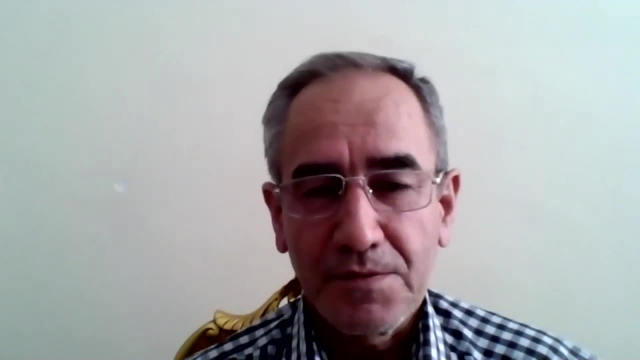 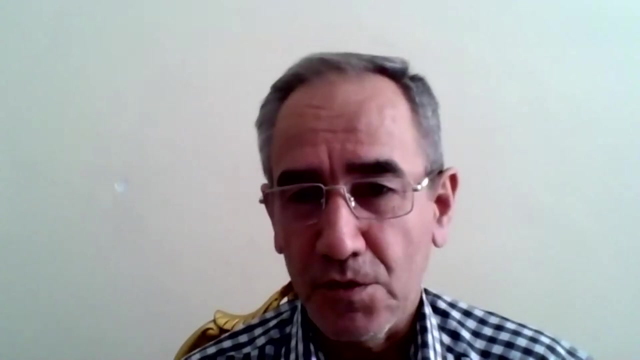 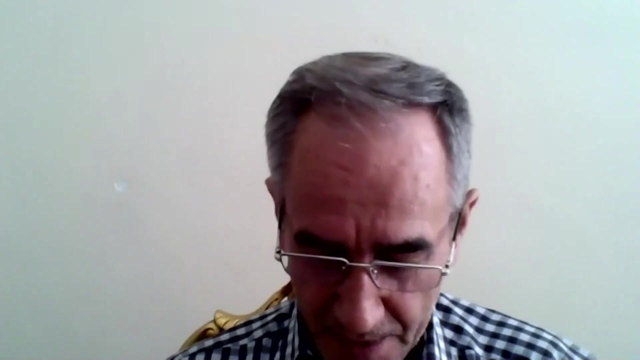 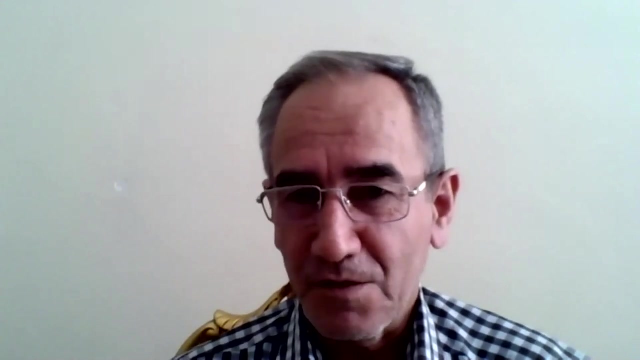 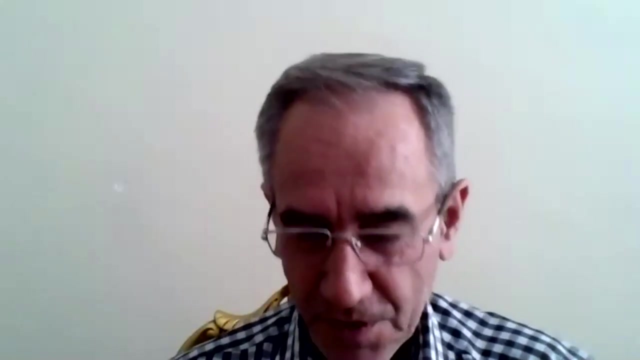 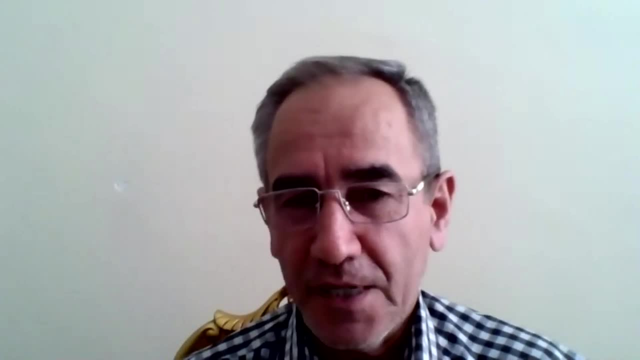 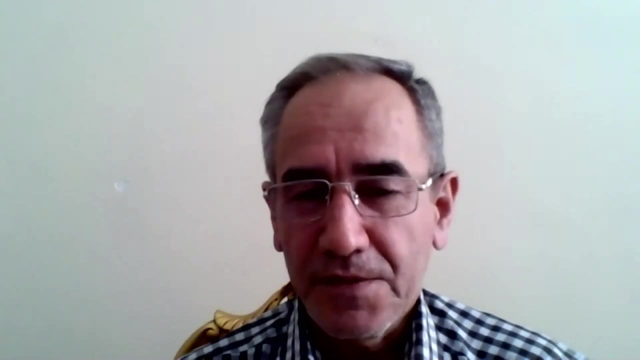 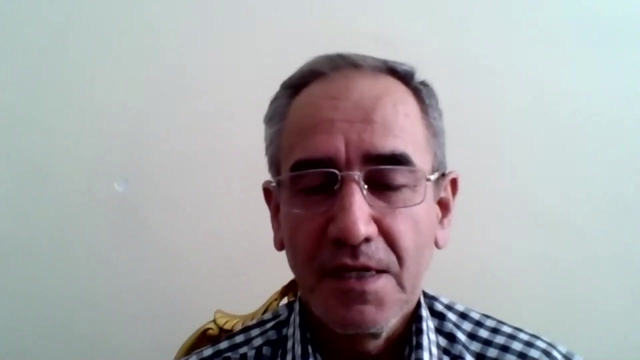 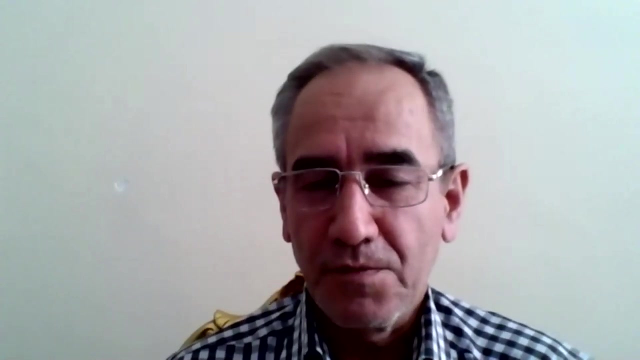 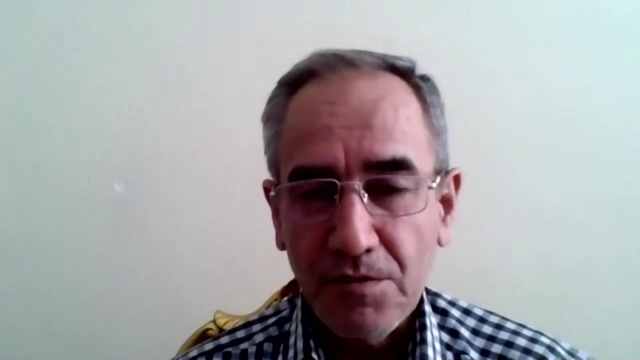 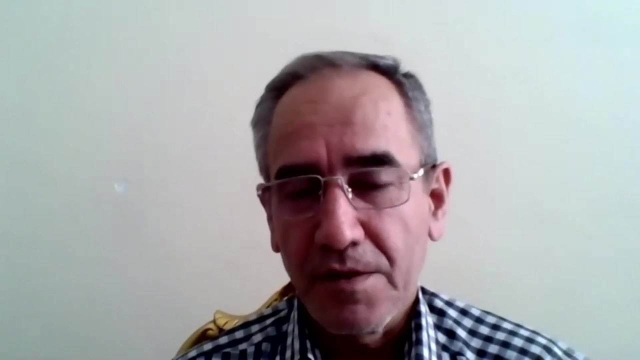 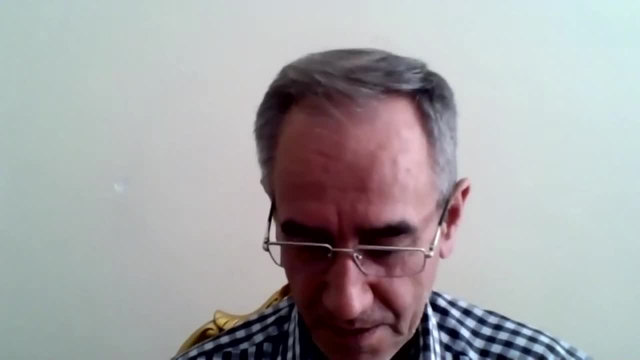 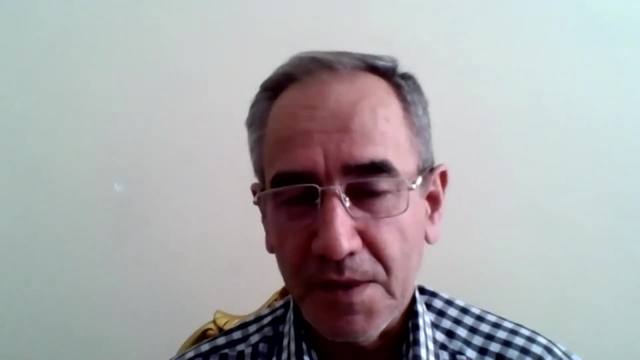 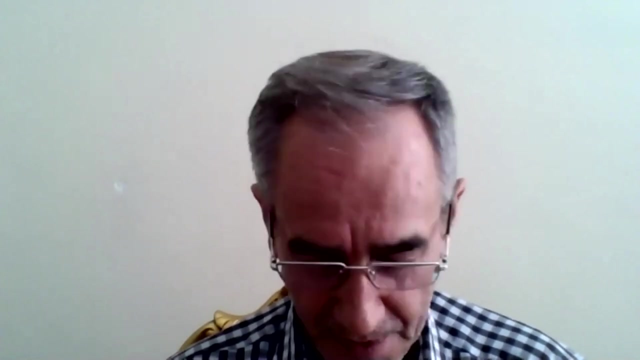 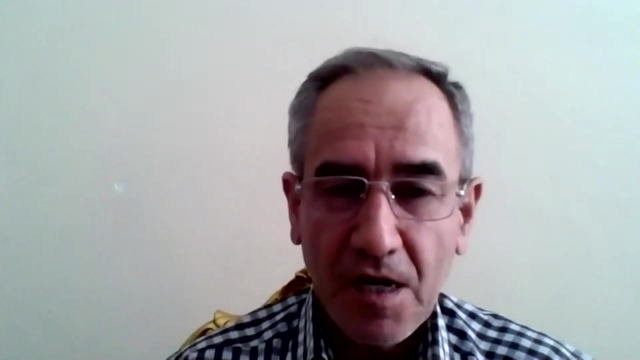 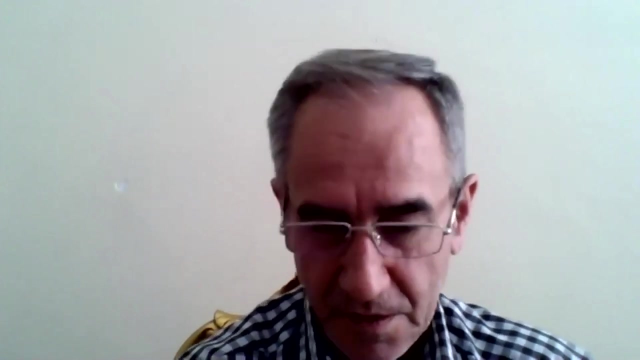 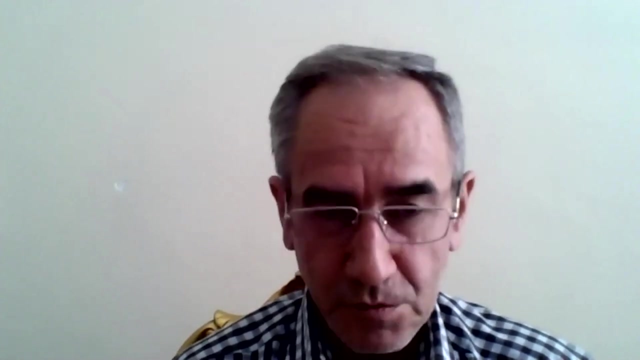 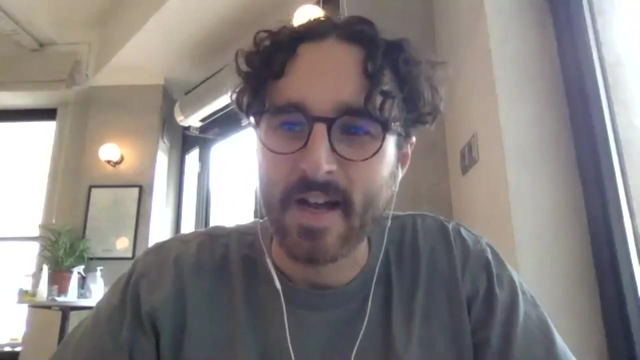 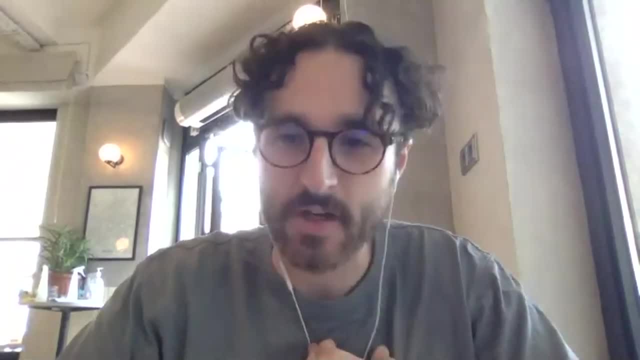 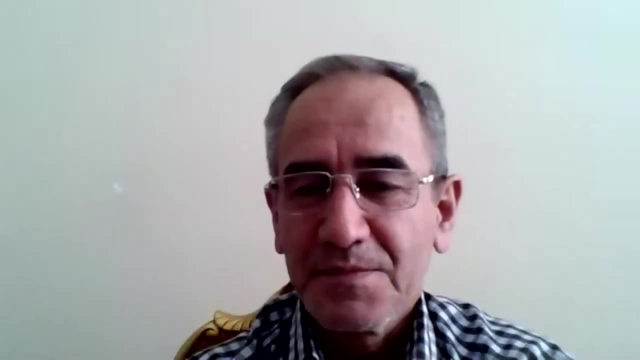 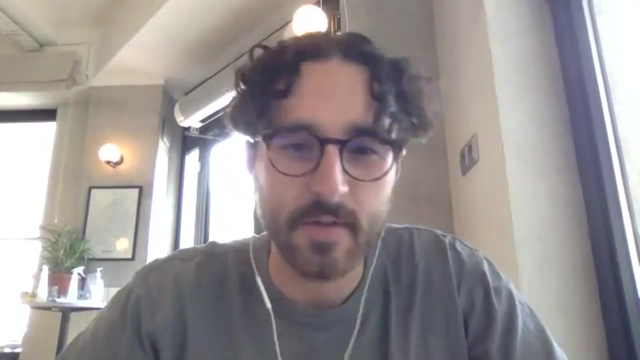 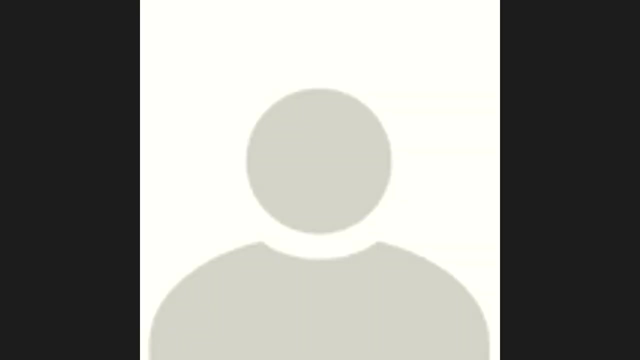 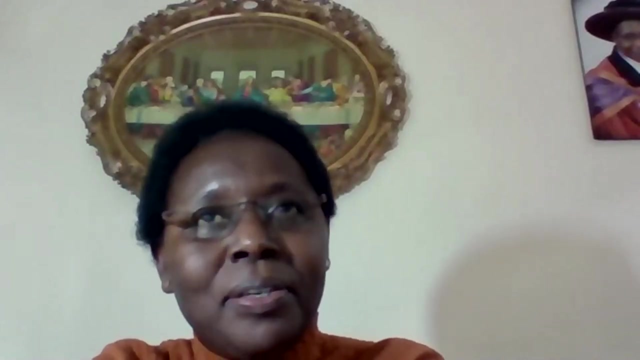 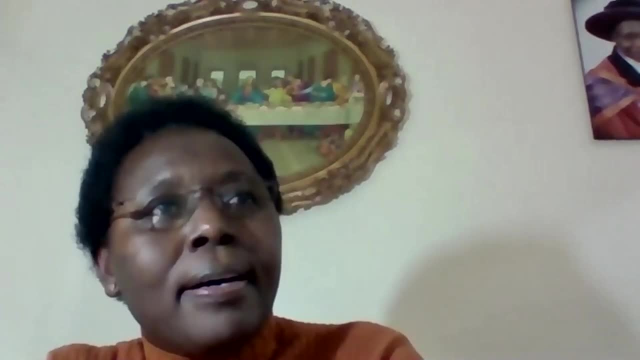 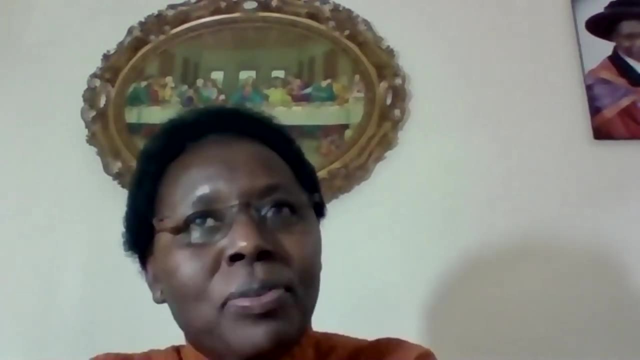 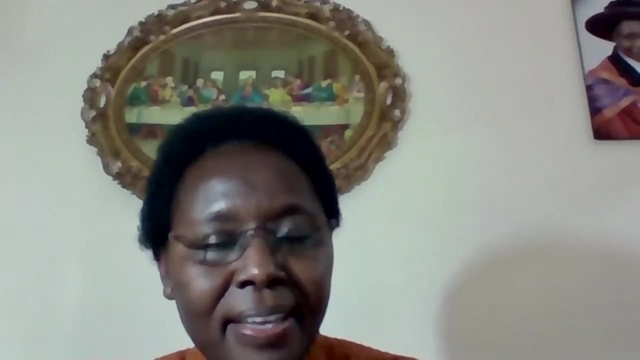 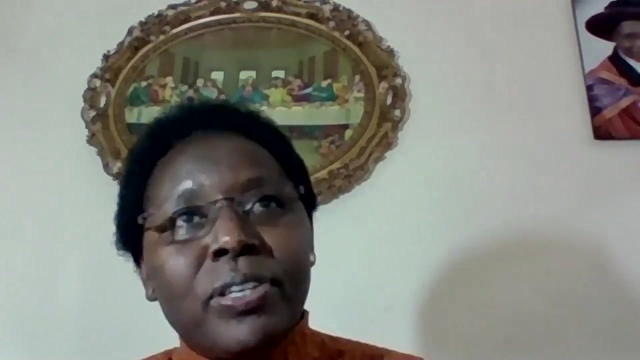 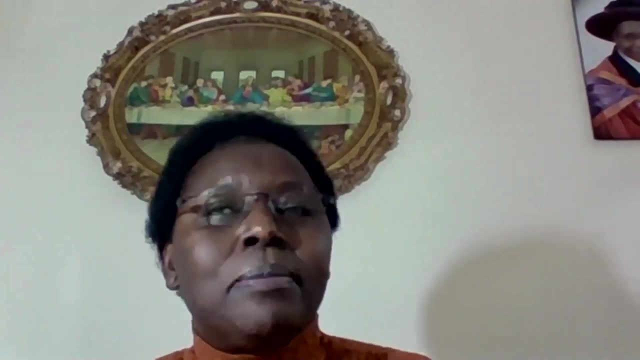 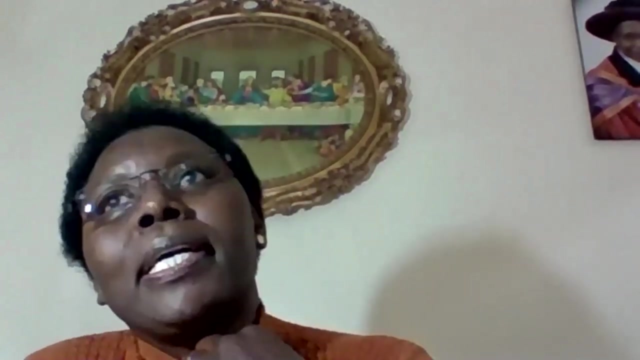 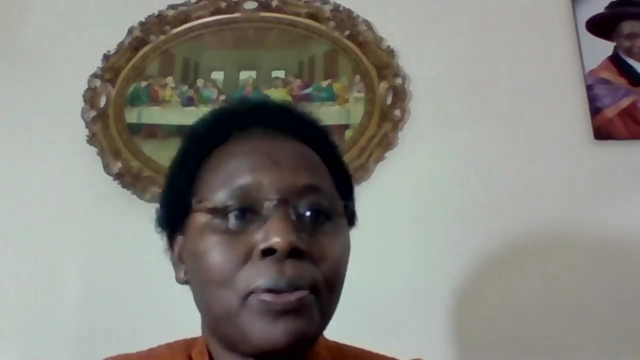 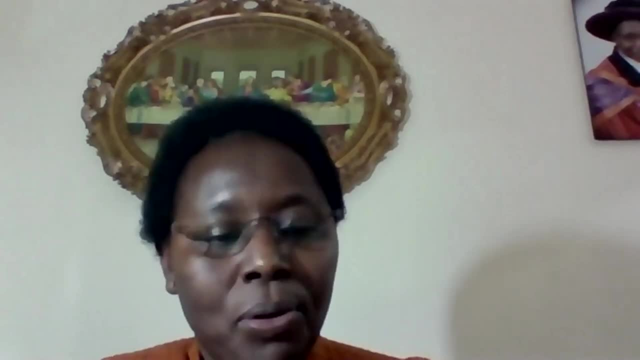 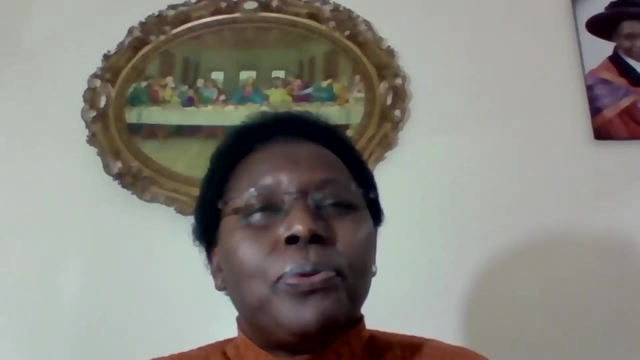 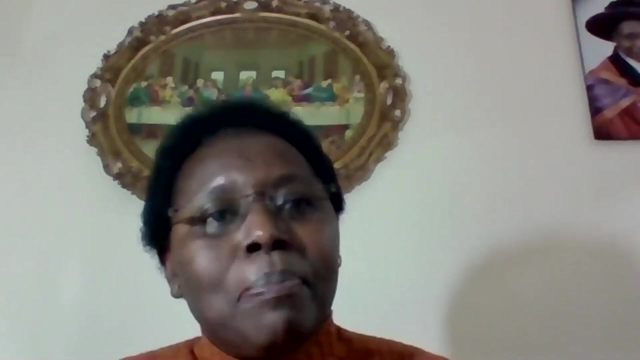 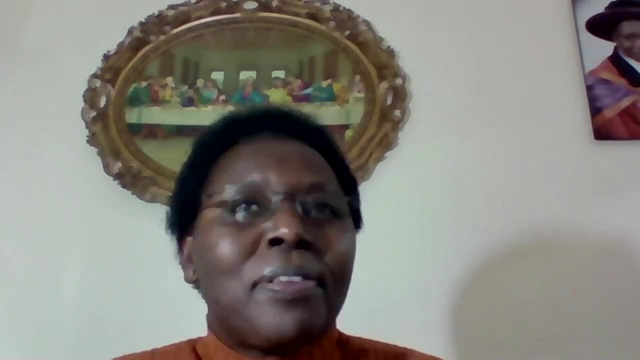 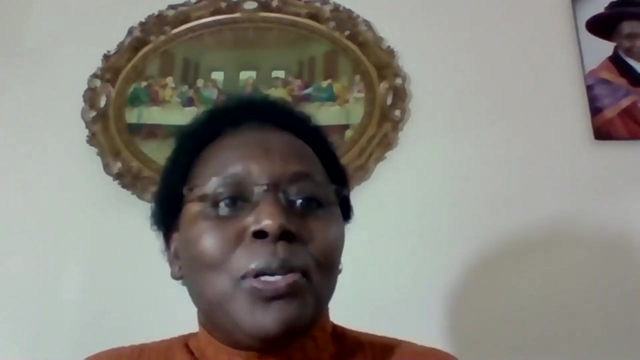 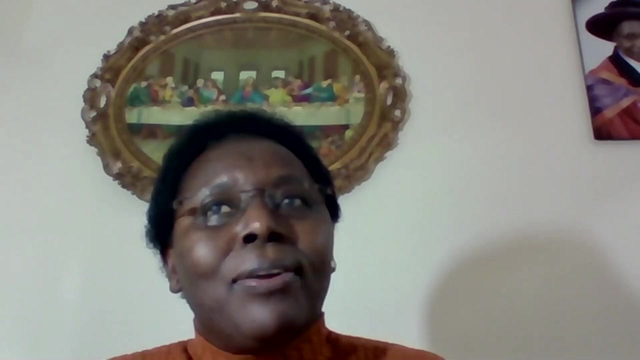 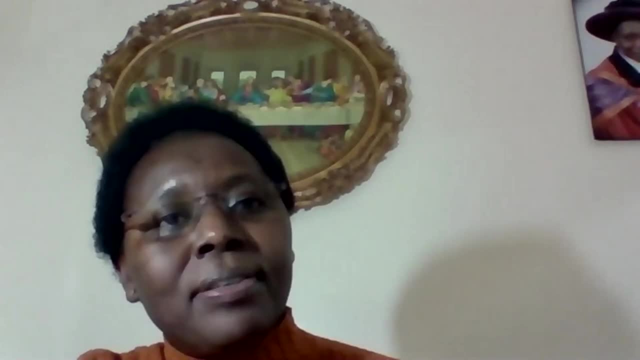 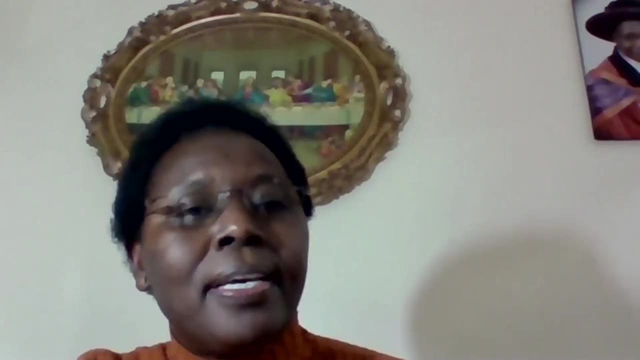 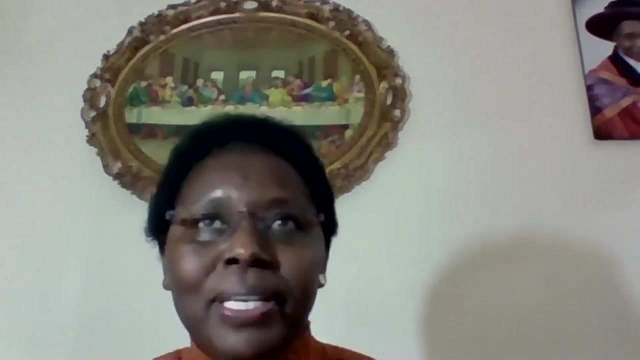 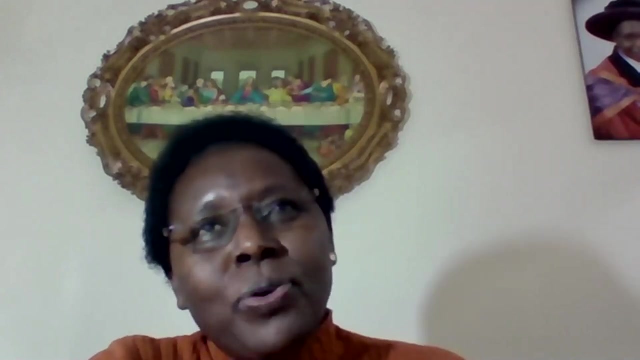 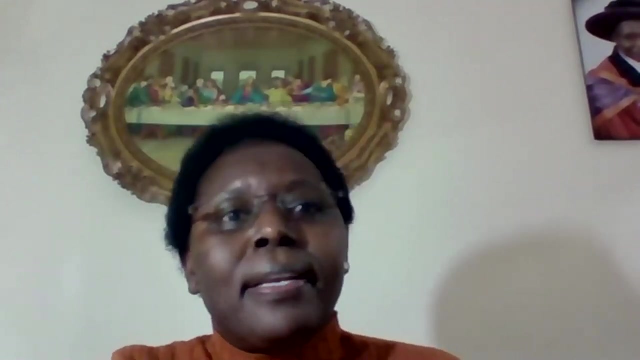 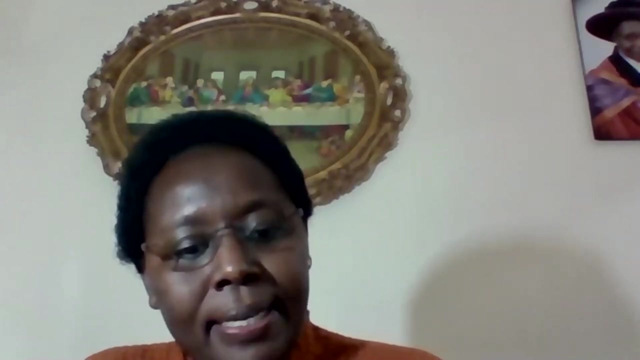 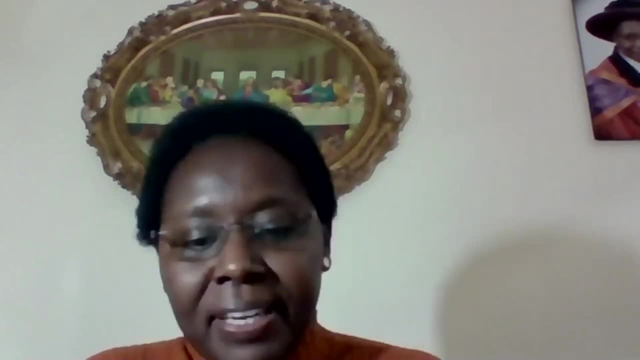 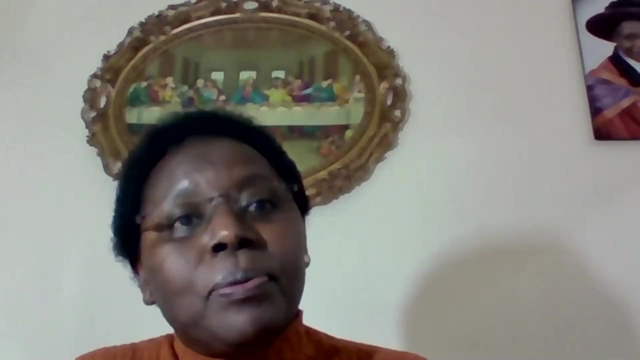 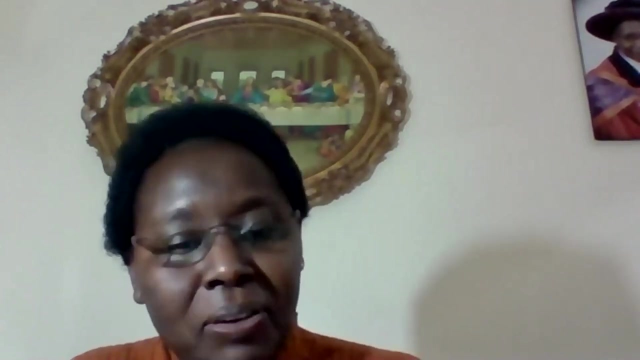 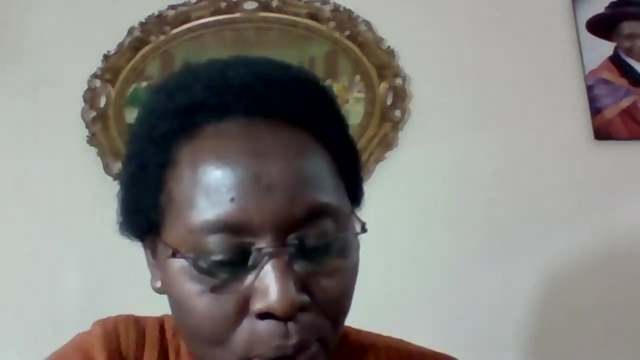 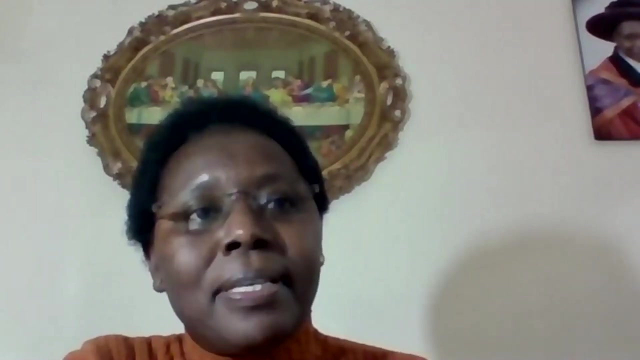 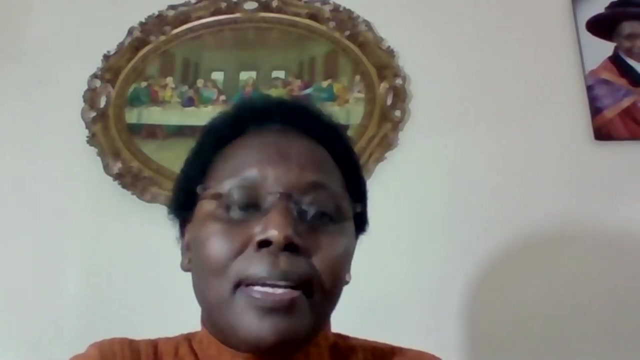 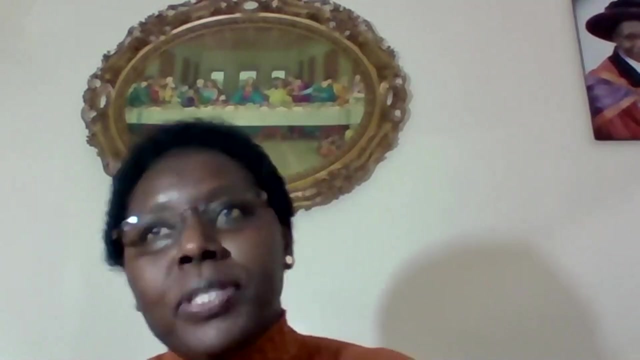 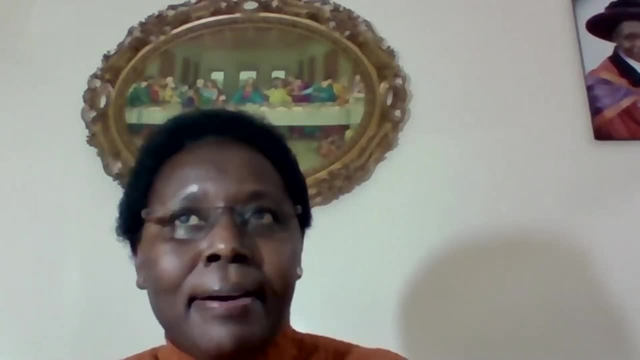 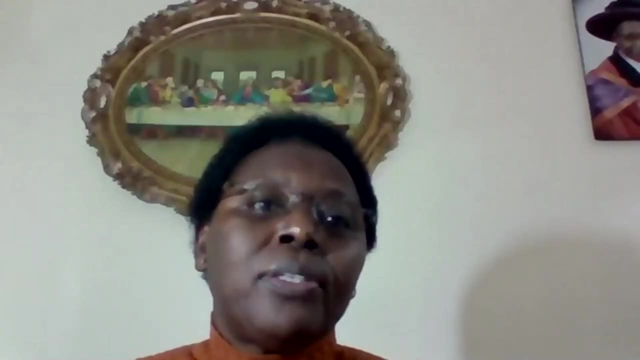 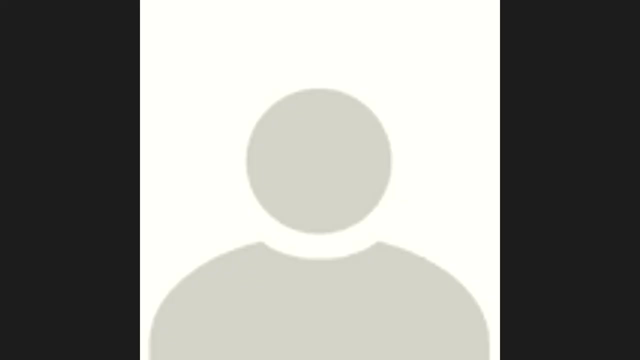 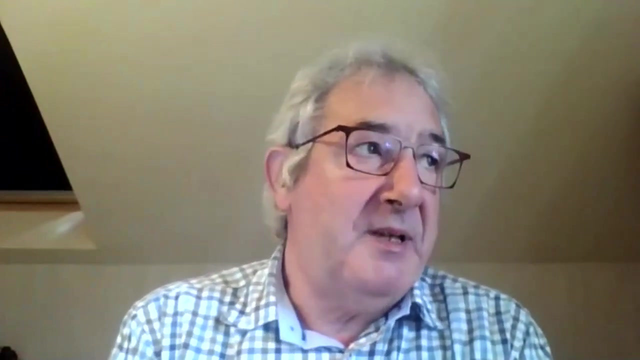 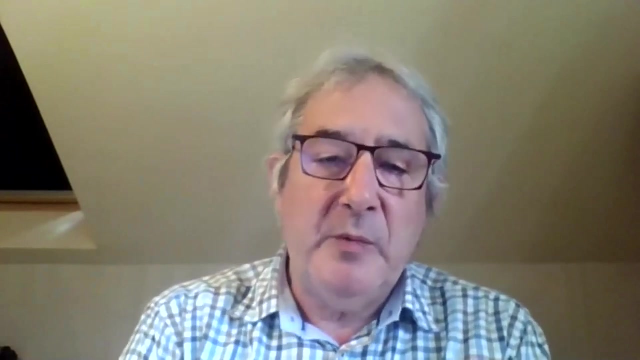 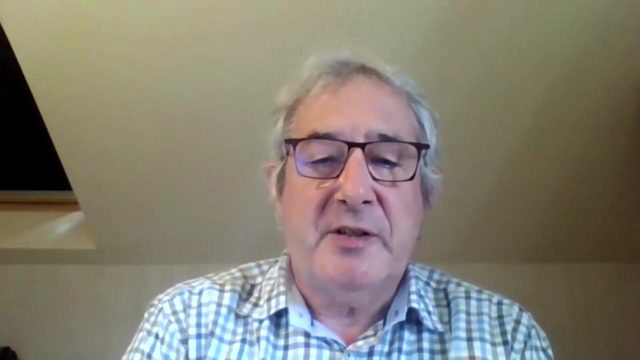 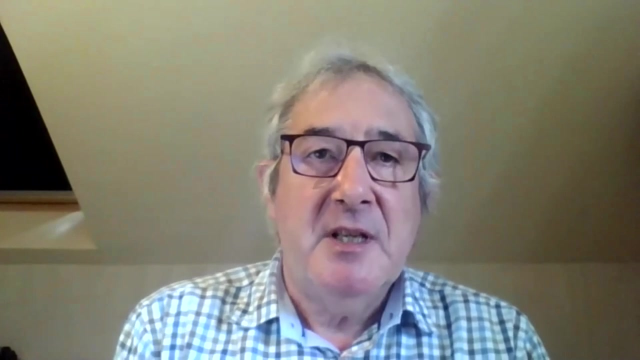 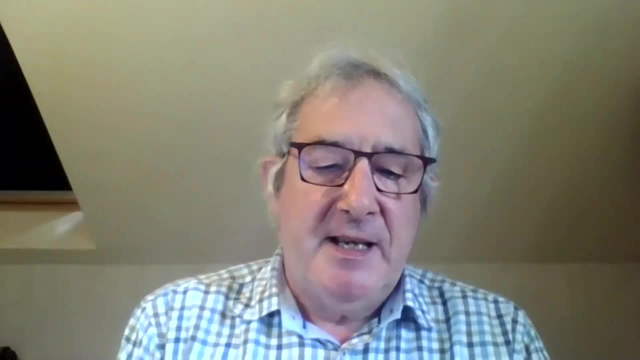 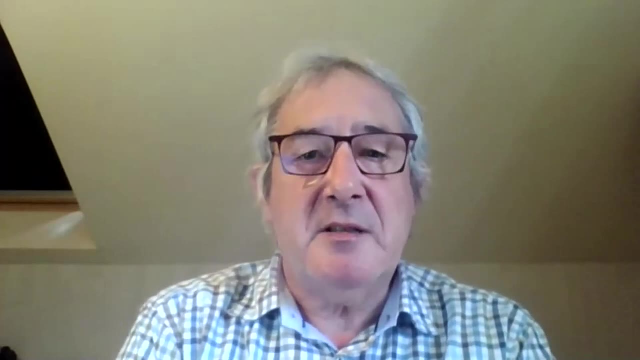 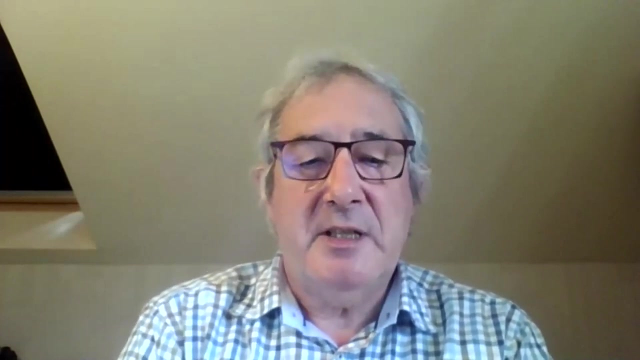 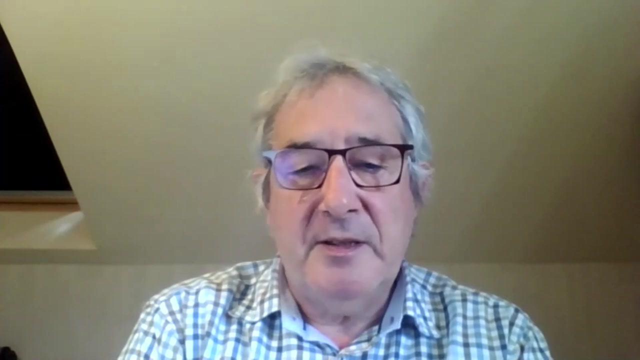 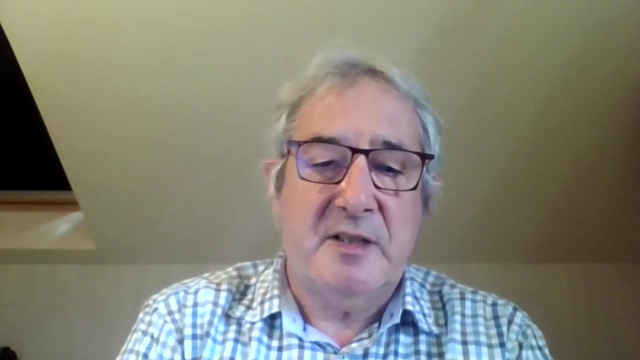 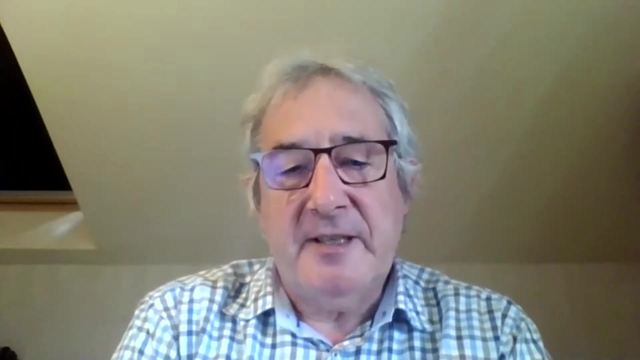 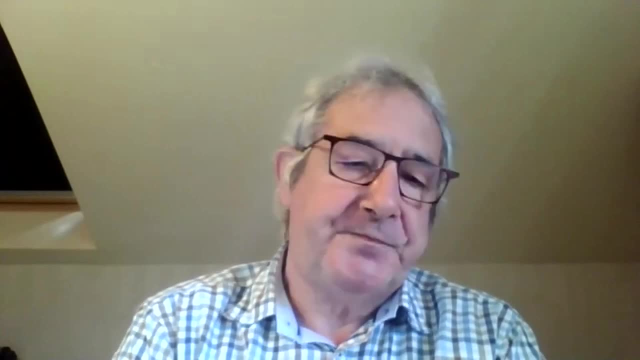 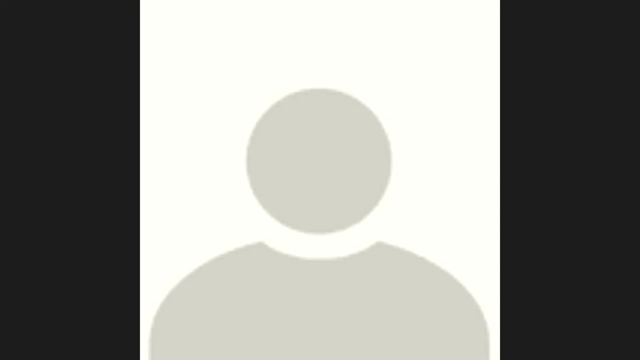 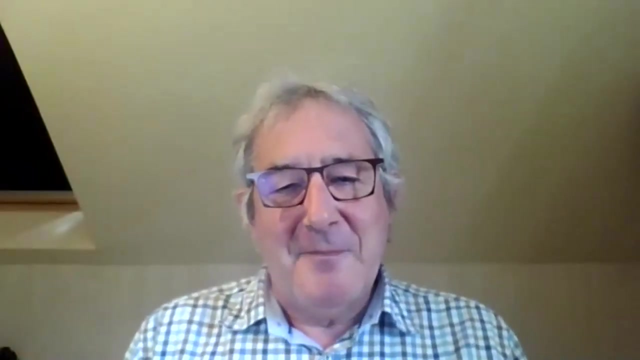 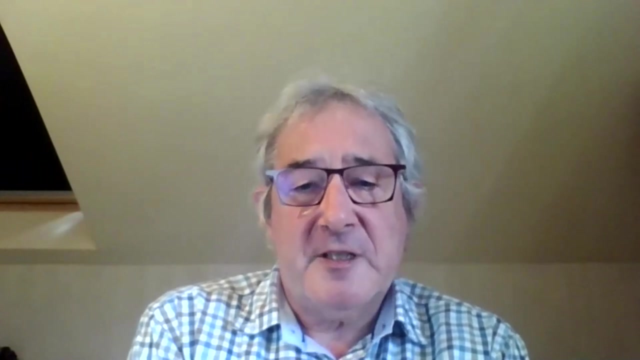 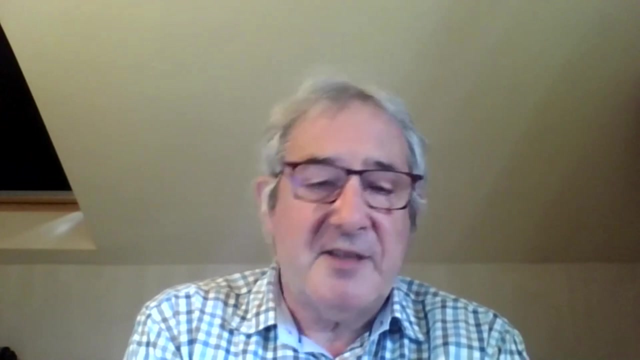 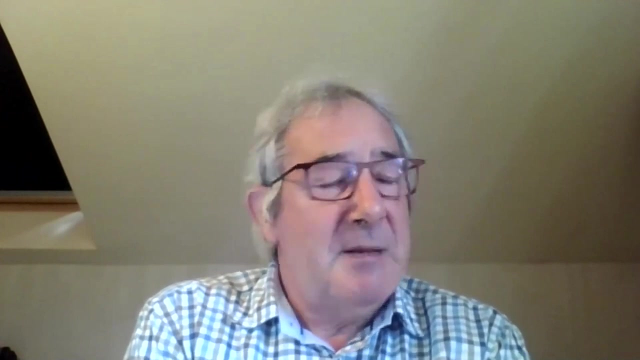 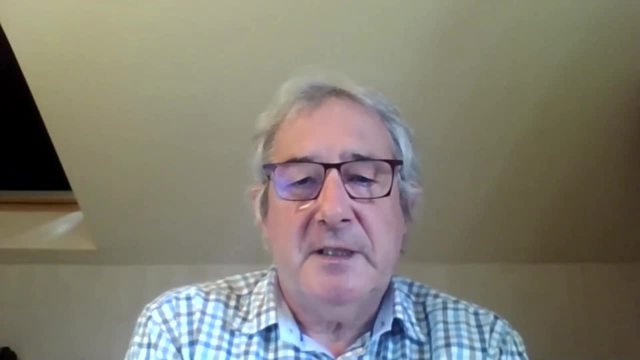 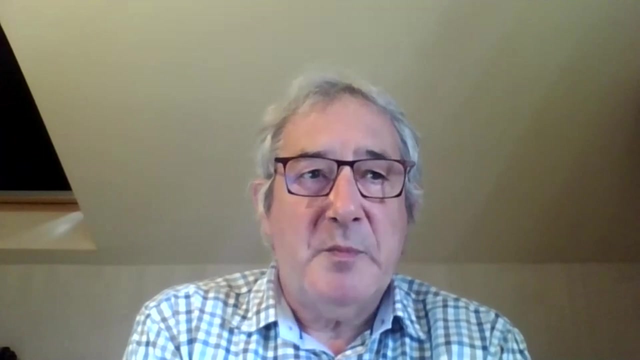 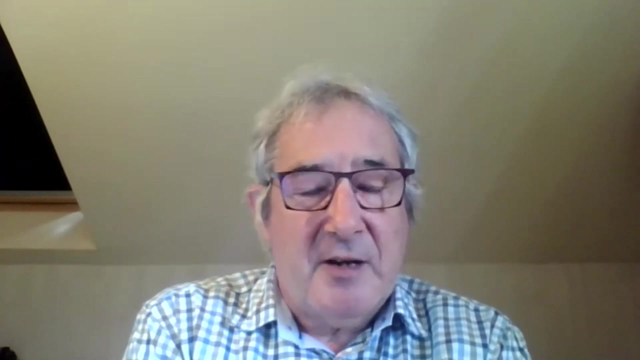 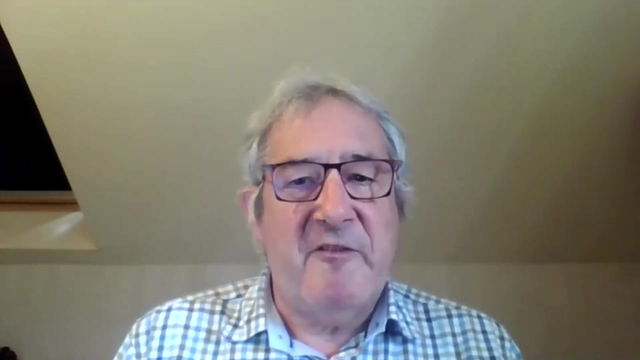 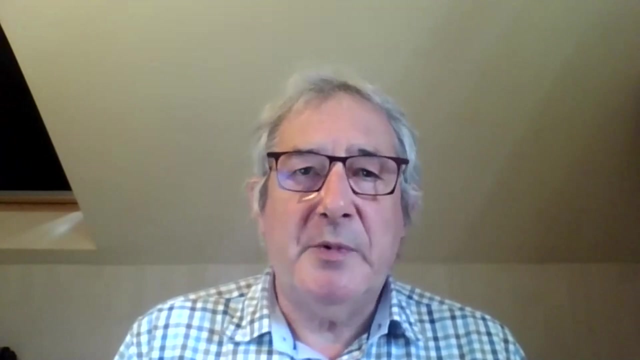 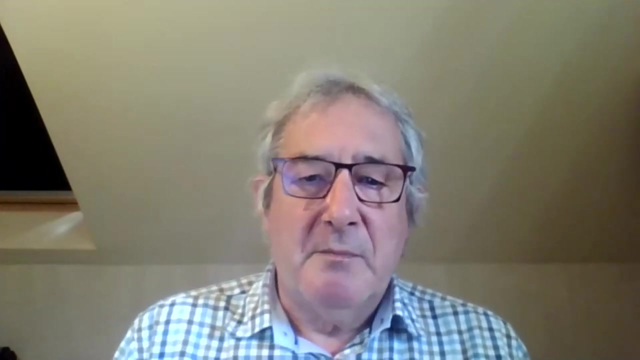 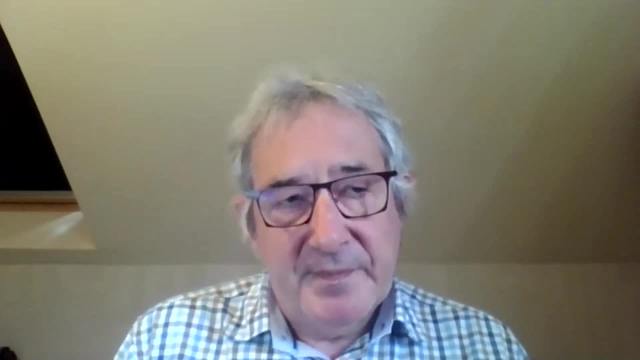 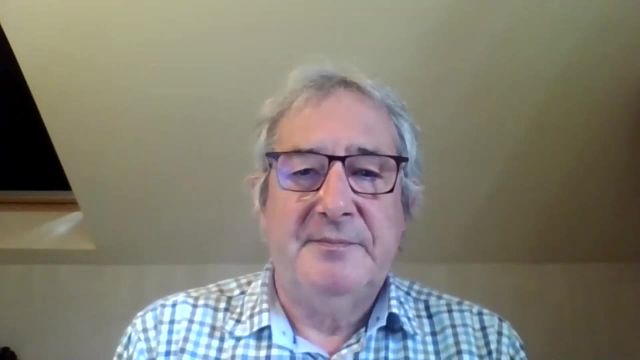 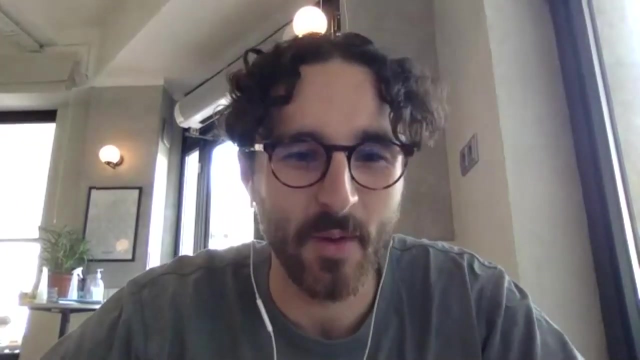 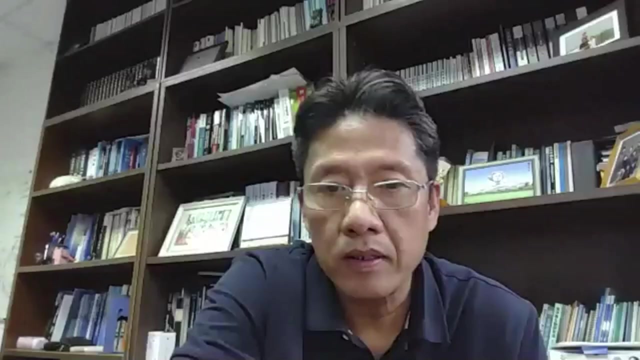 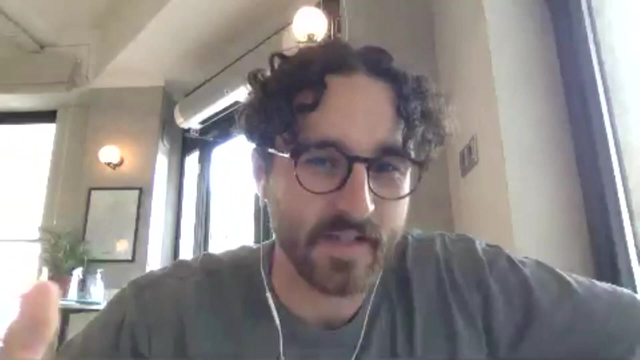 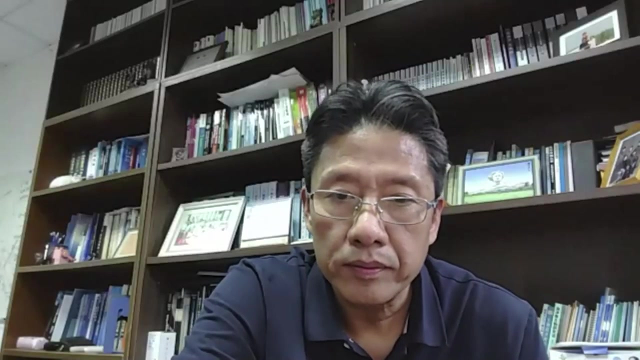 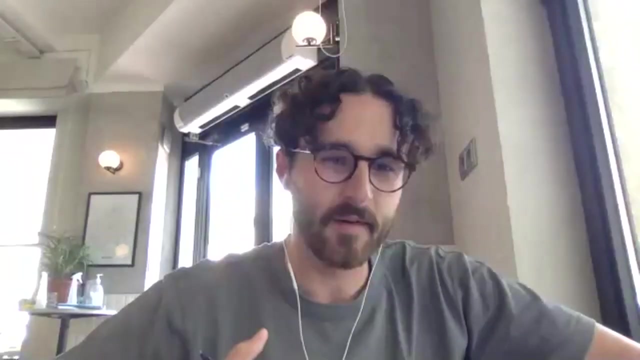 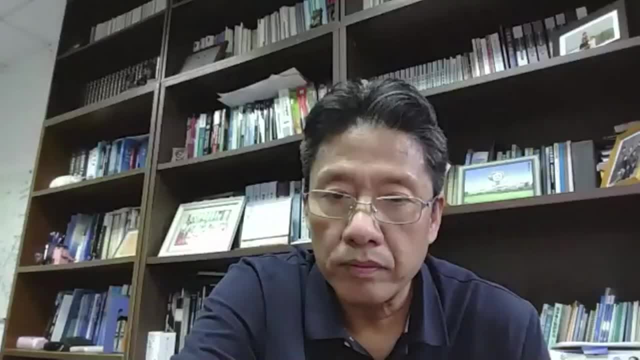 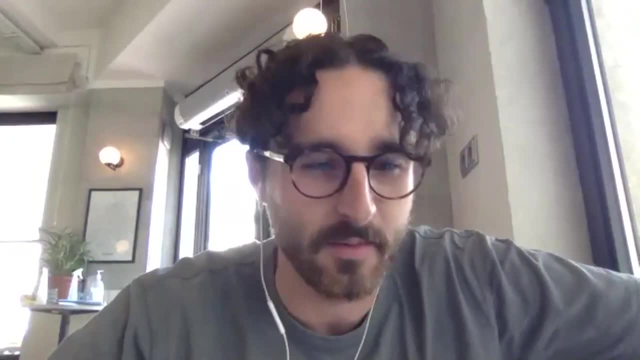 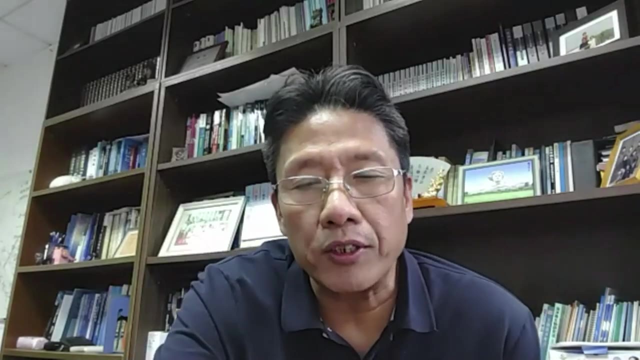 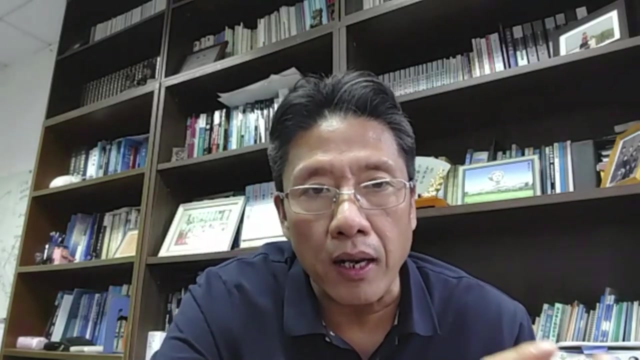 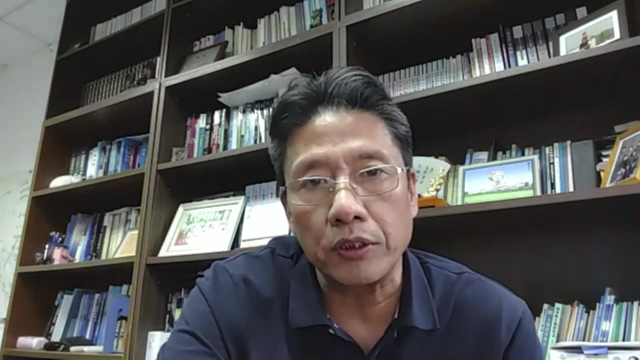 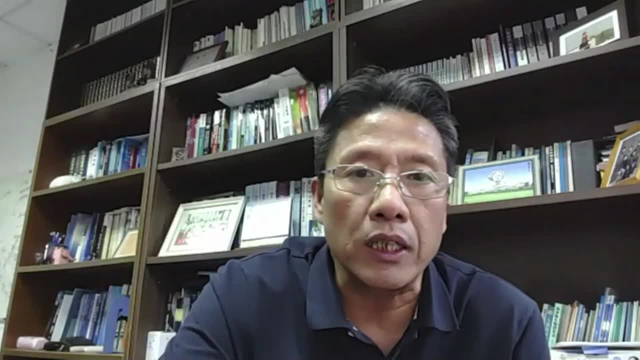 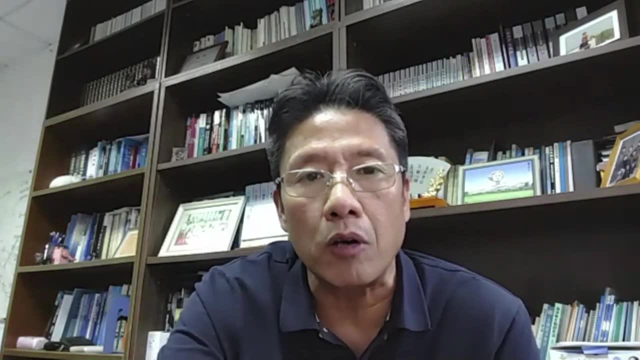 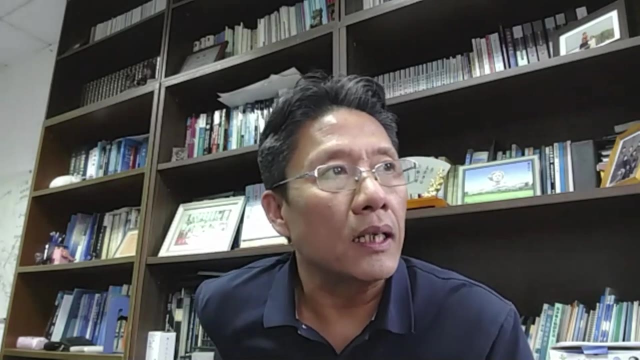 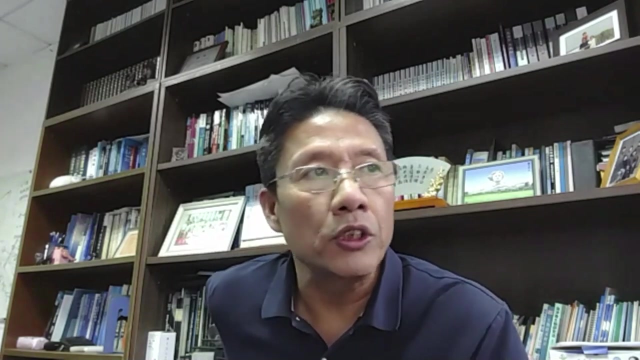 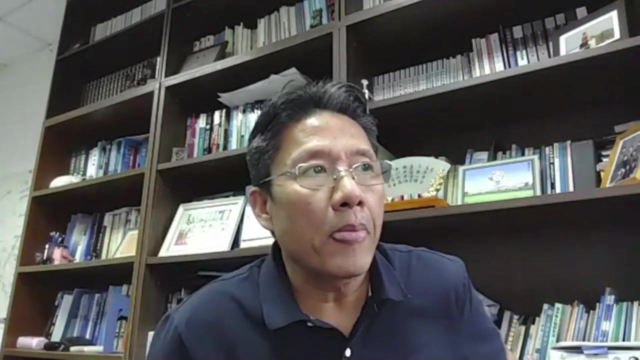 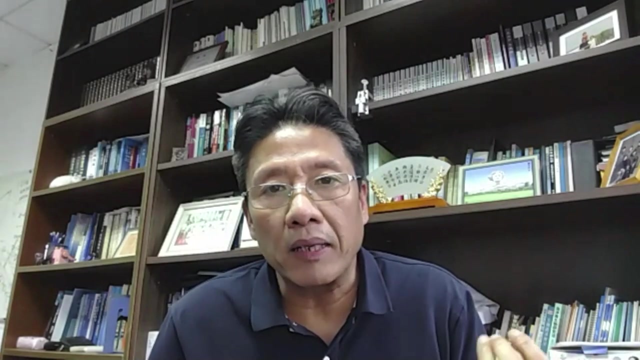 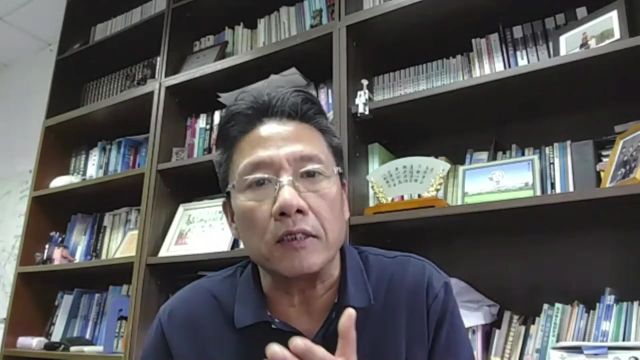 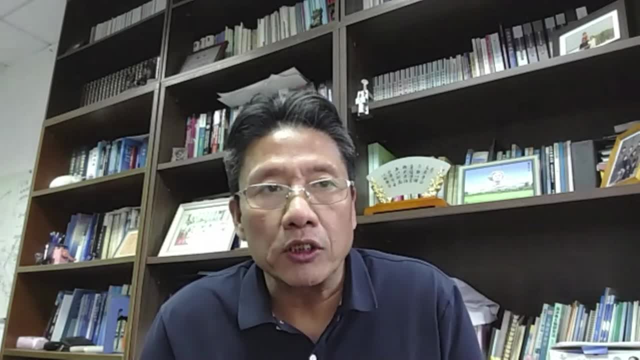 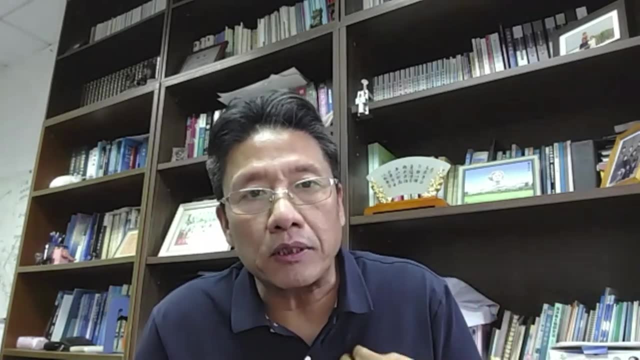 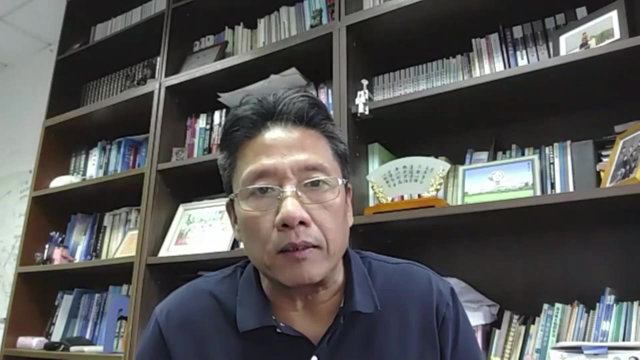 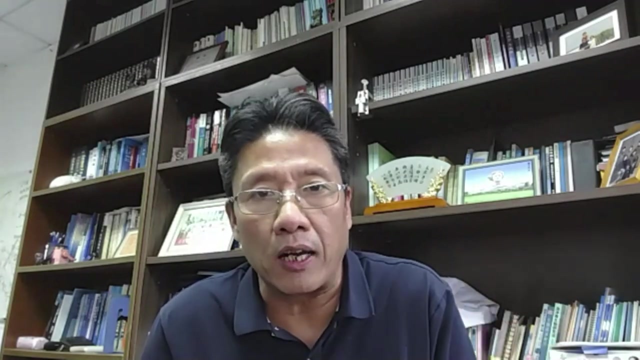 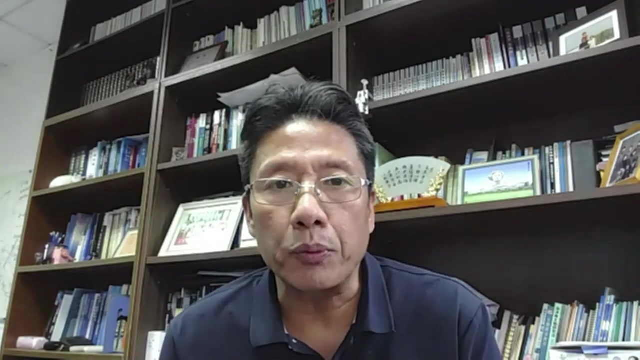 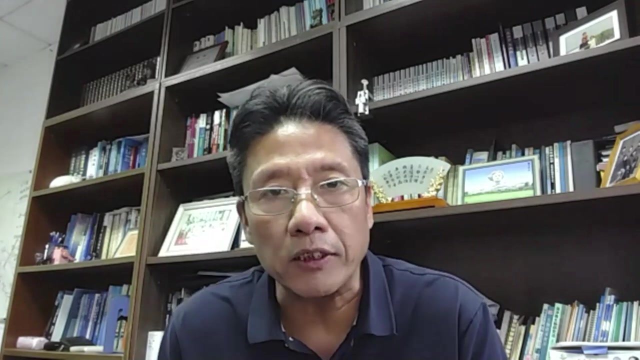 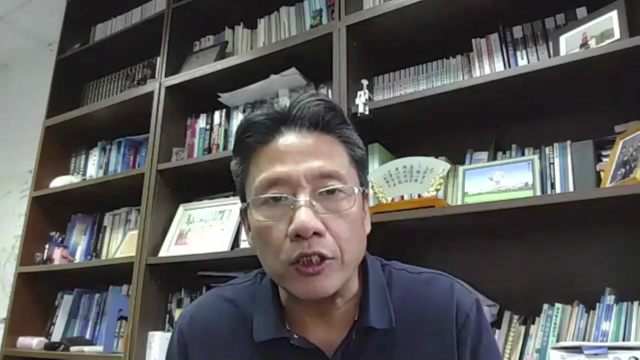 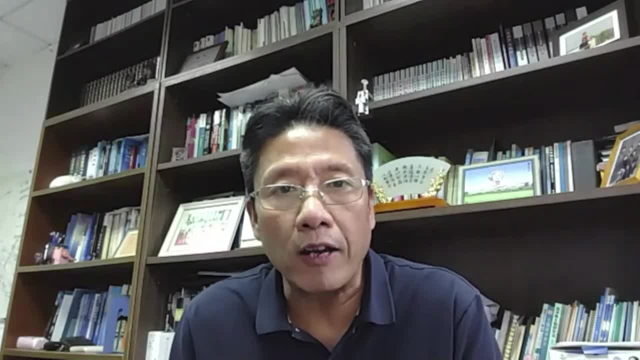 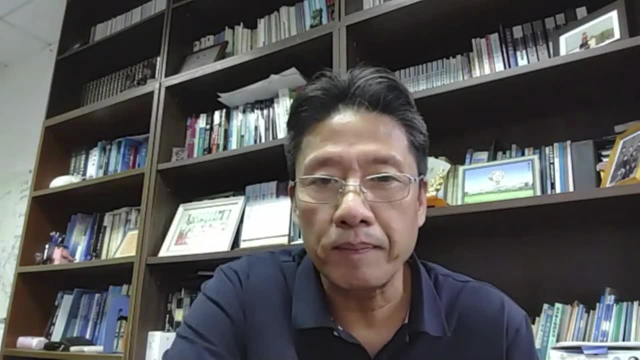 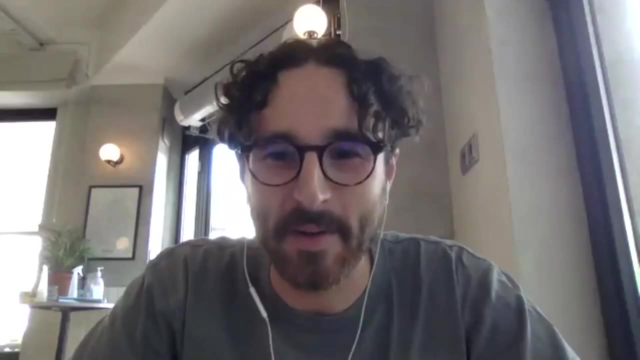 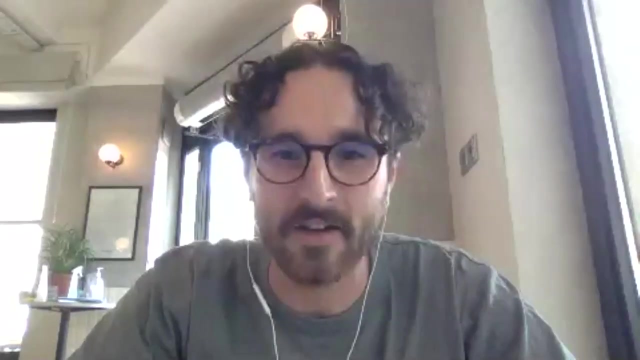 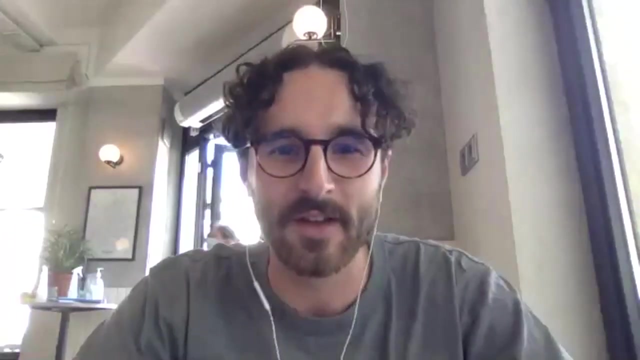 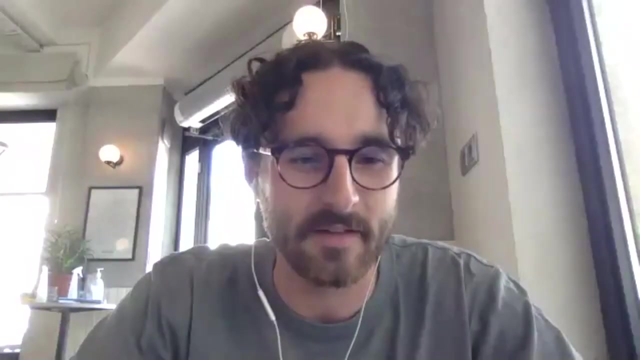 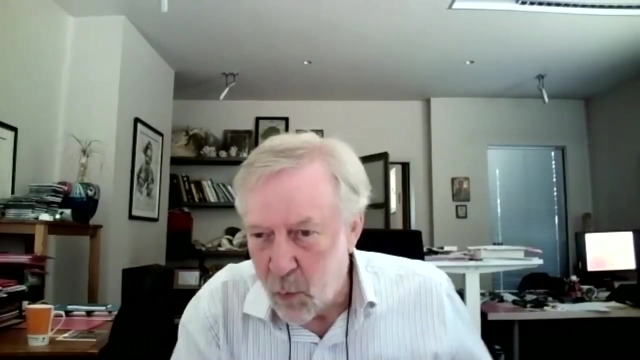 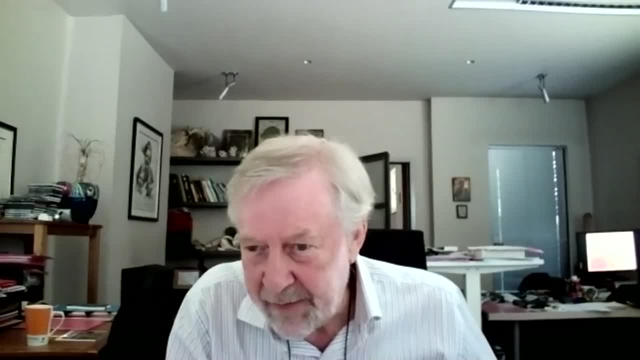 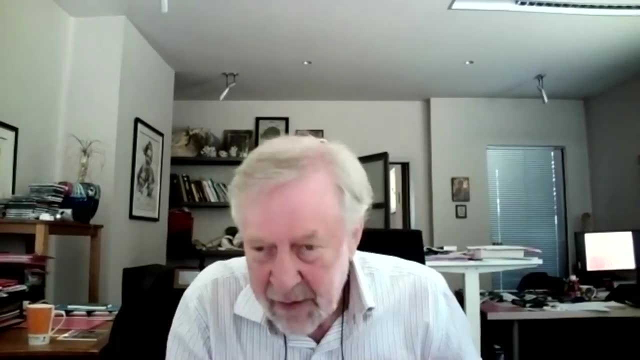 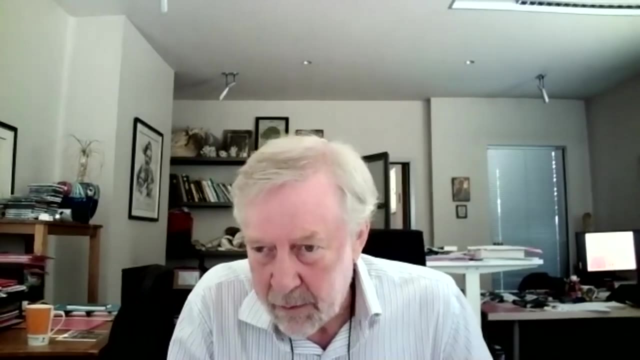 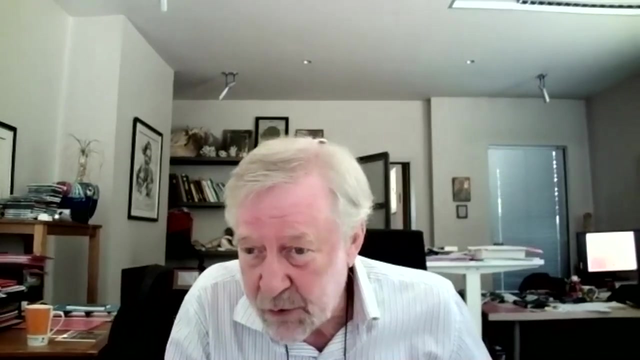 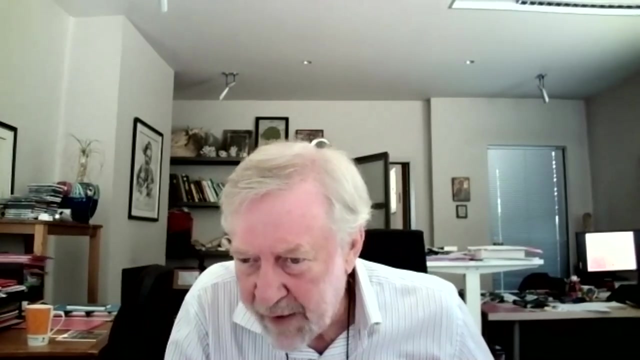 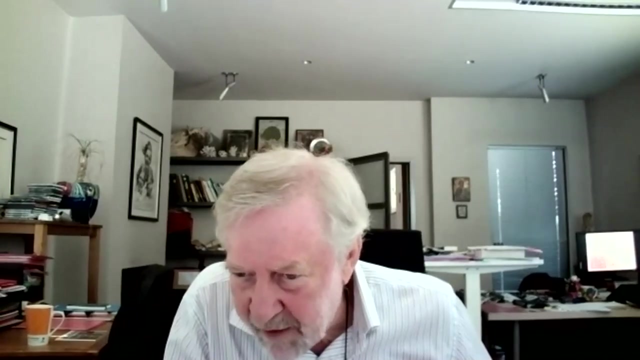 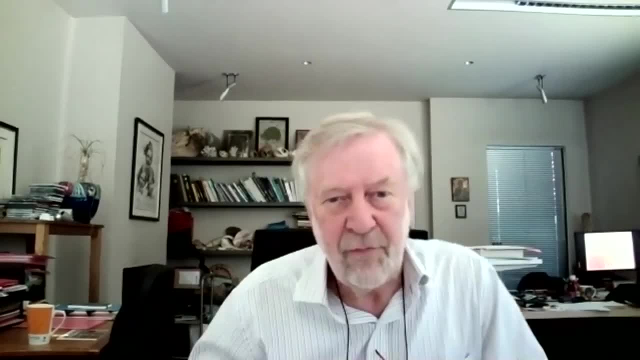 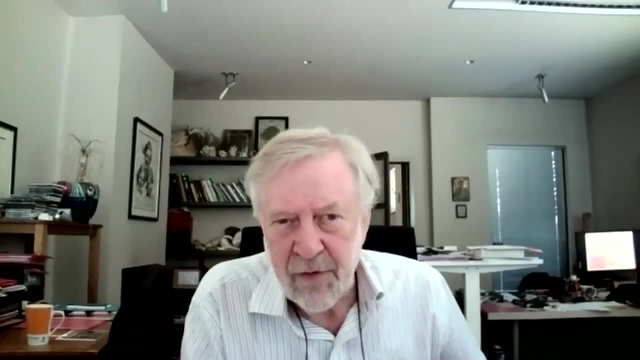 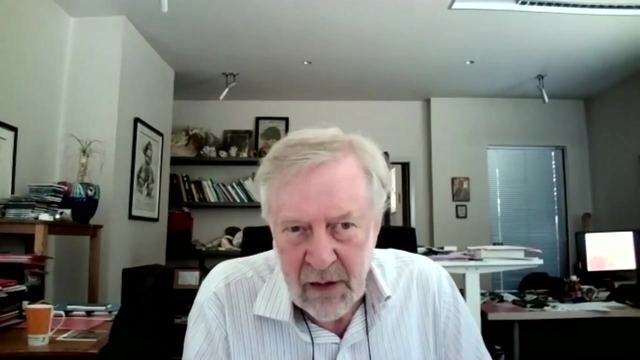 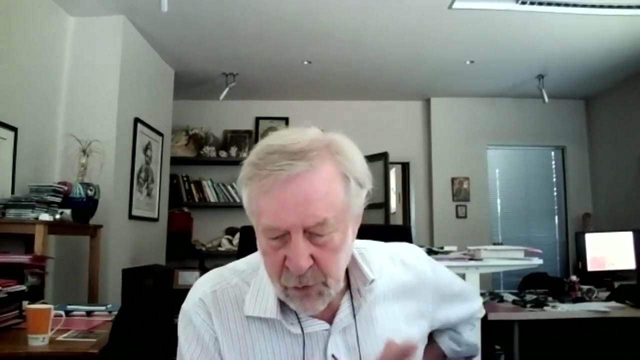 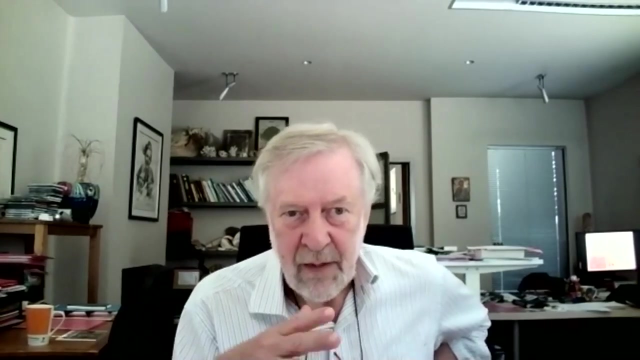 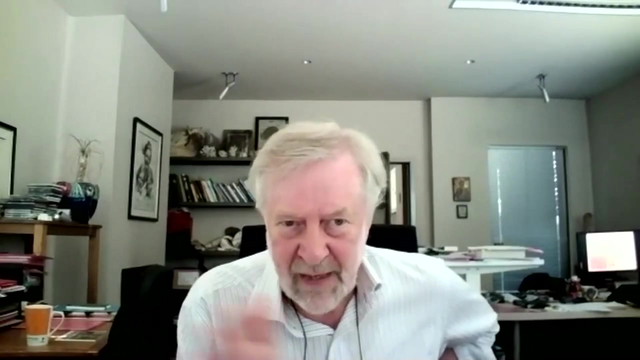 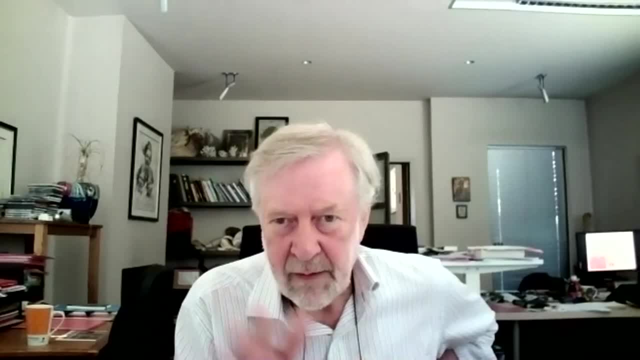 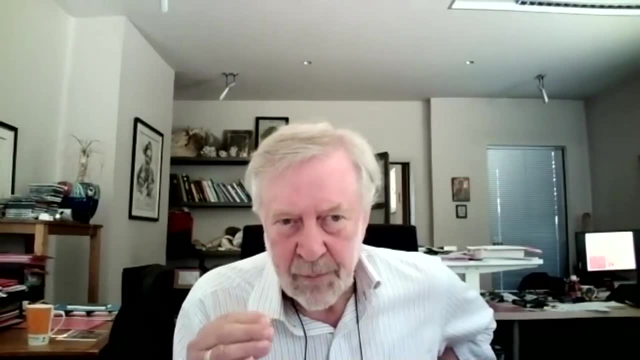 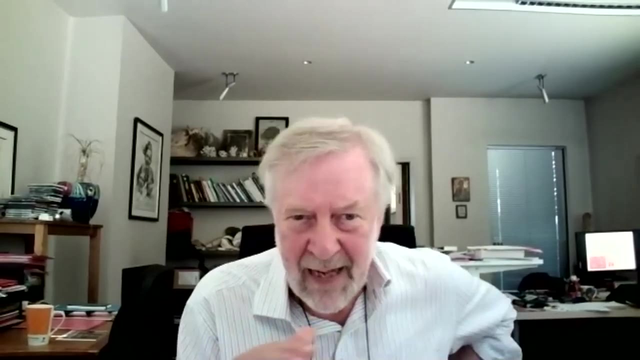 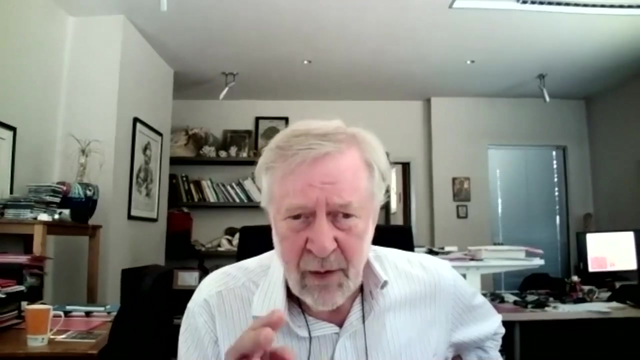 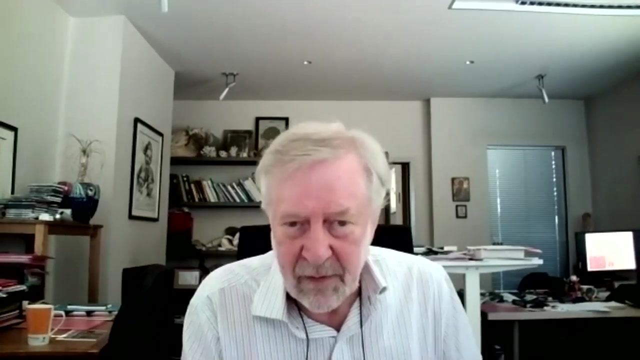 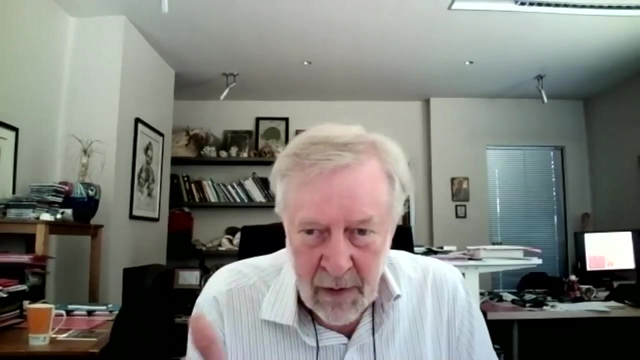 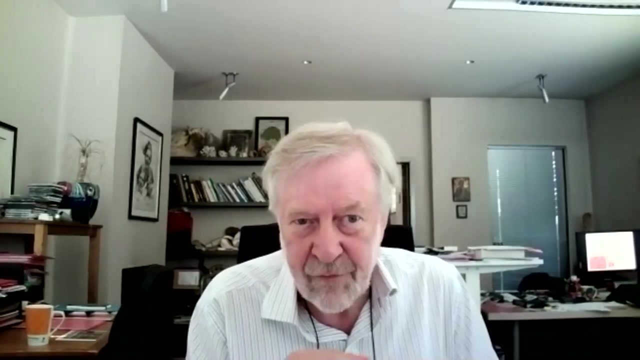 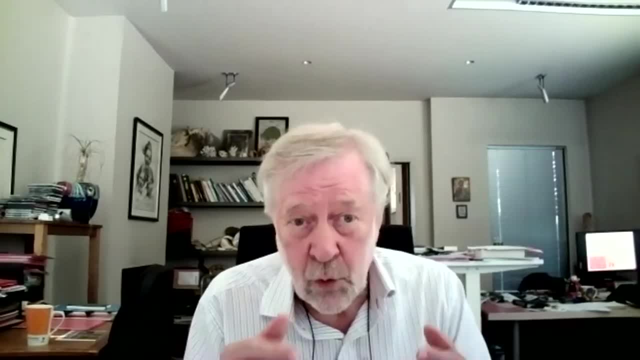 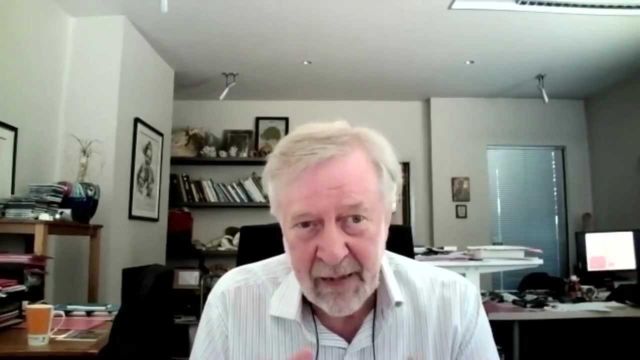 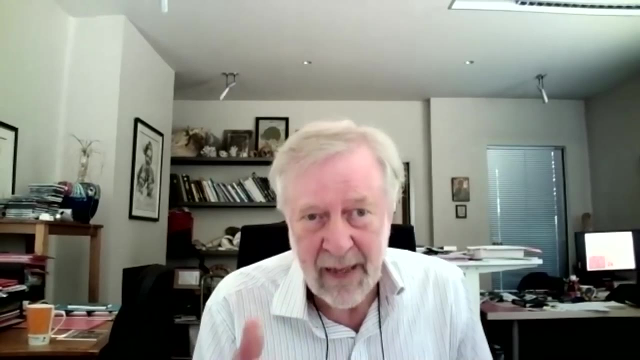 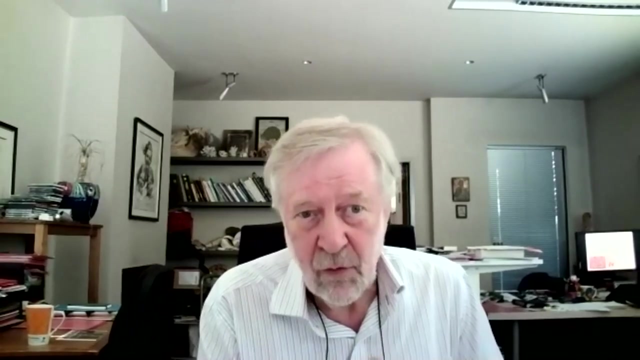 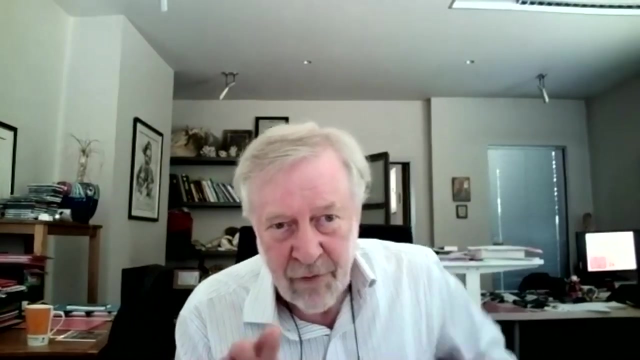 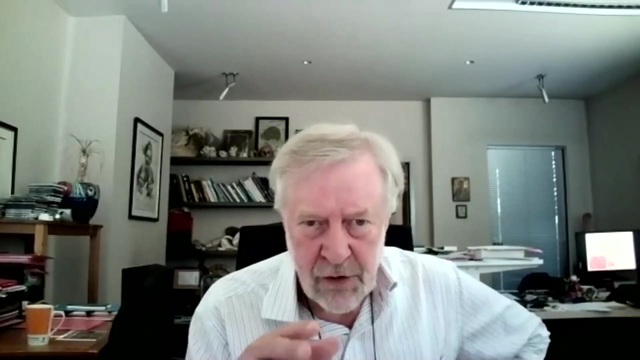 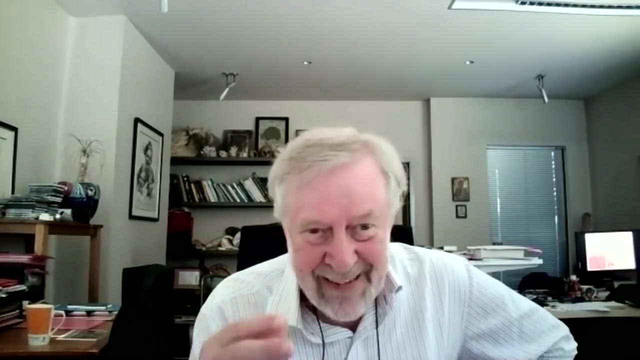 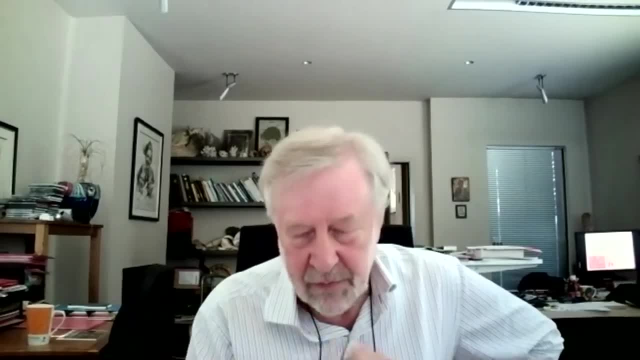 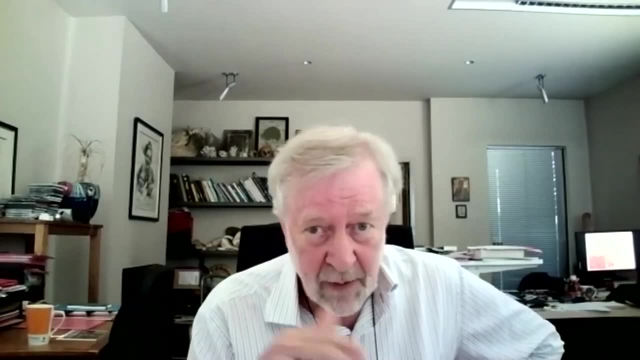 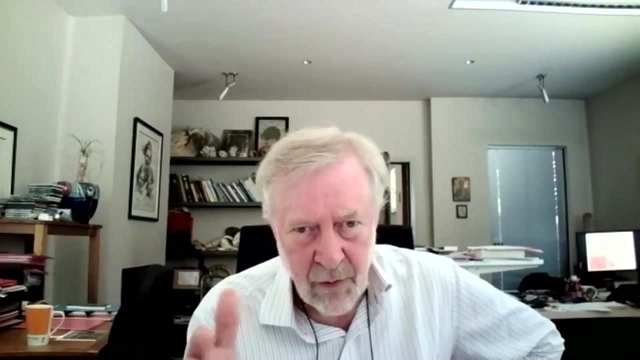 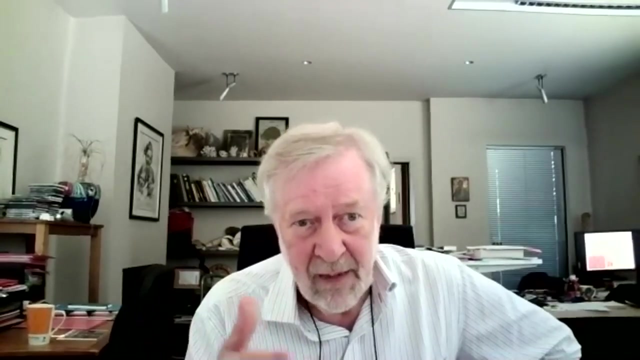 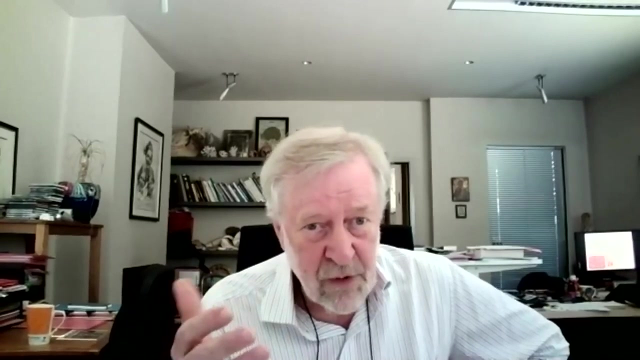 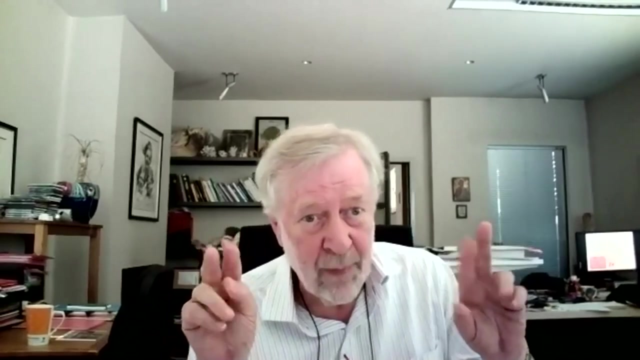 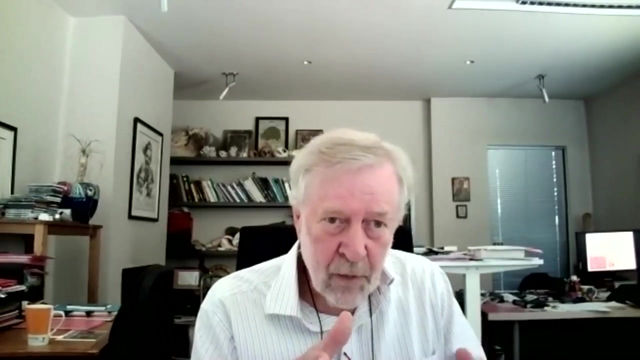